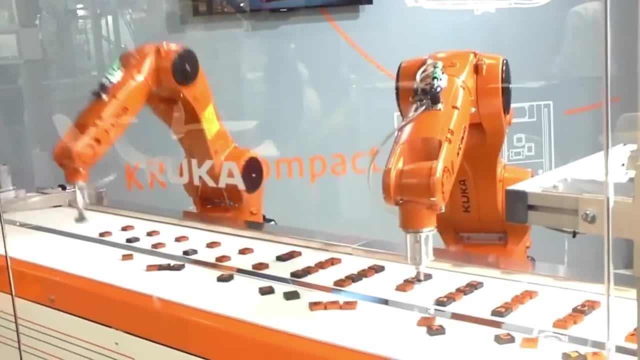 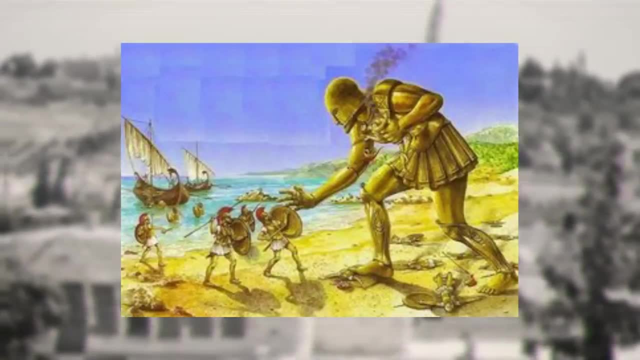 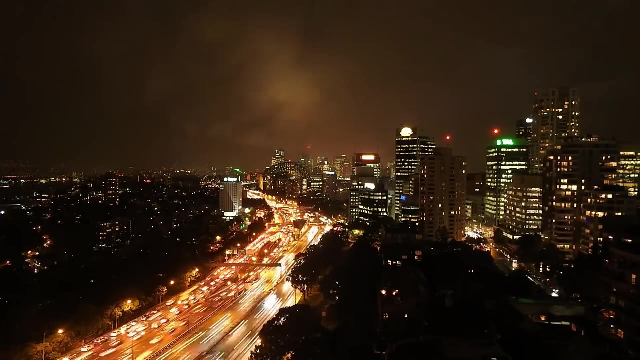 The idea of creating machines that can perform intelligent tasks dates back to ancient times. The Greek myth of Talos, a giant bronze automaton that guarded the island of Crete, is an early example of this concept. However, the modern history of AI begins in the mid-20th century, with the development of electronics. 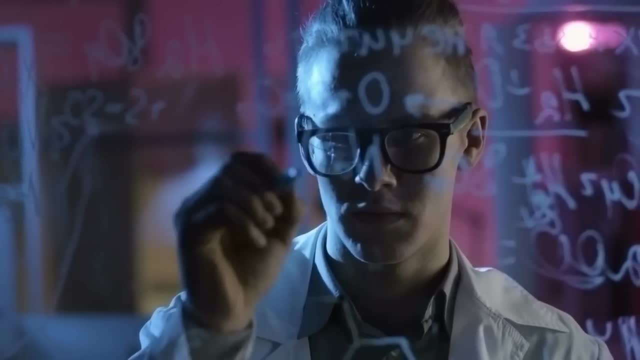 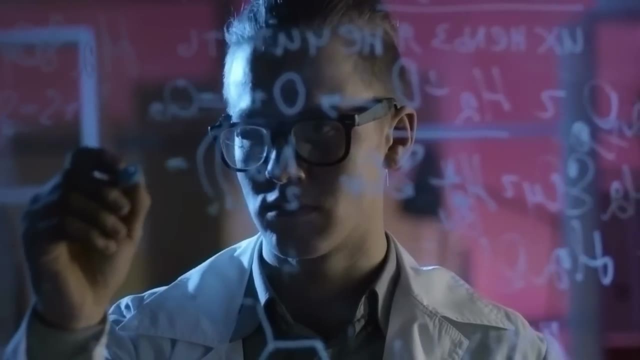 In 1950, the British mathematician and computer scientist Alan Turing proposed the Turing test, a method for determining whether a machine can exhibit intelligent behavior that is indistinguishable from that of a human. This idea laid the foundation for the development of AI. 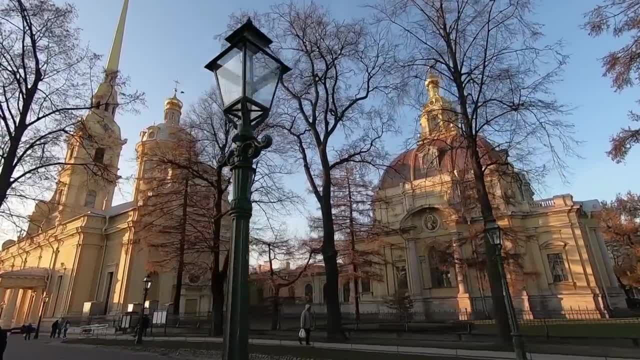 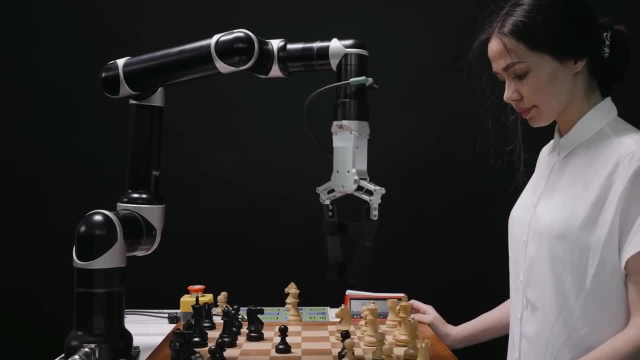 In the 1950s and 1960s, researchers began to develop algorithms and programs that could perform simple tasks such as playing chess and solving mathematical problems. The term artificial intelligence was first used in the United States as a tool for developing AI. 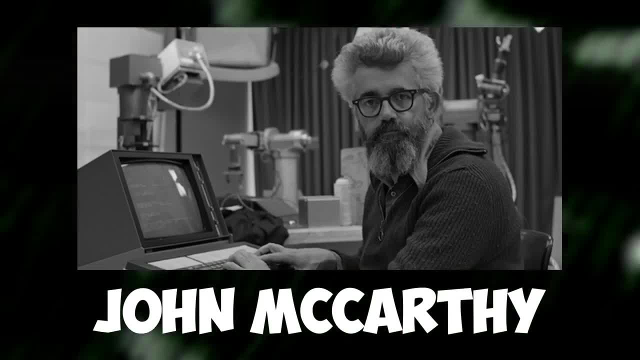 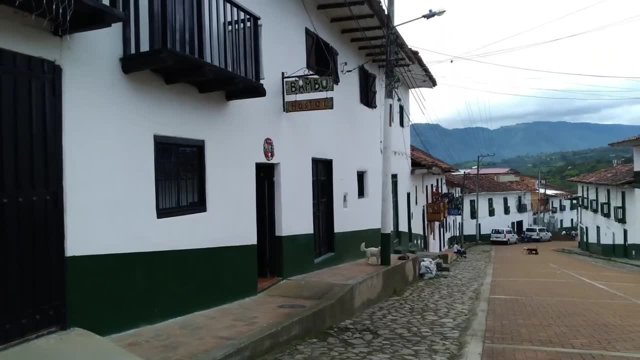 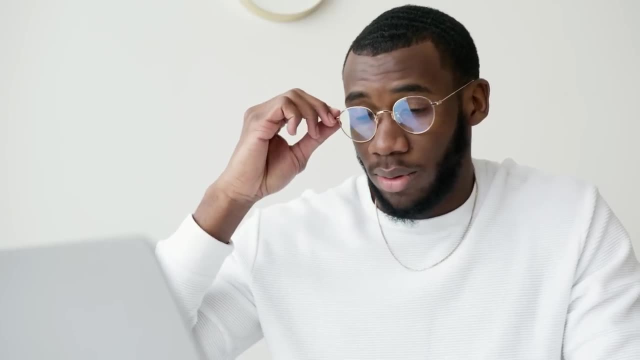 The term artificial intelligence was first used in the United States as a tool for developing AI. The term artificial intelligence was coined in 1956 by John McCarthy, Marvin Minsky, Nathaniel Rochester and Claude Shannon at the Dartmouth Conference. This is located in the third, fourth everyday image of NASA, and the scientists are now 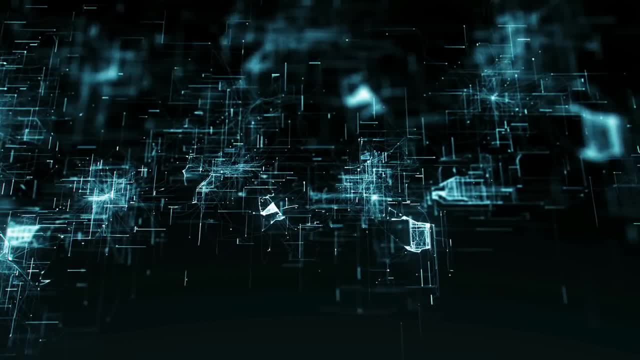 in theNIBC project of the AI research. AI research, the credentialing package defense system, the capability tofrei to bomb ΜF- народ disco principal- was coined in 1956 by John McCarthy, Marvin Minsky, Nathanael Rochester and Claude Shannon at the Dartmouth conference. 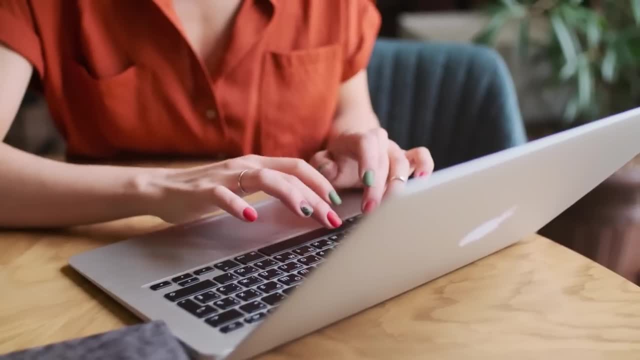 During the 1970s and 1980s, AI research faced setbacks due to technical limitations and unrealistic expectations. However, the development of expert systems, which are computer programs that can simulate the decision-making ability of a human expert in a specific field, 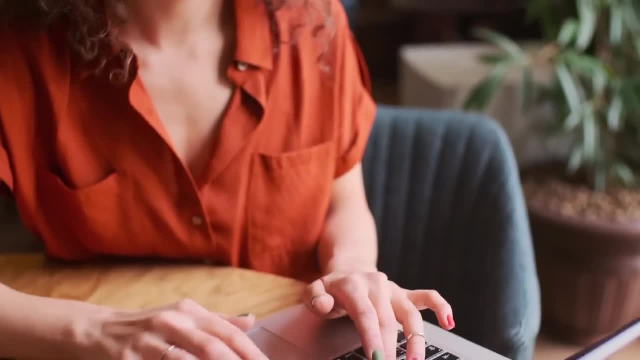 renewed interest in AI research during the 1990s and 2000s in such частwo dalam sulphaults, erscholl. advances in computing power and data storage capacity led to the development of machine learning, a technique that allows machines to learn from experience and improve their 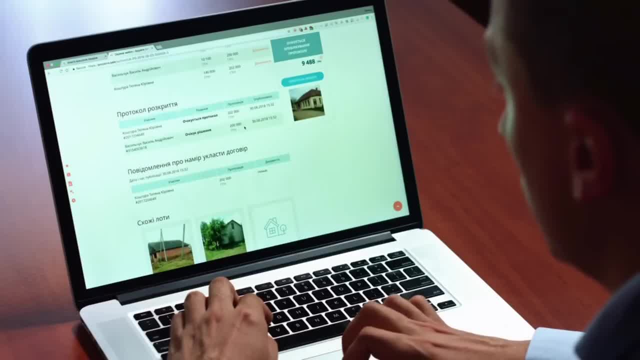 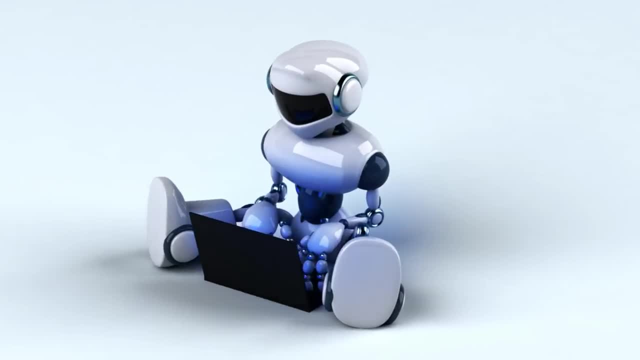 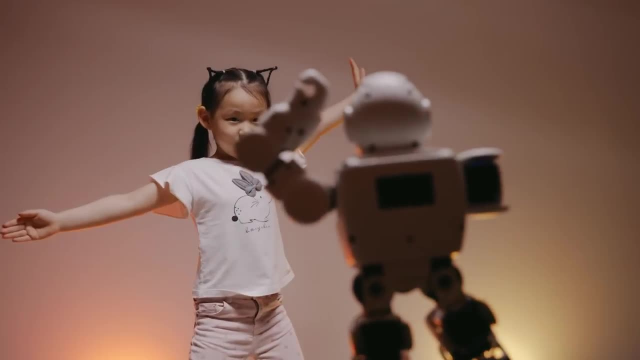 performance. over time, This led to significant advancements in areas such as speech recognition, natural language processing and computer vision. In recent years, deep learning- a type of machine learning that uses artificial neural networks to simulate the structure and function of the human brain- has revolutionized the field of AI. Deep learning has led to 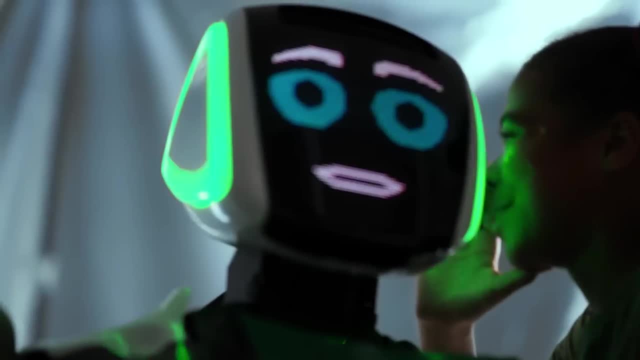 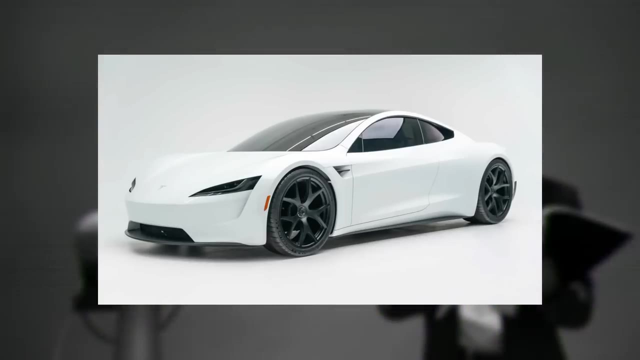 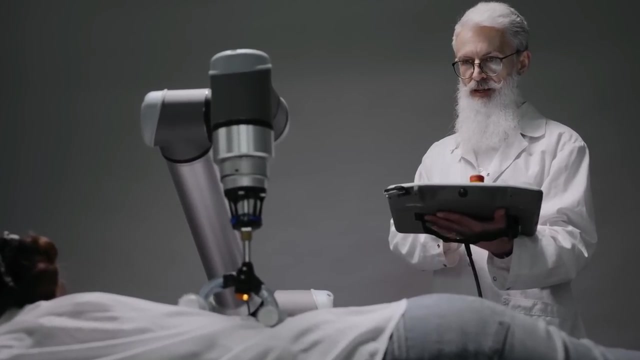 breakthroughs in areas such as image and speech recognition, natural language processing and robotics. Today, AI is used in a wide range of applications, including self-driving cars, virtual personal assistance and medical diagnosis. It is expected to continue to have a significant impact on many aspects of society in the future. Before going deeper, 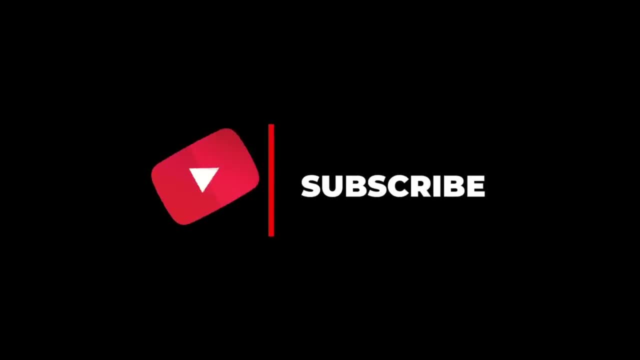 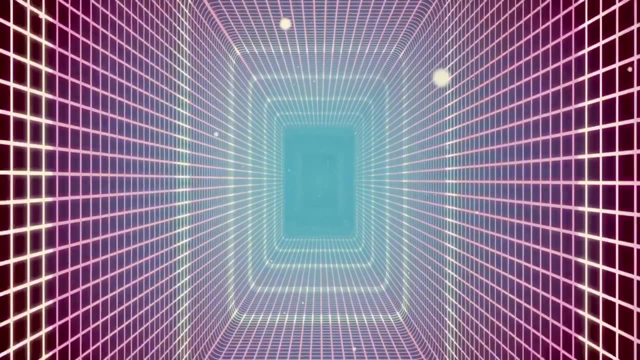 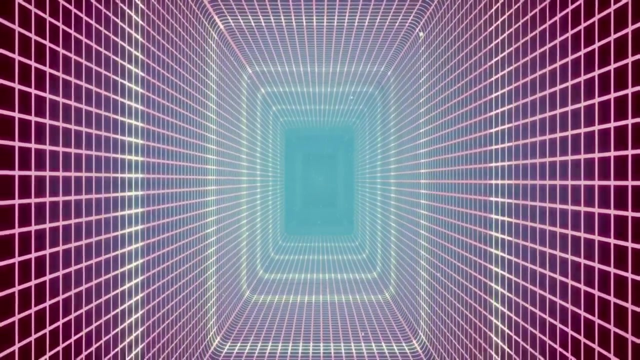 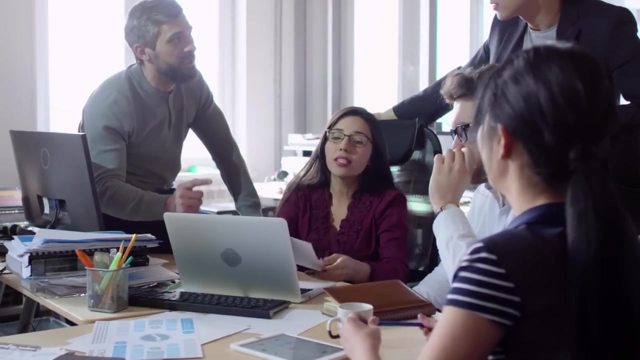 make sure to subscribe to our channel. AI can be classified into different types based on their capabilities and functions. The three main types of AI are as follows. Narrow or weak AI is designed to perform a specific task or set of tasks. This type of AI is trained on a limited dataset and performs 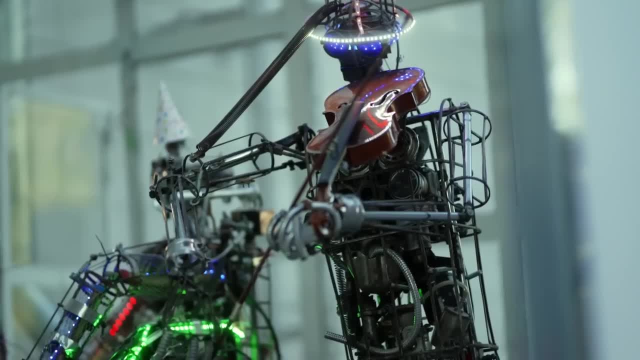 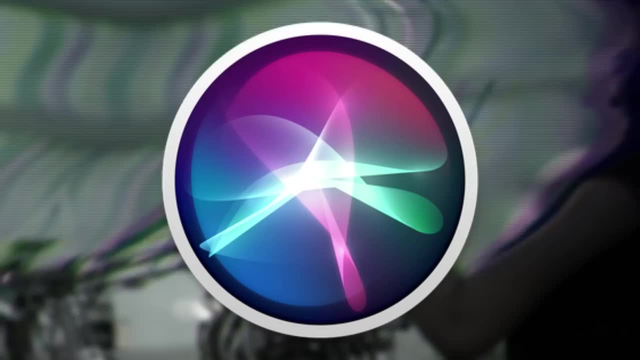 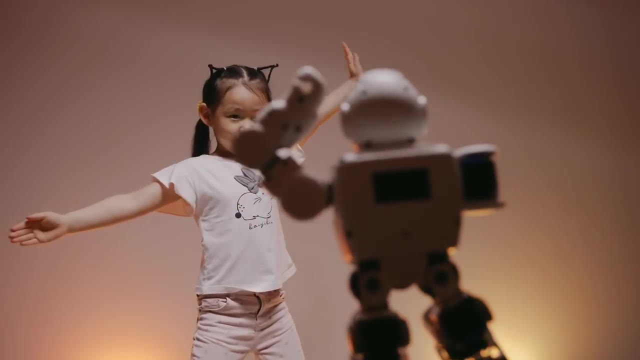 well only in the specific domain it was designed for. Examples of narrow or weak AI include image and speech recognition, language translation and virtual personal assistance like Siri and Alexa. General or strong AI. General or strong AI is designed to perform any intellectual task that. 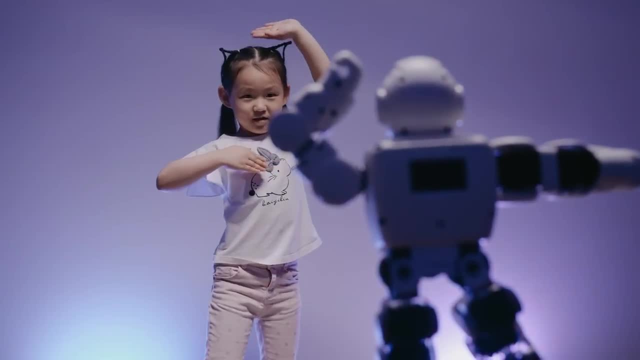 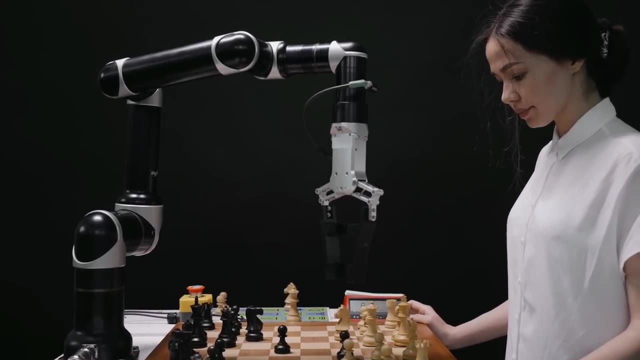 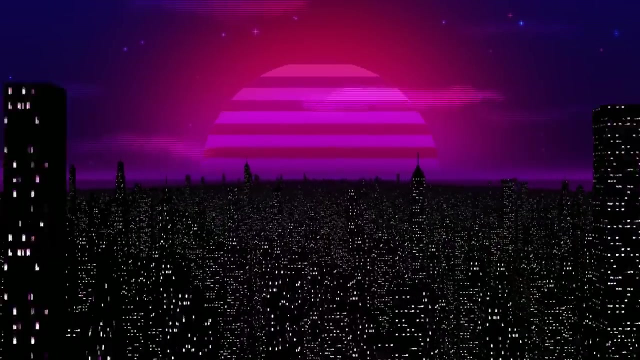 a human can do. This type of AI has the ability to reason, learn and adapt to new situations. General or strong AI does not exist yet and is a goal for future AI development: Artificial superintelligence. Artificial superintelligence is an extension of general or strong AI. It is an AI system that 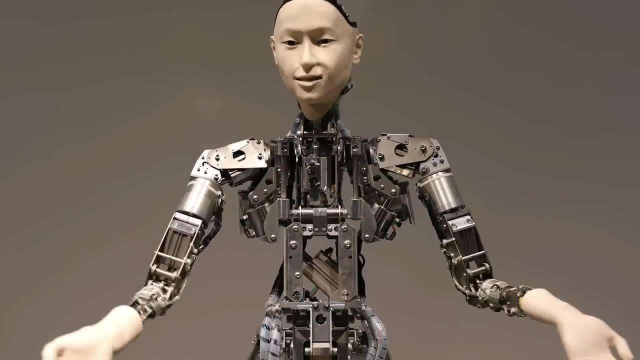 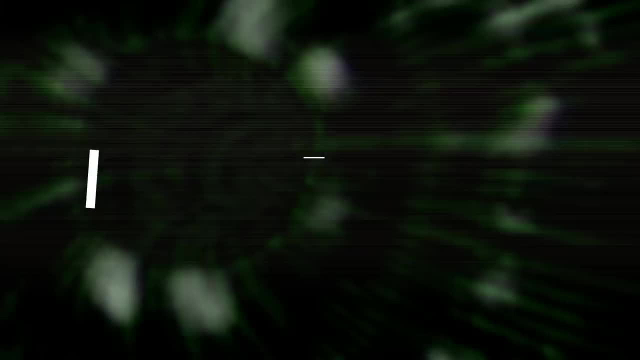 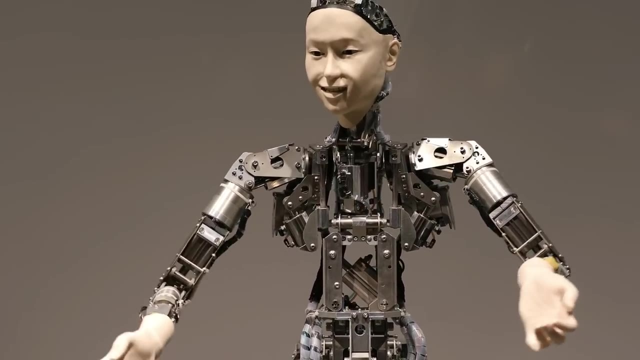 surpasses human intelligence in every possible way. Artificial superintelligence does not exist yet, but it is a theoretical concept that has gained attention in recent years. Artificial intelligence is being used in various applications to improve efficiency, accuracy and decision-making. Some of the key applications of AI are as follows. 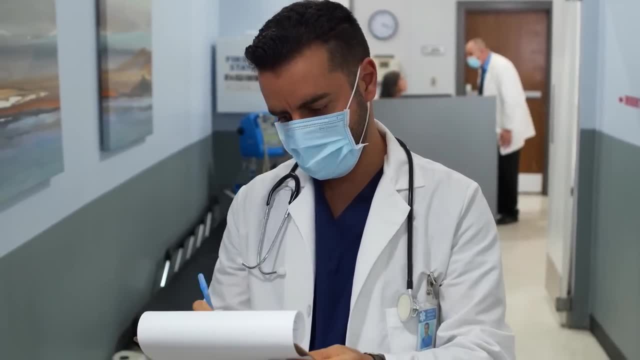 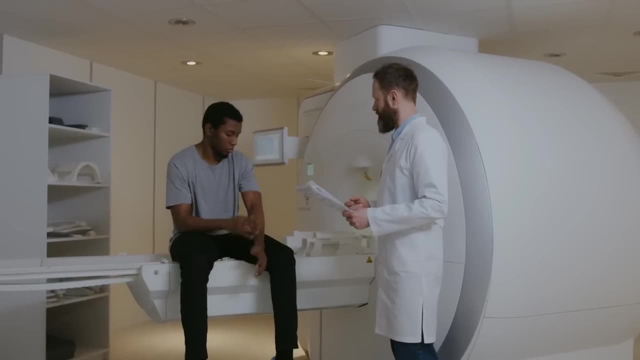 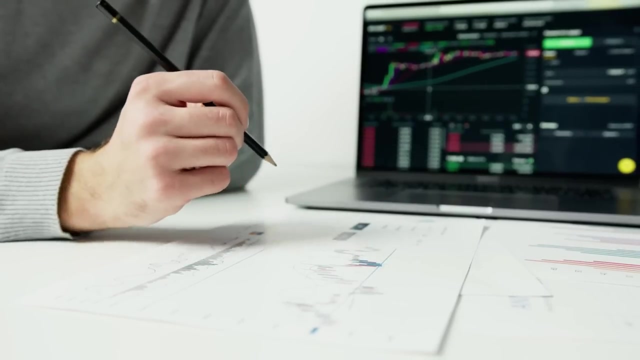 Healthcare: AI is being used in healthcare to improve patient outcomes and reduce costs. AI-powered systems can help doctors diagnose diseases, personalize treatments and monitor patients remotely. Finance AI is being used in finance to detect fraud, manage risk and automate customer service. 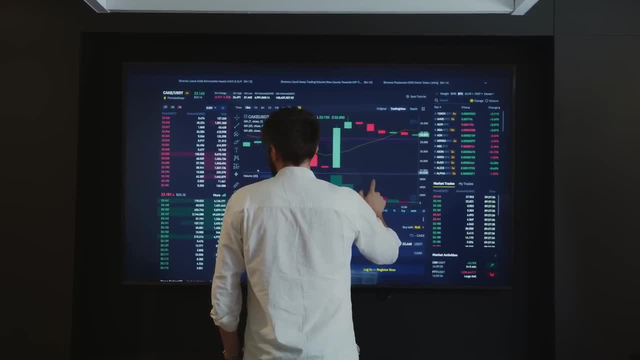 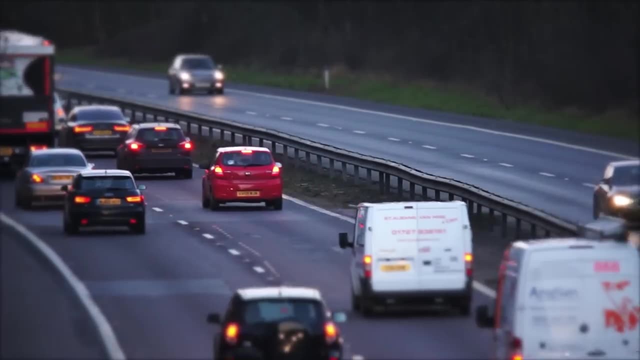 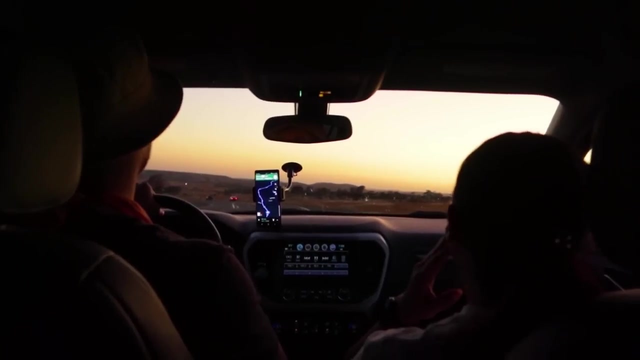 AI-powered chatbots are being used by financial institutions to provide personalized assistance to customers. Transportation: AI is being used in transportation to improve safety, efficiency and sustainability. Self-driving cars use AI to navigate roads, avoid obstacles and make decisions in real time. Education: AI is being used in education to personalize learning. 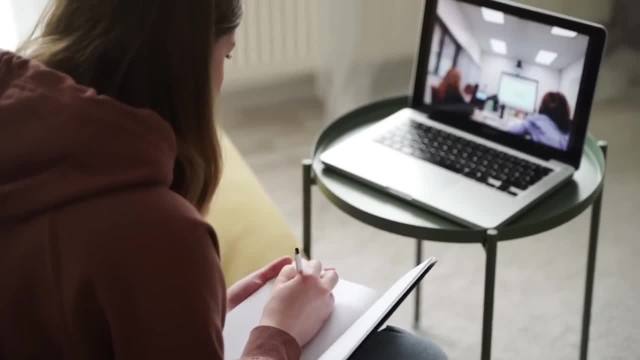 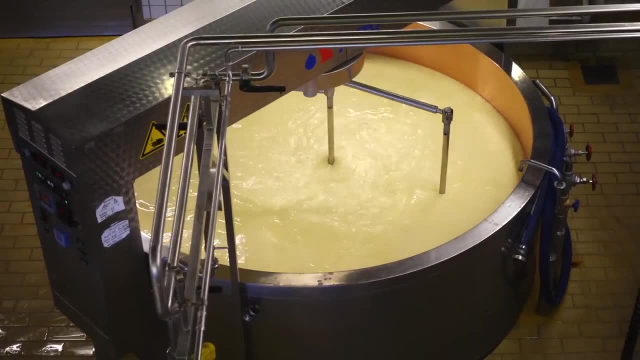 and improve student outcomes. AI-powered tutoring systems can adapt to the individual needs of students and provide feedback to teachers. Manufacturing AI is being used in manufacturing to improve productivity, quality and safety. AI-powered robots are being used in manufacturing to improve productivity, quality and safety. 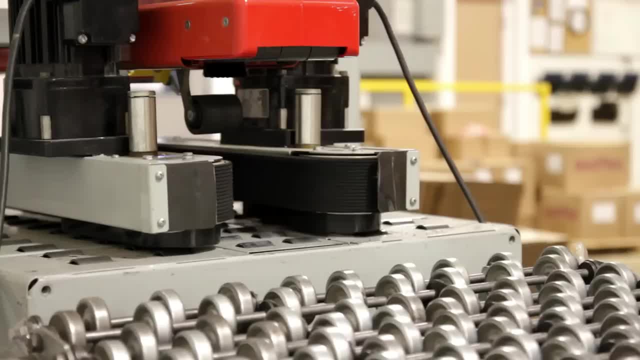 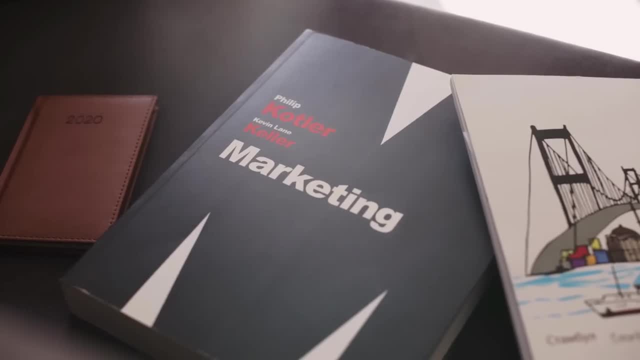 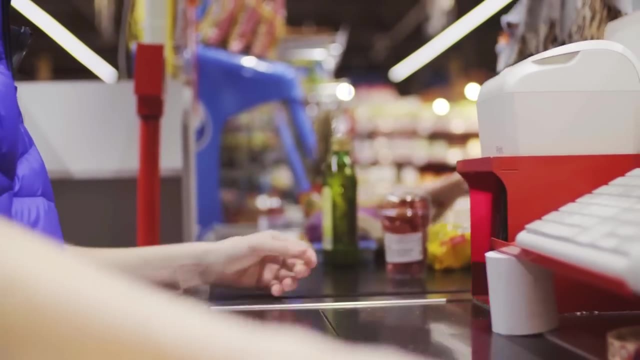 AI-powered robots are being used to perform tasks such as assembly, welding and inspection. Retail: AI is being used in retail to improve customer experience and increase sales. AI-powered systems can analyze customer data to provide personalized recommendations and improve inventory management. Agriculture: AI is being used in agriculture to improve crop yields. 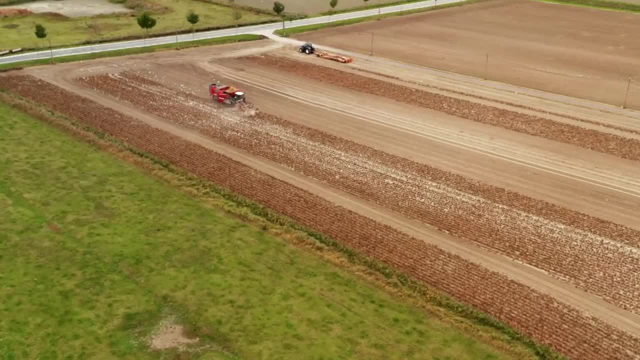 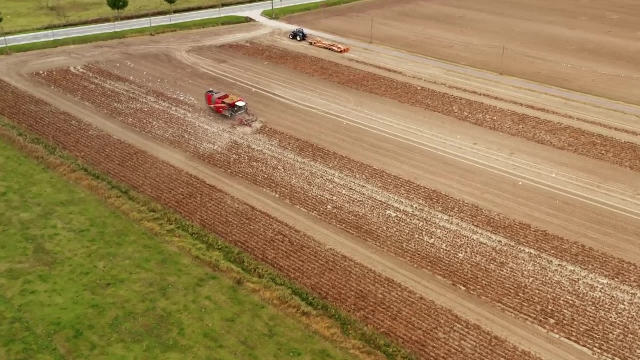 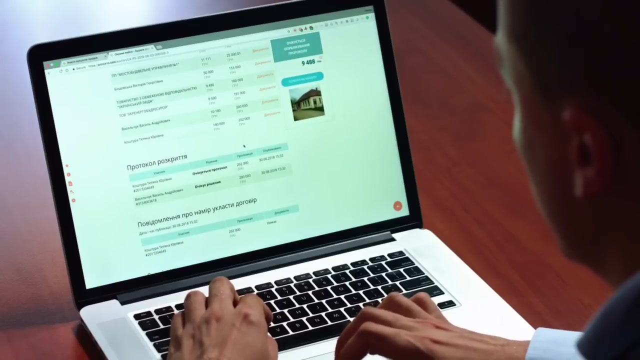 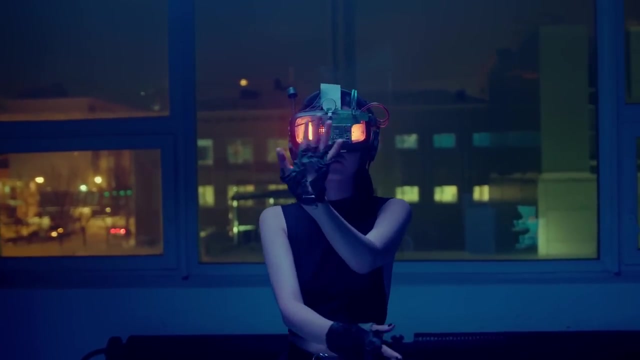 reduce waste and optimize resource usage. AI-powered systems can analyze data from sensors and drones to provide insights on soil health, crop growth and weather patterns. Artificial Intelligence AI has the potential to bring about significant benefits to society. However, it also raises ethical concerns that need to be addressed. Some of the key ethical 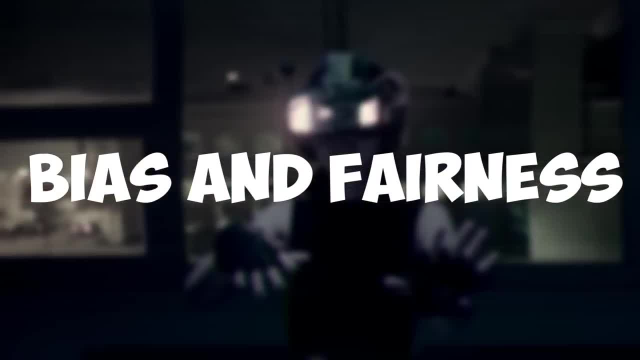 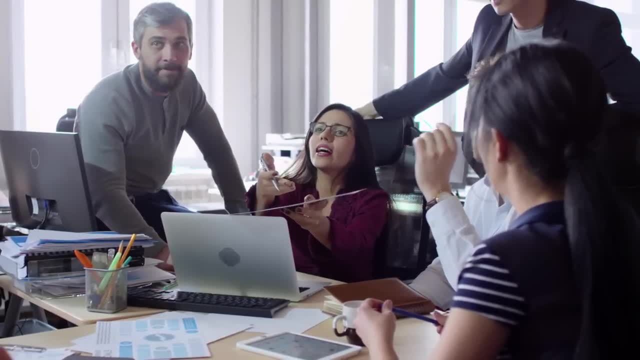 considerations related to AI are as follows: Bias and fairness. AI systems can perpetuate and amplify biases present in society, leading to unfair and unfair decisions. AI systems can fair treatment of certain groups. It is essential to ensure that AI systems are designed and 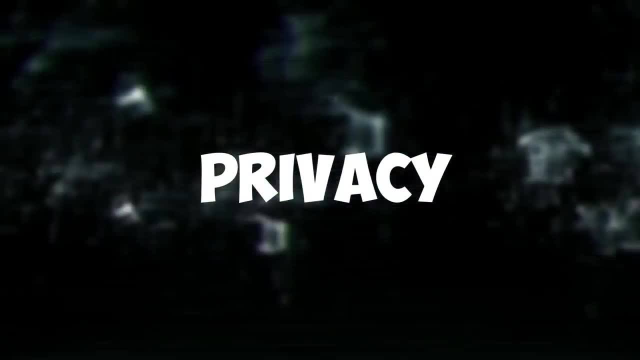 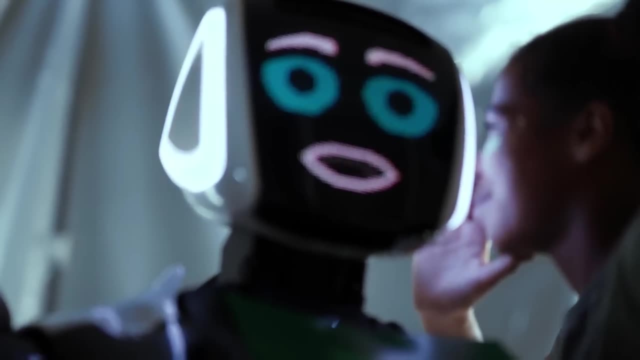 developed in a way that is fair and unbiased. Privacy. AI systems often collect and analyze vast amounts of personal data, raising concerns about privacy and data protection. It is essential to ensure that AI systems are designed and developed in a way that respects individuals'. 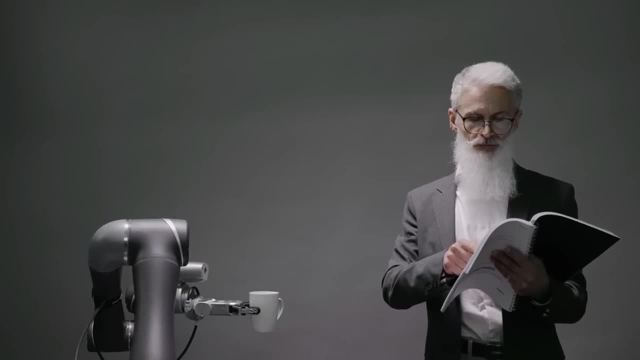 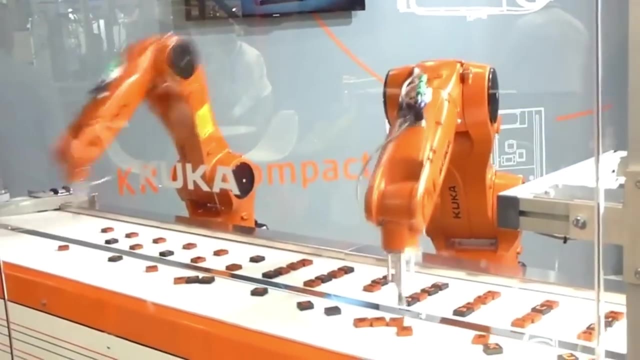 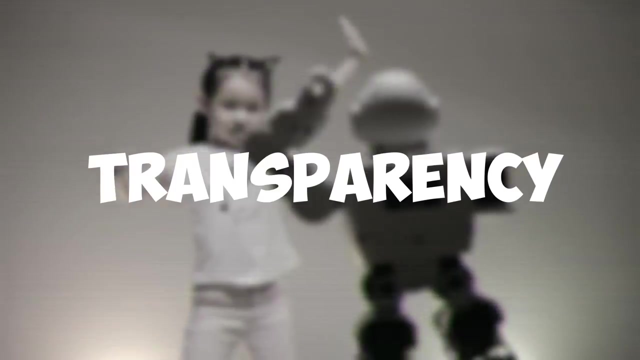 privacy rights Accountability: AI systems can make decisions that have significant consequences for individuals and society as a whole. It is essential to ensure that there is accountability for the decisions made by AI systems and that individuals can challenge and appeal those decisions. Transparency: AI systems can be complex and difficult to understand. 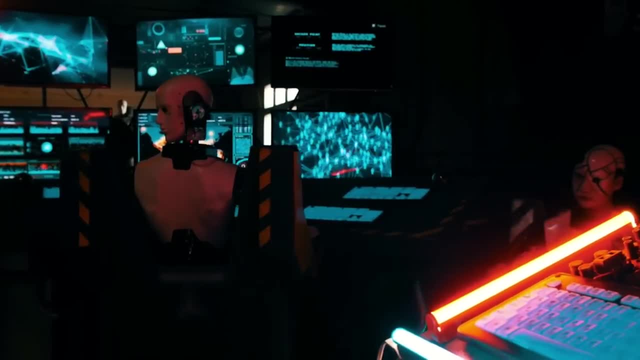 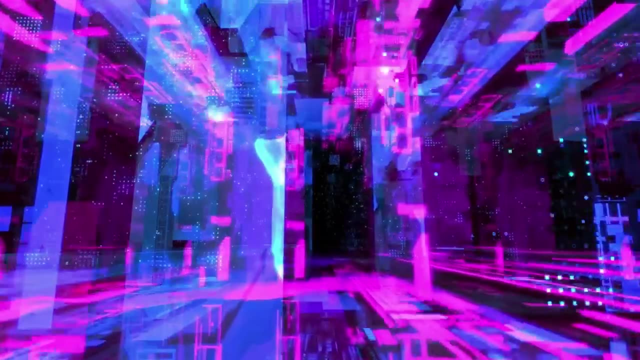 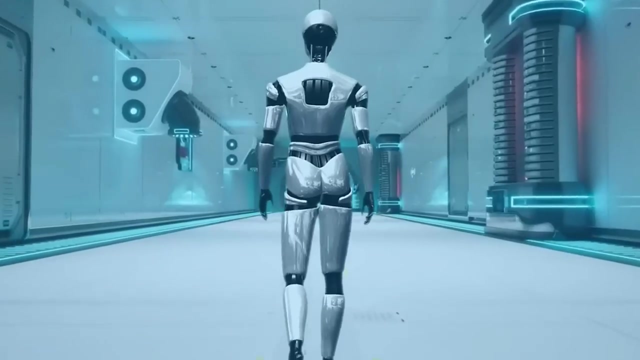 making it challenging to assess their impact and ensure accountability. It is essential to ensure that AI systems are transparent and explainable so that individuals can understand how decisions are made. Safety AI systems can have unintended consequences and pose risks to human safety. It is essential to ensure that AI systems are designed and 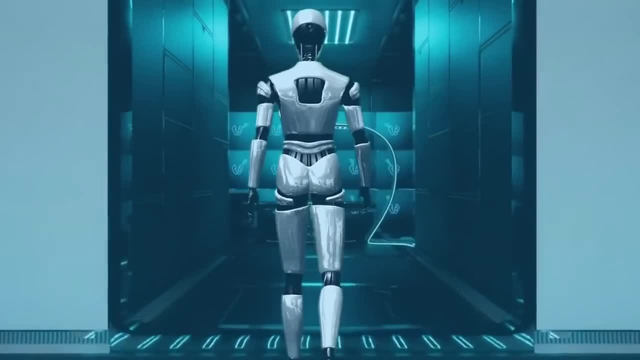 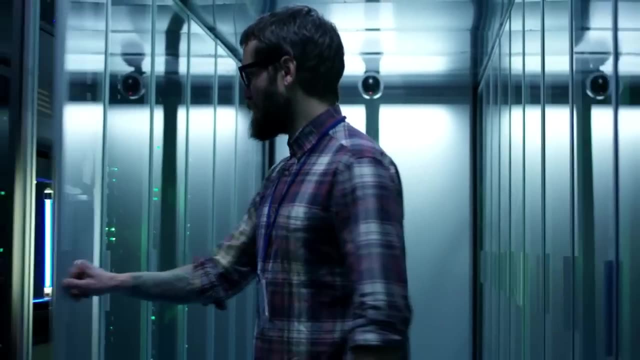 developed in a way that is safe and does not pose a threat to individuals or society. Employment AI has the potential to automate many jobs, leading to job displacement and unemployment. It is essential to ensure that AI is developed and used in a way that supports human employment. 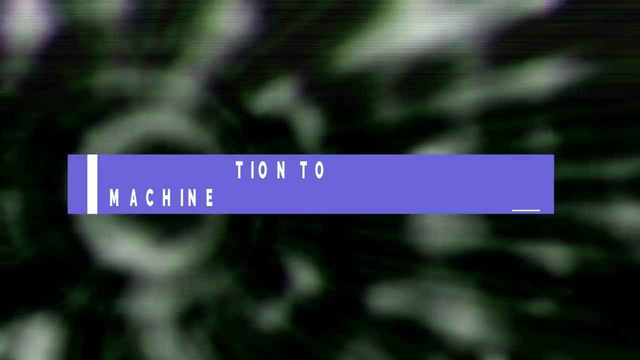 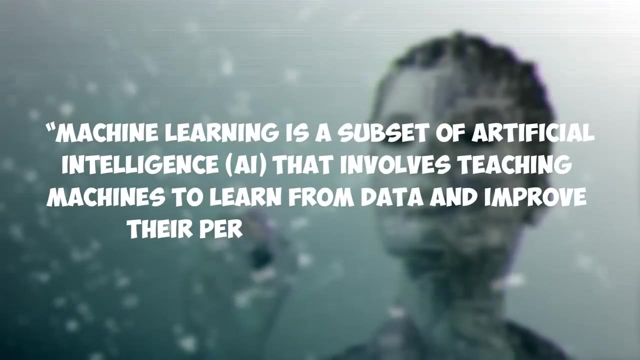 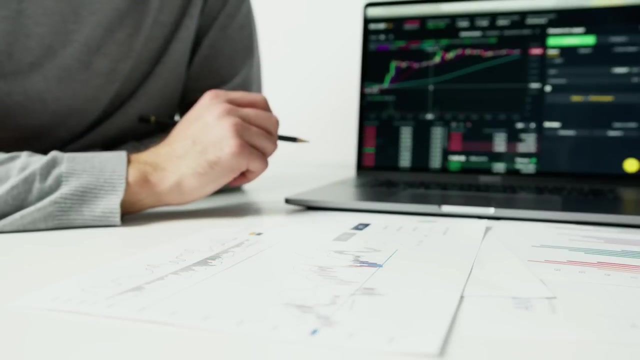 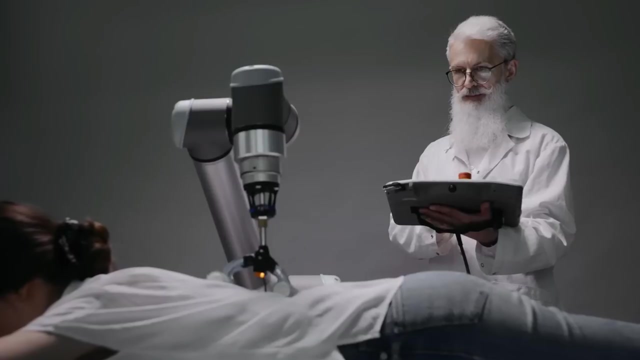 and creates new job opportunities. Machine learning: Machine learning is a set of artificial intelligence AI that involves teaching machines to learn from data and improve their performance over time. ML algorithms use statistical techniques to enable machines to identify patterns and make predictions without being explicitly programmed. There are three. 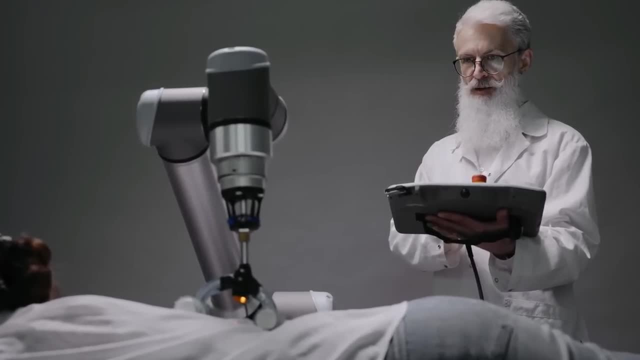 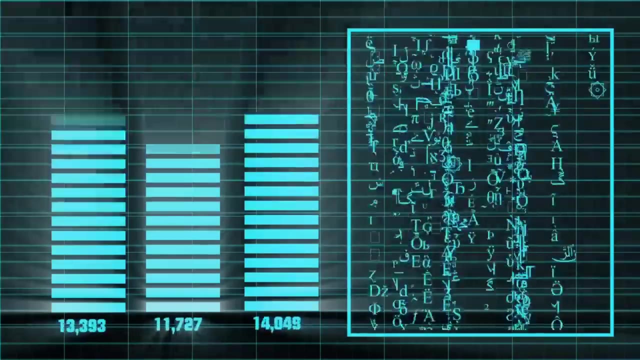 main types of ML: supervised learning, unsupervised learning and reinforcement learning. Supervised learning: In supervised learning, machines are trained on labeled data, meaning that the data is already categorized or classified. It is essential to ensure that machines are trained on labeled data. 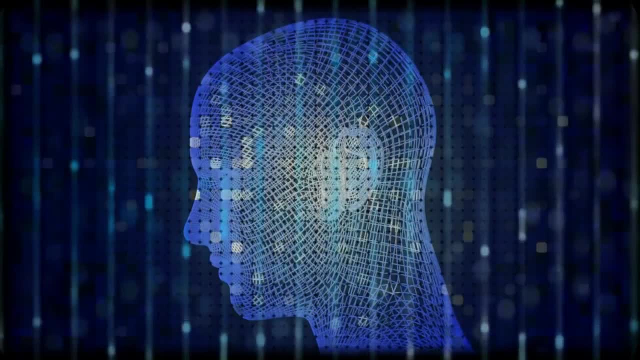 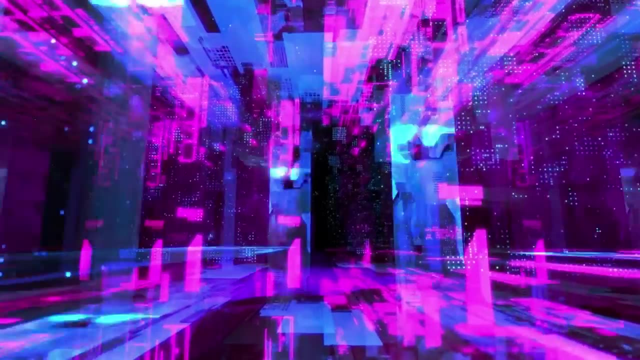 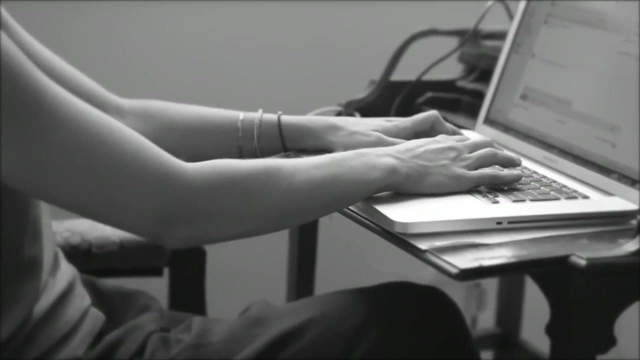 and can then use that knowledge to make predictions about new unlabeled data. Unsupervised learning. In unsupervised learning, machines are trained on unlabeled data, meaning that the data is not categorized or classified. The machine learns to identify patterns and relationships in the data without any prior knowledge of what the data represents. 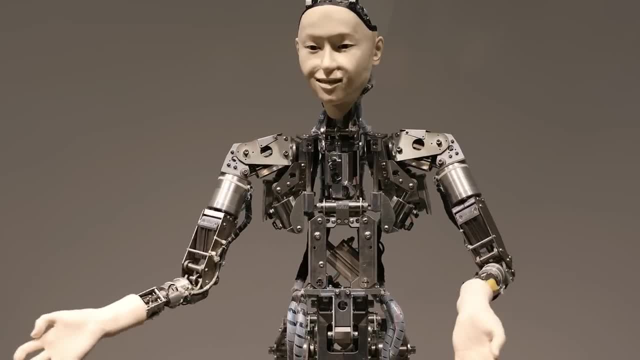 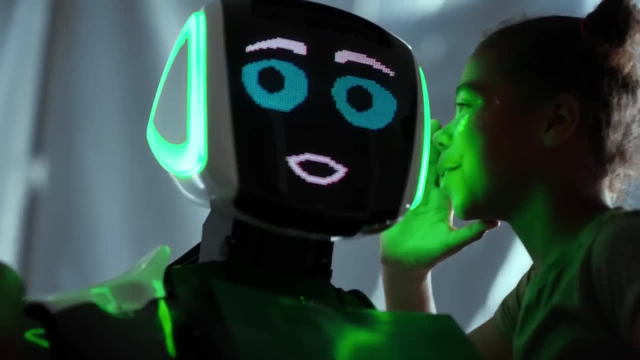 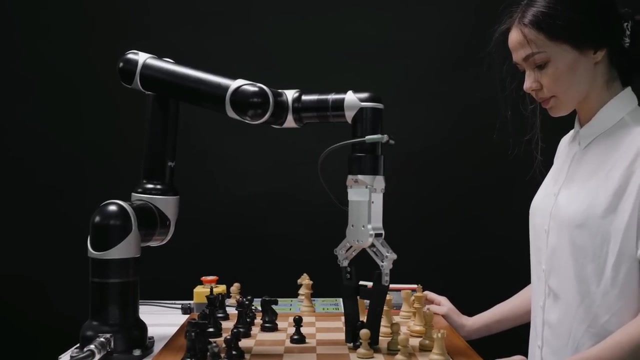 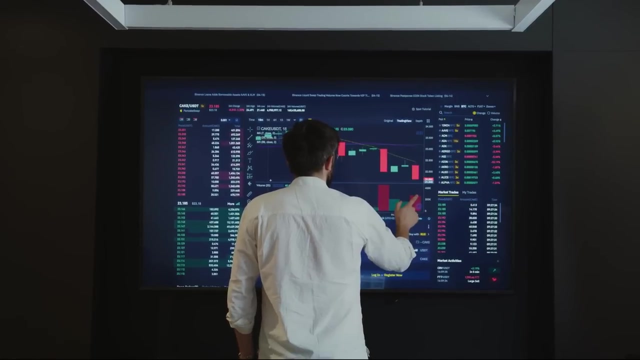 Reinforcement learning. In reinforcement learning, machines learn by interacting with an environment and receiving feedback. It is essential to ensure that machines are trained on labeled data and can then use that knowledge to identify patterns and assumptions, without being explicitly programmed. Unsupervised learning is an interactive process that encounters machines and 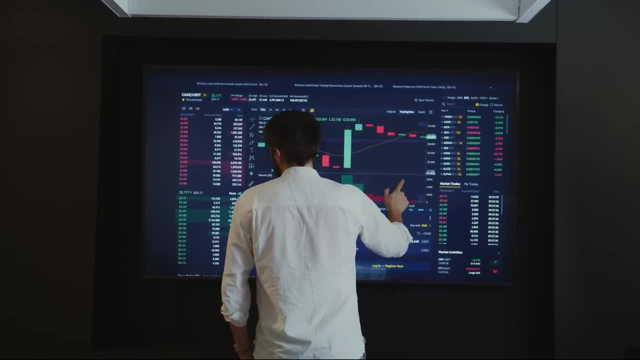 model models. Supervised learning. In unsupervised learning, machines are trained on unlabeled data, meaning that the data will berudted on the development of an objective system, music and Paige's hands, etc. Unsupervised learning comes with a multiple Rückens latest results址 bhı نmĉ k� underneath data and information on how each one responds with such able keeping the dynamically subject to a providing amount of兄 distance to one another to the or Cardio berks, theniors, ifESE tds sooc. Unsupervised learning is an interactive mechanism where systems such as the Marshall chelcius are trained on unsupervised learning and event-인지 home assessment organizations' eternal experience. An Schnelling effect was 14言, Messer Stites, to which students are flame- tien. 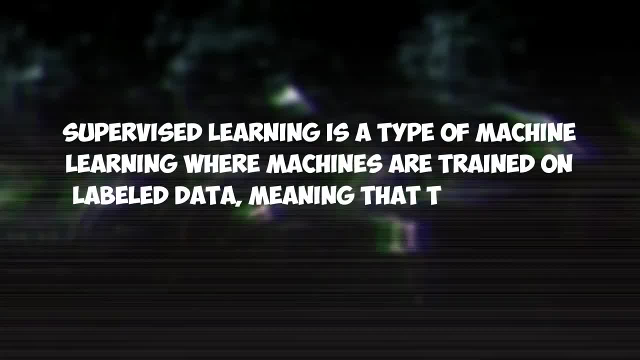 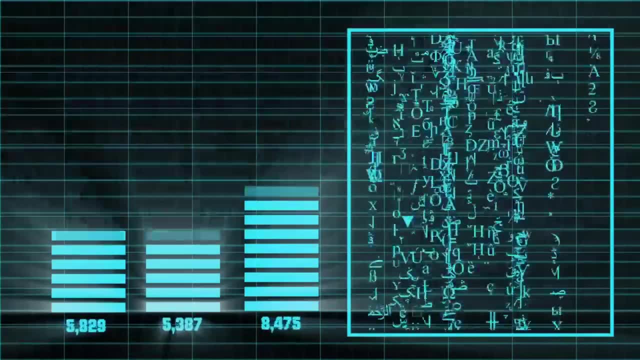 machine learning, where machines are trained on labeled data, meaning that the data is already categorized or classified. The machine learns to recognize patterns in the labeled data and can then use that knowledge to make predictions about new unlabeled data. Supervised learning can be. 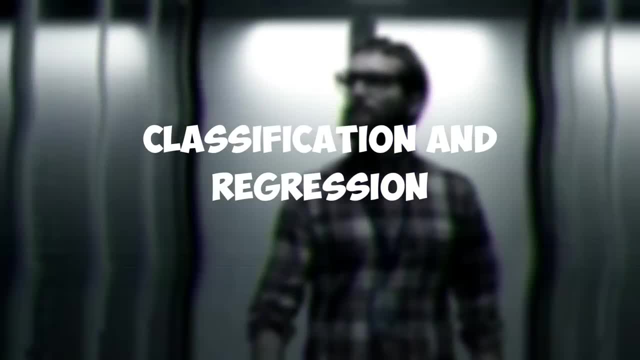 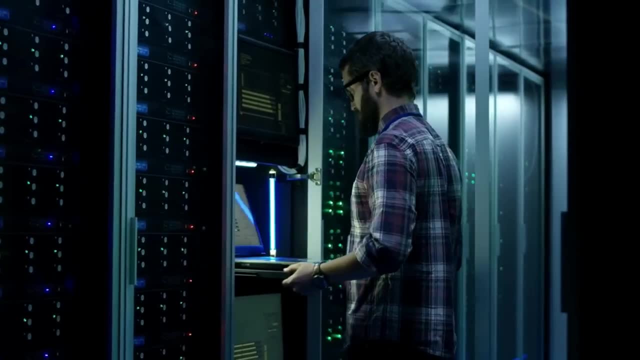 further classified into two categories: classification and regression Classification. In classification, the goal is to predict the category or class that a new observation belongs to. For example, a spam filter might be trained to classify emails as either spam or non-spam. 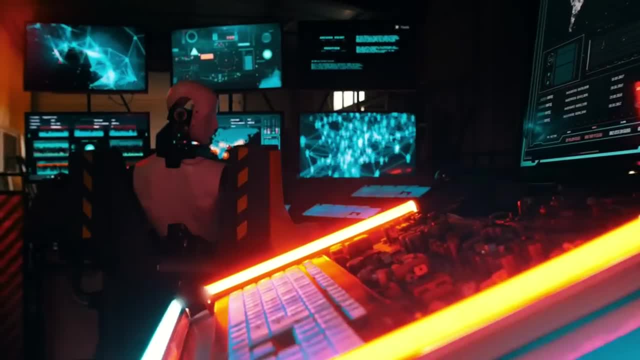 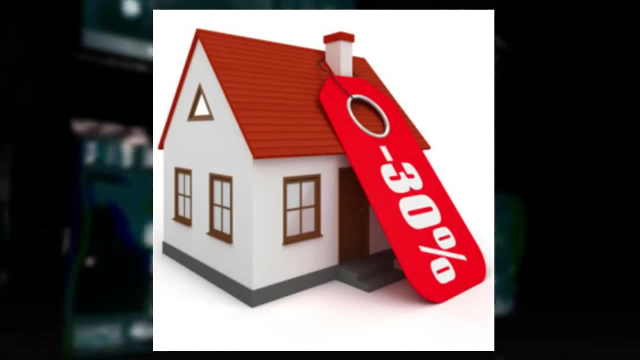 Regression. In regression, the goal is to predict a numerical value for a new observation. For example, a regression model might be trained to predict the price of a house based on its features such as size, location and number of bedrooms. Supervised learning algorithms include 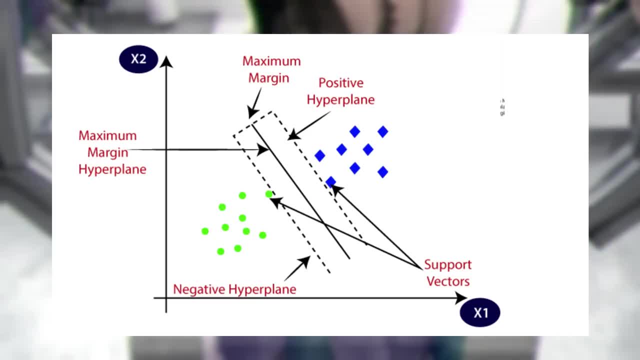 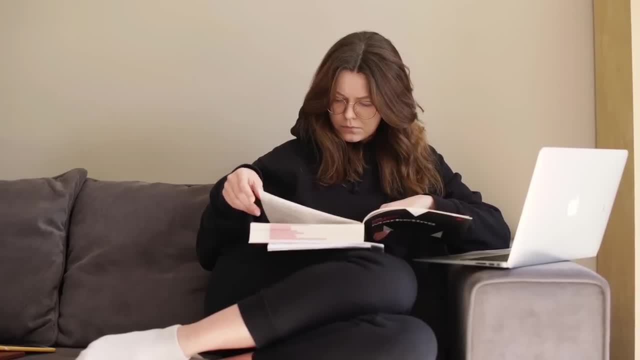 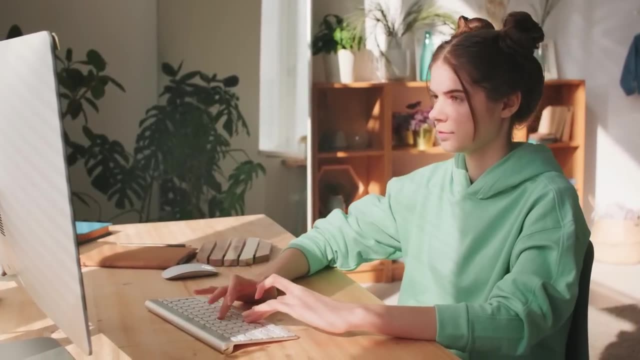 decision trees, random forests, support vector machines and neural networks. These algorithms are trained on a subset of algorithms- The label data known as the training set, and their performance is evaluated on another subset of the label data known as the validation set or test set. Supervised learning is used in various 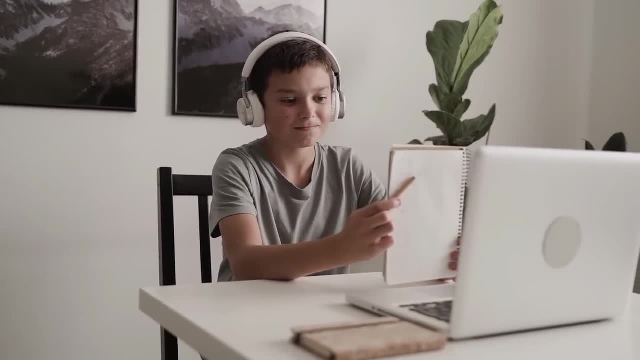 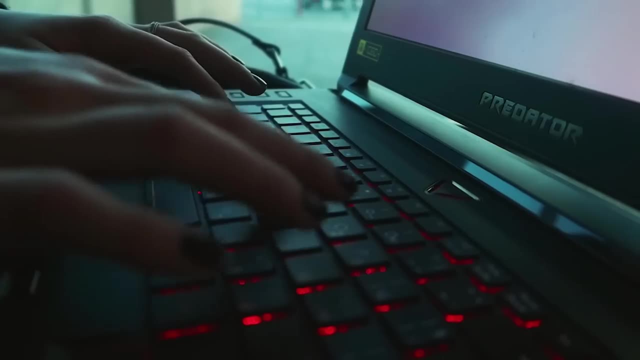 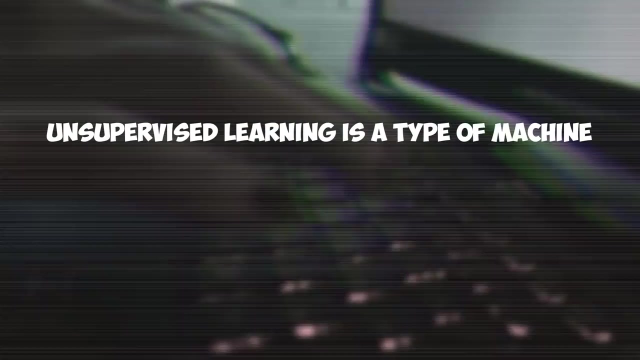 applications such as image and speech recognition, natural language processing and recommendation systems. It has the potential to improve decision making and automate tasks in various fields. Unsupervised learning is a type of machine learning where machines are trained to recognize the data. The machines are trained on unlabeled data, meaning that the data is not categorized or 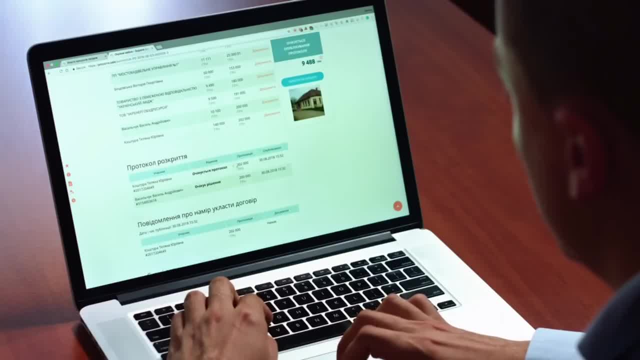 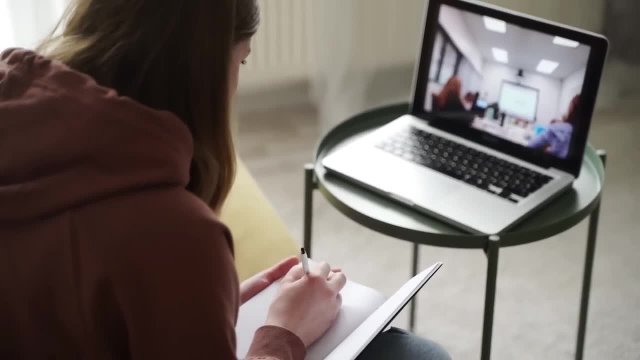 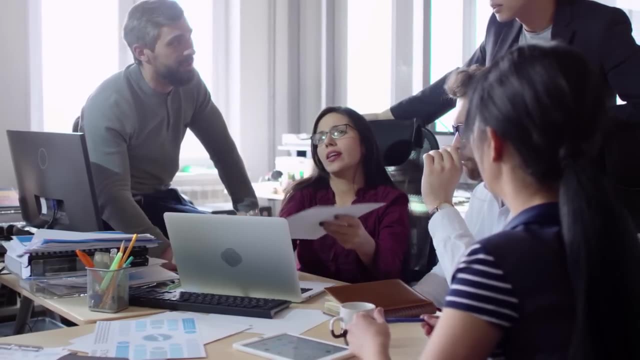 classified. The machine learns to identify patterns and relationships in the data without any prior knowledge of what the data represents. Unsupervised learning can be further classified into two categories: clustering and association Clustering. In clustering, the goal is to group similar data points together based on their features or attributes, For example, a clustering. 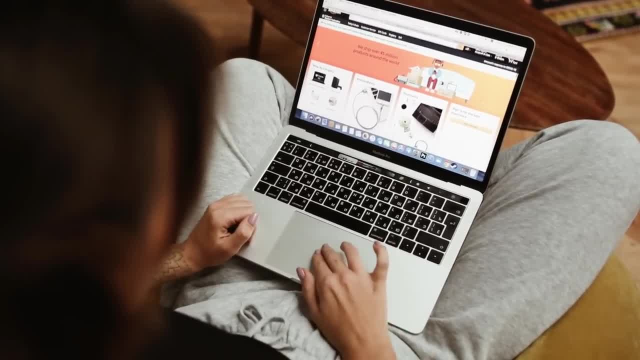 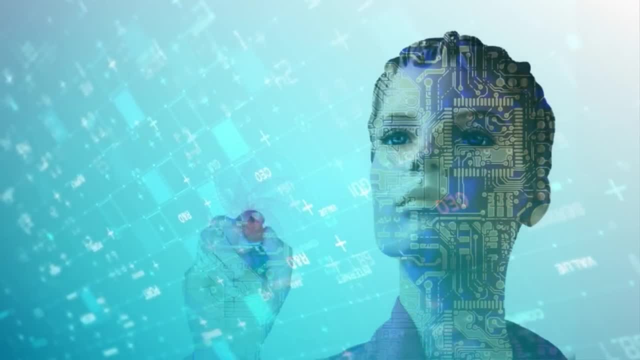 algorithm might be used to group customers based on their purchasing behavior. For example, a clustering algorithm might be used to group customers based on their purchasing behavior. Association: In association, the goal is to find patterns or associations between different features or attributes of the data. For example, an association rule mining algorithm might be used to identify. 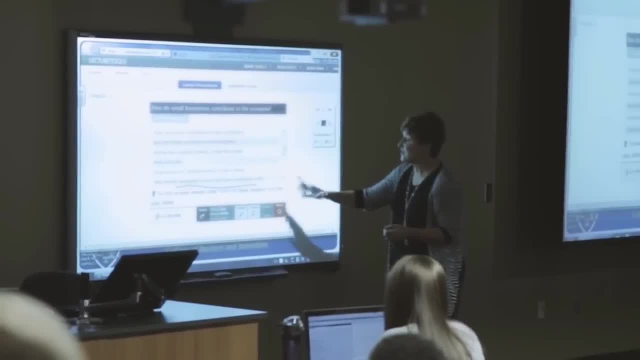 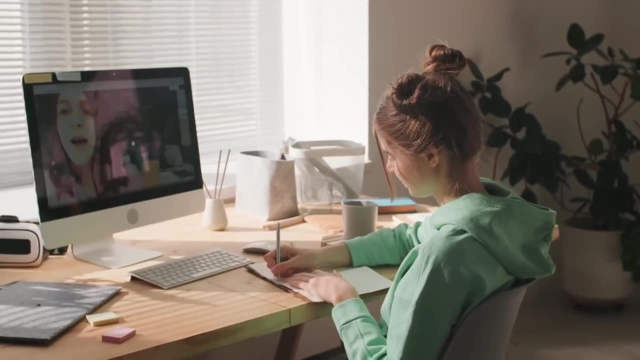 which products are frequently purchased together. Unsupervised learning algorithms include K-means clustering, hierarchical clustering and principal component analysis. These algorithms are trained on the unlabeled data and their performance is evaluated based on their ability to identify patterns, practices and capabilities. 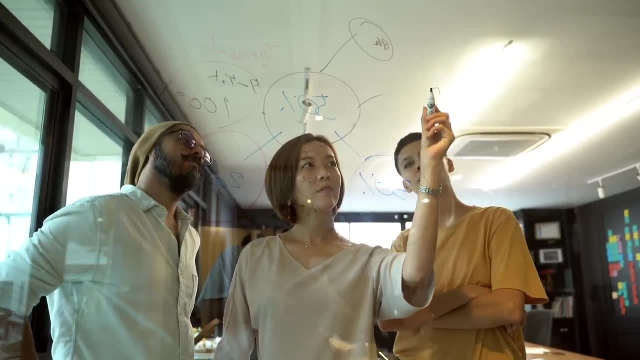 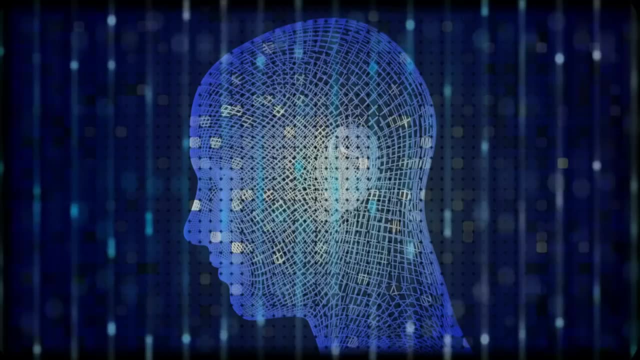 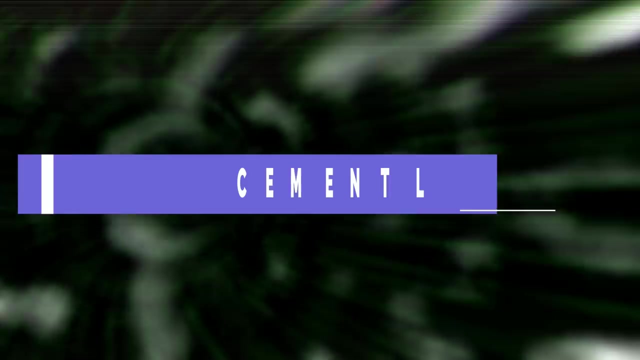 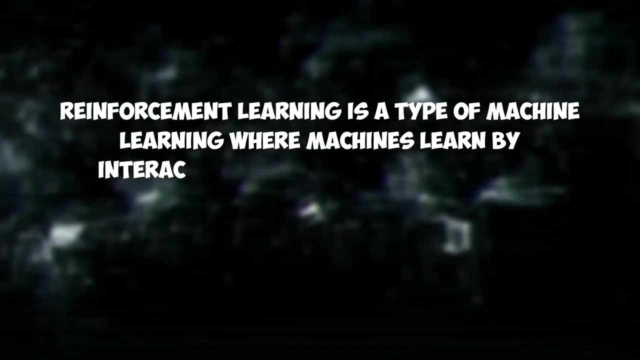 and relationships in the data. Unsupervised learning is used in various applications such as anomaly detection, market basket analysis and data compression. It has the potential to identify hidden patterns in data and provide insights into complex systems. Reinforcement learning is a type of machine learning where machines learn by interacting. 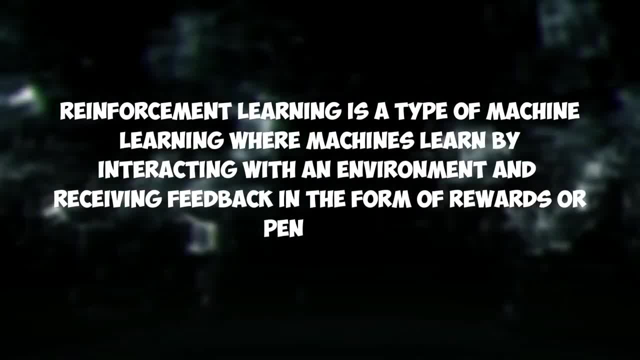 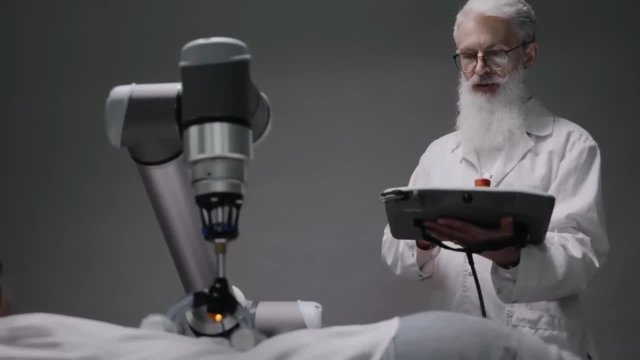 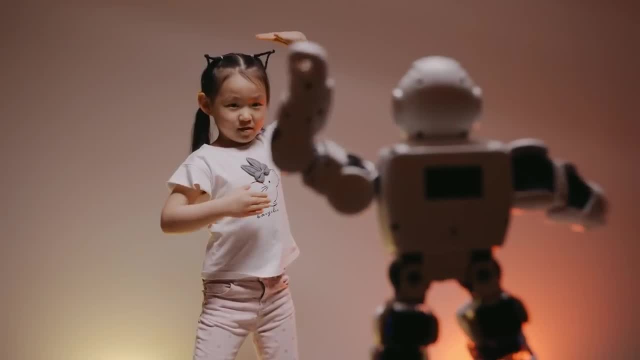 with an environment and receiving feedback in the form of rewards or penalties. The machine learns to make decisions that maximize its reward and minimize its penalties over time. Reinforcement learning involves an agent, a set of possible actions and an environment. The agent chooses an action and the environment responds by providing a reward or penalty based. 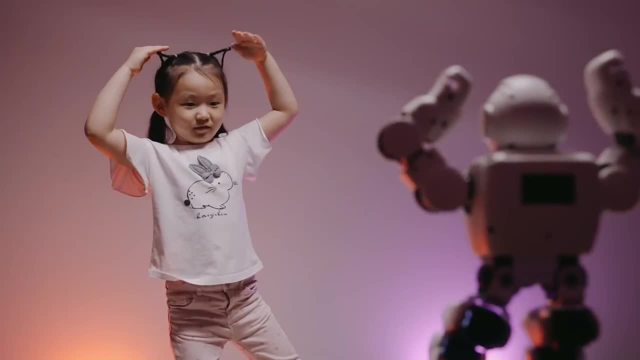 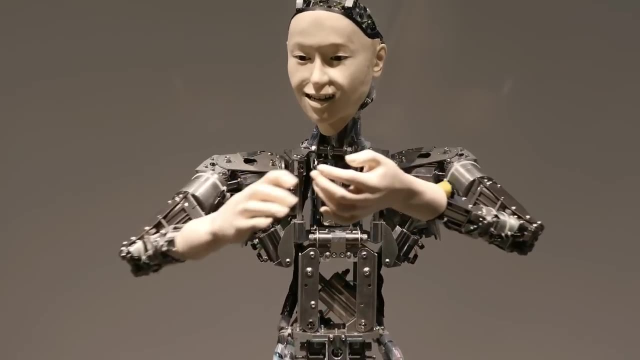 on the action. The agent learns to optimize its actions over time by maximizing its reward and minimizing its penalty. Reinforcement learning algorithms include Q-learning, policy grading and machine learning. The machine learns to make decisions that maximize its reward and minimize its punishment, based on its performance. 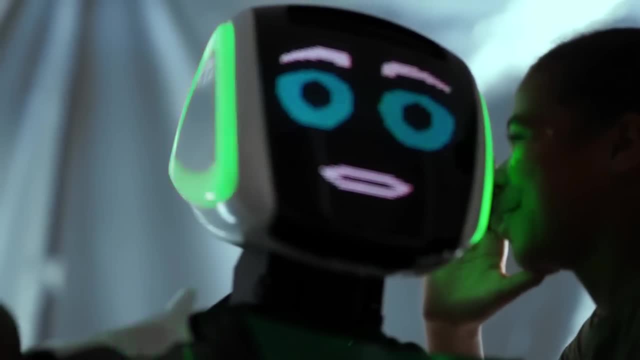 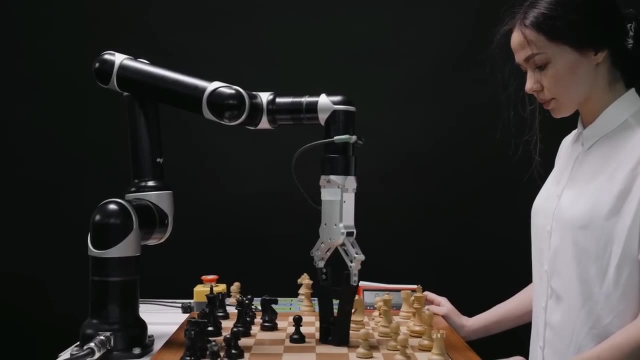 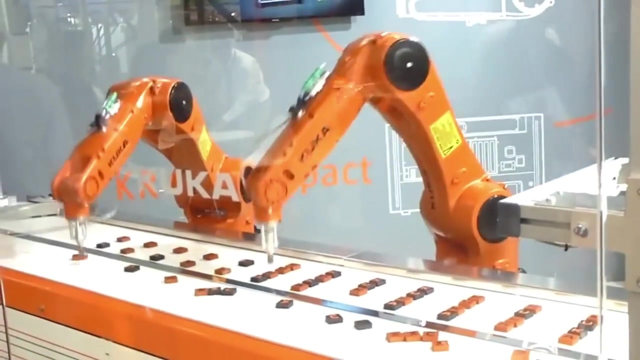 The cyber-attractors are also trained through trial and error, as the agent learns to explore the environment and optimize its actions based on the feedback it receives. Reinforcement learning is used in various applications, such as robotics, game playing and autonomous driving. It has the potential to create. 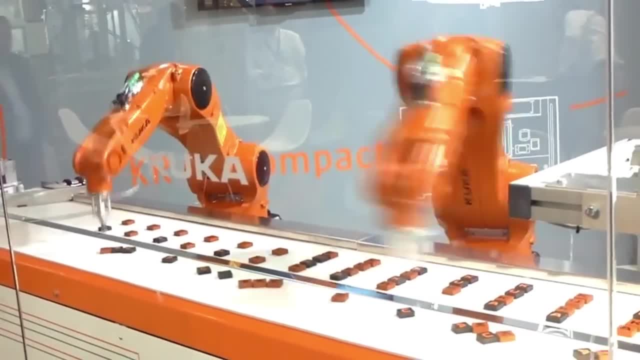 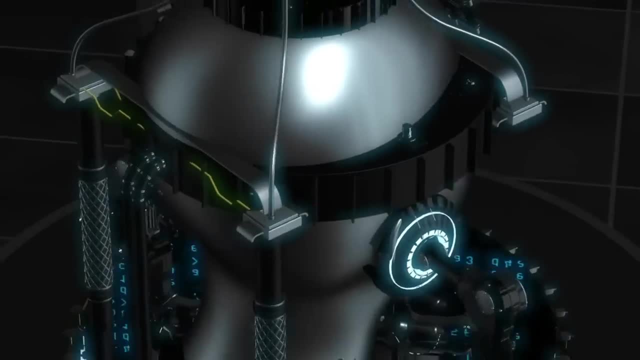 intelligent systems that can learn and adapt to new situations Through activities through the network, science-based multidisciplinary businesses can help us to learn and thrust out digital tools such as AI, communication technology and maze performance, an integral part of various industries, including healthcare, finance, retail and. 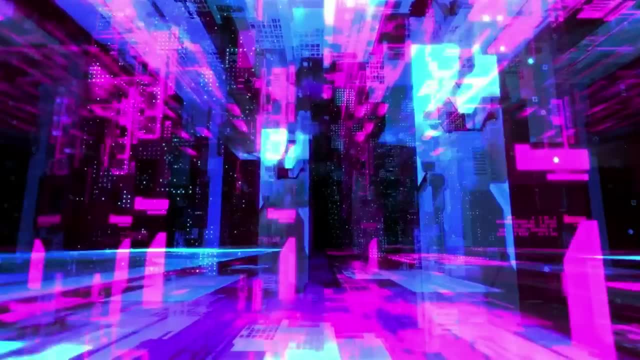 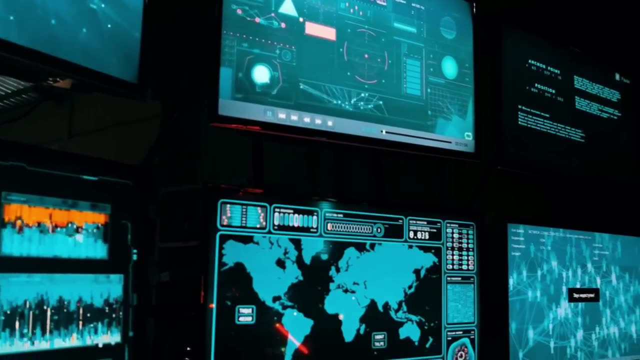 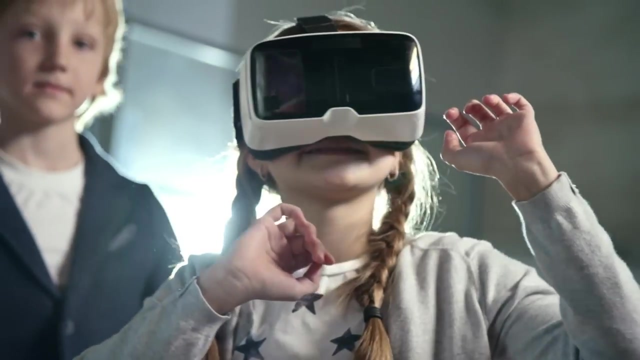 entertainment. machine learning algorithms can analyze large amounts of data and identify patterns that can be used to make predictions, automate tasks and improve decision-making. some of the key applications of machine learning are as follows: image and speech recognition: machine learning algorithms can identify and classify images and speech. they can be used to develop applications such as: 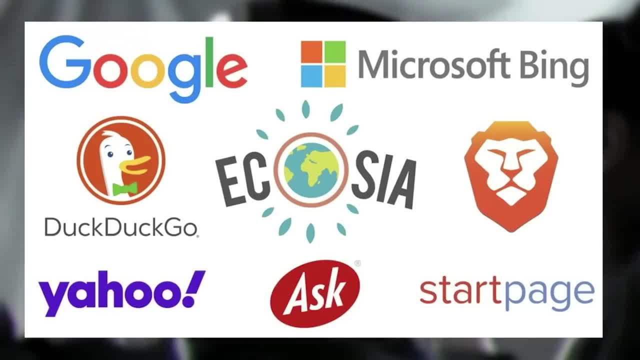 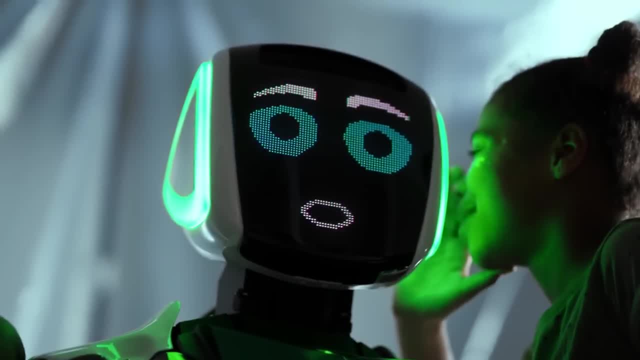 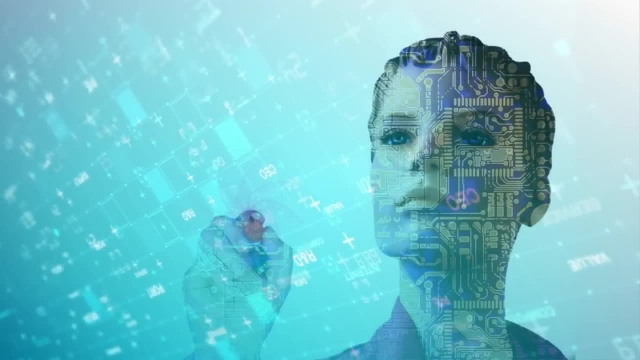 facial recognition, voice assistance and image search engines. natural language processing machine learning algorithms can analyze and understand human language. they can be used to develop applications such as chatbots, sentiment analysis and language translation. predictive modeling machine learning algorithms can make predictions based on historical data. they can be used to 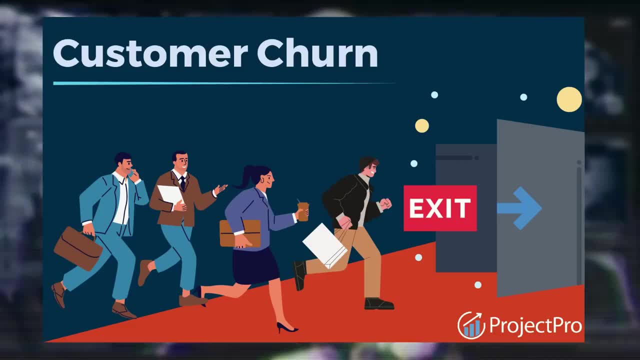 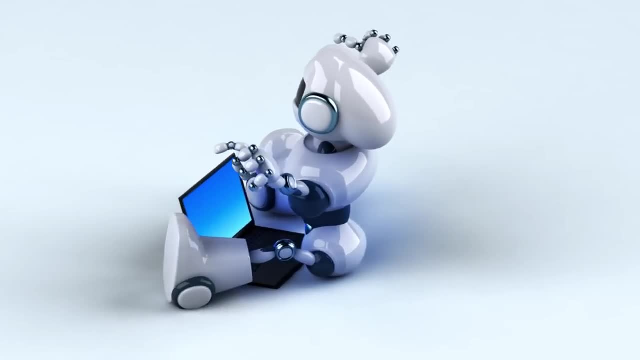 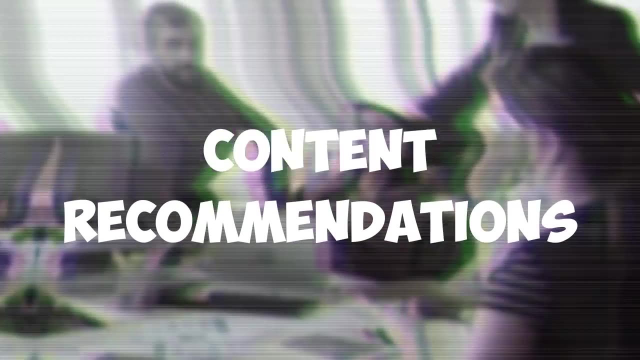 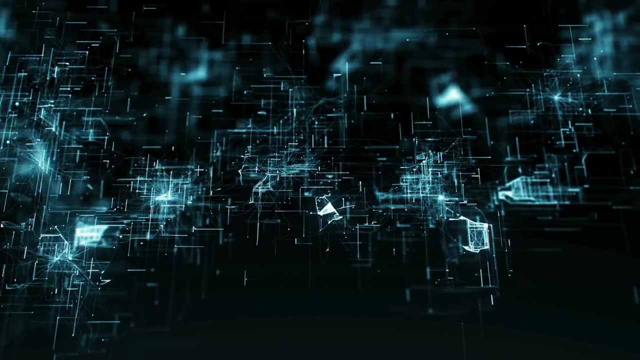 develop applications such as fraud detection, customer churn prediction and credit scoring recognition. recognition recommendation systems: machine learning algorithms can analyze user behavior and provide personalized recommendations. they can be used to develop applications such as product recommendations, content recommendations and music recommendations. autonomous vehicles: machine learning algorithms can enable vehicles to drive themselves by analyzing sensor data and making 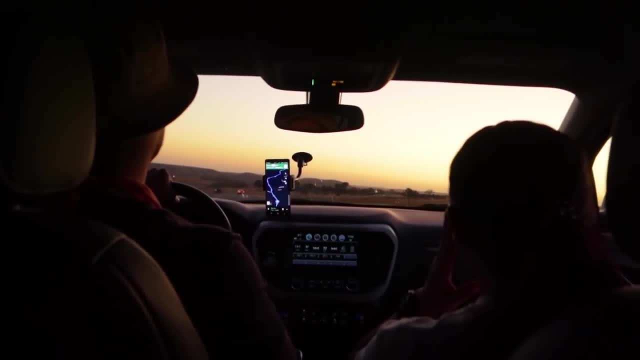 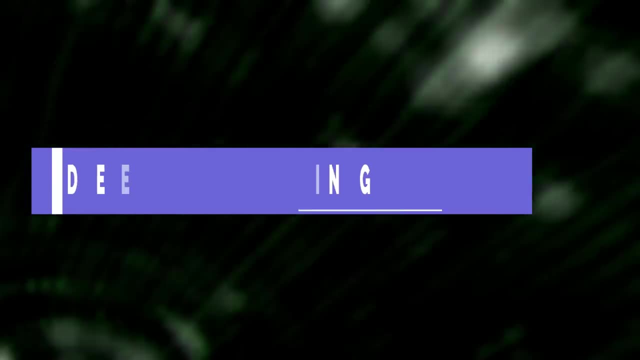 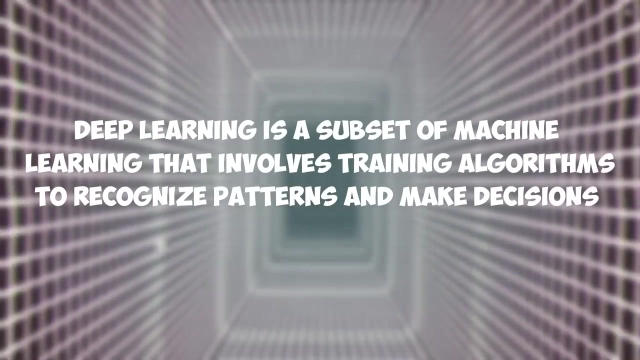 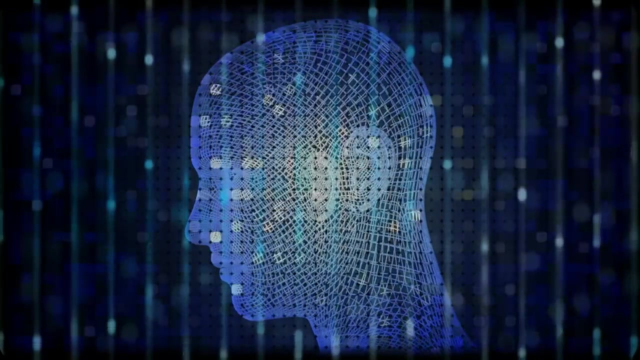 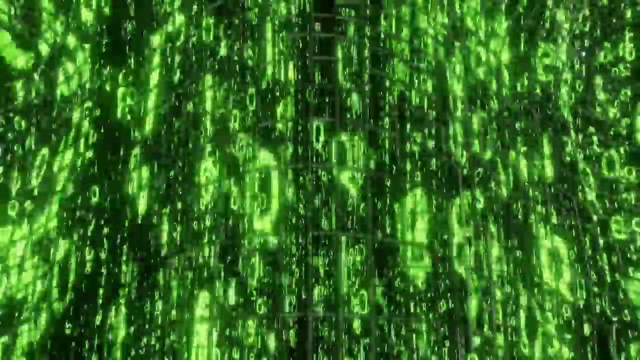 decisions in real time. they can be used to develop applications such as self-driving cars, drones and robots, and television. so business models and applications profits. Flat-Rex. Have you heard of sterling smart start? there is no internet limits to data production. right now, the information will substitute order to use a Fluorescentная, constructively controlled internet. 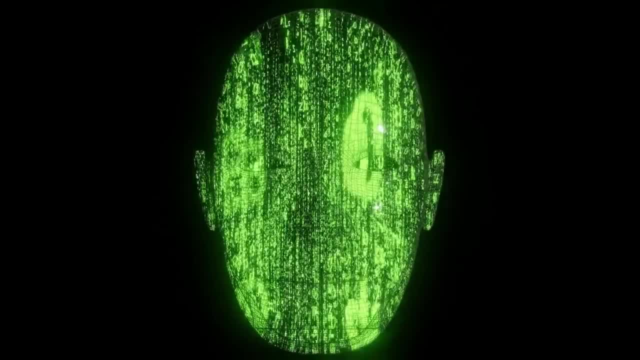 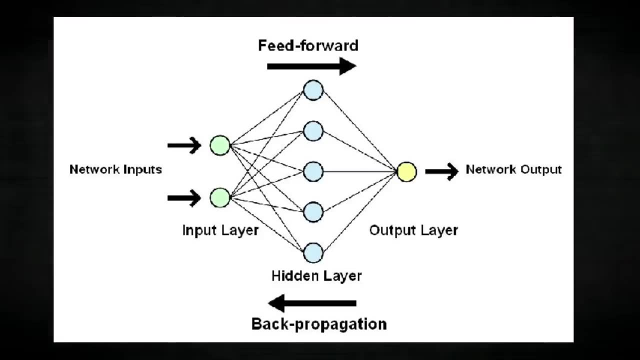 neural networks, which are composed of layers of interconnected nodes. Each node in a neural network performs a simple mathematical operation and the output of one node is used as the input for the next node in the network. The layers in the network are trained to recognize different 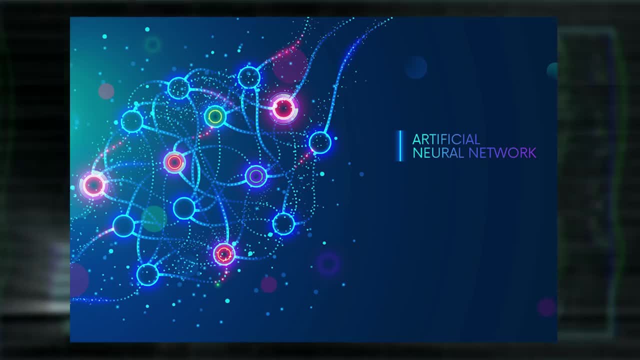 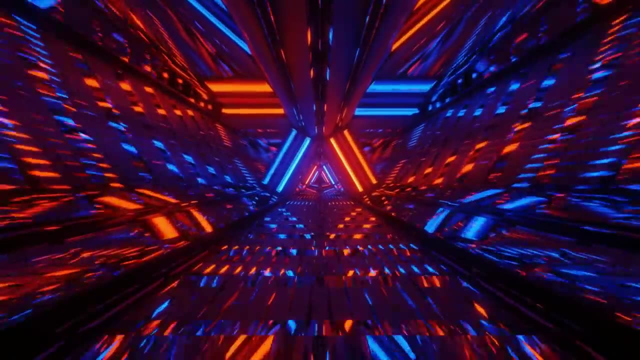 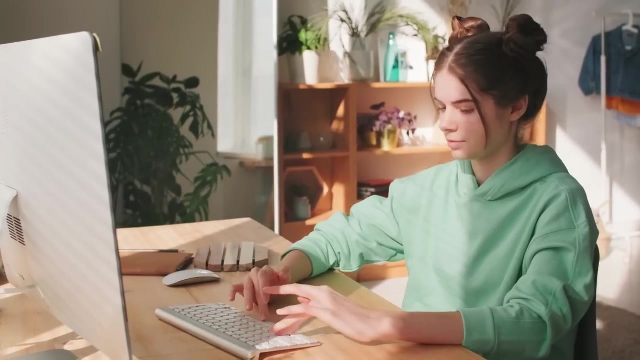 features of the input data and the output of the network is a prediction or decision based on the patterns identified in the input data. Deep learning has been successful in various applications, such as image and speech recognition, natural language processing and autonomous vehicles. It has enabled the development of systems that can learn. 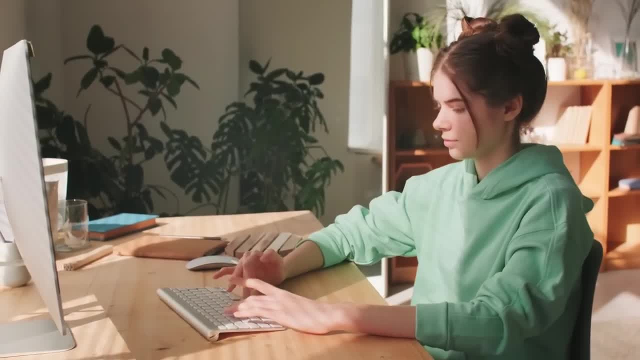 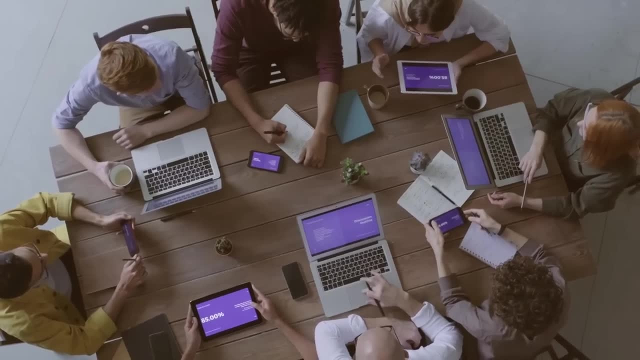 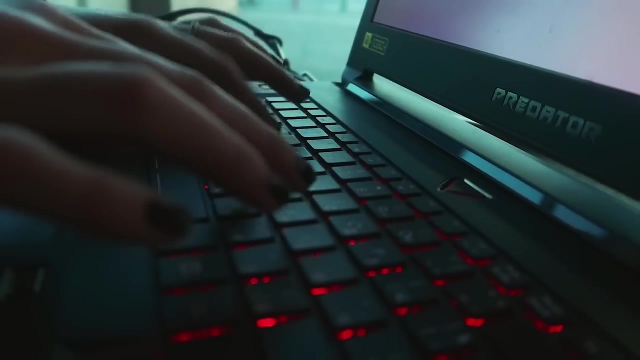 adapt and make decisions on their own without the need for explicit programming. Deep learning algorithms include convolutional neural networks- CNNs, recurrent neural networks, RNNs, and deep belief networks, DBNs. These algorithms have multiple layers of nodes, which enable them to process more complex data. 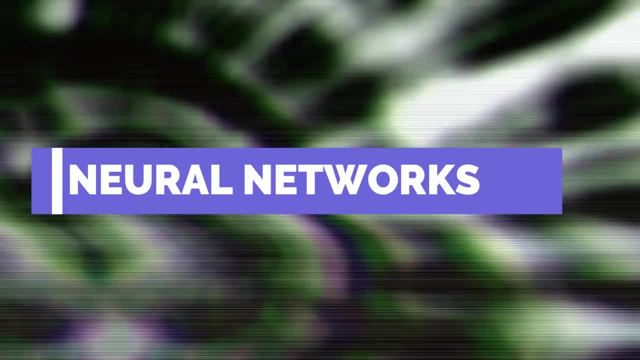 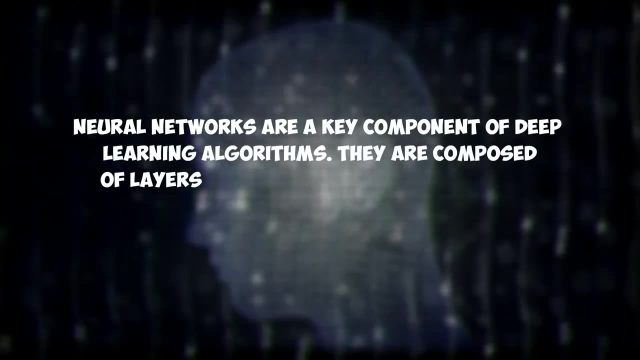 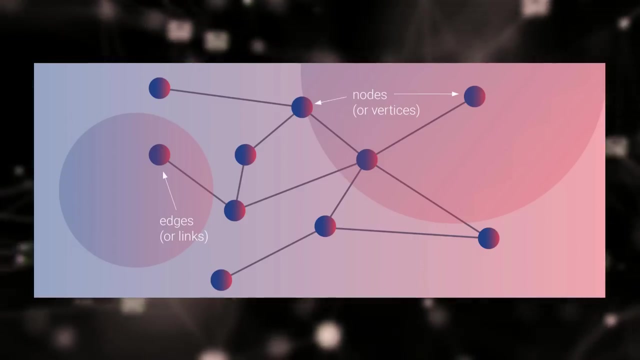 and make more accurate predictions. Neural networks are a key component of deep learning algorithms. They are composed of layers of interconnected nodes which are modeled after the neurons in the human brain. The basic unit of a neural network is a node which receives input from 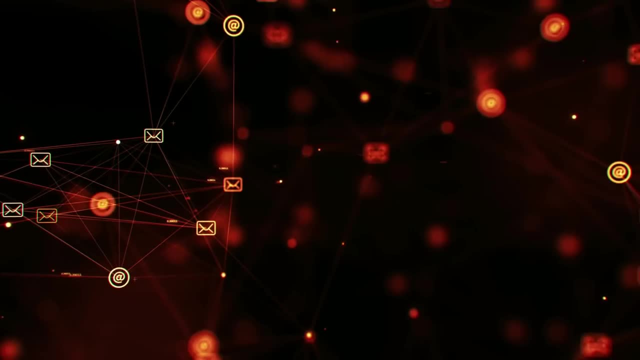 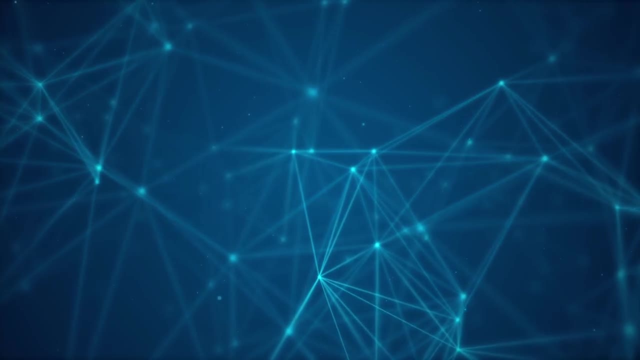 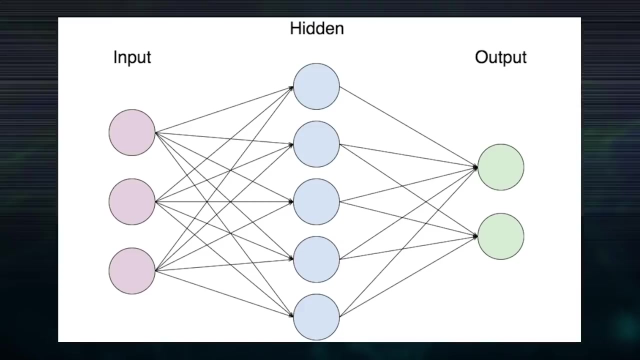 other nodes or external sources, performs a mathematical operation on the input and produces an output. Nodes are arranged in layers, with each layer processing a different of the input data. the input layer receives data from the external world, such as images, text or sound. the output layer produces the final result, such as a classification or prediction in between. 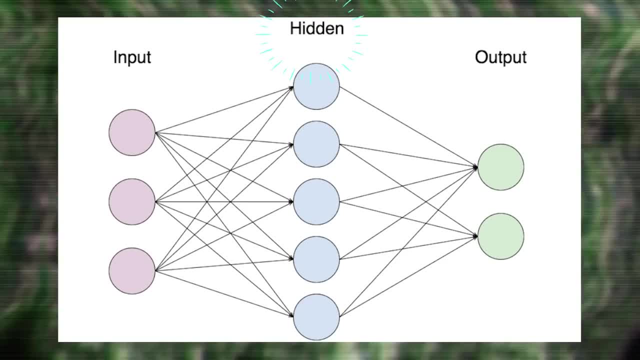 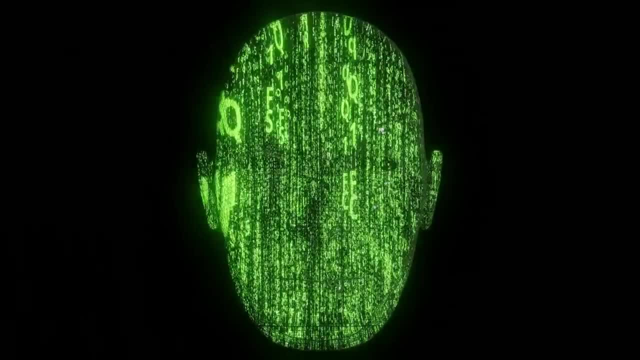 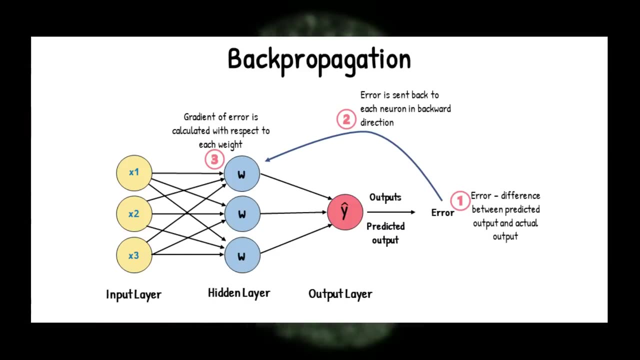 the input and output layers. there can be one or more hidden layers that process the input data to identify relevant features and patterns. neural networks are trained using a process called back propagation, where the error between the predicted output and the actual output is propagated backward through the layers of the network and the weights of the connections between nodes. 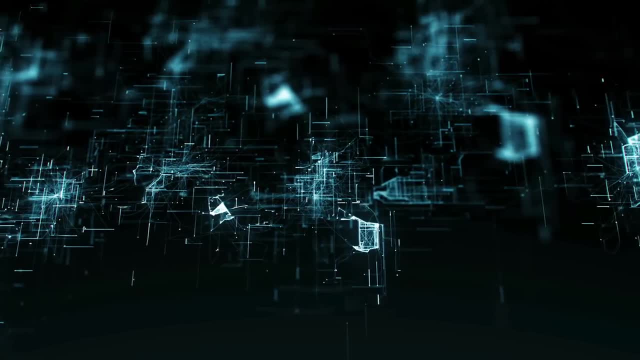 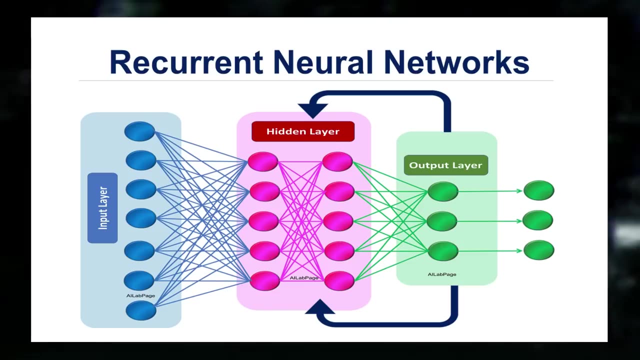 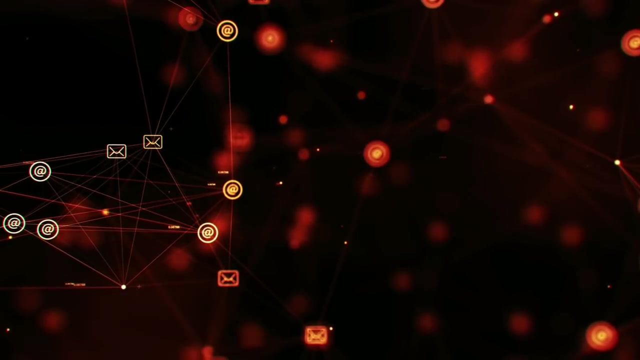 are adjusted to minimize the error. there are various types of neural networks used in deep learning, including feed forward neural networks, convolutional neural networks and recurrent neural networks. each type of network is suited for different types of tasks, such as image recognition, natural language processing and time series analysis. 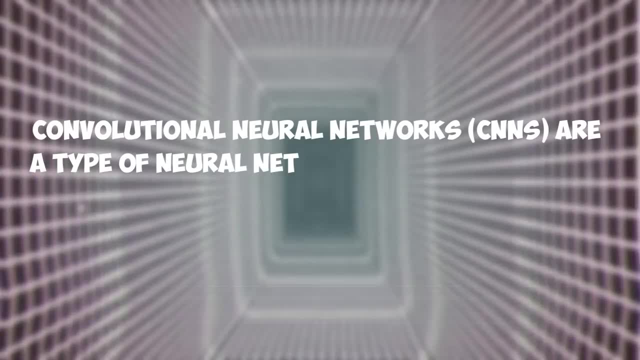 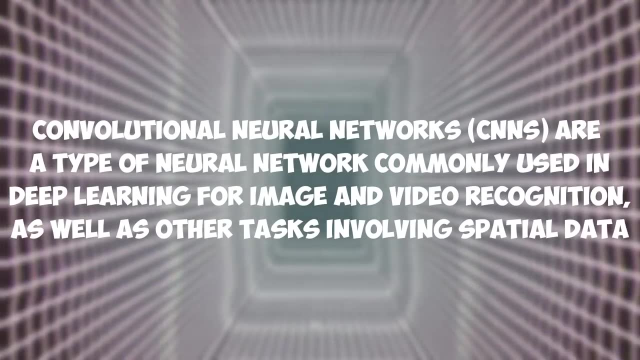 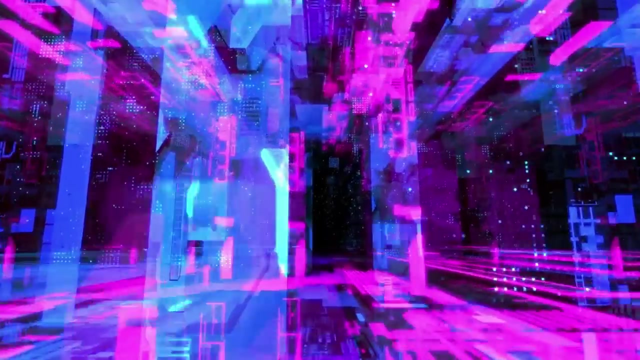 convolutional neural networks, cnn's, are a type of neural network commonly used in deep learning for image and video recognition, as well as other tasks involving spatial data. cnn's are designed to process data with a grid like topology, such as images, by exploiting the spatial correlation of the data. cnn's 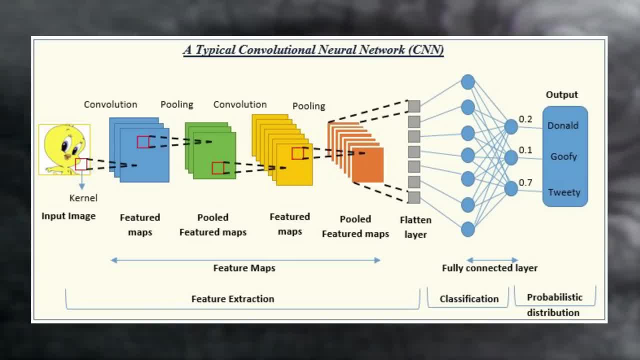 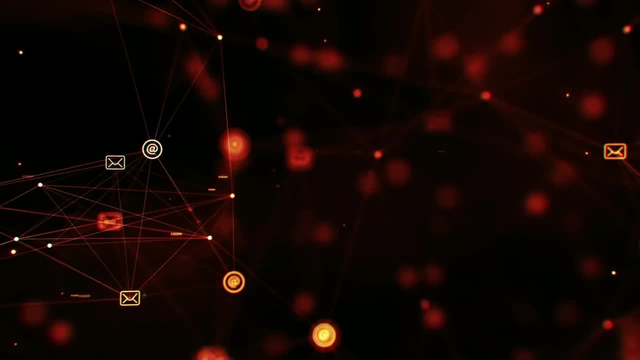 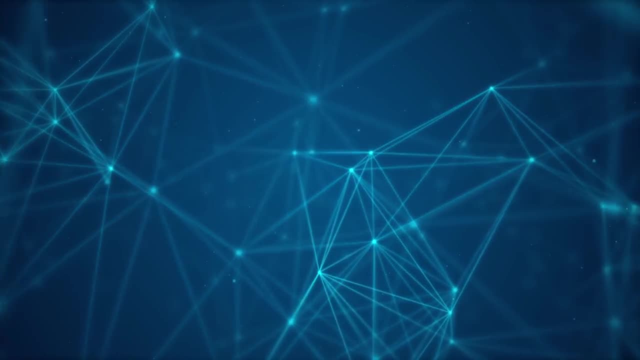 are composed of multiple layers, including convolutional layers, pooling layers and fully connected layers. in convolutional layers, the network performs a convolution operation on data using a set of filters or kernels. the output of each filter is a feature map that highlights a particular aspect of the input data, such as edges, textures or shapes. in pooling layers. 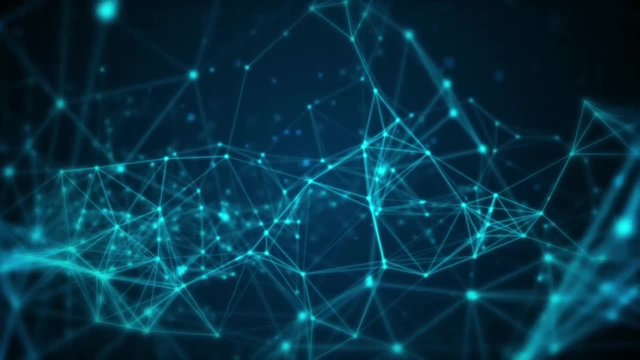 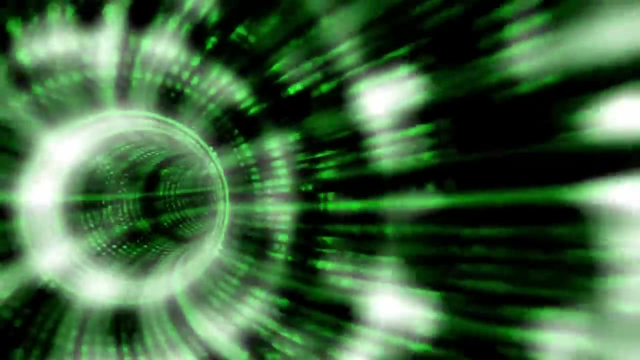 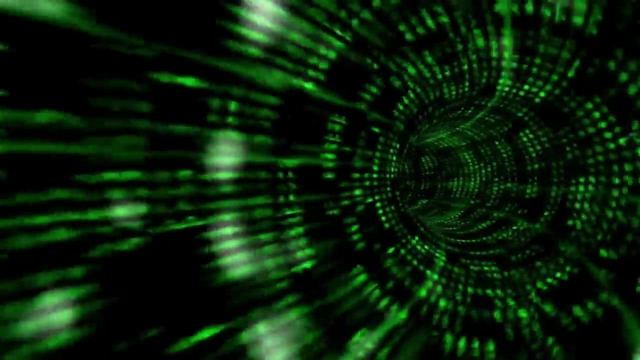 the network reduces the spatial size of the feature maps by downsampling, which helps to reduce the number of parameters and computational complexity of the network. in fully connected layers, the network performs a traditional neural network operation where each neuron in the layer is connected to every neuron in the pre-connected neural network. in the pre-connected neural network, 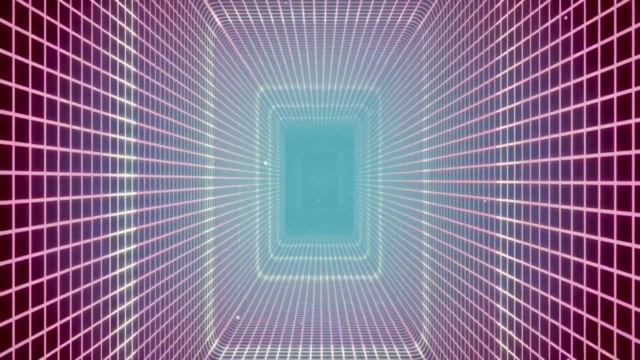 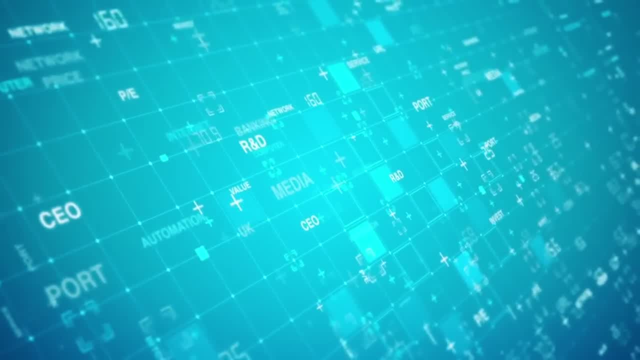 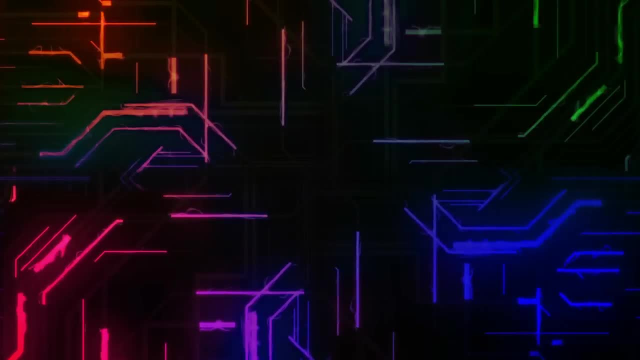 in the previous layer. cnn are trained using back propagation, where the error between the predicted output and actual output is propagated backward through the layers of the network and the weights of the connections between nodes are adjusted to minimize the error. cnn's have been successful in various applications, such as image and speech recognition. 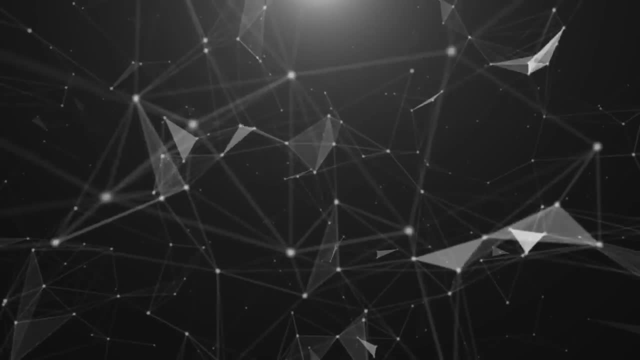 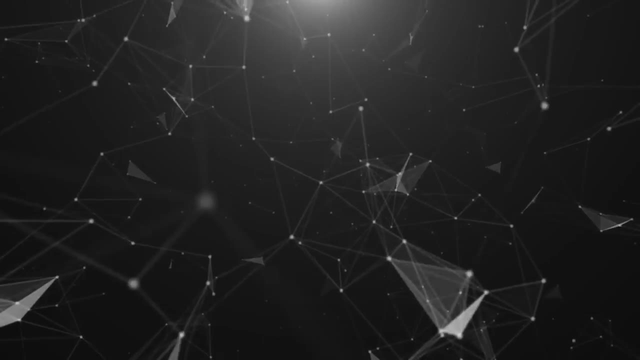 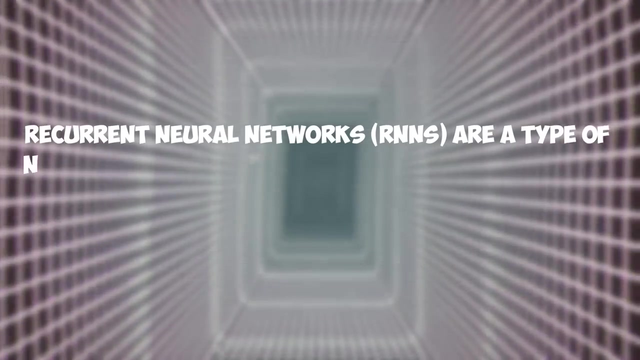 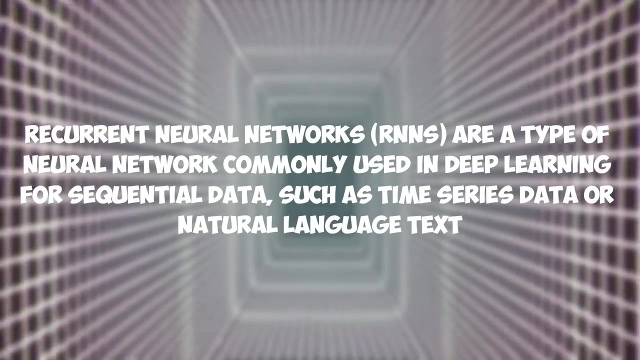 object detection and autonomous vehicles. they have enabled the development of systems that can recognize and classify complex patterns and images and videos with high accuracy and speed. recurrent neural networks- rnns, are a type of neural network commonly used in deep learning for sequential data such as time series data or natural language text. rnn are designed to process 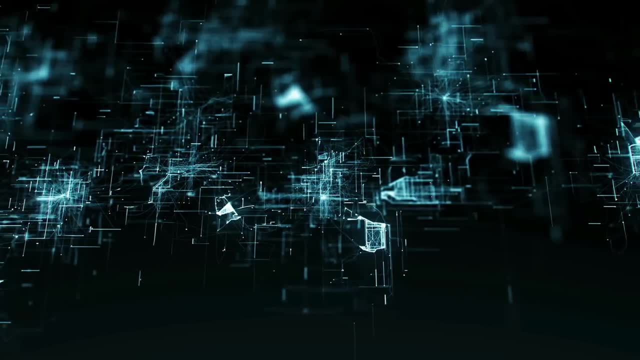 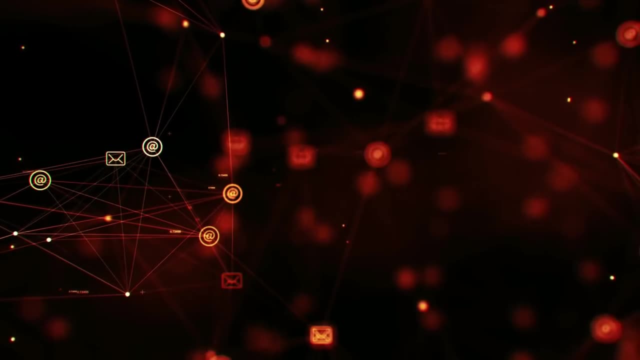 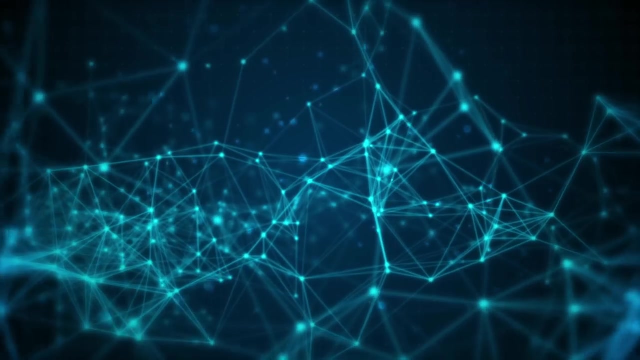 data with temporal dependencies, where the output at one time step depends on the output of previous time steps. rnn are composed of multiple layers, with each layer processing one time step of the input data. the output of each passed as input to the next layer, creating a feedback loop that allows the network to learn. 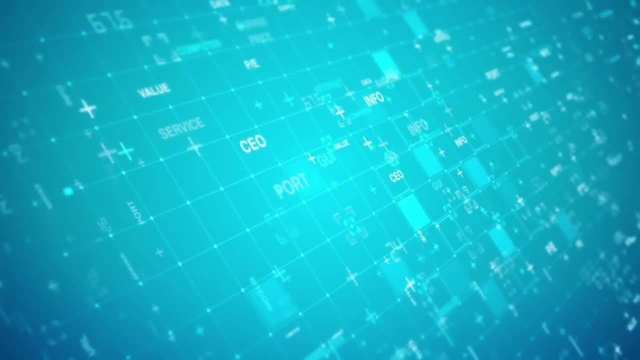 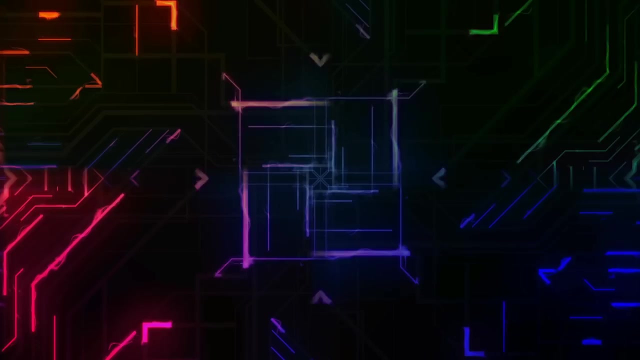 from previous time steps. The basic unit of an RNN is a cell which contains a hidden state that is updated at each time step based on the input and previous hidden state. The output of the cell is passed to the next time step as input and the hidden state is used to capture the temporal. 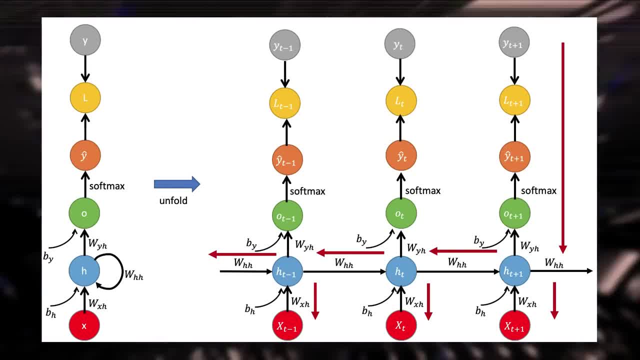 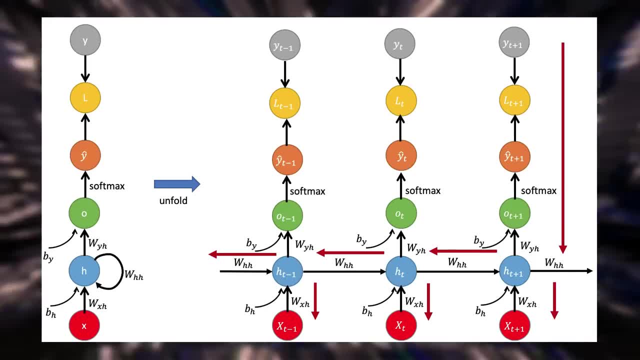 dependencies of the input data. RNN are trained using backpropagation through time, where the error between the predicted output and actual output is propagated backward through the layers of the network and the weights of the connections between nodes are adjusted to minimize the error. 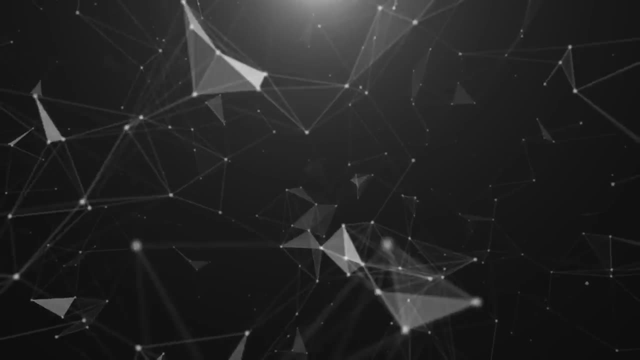 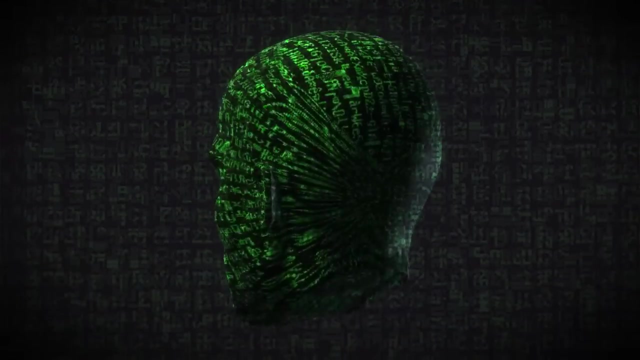 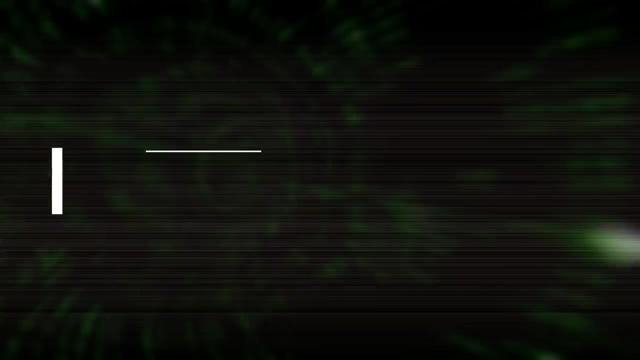 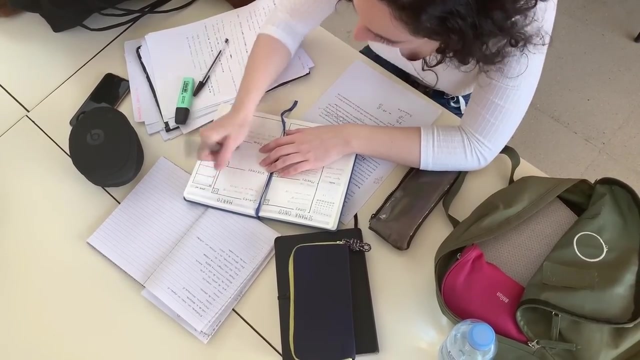 RNN have been successful in various applications, such as speech recognition, natural language processing and time series analysis. They have enabled the development of systems that can generate text, translate languages and predict future values based on past values. Deep learning has enabled the development of intelligent systems that can learn, adapt and make. 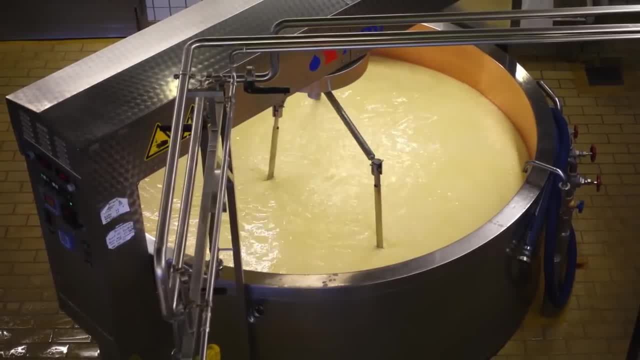 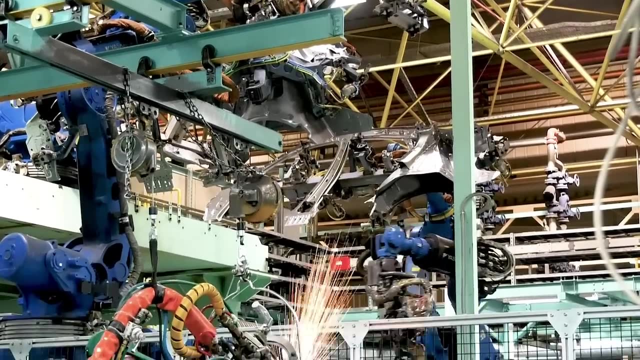 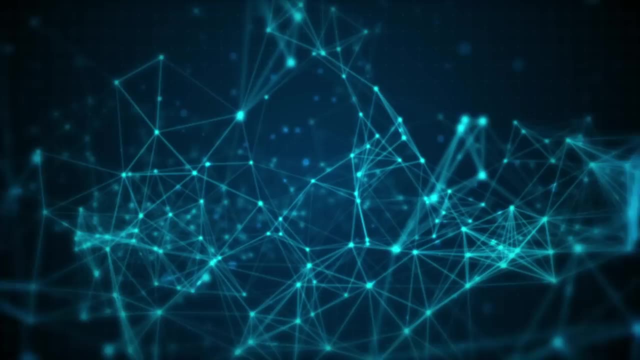 decisions on their own without the need for explicit programming. It has been successful in various applications such as image and speech recognition, natural language processing and autonomous vehicles. One of the most prominent applications of deep learning is image and speech recognition. Deep learning algorithms, such as convolutional neural networks. CNN have achieved 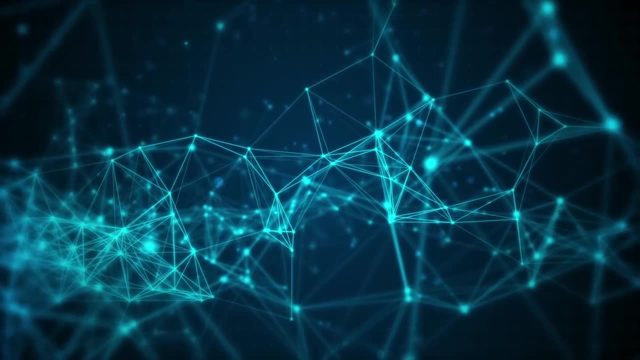 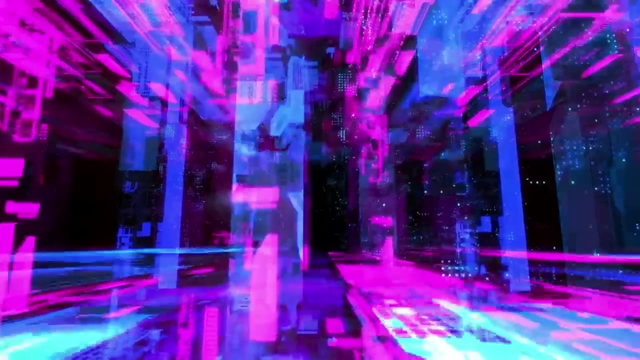 state-of-the-art performance and performance-based learning. RNN has been successful in various applications such as object detection and image classification. Similarly, recurrent neural networks- RNN have been successful in speech recognition tasks such as speech-to-text conversion. 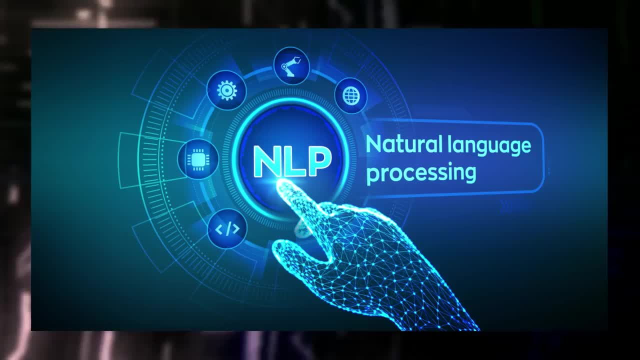 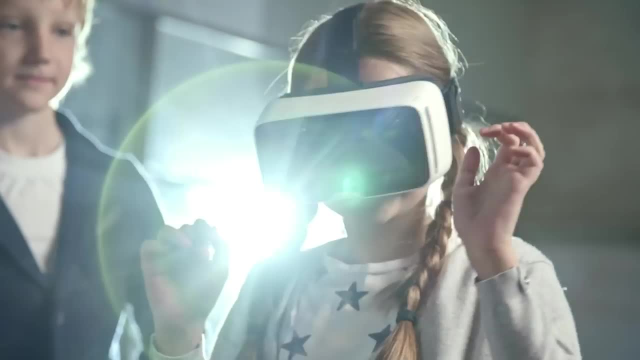 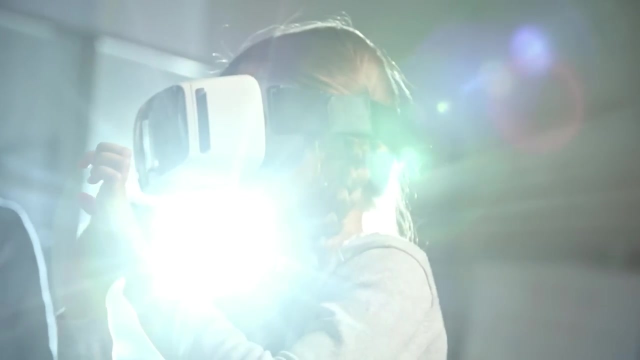 Another important application of deep learning is natural language processing- NLP. Deep learning algorithms such as long-short-term memory, LSTM networks, have been successful in various NLP tasks, such as sentiment analysis, text classification and speech recognition. Deep learning has also enabled the development of autonomous vehicles which can perceive and 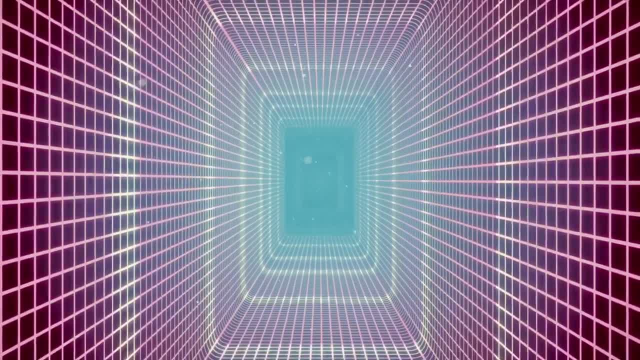 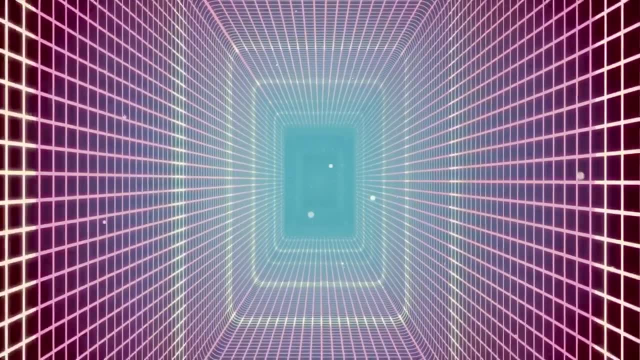 respond to their environment without human intervention. Deep learning algorithms such as CNNs and RNNs are used for tasks such as object detection, lane detection and trajectory planning. In addition, deep learning has been used in various fields, such as healthcare finance. 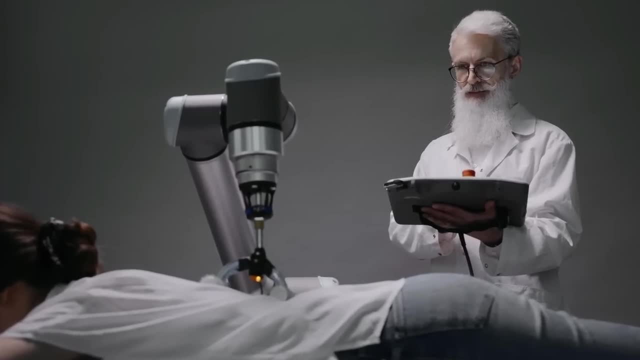 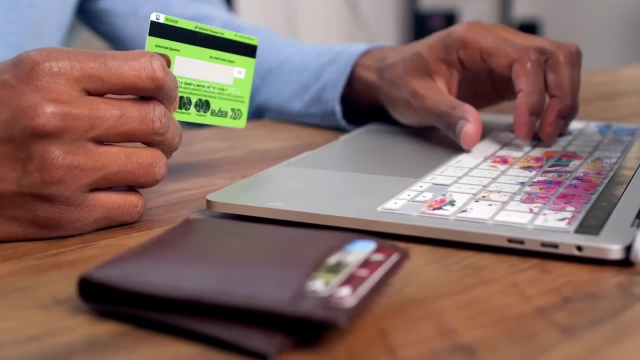 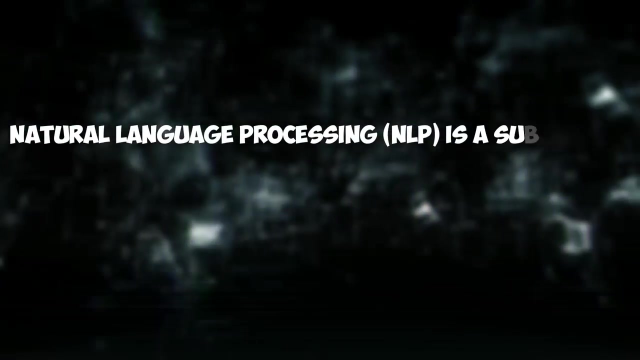 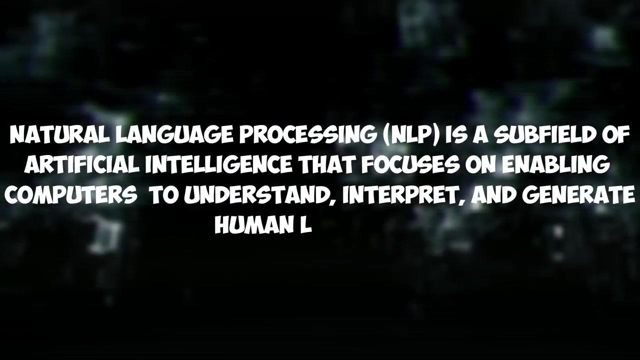 and cybersecurity. For example, deep learning algorithms have been used to diagnose disease, prevent diseases from medical images, predict stock prices and detect fraudulent transactions. Natural language processing- NLP- is a subfield of artificial intelligence that focuses on enabling computers to understand, interpret and generate human language. It involves the development of 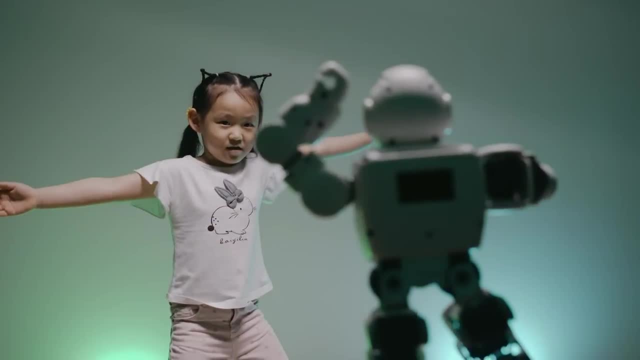 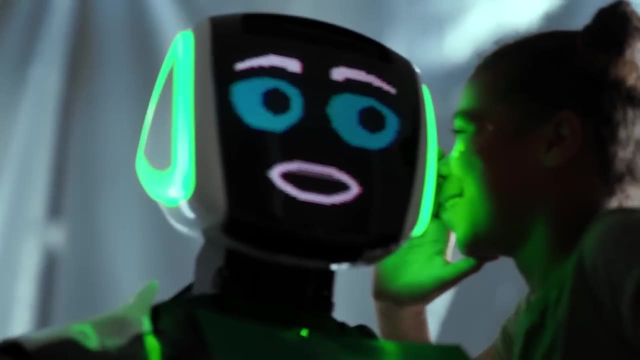 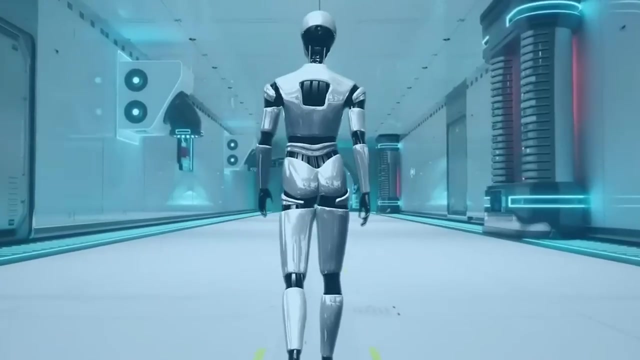 algorithms and models that can analyze and manipulate natural language data, such as text, speech and dialogue. NLP is used in various applications, such as chatbots, virtual assistants, sentiment analysis, text classification and machine translation. It involves various tasks, such 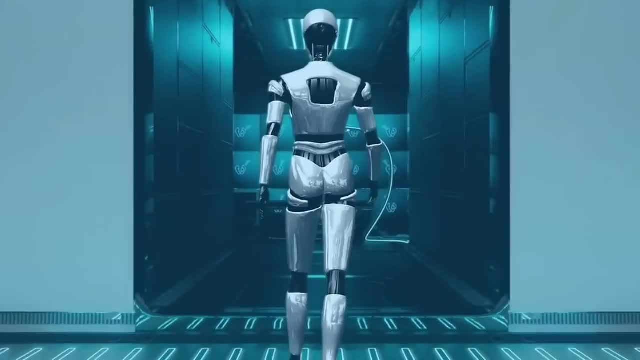 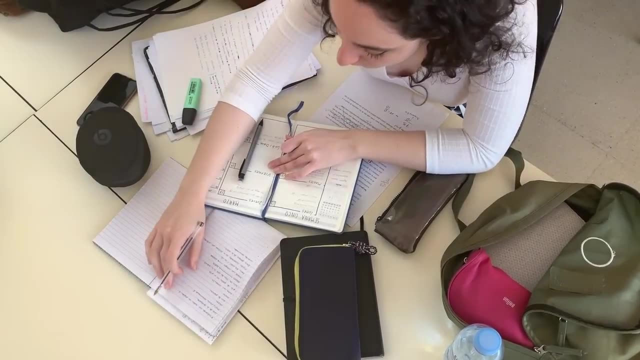 as syntactic analysis, semantic analysis and discourse analysis. Syntactic analysis involves the study of the grammatical structure of sentences, such as parts of speech, sentence structure and syntax. Semantic analysis involves the study of the meaning of words and their 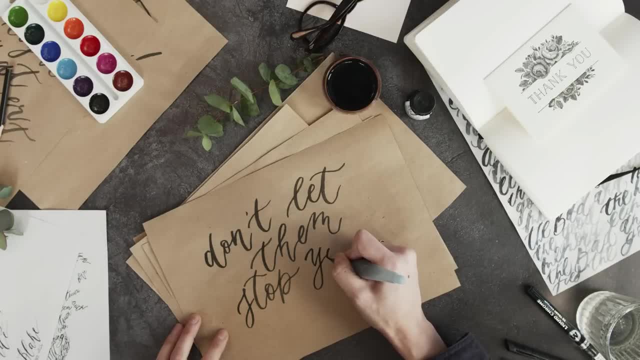 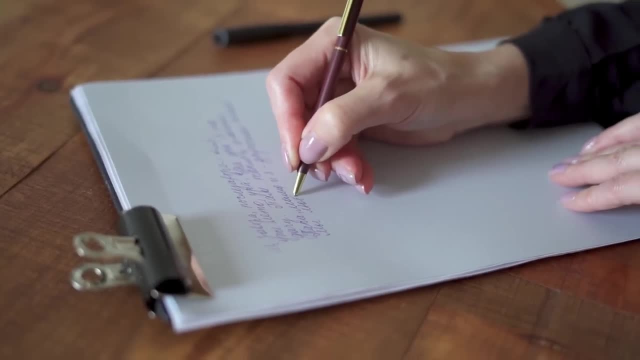 such as word-sense disambiguation and named entity recognition. Discourse analysis involves the study of the structure and coherence of text, such as topic modeling and summarization. NLP algorithms and models are typically based on machine learning and deep learning techniques. 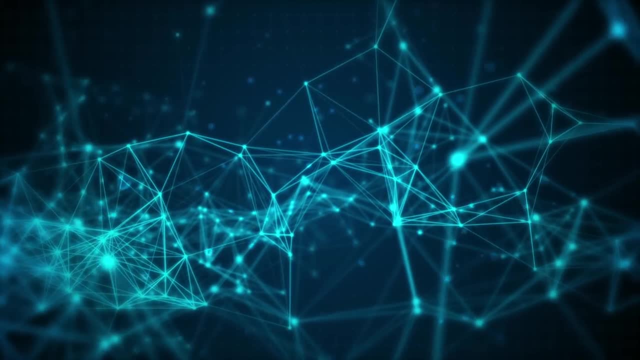 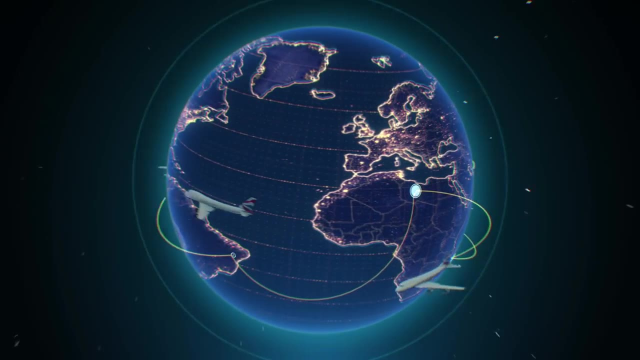 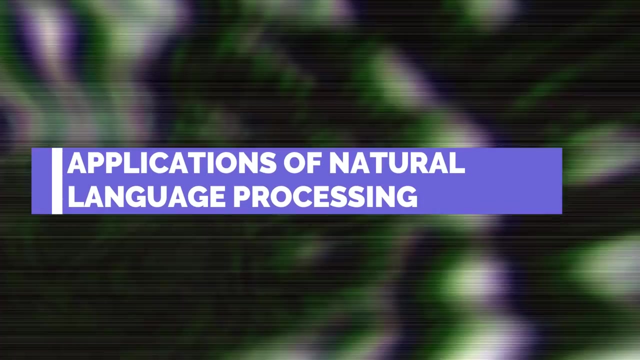 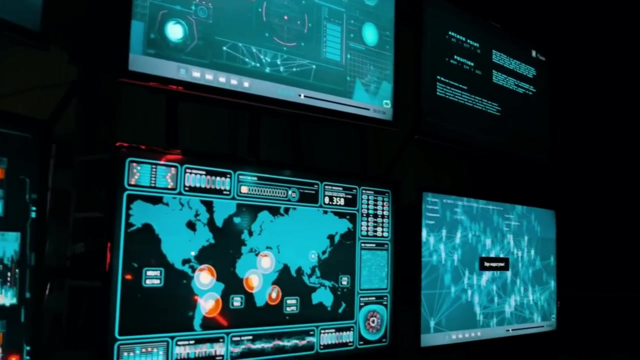 such as convolutional neural networks, CNN, and recurrent neural networks, RNN. These algorithms and models are trained on large datasets of natural language data, such as corpora and annotated datasets, to learn patterns and relationships in the data. Natural language processing. NLP has various applications in different fields. 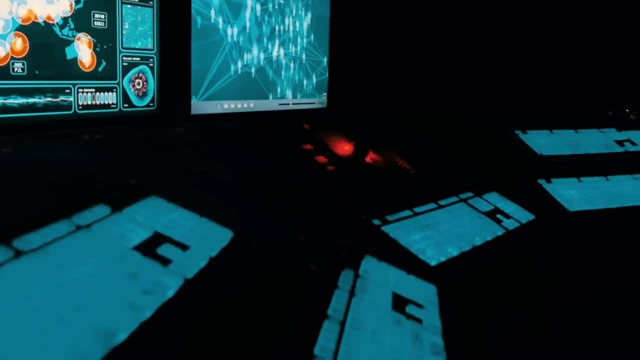 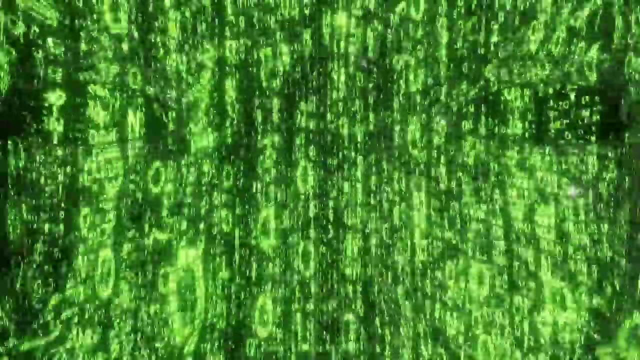 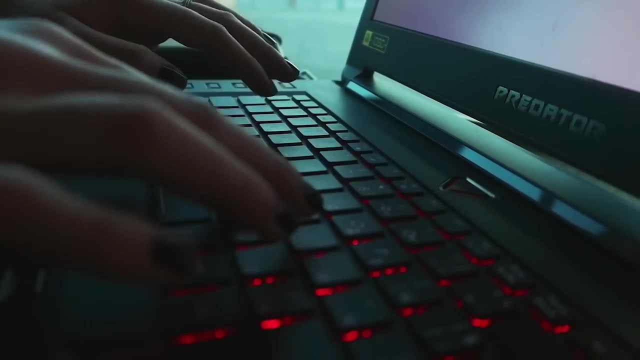 including healthcare, education, finance and customer service. Sentiment analysis. Sentiment analysis involves the analysis of text data to determine the sentiment of the text, whether it is positive, negative or neutral. It is used in various applications, such as social media monitoring. 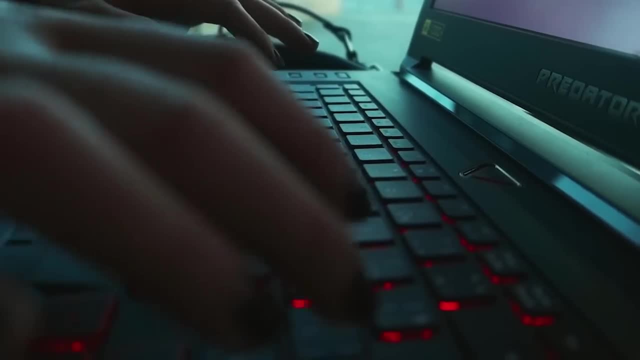 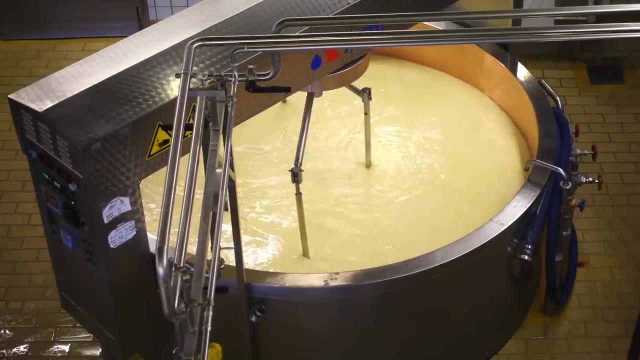 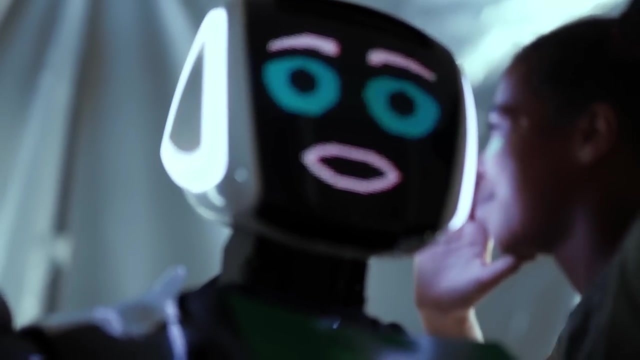 customer feedback, analysis and market research. Machine translation: Machine translation involves the automatic translation of text from one language to another. It is used in various applications such as language learning, communication and cross-border e-commerce, Chatbots and virtual assistants. 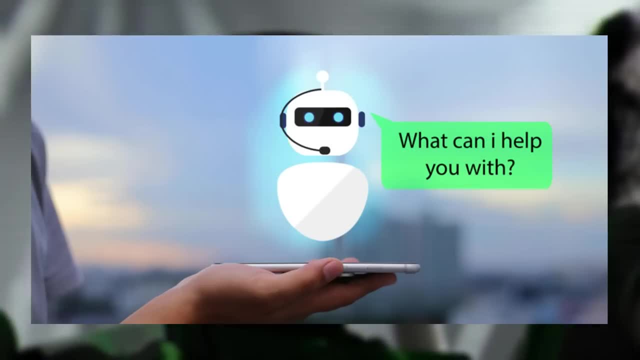 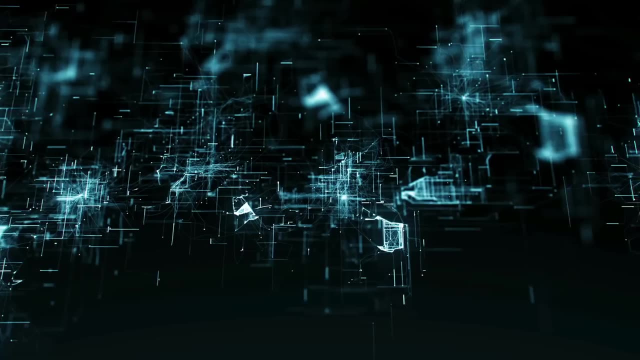 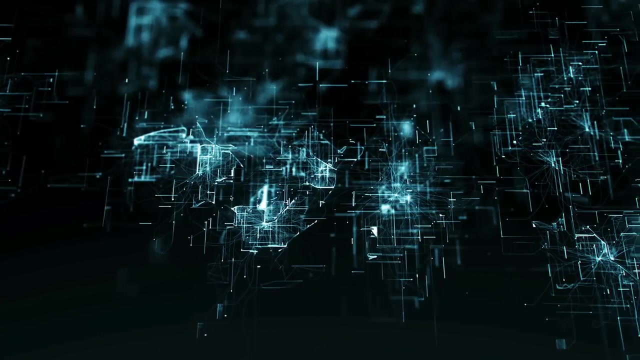 Chatbots and virtual assistants are intelligent agents that can interact with users in natural language. They are used in various applications, such as customer service, personal assistance and sales support. Named entity recognition. Named entity recognition NER involves the identification and classification of named entities and text. 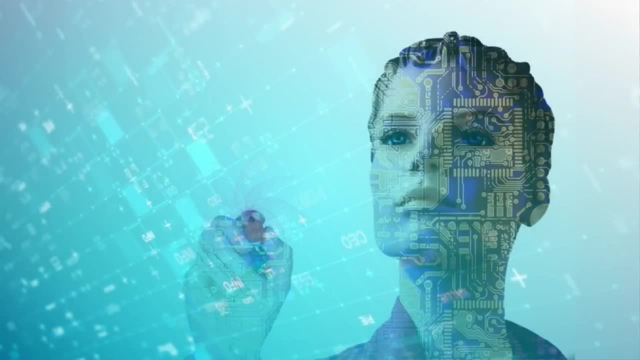 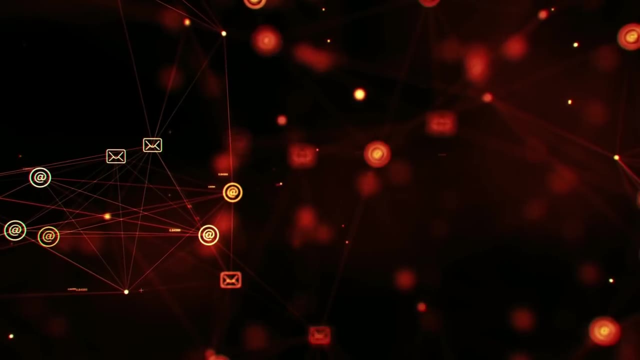 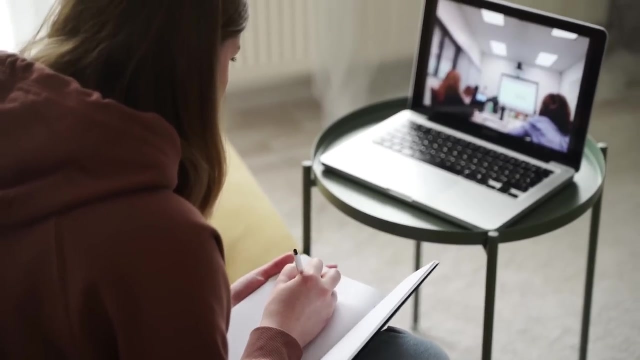 into predefined categories, such as person, organization, location and date. It is used in various applications, such as information extraction, document classification and question answering. Text summarization: Text summarization involves the extraction of key information from text data and presenting it in a condensed form. 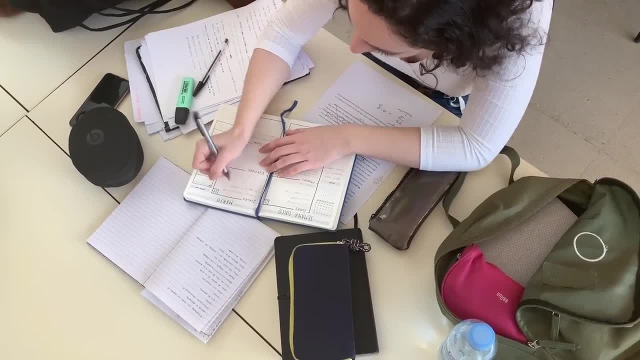 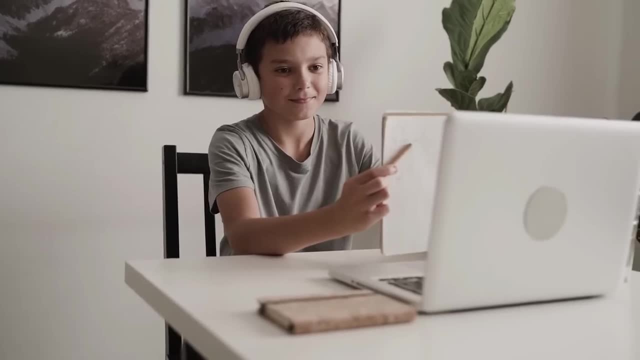 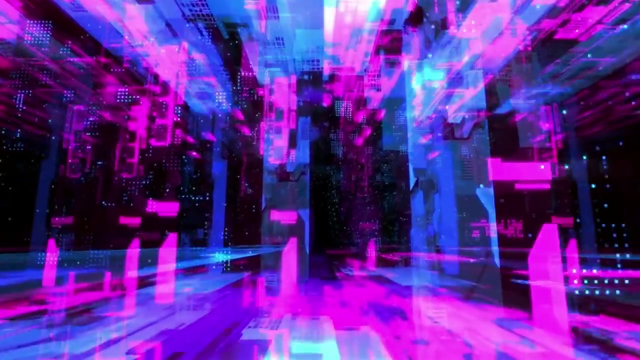 It is used in various applications such as news article summarization, document summarization and email summarization. Text classification: Text classification involves the categorization of text into predefined categories or classes. It is used in various applications such as sentiment analysis, topic modeling and spam filtering. 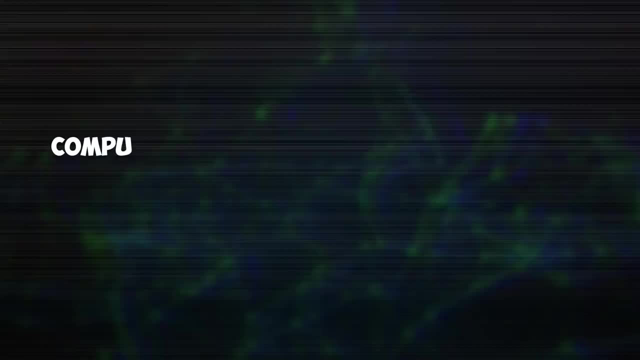 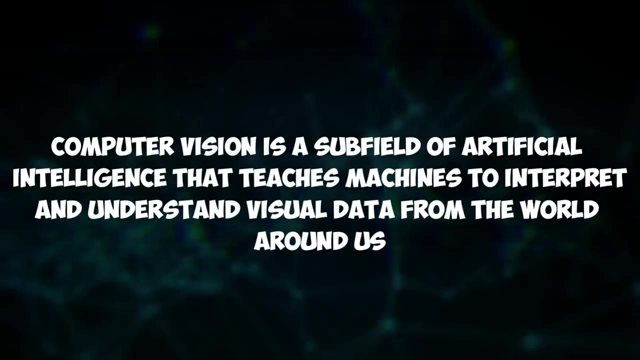 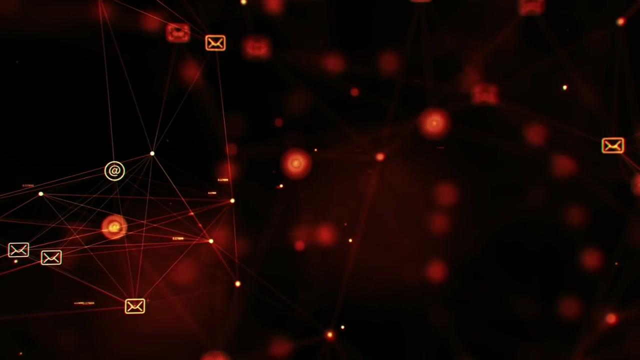 Named entity recognition. Named entity recognition. Named entity recognition: What kind of technologies do you use? Named entity recognition includes partnerships of the n PS systems and partners. to the엔eteesite a insight. Named entity recognition involves the classification and classification of yd-key at a public or private level. 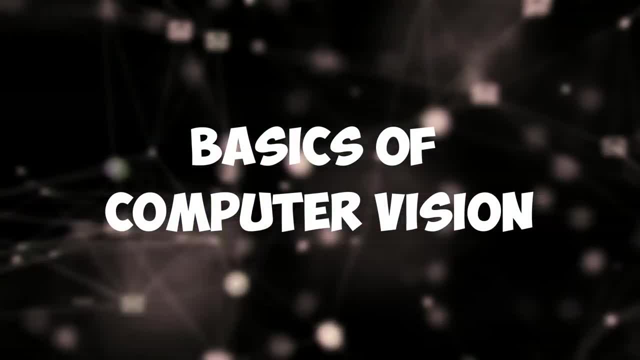 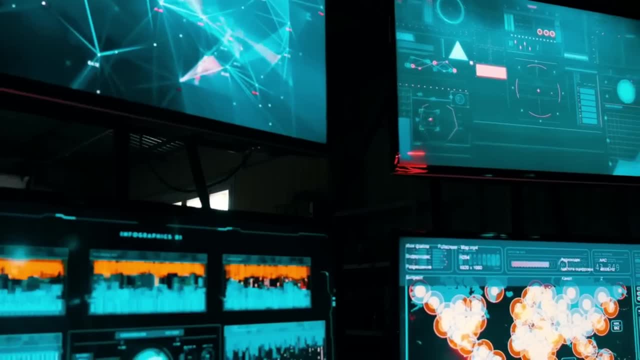 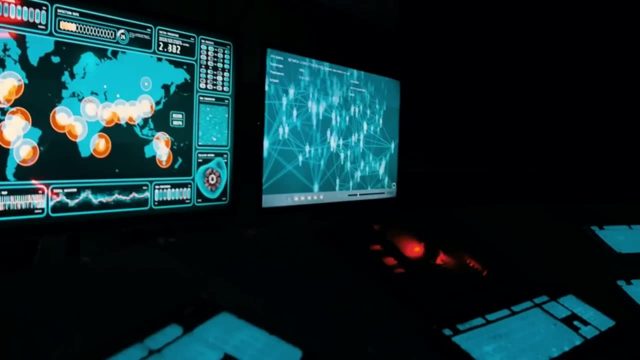 Named entity recognition involves the classification and classification of physical and physical data, Named entity recognition, visual data such as images and videos, to extract useful information. This information can then be used to perform a variety of tasks, such as recognizing objects, detecting faces and tracking. 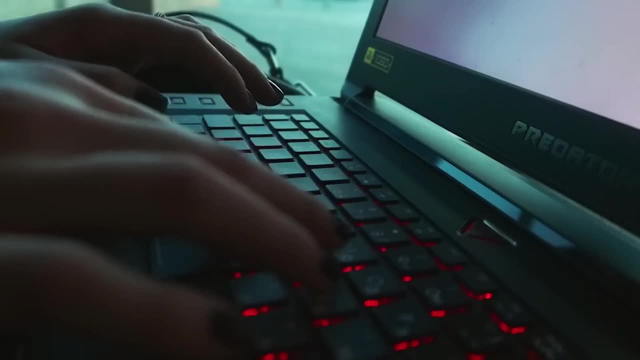 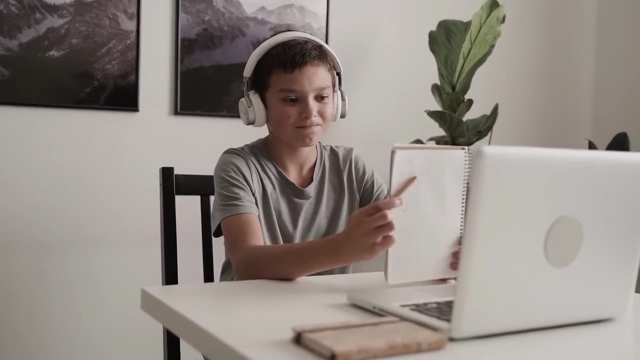 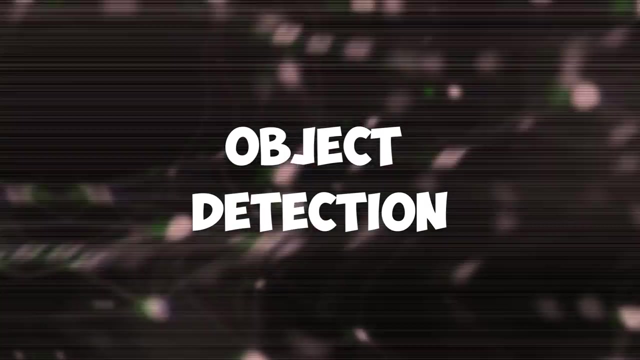 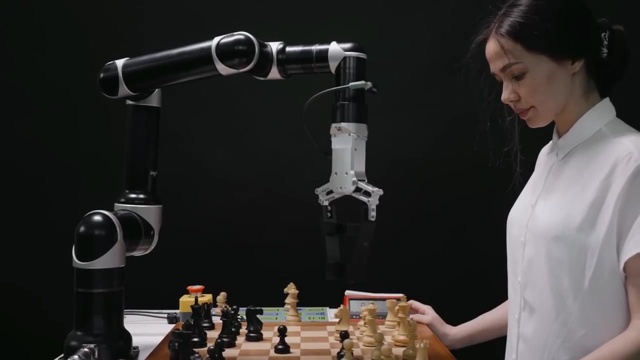 movements. Image recognition is a fundamental task in computer vision. It involves identifying objects or patterns within an image. Machine learning algorithms are trained on large data sets of labeled images to recognize different objects and patterns. Object detection is a more complex task that involves identifying specific objects within an image and drawing bounding boxes. 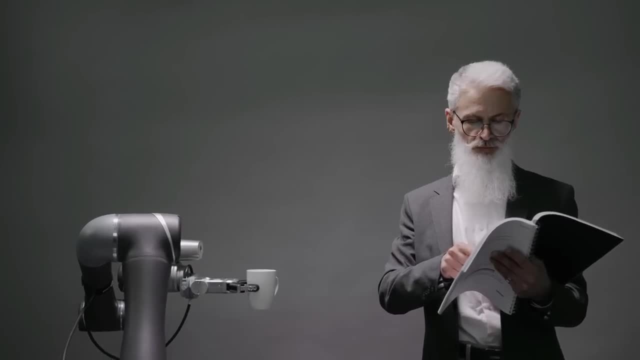 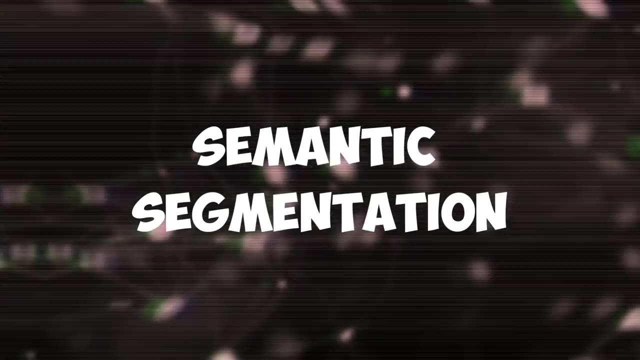 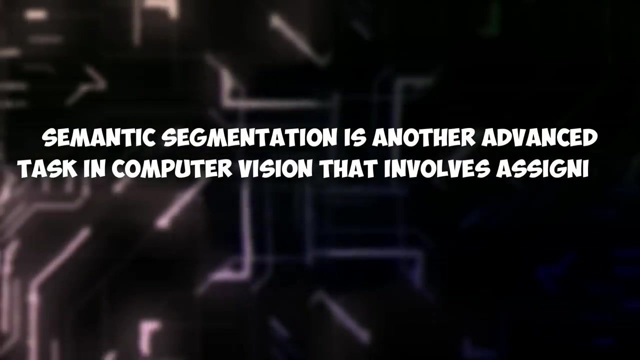 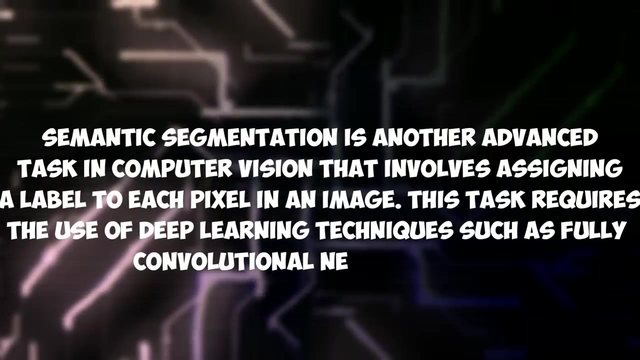 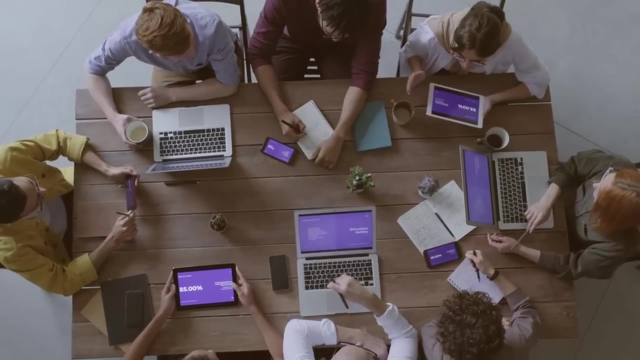 around them. This task requires the use of advanced algorithms such as YOLO- You Only Look Once- and RCNN, region-based convolutional neural networks. Semantic segmentation is another advanced task in computer vision. Computer vision involves the use of various machine learning and deep learning techniques. 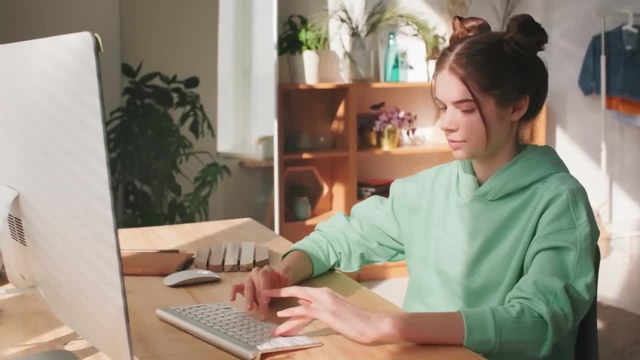 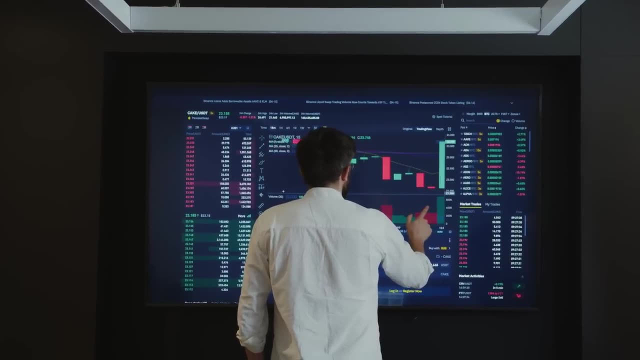 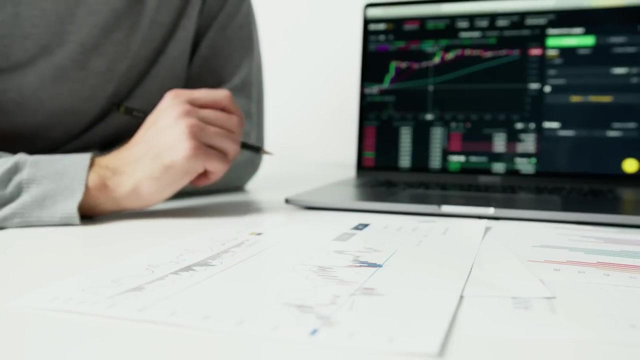 to analyze and interpret visual data. Convolutional neural networks are the most commonly used deep learning technique in computer vision. They consist of layers of interconnected neurons that can learn to recognize specific objects. Other deep learning techniques used in computer vision include recurrent neural networks. 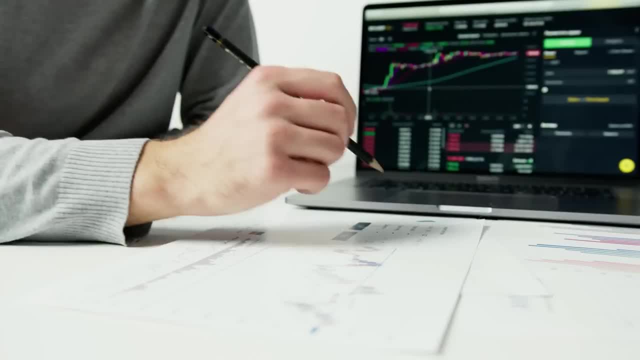 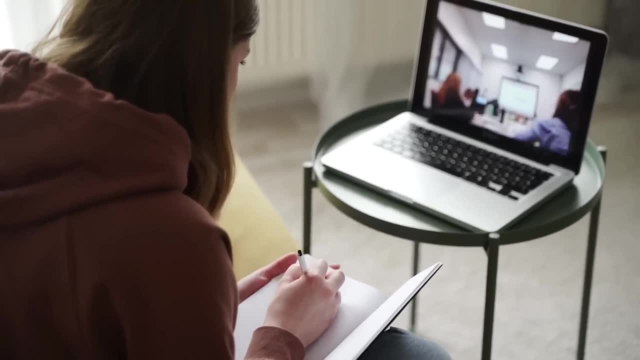 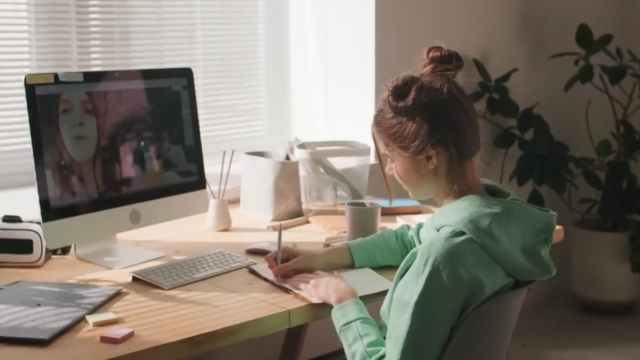 RNN, generative adversarial networks, GAN and deep reinforcement learning. Computer vision faces several challenges, including noisy, low-quality and large-scale data. Another challenge is ensuring that the algorithms used in computer vision are robust to changes in lighting conditions, scale and rotation. 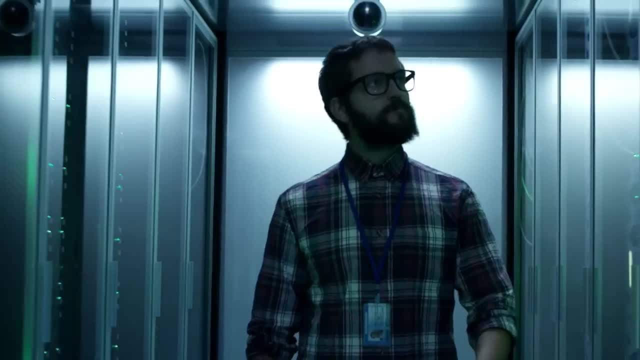 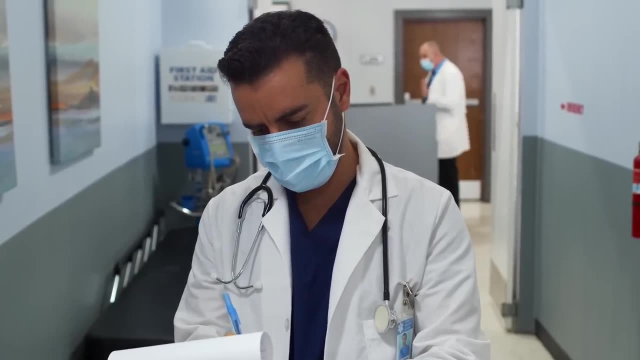 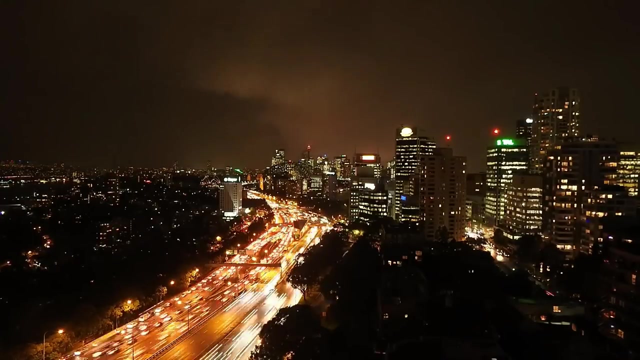 Computer vision has a wide range of applications in different industries, including healthcare, security and manufacturing. In healthcare, computer vision is used to analyze medical images and assist in the diagnosis of diseases. In security, computer vision is used for facial recognition and object detection to improve public safety. 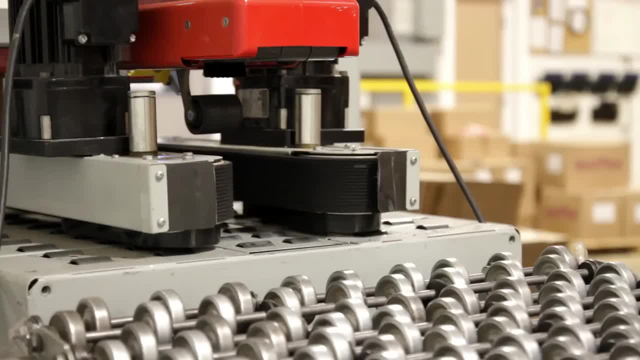 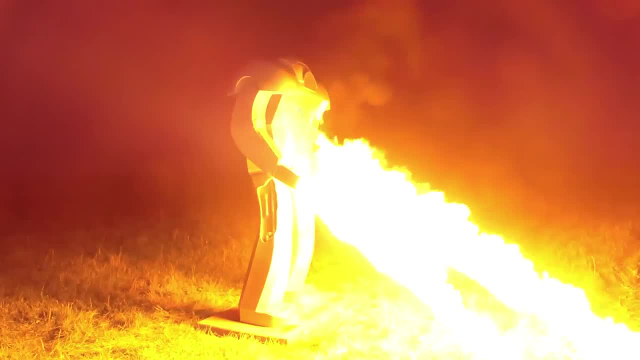 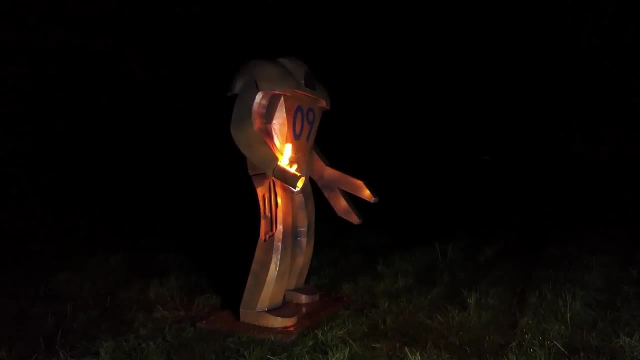 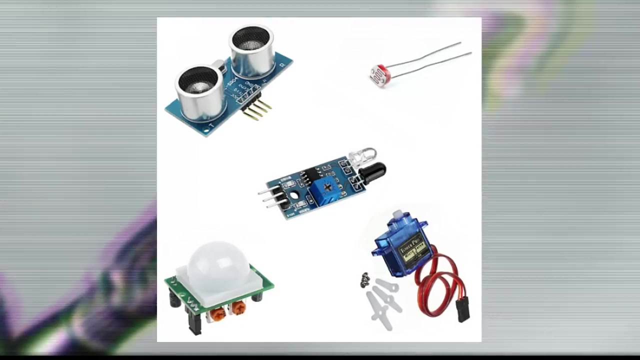 In manufacturing. computer vision is used for quality control and defect detection in production lines. Robotics and AI are two closely related fields that are working together to create advanced robotic systems that can perform tasks autonomously. A robotic system consists of several key components, including sensors, actuators and control. 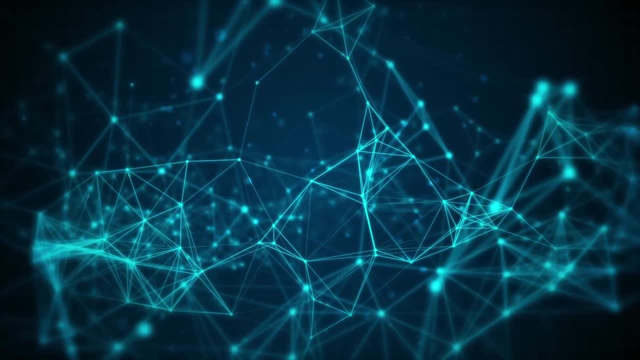 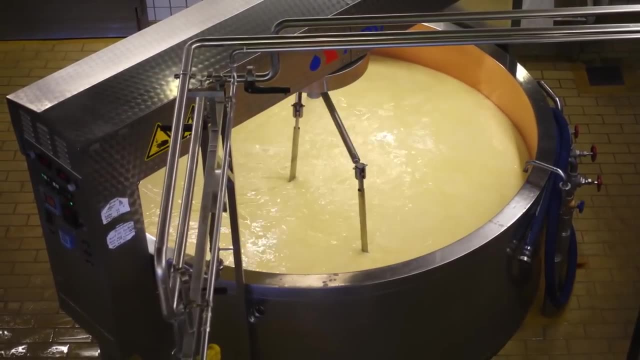 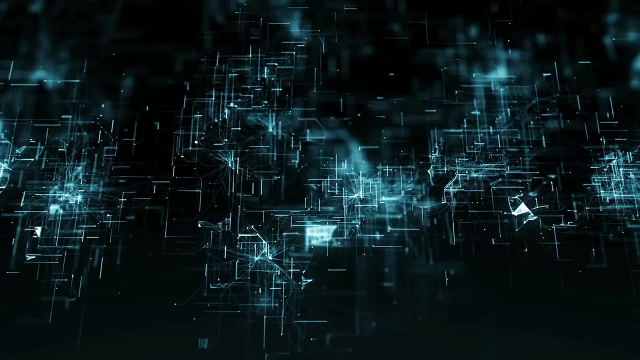 systems. Sensors are used to detect and measure the physical world, while actuators are used to manipulate it. Control systems are used to interpret sensor data. AI algorithms are used to provide decision-making capabilities to the control system. The AI algorithms take in sensor data and provide commands to the control system to determine. 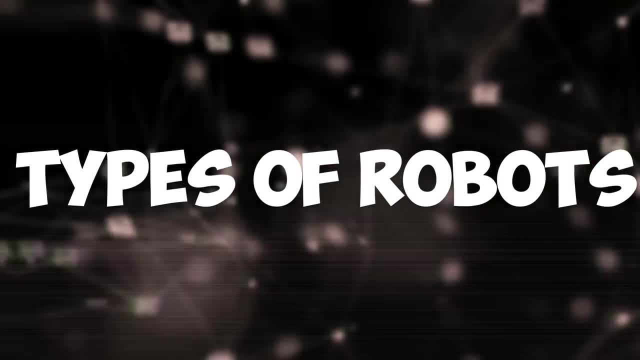 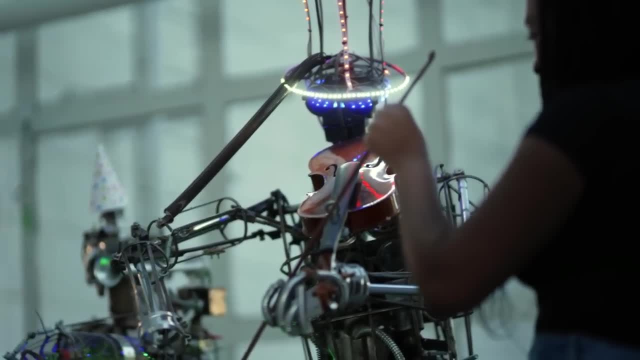 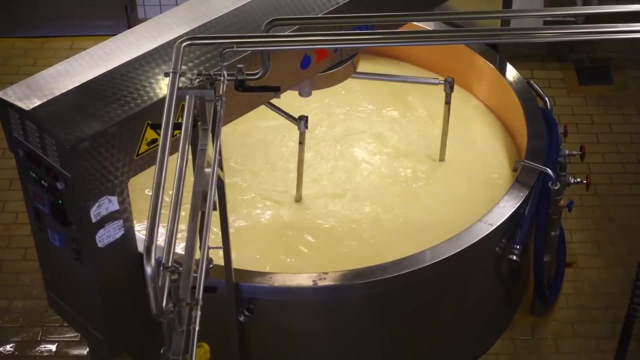 how the robotic system should act. There are many different types of robots, each with their own unique set of challenges. Some examples of robots include: Industrial robots: These robots are used in manufacturing and perform tasks such as welding in assembly. autonomous robots: these robots are used in environments that are dangerous or 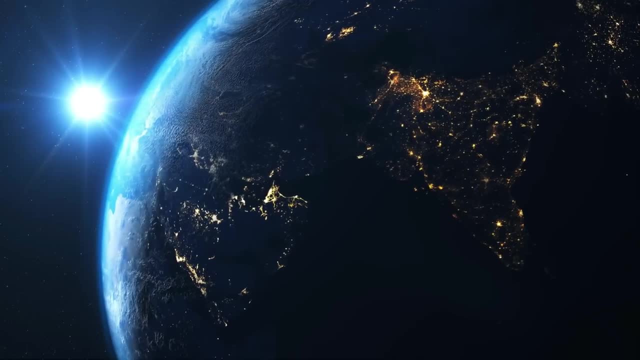 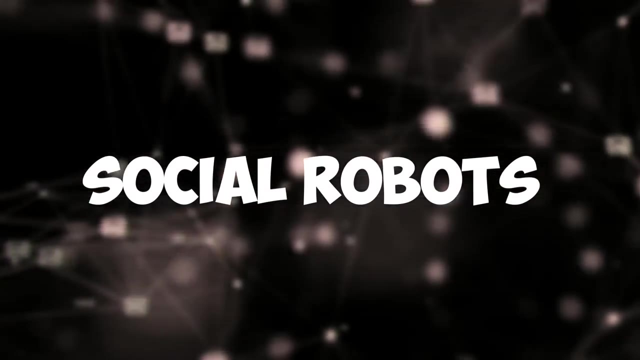 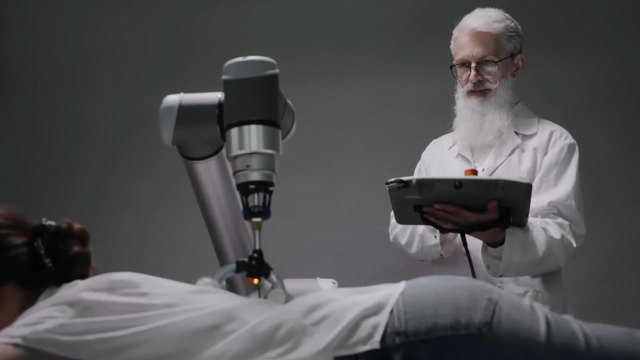 difficult for humans to operate in. for example, autonomous robots can be used in space exploration, where humans cannot survive without life support. social robots: these robots are designed to interact with humans and provide assistance or companionship. for example, social robots can be used in healthcare settings to help patients with tasks or provide companionship. one of the 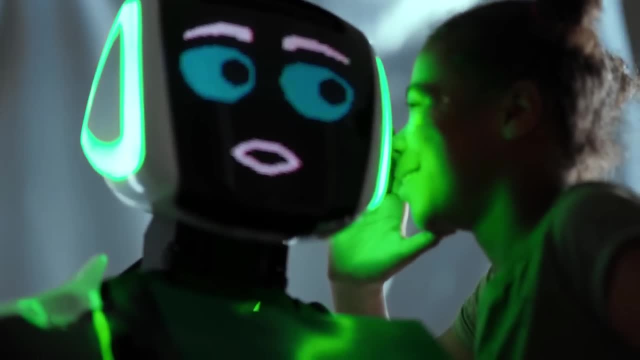 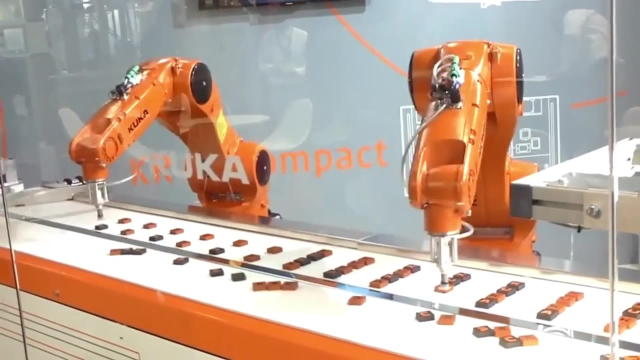 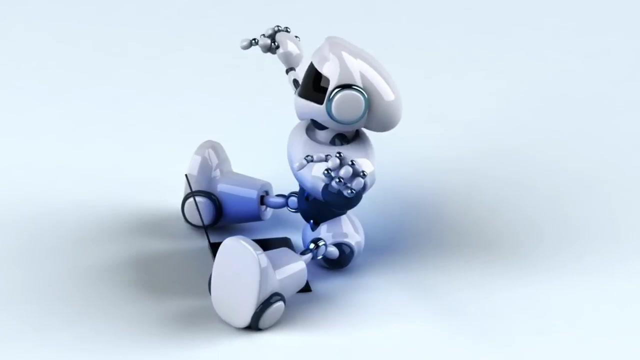 key challenges in the field of robotics and ai is the need for reliable and accurate performance. this requires the development of sophisticated algorithms and control systems, as well as the use of advanced sensing technologies and hardware. another challenge is the ethical implications associated with advanced robotic systems. for example, there are concerns about the potential 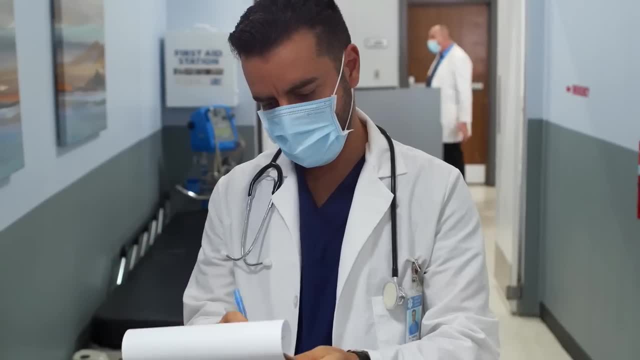 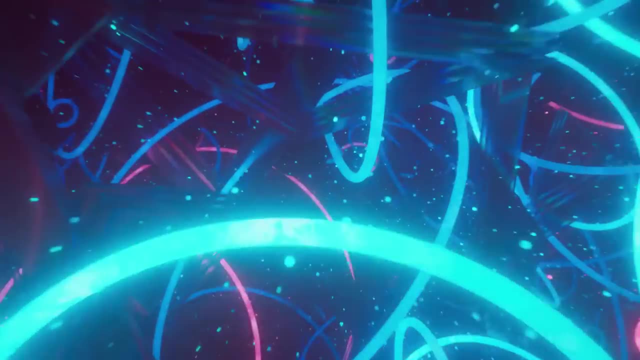 for job displacement. as robots become more advanced and are able to perform tasks that were previously done by humans, there's also a need to ensure safety and safety of the robot. there's also a need to ensure safety and accountability in autonomous systems. as robots become more intelligent and autonomous, there is a risk of unintended consequences if they 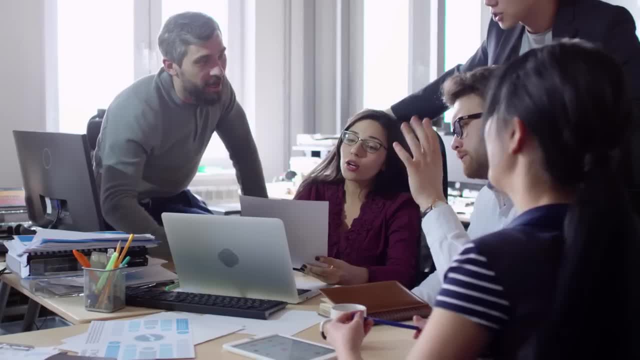 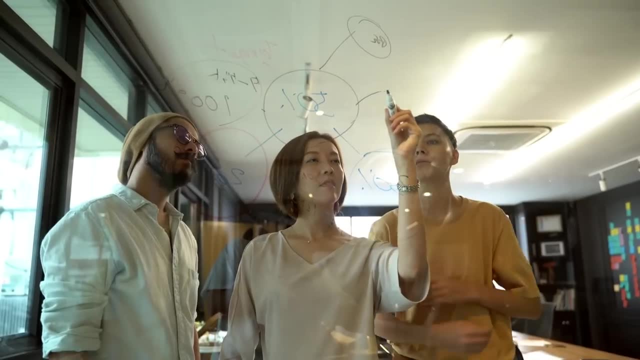 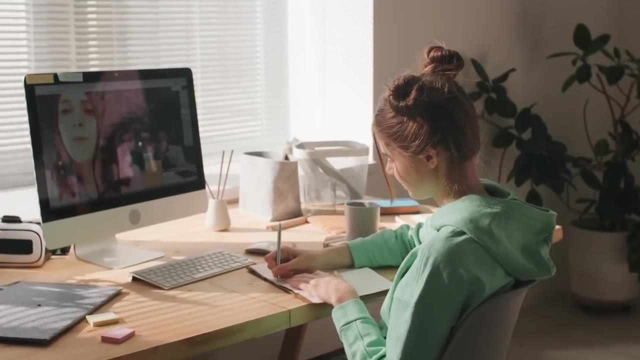 are not programmed correctly. as the use of advanced robotic systems becomes more widespread, there are ethical implications that must be considered. one of the key ethical concerns is the potential for job displacement as robots become more advanced and are able to perform tasks that were previously done by humans. another ethical concern is the potential. 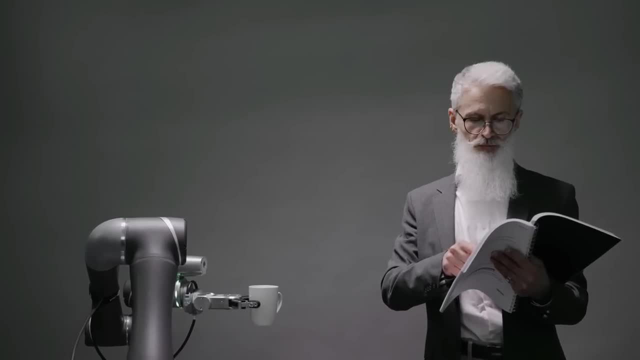 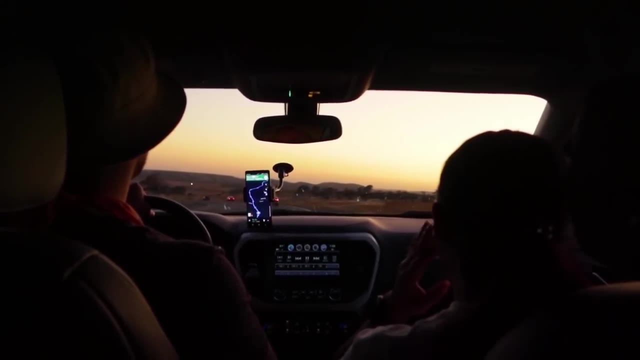 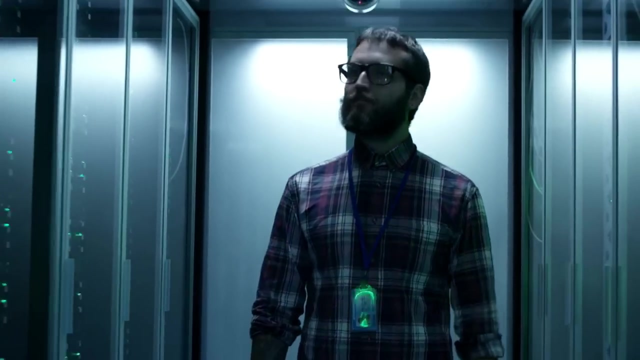 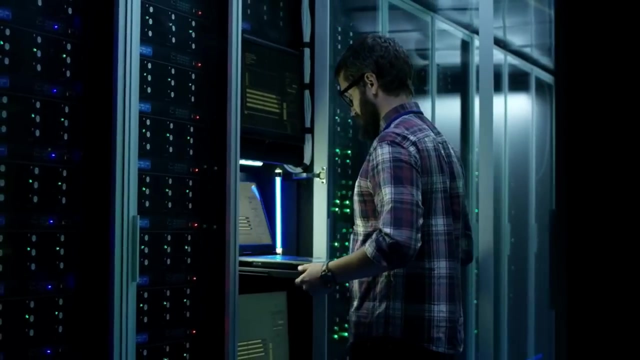 for unintended consequences if robots are not programmed correctly. for example, a self-driving car may make a decision that is harmful to humans if it is not programmed to prioritize human safety. as robotics and artificial intelligence ai continue to advance, the potential applications of these technologies are becoming increasingly diverse and exciting. let's explore some of the 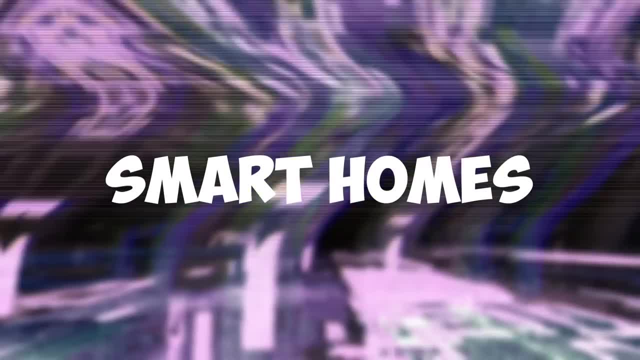 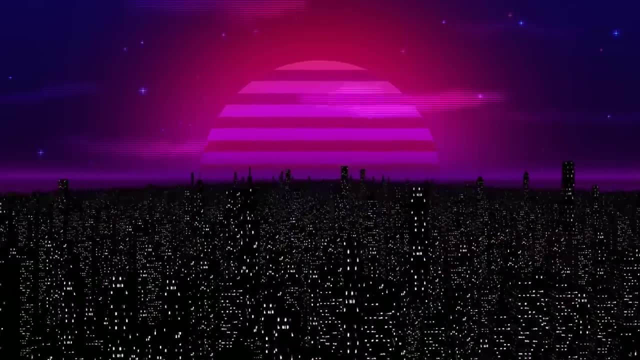 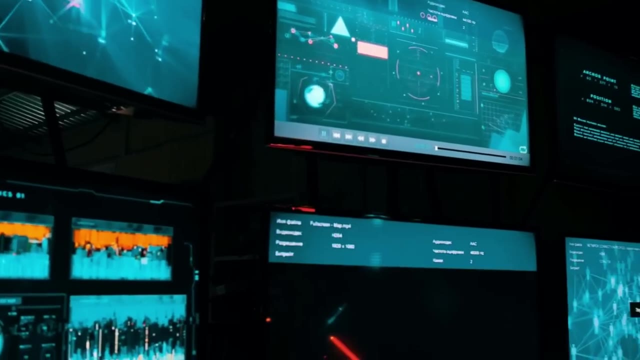 potential future applications of robotics and ai. one potential application of robotics and ai is in the development of smart homes. smart homes are homes that are equipped with sensors, cameras and other technologies that allow for remote monitoring and control of various systems and appliances. for example, a smart home, 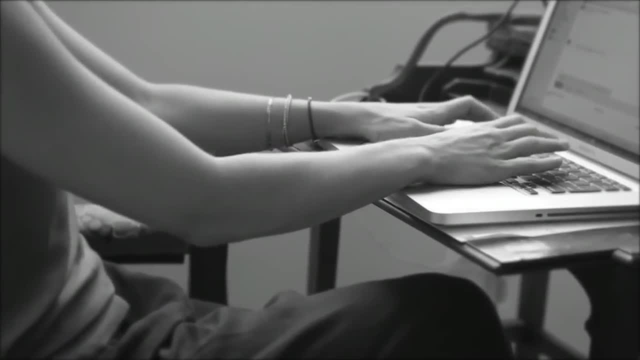 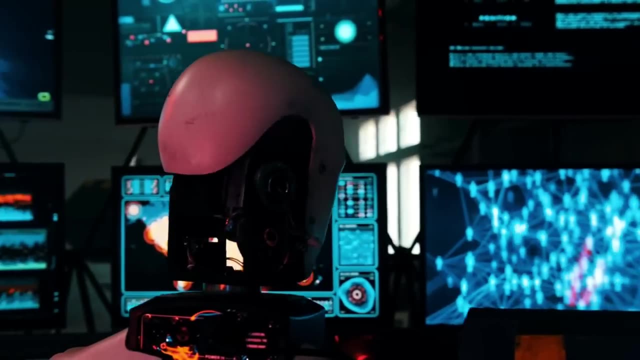 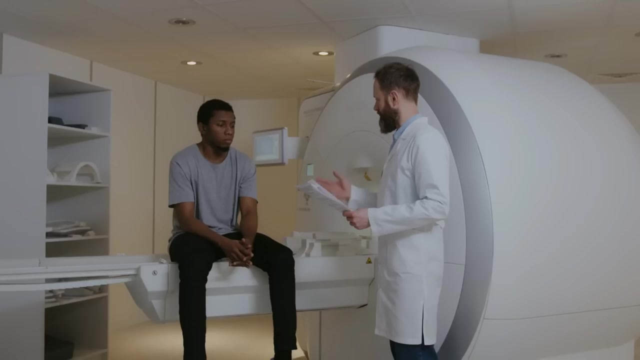 could be equipped with a robotic vacuum cleaner that automatically cleans the floors when the homeowner is away. in addition, smart homes could be equipped with ai powered personal assistance that can help with tasks such as cleaning the floors and cleaning the floors of the home, such as scheduling appointments and ordering groceries. another potential application of 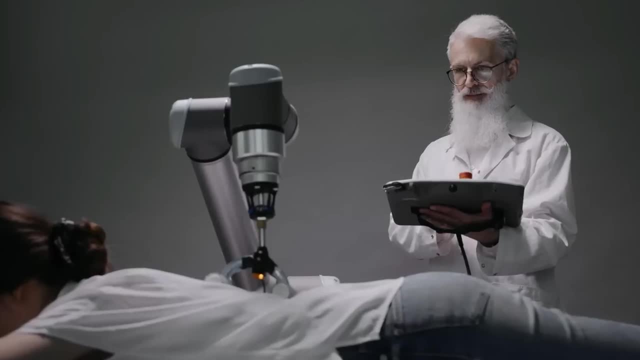 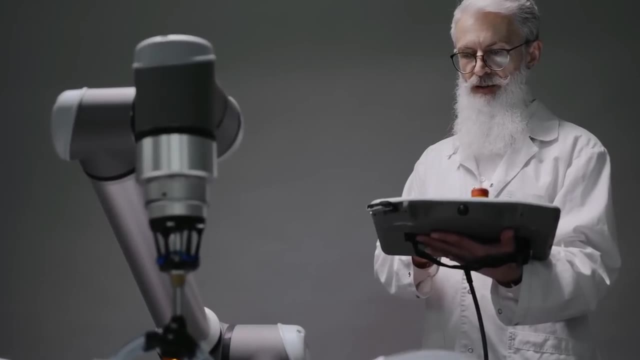 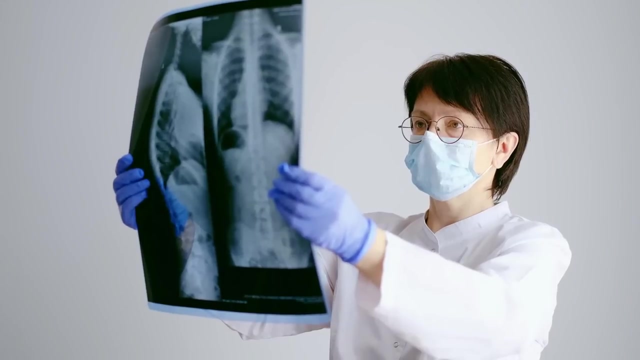 robotics and ai is in the healthcare industry. robots and ai systems could be used to monitor patients and provide assistance with tasks such as administering medication and providing physical therapy. for example, a robot could be used to monitor a patient's vital signs and alert healthcare providers if there are any changes that require attention. in addition, robots could be used to: 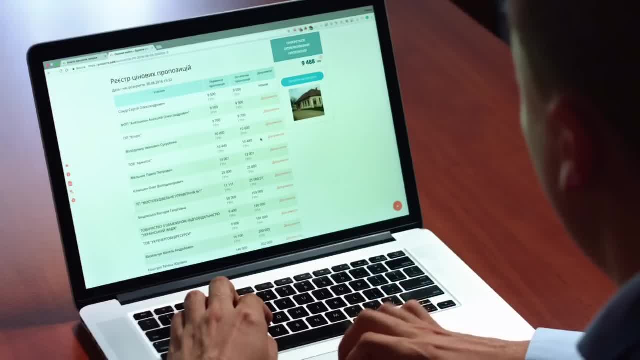 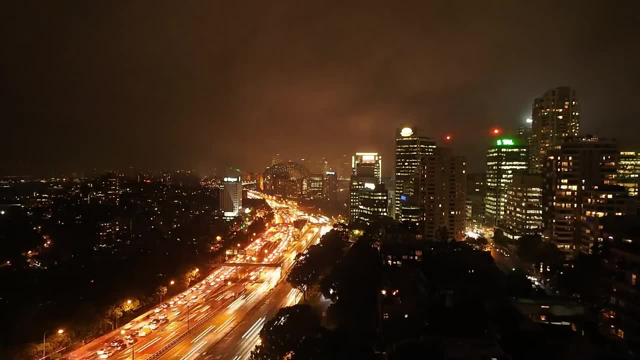 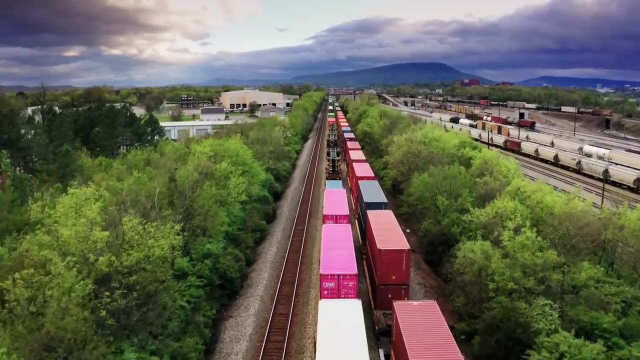 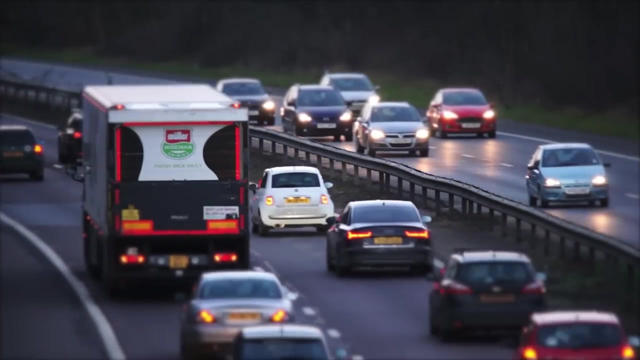 assist with physical therapy, providing patients with personalized feedback and guidance. robots and ai systems could also have a significant impact on transportation. self-driving cars and trucks are already being developed and tested, and these systems have the potential to greatly reduce accidents and improve traffic flow. in addition, robots could be used for 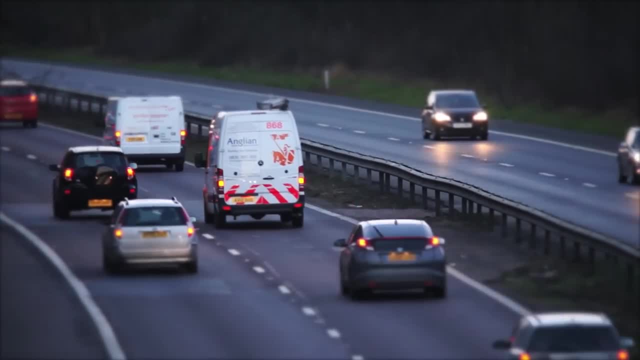 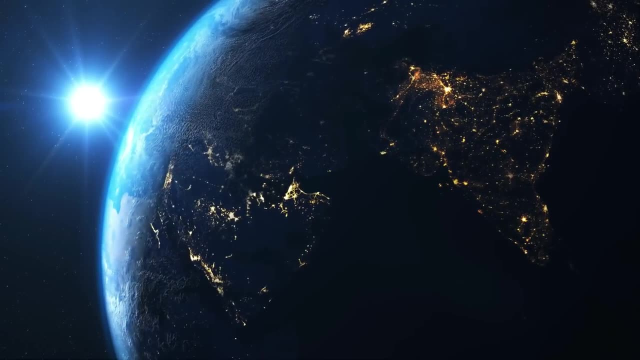 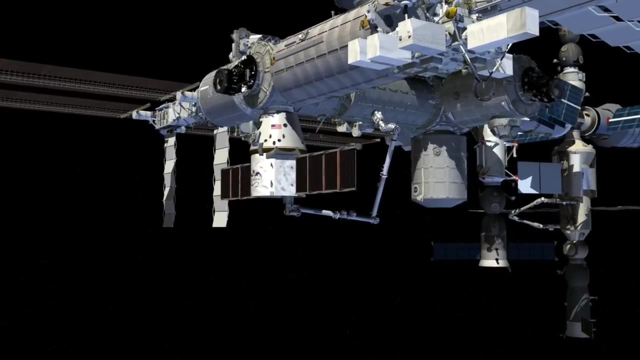 tasks such as package delivery, reducing the need for human drivers and improving efficiency. finally, robotics and ai could play a significant role in space exploration. ebahn Sketch robots could be used to explore the surface of other planets and moons, collecting samples and conducting experiments. in addition, robots could be used to build and maintain infrastructure on other planets, making it possible for 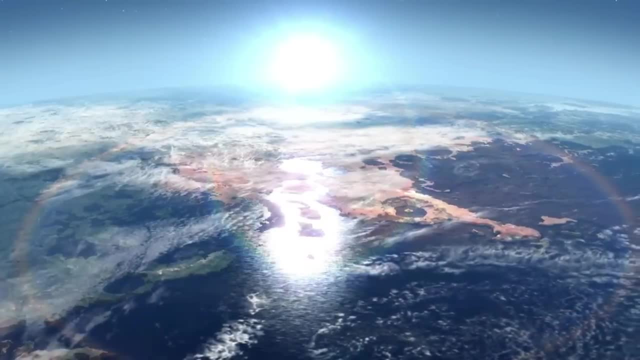 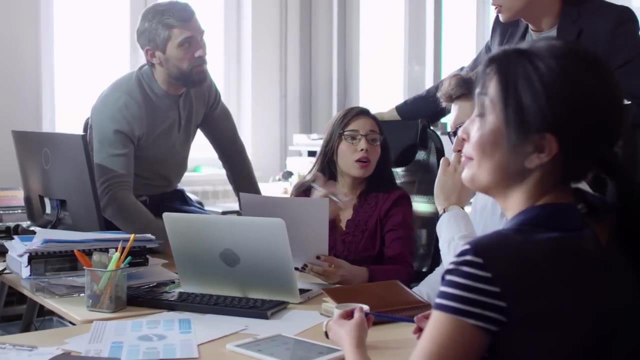 humans to live and work in space for extended periods of time. artificial intelligence- artificial intelligence ai- is rapidly gaining virtual burns. artificial intelligence ai is rapidly getting darkening nutrients and drinks from human cells through artificial, implicit AIem roadmaping to enable artificial intelligence. hey, either you can either accept artificial intelligence or artificial intelligence, or artificial intelligence right away, or stop artificial intelligence. but you can get the final brain than artificial intelligence is an important principle and that's going to boost the genre of AI which is the core of AI. 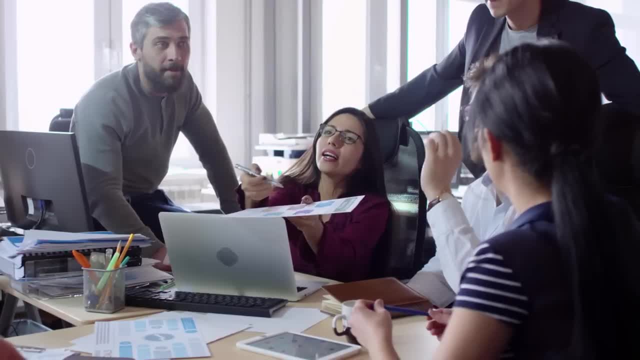 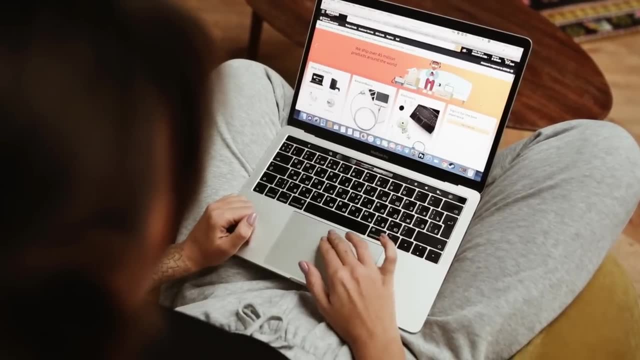 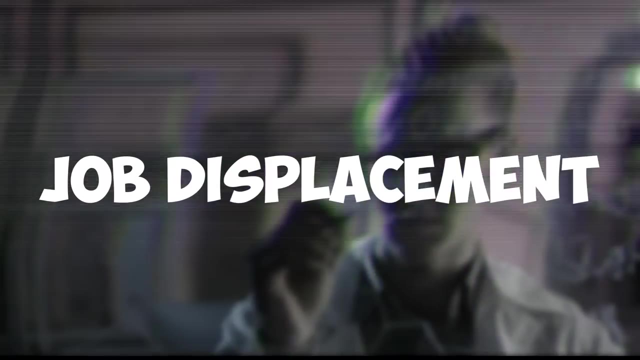 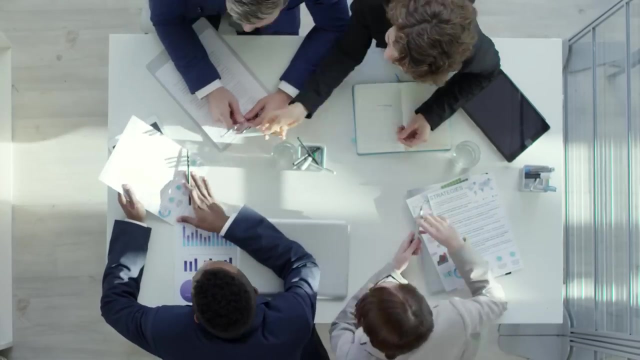 rapidly transforming the job market, with some jobs becoming automated and new jobs emerging that require AI skills. While AI has the potential to improve efficiency and productivity in many industries, it is also creating concerns about job displacement and the need for new skill sets. One of the most significant impacts of AI on employment is the potential for job displacement. 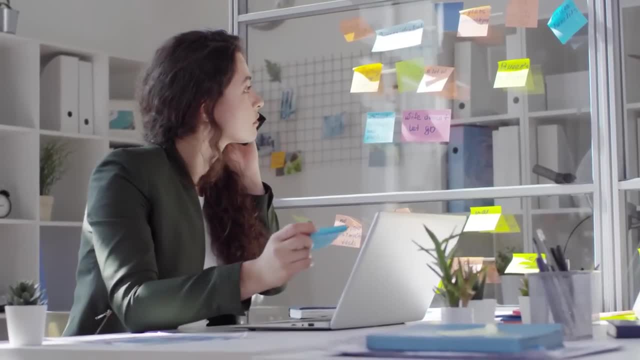 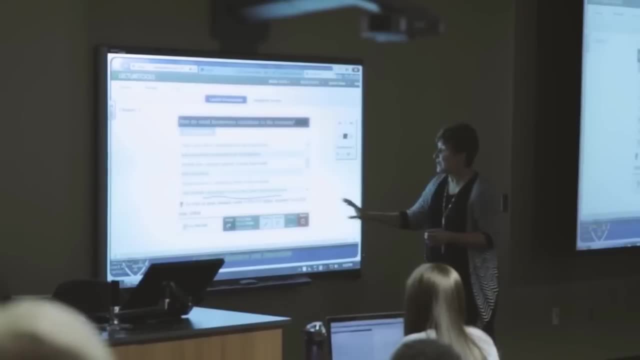 As AI becomes more advanced, it has the ability to automate tasks that were previously performed by humans, such as data entry, customer service and manufacturing. This has led to concerns about the loss of jobs and the need for workers to acquire new skills in order to remain employable. 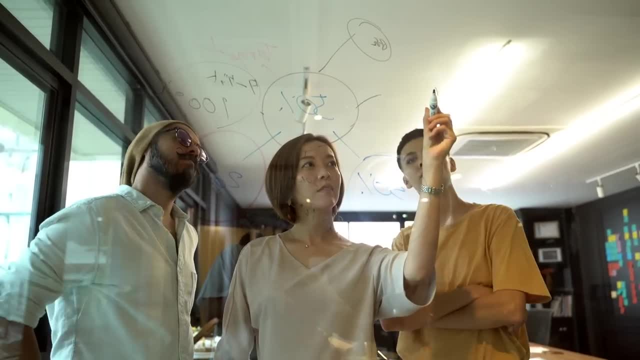 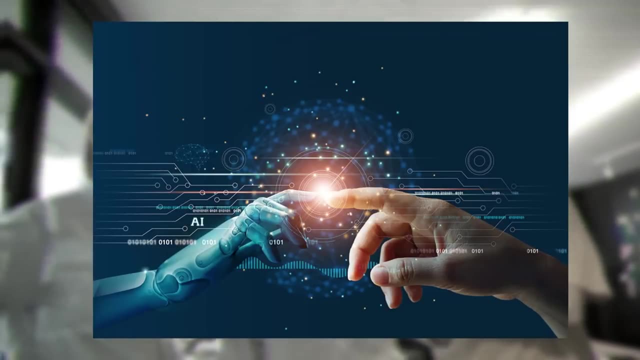 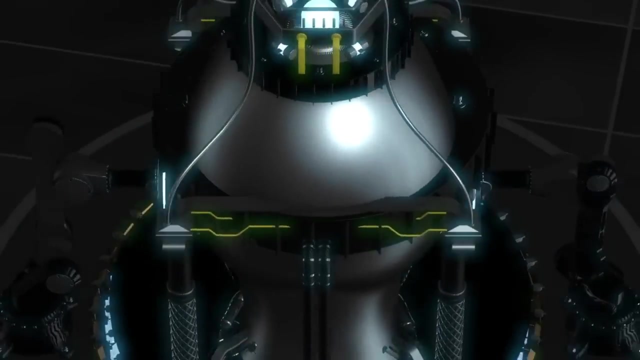 However, it is important to note that, while AI may lead to job displacement in certain industries, it is also creating new job opportunities in other areas, such as AI development and data analysis. As AI continues to evolve, it is creating new job opportunities that require specialized 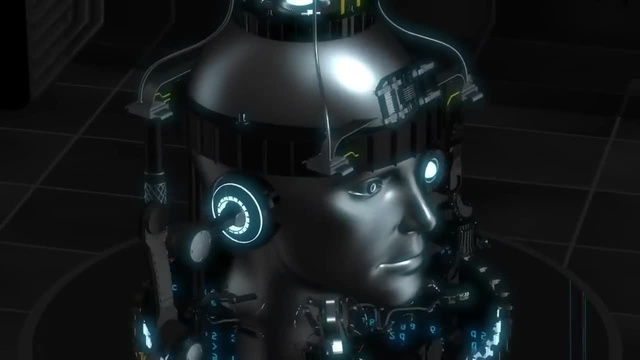 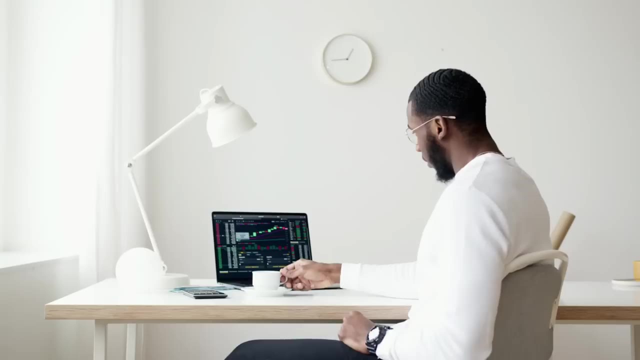 skills in AI development, data analysis and machine learning. These jobs are in high demand and offer high salaries, making them an attractive career choice for many workers. In addition, AI is also creating new job opportunities in industries that are leveraging AI to improve. 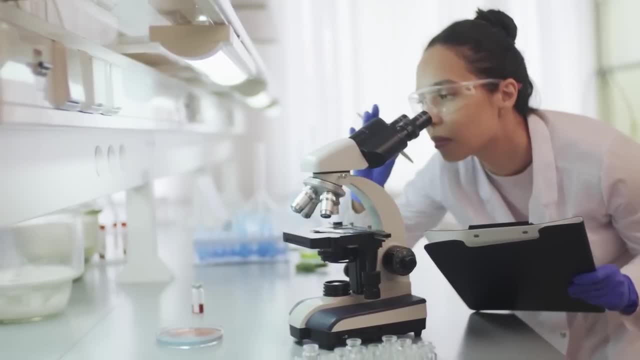 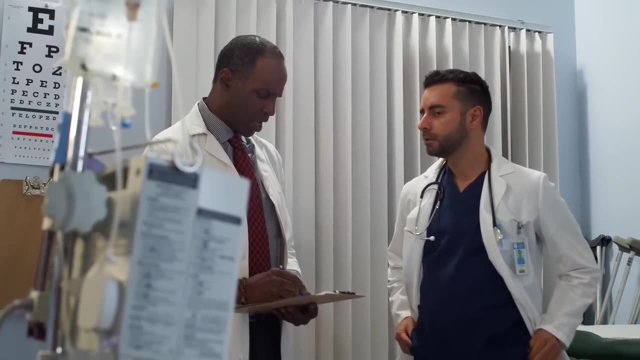 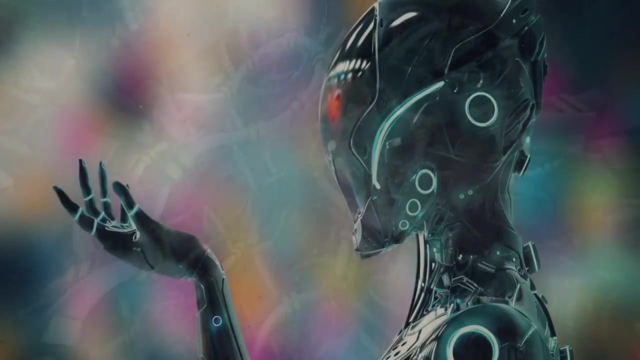 efficiency and productivity. For example, in the healthcare industry, AI-powered tools are being used to improve patient outcomes and reduce costs, Creating new job opportunities for healthcare professionals who have expertise in AI. As AI continues to transform the job market, it is also creating a need for new skill sets. Workers who are able to adapt to these changes and acquire new skills will be better positioned to remain employable in the future. Some of the skills that are in high demand in the AI job market include programming languages such as Python and R, data analysis and machine learning skills. 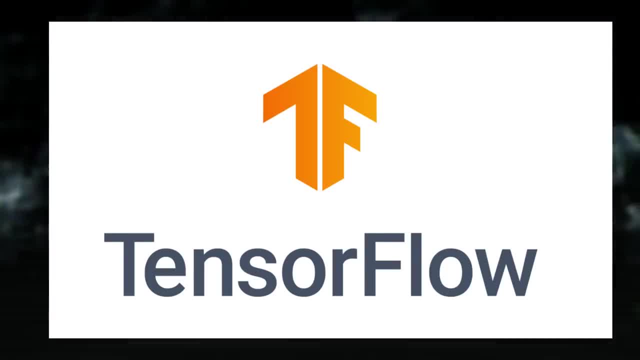 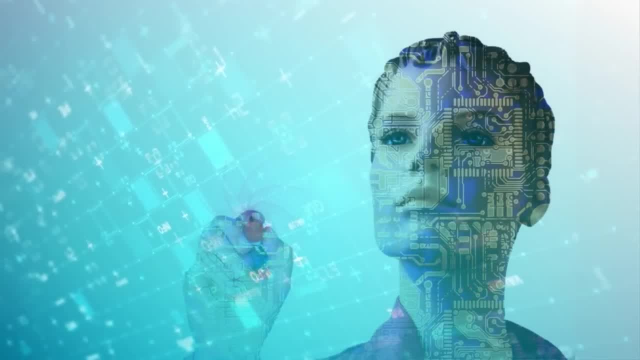 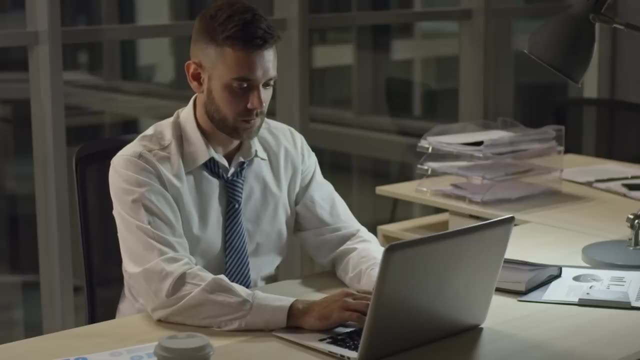 And experience with AI development. In order to address the need for new skills in the AI job market, many companies and organizations are implementing upskilling and reskilling programs for their employees. These programs provide workers with the opportunity to acquire new skills and stay competitive. 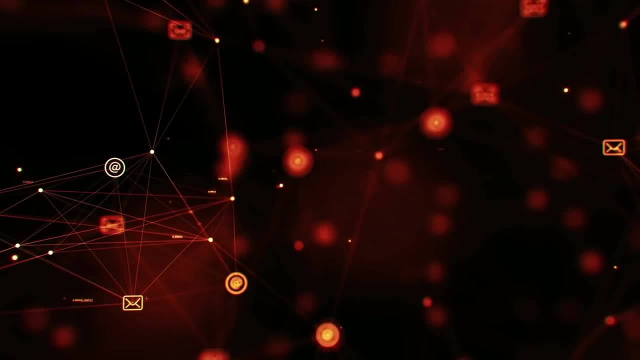 in the job market. In addition, governments and educational institutions are also implementing programs to support the development of AI skills. For example, in the United States, there are many companies and organizations that are implementing upskilling and reskilling programs for their employees. 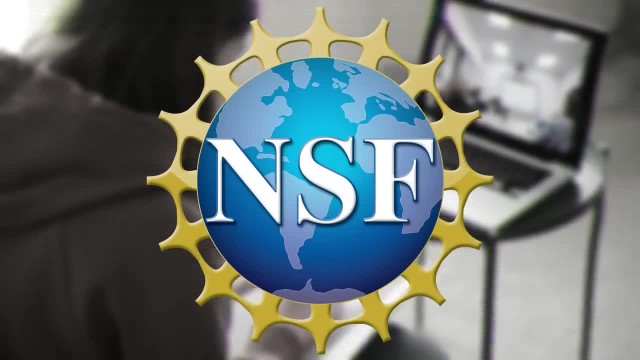 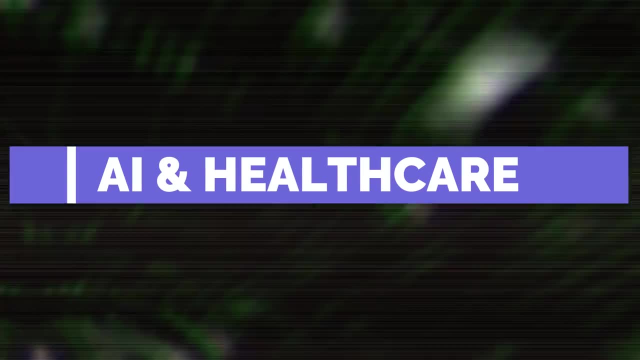 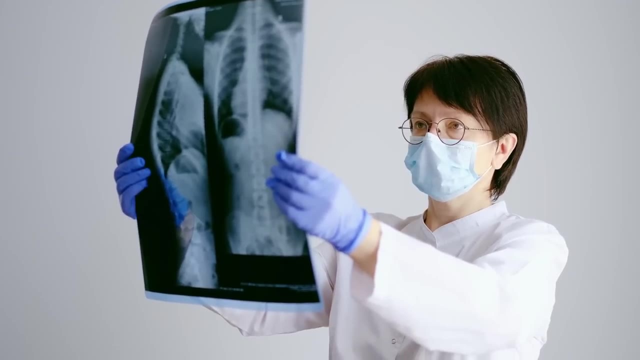 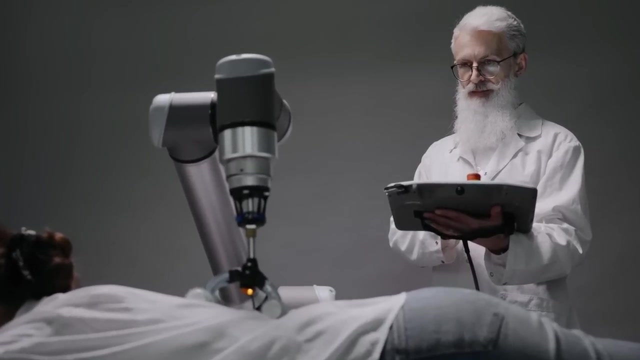 In the United States, the National Science Foundation has launched a program to support the development of AI skills and promote AI research. Artificial intelligence is transforming the healthcare industry by improving patient outcomes, reducing costs and streamlining administrative tasks From diagnosis to treatment. AI is being used to enhance the accuracy and efficiency of 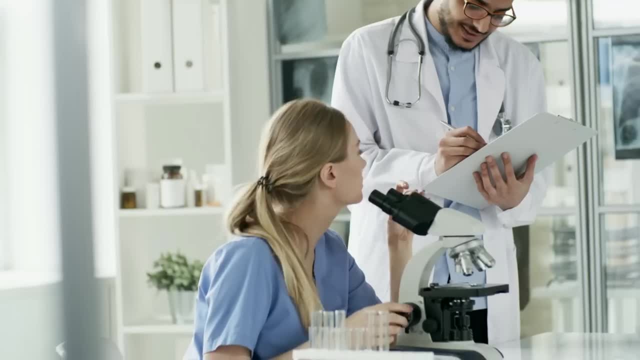 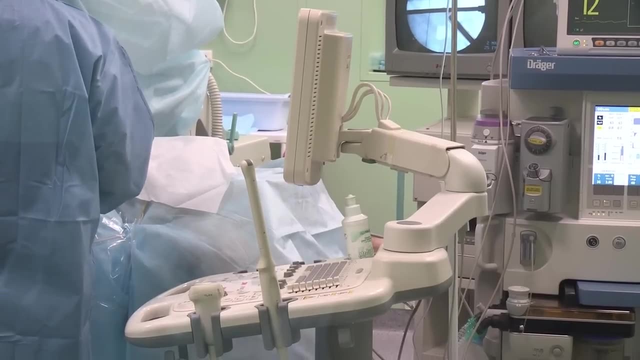 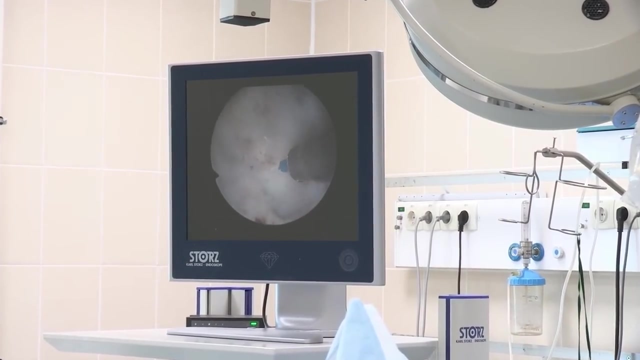 healthcare services. AI is being used to improve the accuracy and speed of medical diagnosis and treatment. Machine learning algorithms can analyze large datasets of medical information and identify patterns that may be difficult for humans to detect. This can help healthcare professionals to make more accurate diagnoses and develop personalized 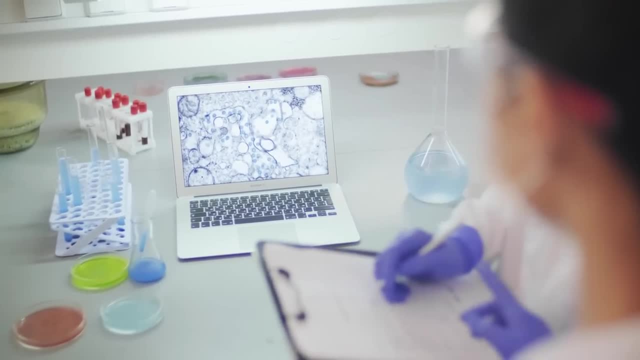 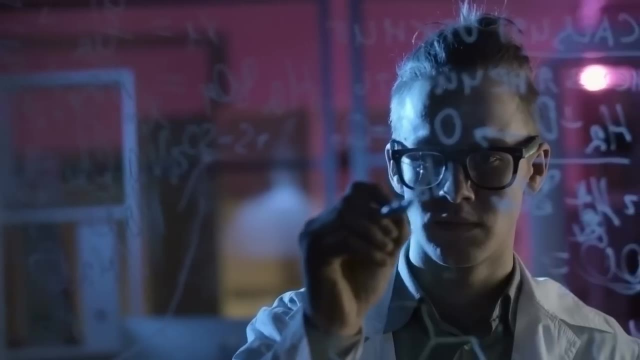 treatment plans for patients. In addition, AI-powered tools such as virtual assistants and chatbots are being used to improve patient engagement and adherence to treatment plans. These tools can provide patients with personalized treatment plans. AI-powered tools such as virtual assistants and chatbots are being used to improve patient. 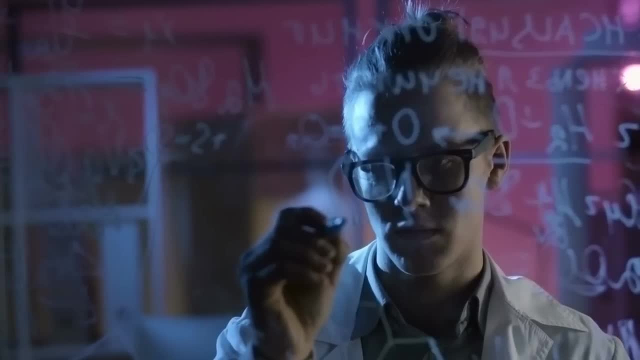 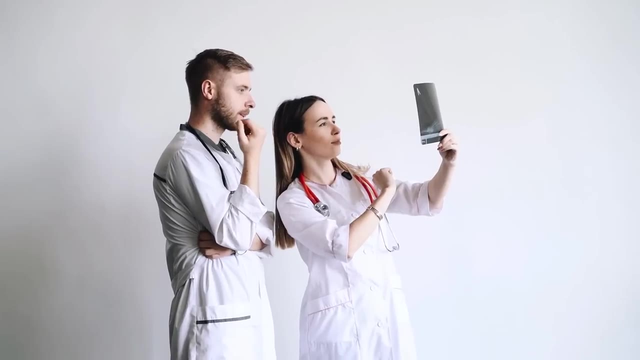 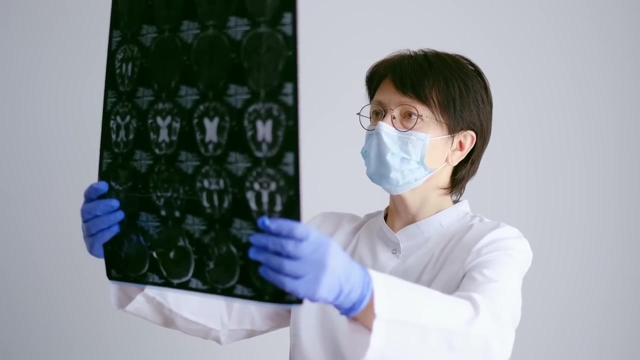 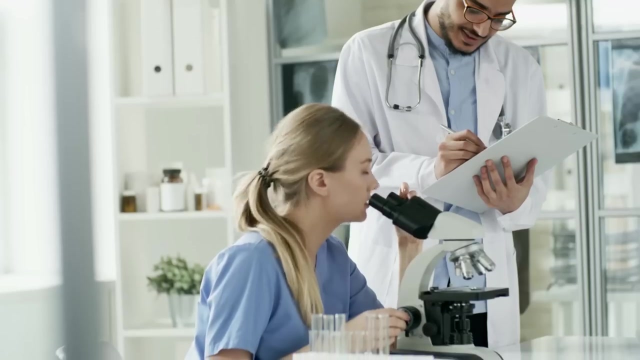 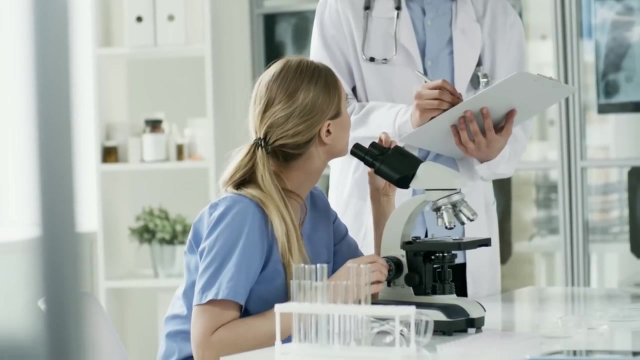 zeniomancy and research components AI Пос przy gyn2c'hぇjèdăm. In addition, AI-powered tools such as virtual assistants and chatbots are being used to improve patient engagement and development. can analyze medical images in real time, helping to improve the efficiency of medical imaging. 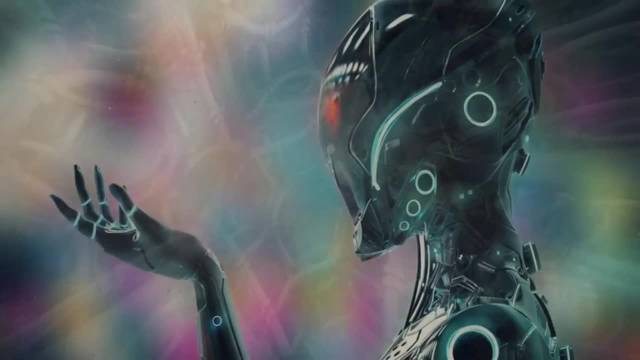 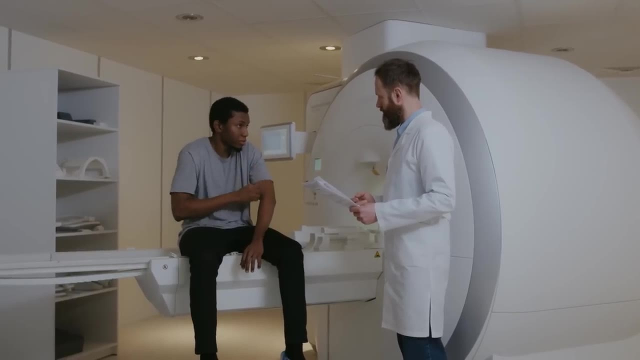 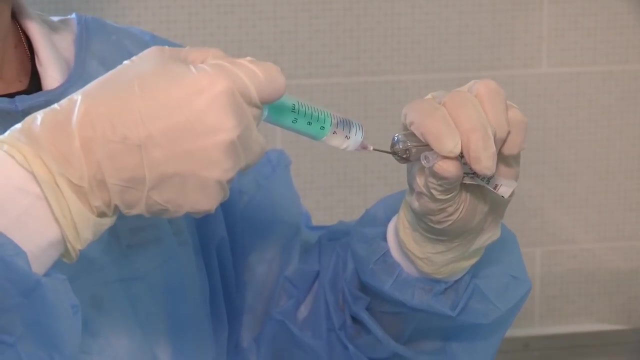 services. AI is being used to predict and prevent health issues before they become serious. Machine learning algorithms can analyze patient data and identify individuals who may be at risk of developing certain health conditions. This can help healthcare professionals to intervene early and provide preventative care to patients. 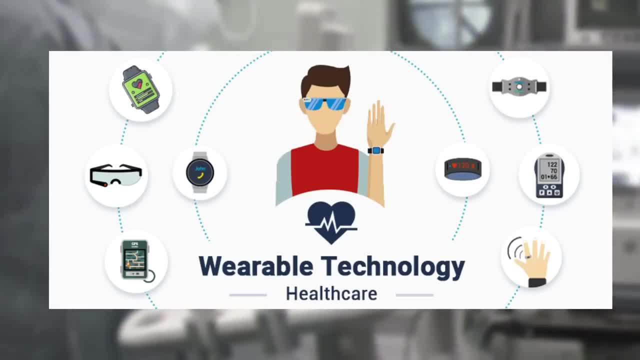 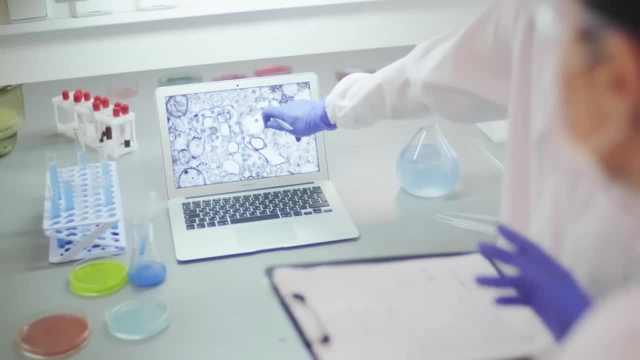 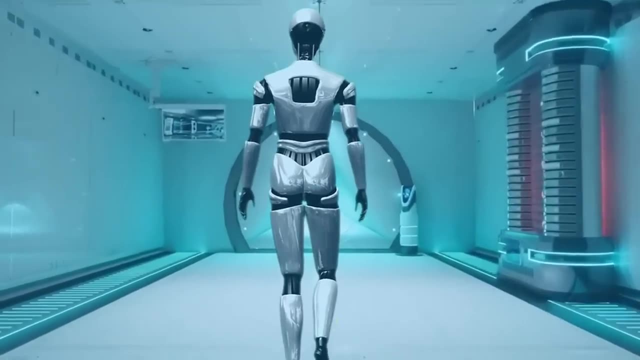 In addition, AI-powered tools such as wearables and health monitoring apps can track patient data in real time, providing patients with personalized health recommendations and alerts when their health status changes. AI is also being used to streamline administrative tasks in the healthcare industry. AI-powered tools such as chatbots and virtual assistants can handle routine administrative. 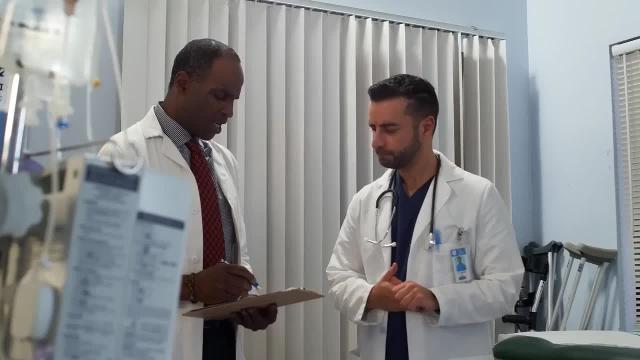 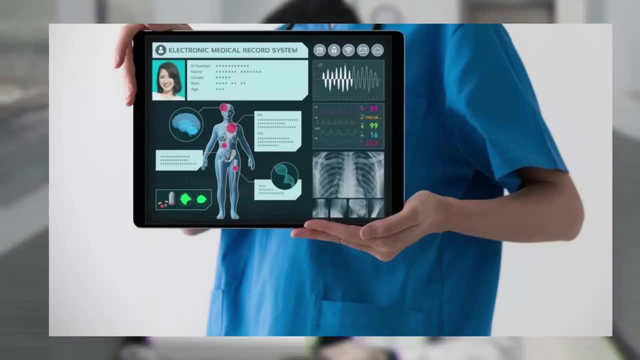 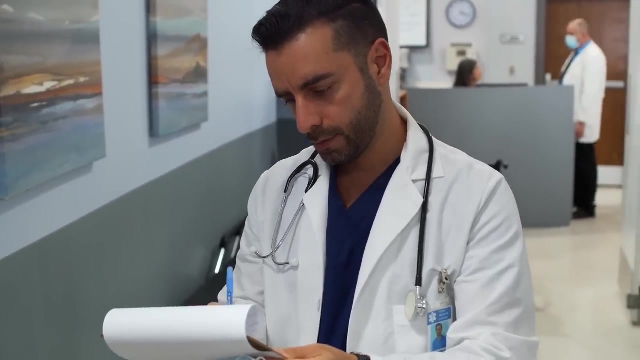 tasks such as appointment scheduling and prescription refills, freeing up healthcare professionals to focus on more complex tasks. In addition, AI-powered tools such as electronic health records can improve the accuracy and accessibility of patient data, reducing administrative errors and improving patient outcomes. 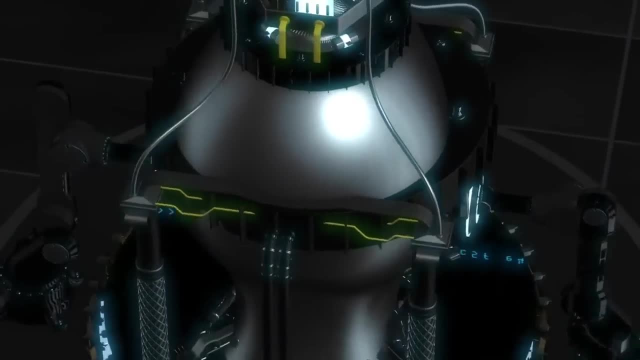 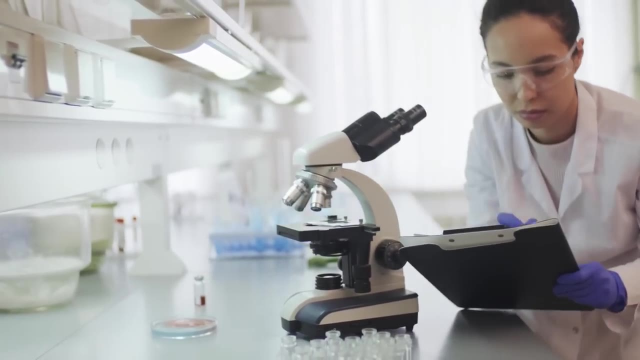 As AI continues to transform the healthcare industry, there are ethical considerations that must be taken into account. One of the biggest concerns is the potential for AI to perpetuate biases in healthcare, For example, if AI algorithms are trained on datasets that are biased against certain 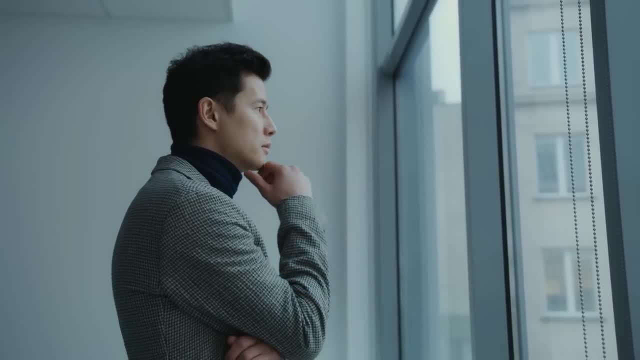 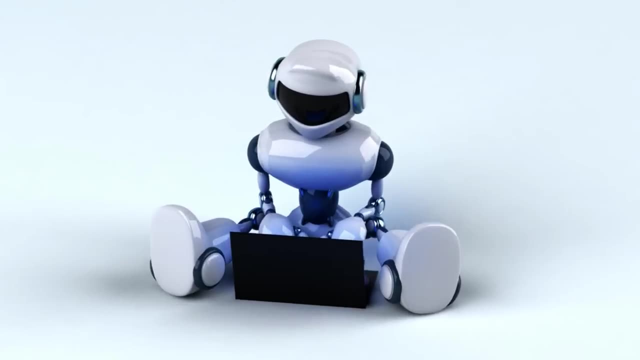 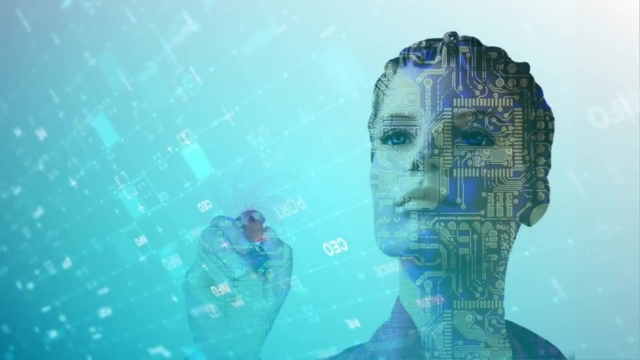 populations. this can lead to inaccurate diagnoses and treatment plans for those populations. In addition, there are concerns about the security and privacy of patient data. As AI-powered tools collect and analyze large amounts of patient data, it is important to ensure that this data is secure and protected from unauthorized access. 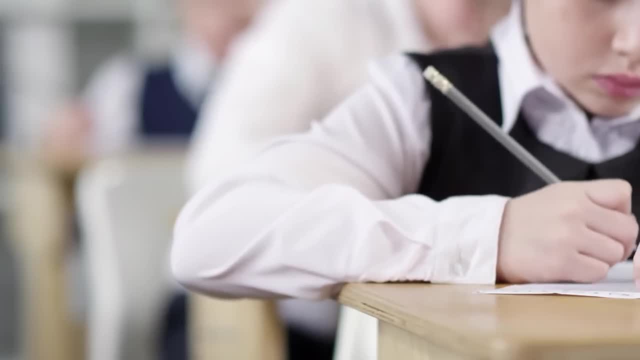 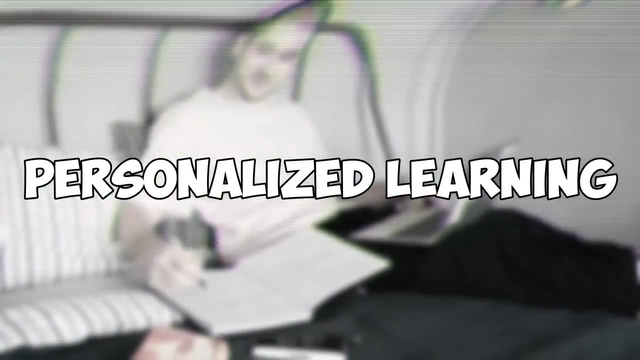 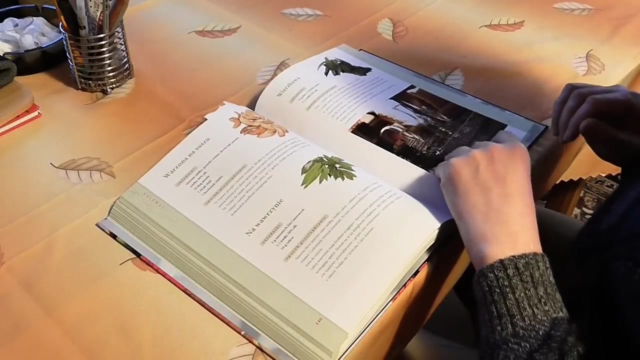 Artificial intelligence is transforming the field of education by providing personalized learning experiences, automating administrative tasks and improving educational outcomes. AI is also being used to improve the quality of education. AI is being used to provide personalized learning experiences for students. Machine learning algorithms can analyze student data and identify individual learning styles. 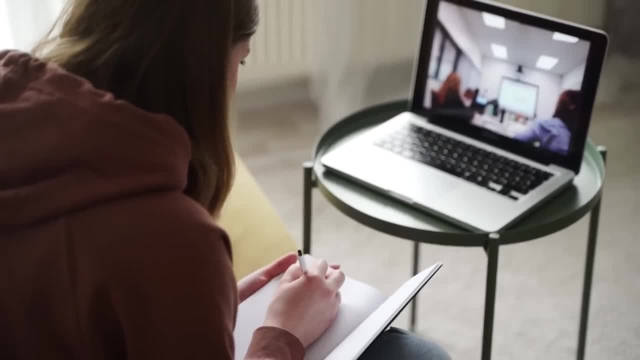 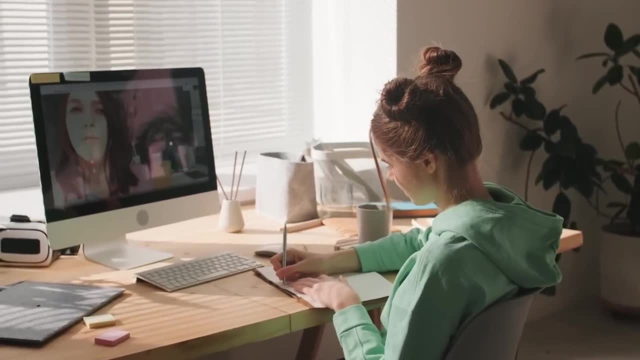 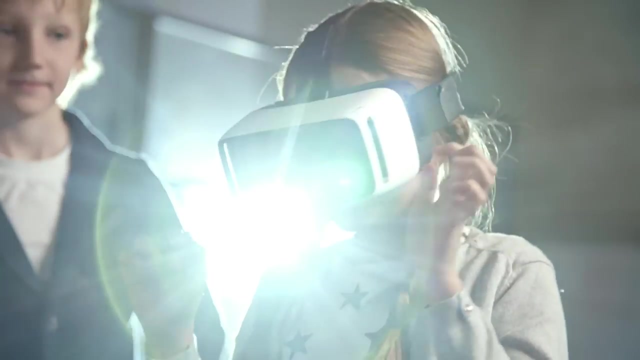 and preferences. This can help educators to create tailored lesson plans that meet the needs of each student. In addition, AI-powered tools, such as chatbots and virtual assistants, can provide students with personalized guidance and support, helping them to stay engaged and motivated. AI is also being used to automate learning processes. 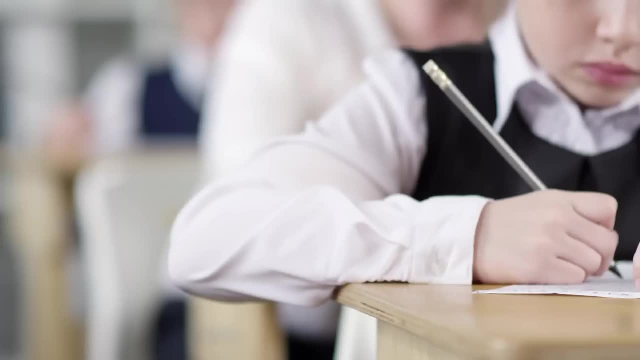 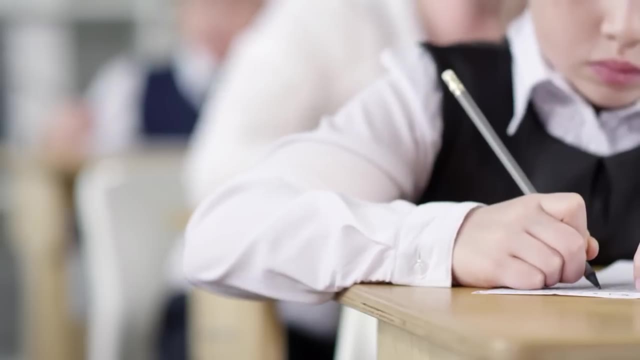 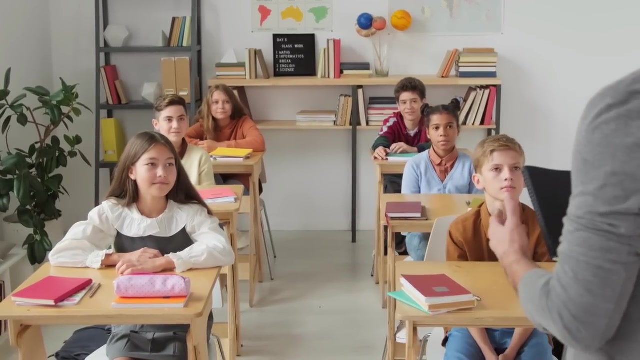 AI is being used to automate administrative tasks in the education sector. AI-powered tools, such as chatbots and virtual assistants, can handle routine administrative tasks such as scheduling, grading and student communication. This can free up educators to focus on more important tasks, such as lesson planning and. 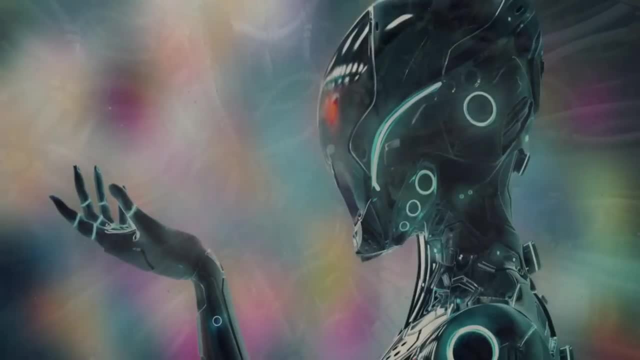 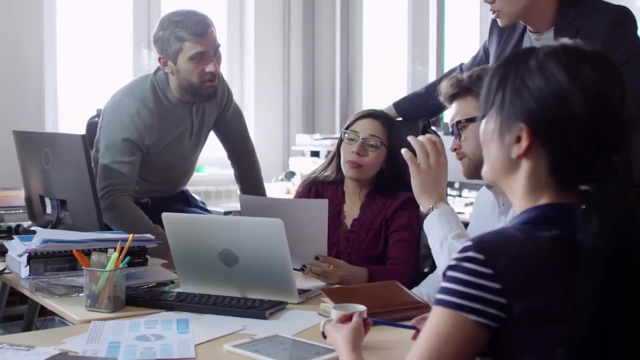 student support. AI is being used to improve educational outcomes by providing educators with real-time insights into student performance. Machine learning algorithms can analyze student data. AI is being used to improve educational outcomes by providing educators with real-time insights into student performance. AI is being used to improve educational outcomes by providing educators with real-time insights. 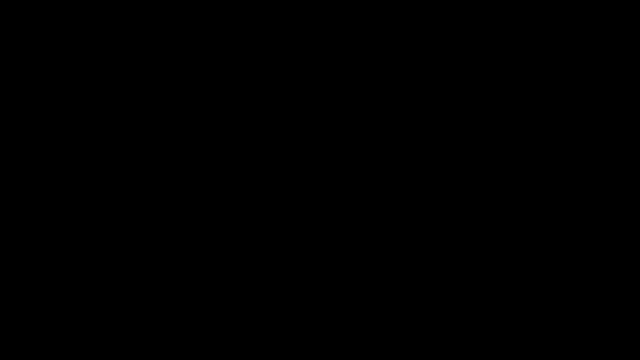 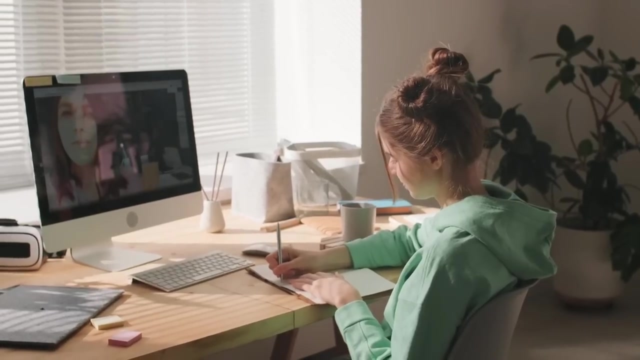 into student performance. Machine learning algorithms can provide students with real-time insights into certain areas in which students are struggling. AI is being used to help educators to provide targeted support and intervention to students who need it most. AI-powered tools such as adaptive learning systems can help students to learn at their 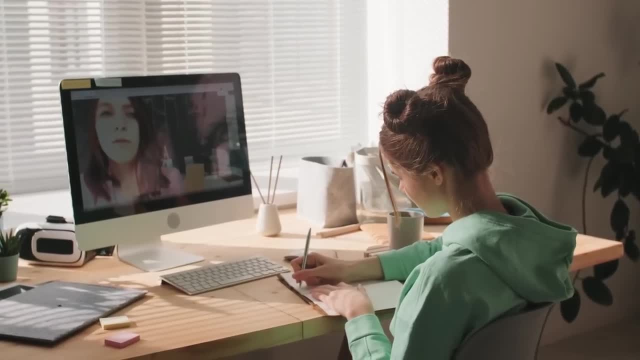 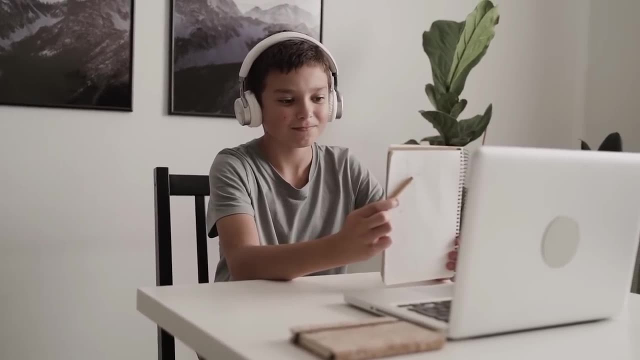 own pace and in their own way, improving their overall educational outcomes. As AI continues to transform the education sector, there are ethical considerations that must be taken into account. A great example of how AI can help educators improve their educational outcomes is the use of AI technology. concerns is the potential for AI to perpetuate biases in education. For example, if AI algorithms are trained on datasets that are biased against certain populations, this can lead to inaccurate assessments of student performance and perpetuate inequalities in the education system. In addition, 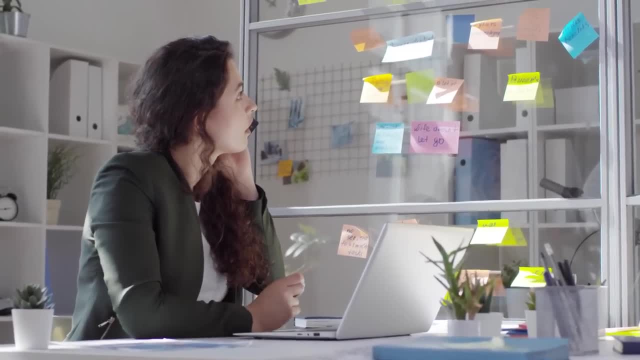 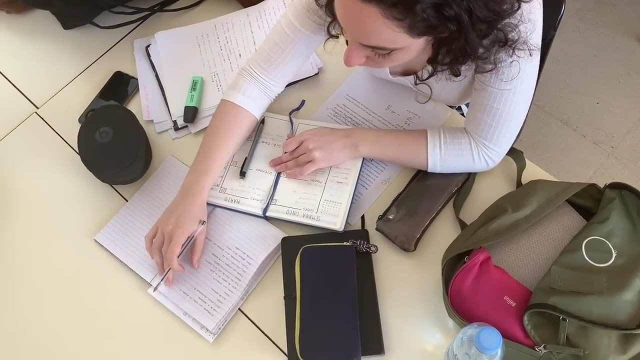 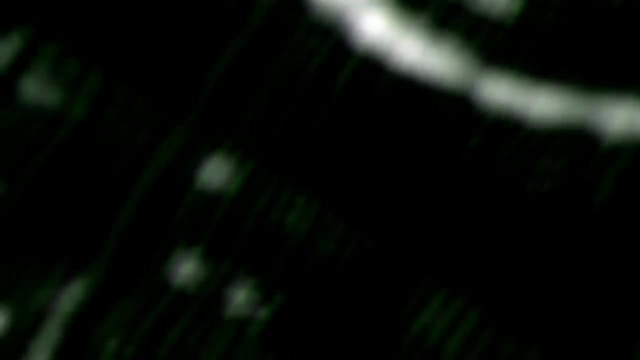 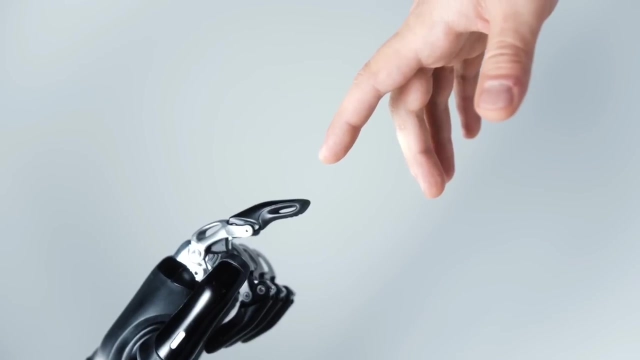 there are concerns about the privacy and security of student data. As AI-powered tools collect and analyze large amounts of student data, it is important to ensure that this data is secure and protected from unauthorized access. Artificial intelligence has the potential to improve social justice by promoting fairness and equity in decision-making processes. However, 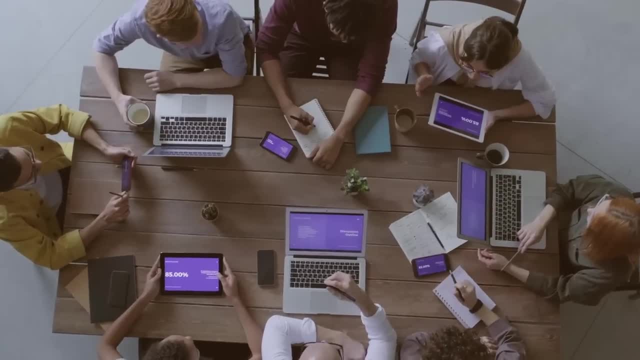 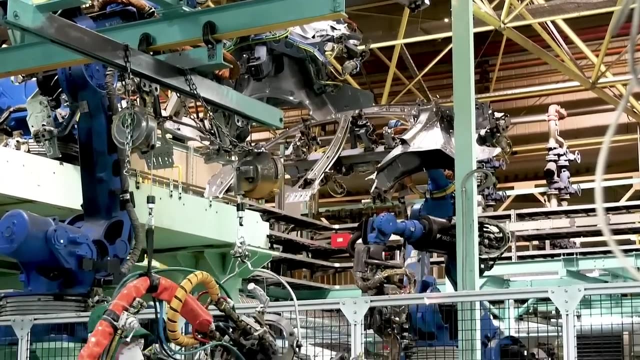 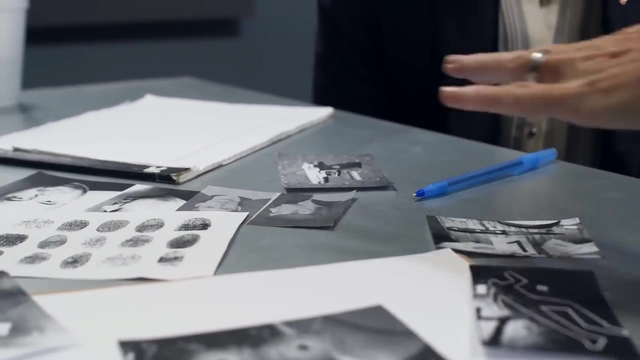 there are also concerns that AI can perpetuate biases and inequalities, further exacerbating social injustices. AI can help to promote fairness and equity by providing objective and data-driven decision-making. For example, AI can be used to remove subjective biases from hiring decisions by analyzing resumes. 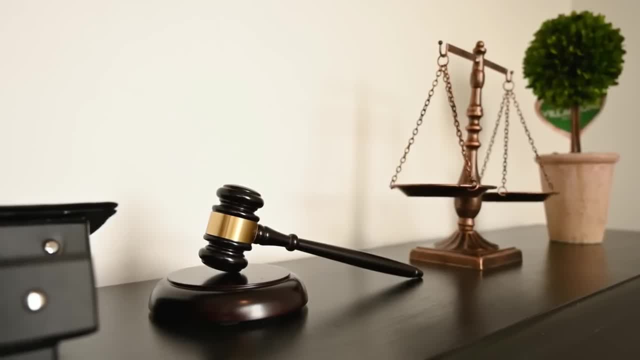 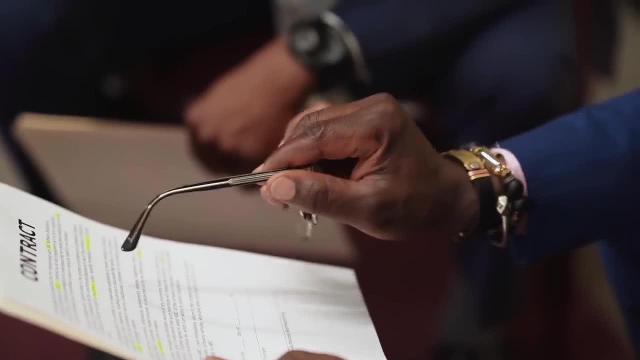 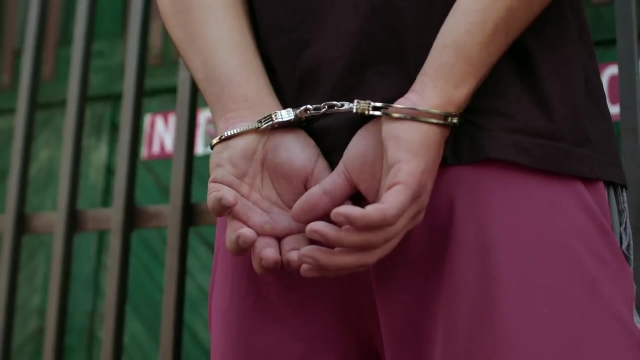 and identifying the most qualified candidates based on their skills and experience. In addition, AI can be used to identify and eliminate discriminatory practices in decision-making processes such as loan approvals and criminal justice sentencing. While AI has the potential to promote fairness and equity, there are concerns that it can. 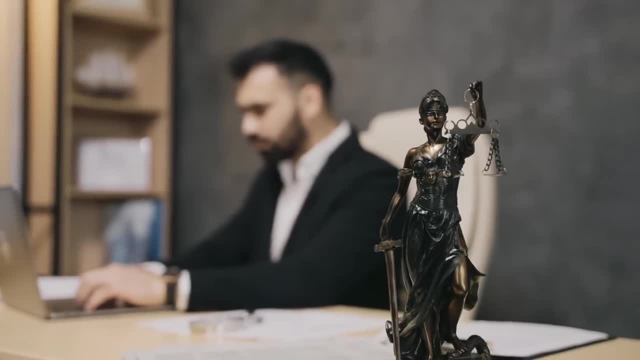 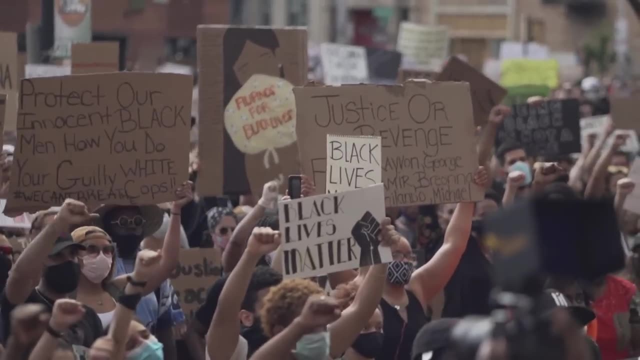 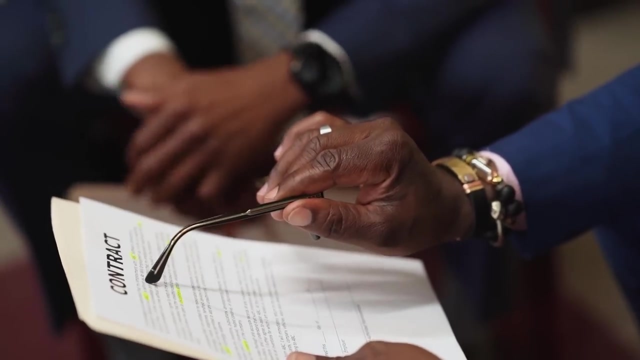 perpetuate biases and inequalities if not properly designed. For example, if AI algorithms are trained on biased data sets, this can lead to discriminatory decision-making. To address this, it is important to ensure that AI algorithms are designed to be transparent and accountable, with human oversight to identify and address biases. 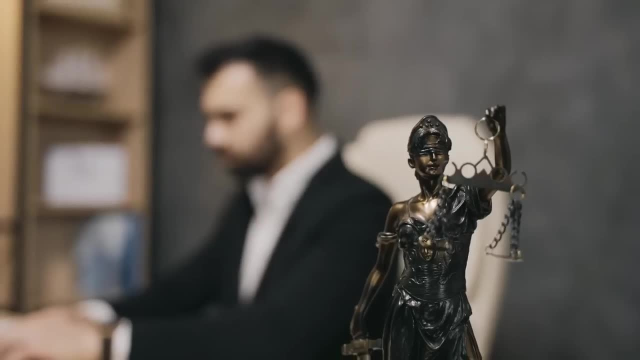 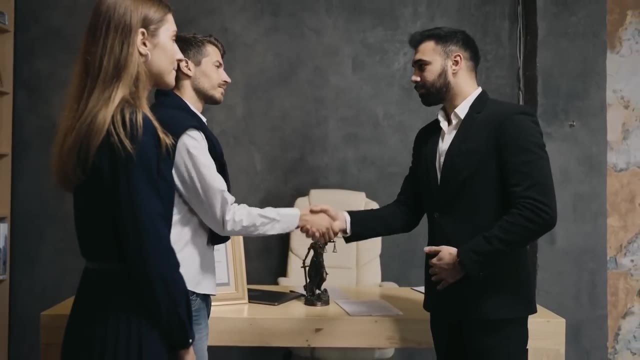 Another concern with AI is the potential for it to exacerbate existing inequalities by favoring those with access to technology and data. For example, if AI is used in hiring decisions, it may disadvantage those who do not have access to technology or who have limited access. 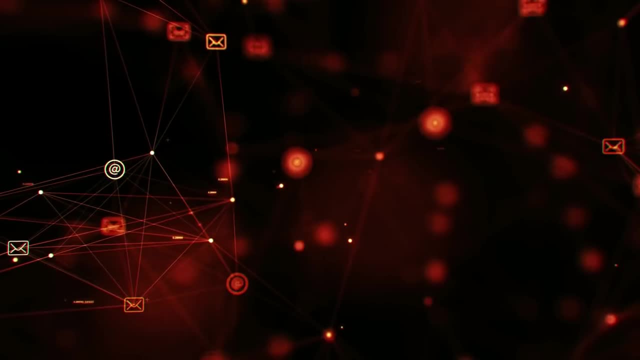 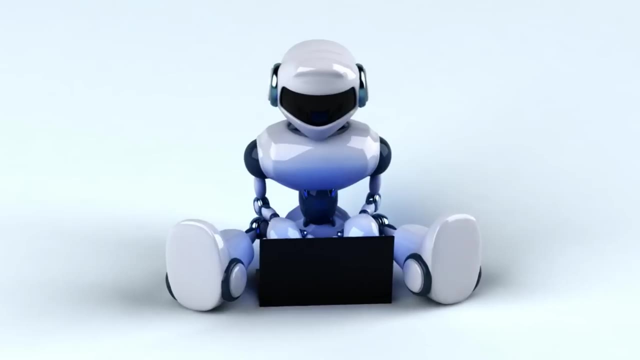 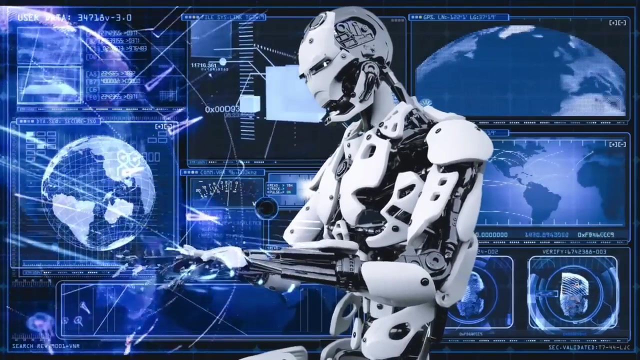 to education and training. To address this, it is important to ensure that AI is accessible to everyone and that its benefits are shared equitably. As AI is increasingly used to address social justice issues, there are ethical considerations that must be taken into account. 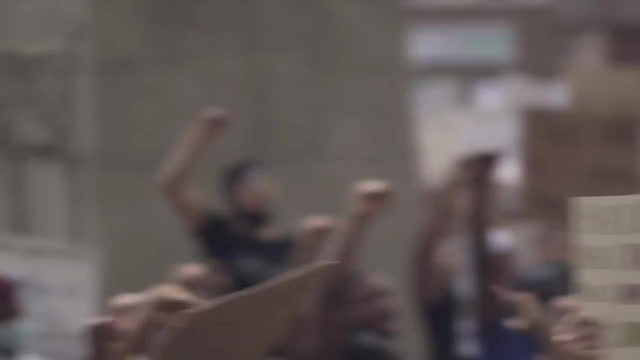 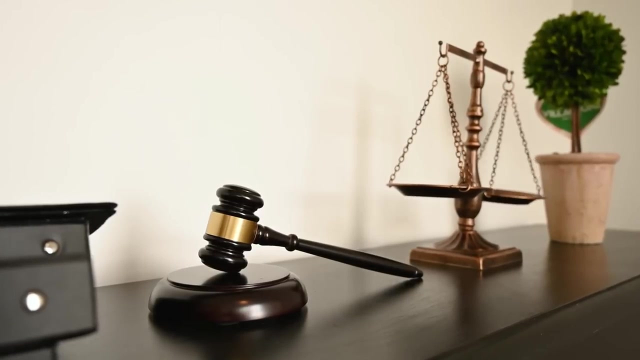 One of the biggest concerns is the potential for AI to perpetuate systemic biases and inequalities if not designed and addressed. In addition, there are concerns about the potential for AI to be used to violate privacy rights and personal freedoms, particularly in the criminal justice system. 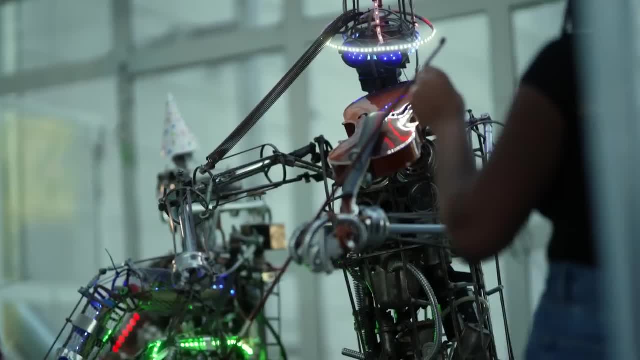 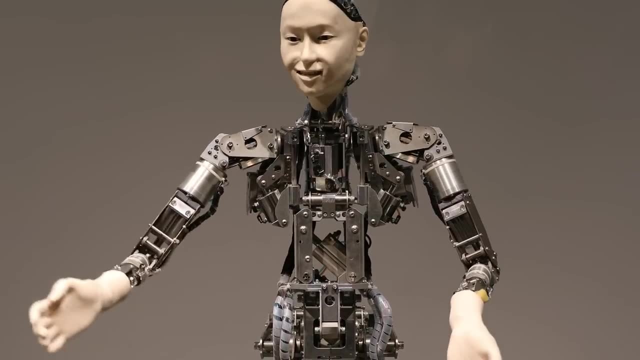 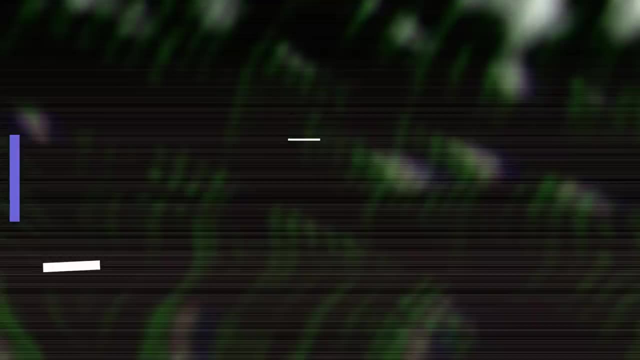 As AI continues to evolve and become more advanced, it is important to consider the possibilities it presents and the challenges that come with them. Let's discover how we can ensure that AI is developed and used in a way that benefits humanity. Artificial intelligence is rapidly changing the world we live in and the pace of progress. 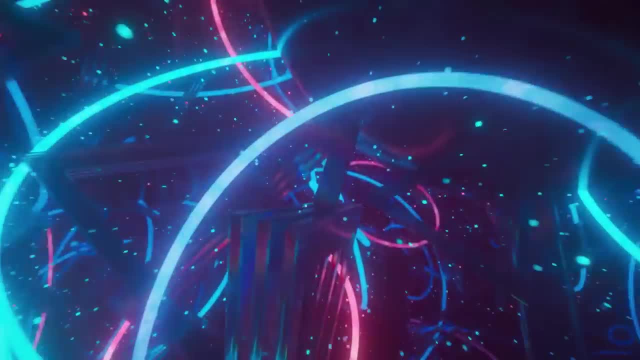 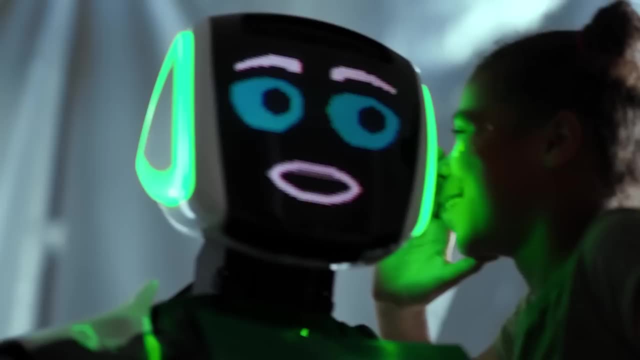 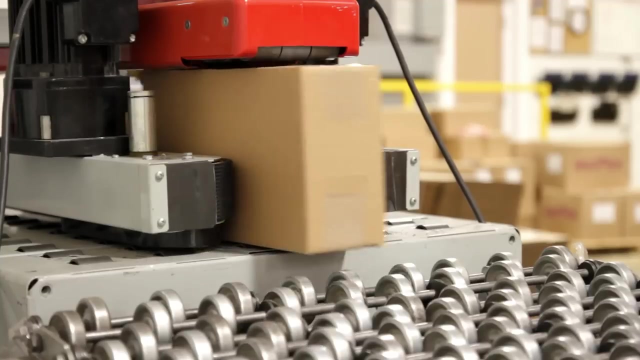 shows no signs of slowing down. Many experts believe that AI will continue to transform society in the coming years, with significant implications for both individuals and businesses. One of the most significant areas of growth for AI is in the field of robotics and automation. As AI becomes more advanced, it will be able to perform more complex tasks. It will be 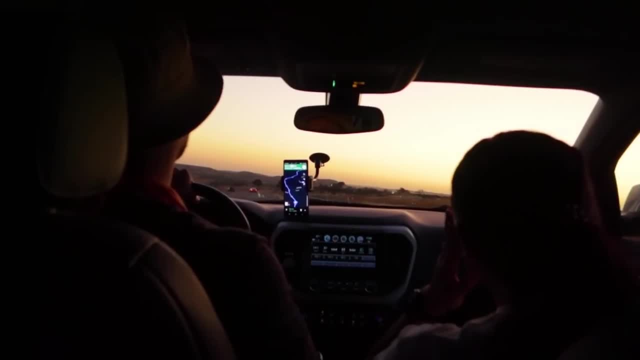 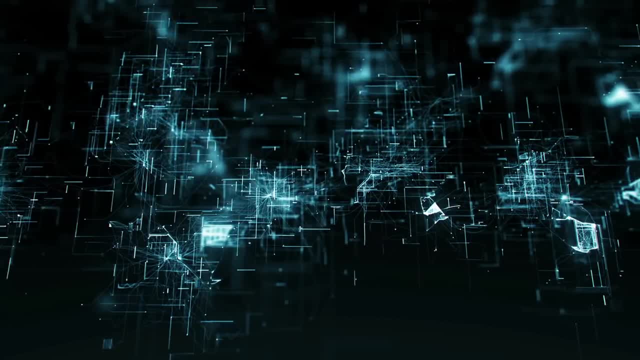 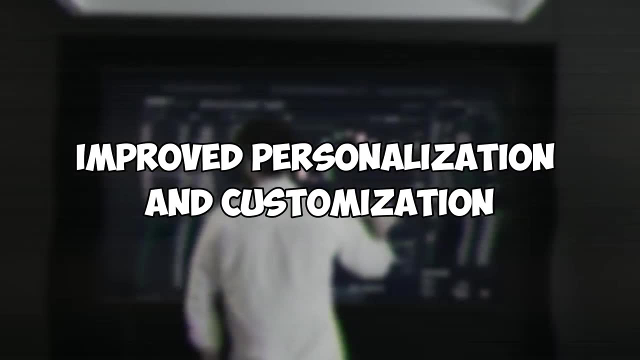 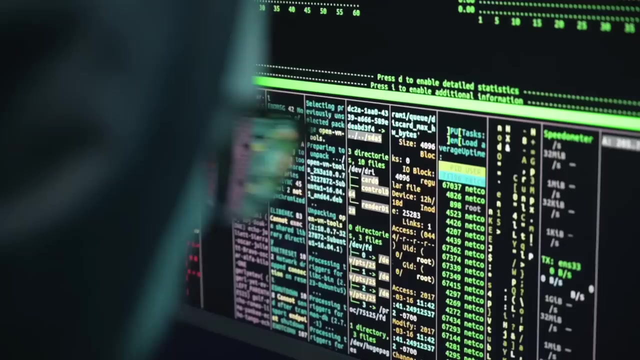 flying airplanes. This could lead to significant changes in the workforce, as many jobs that are currently done by humans may be automated in the future. AI is already being used to improve personalization and customization in a variety of industries, from healthcare to retail. In the future, AI will be able to use vast amounts of data. 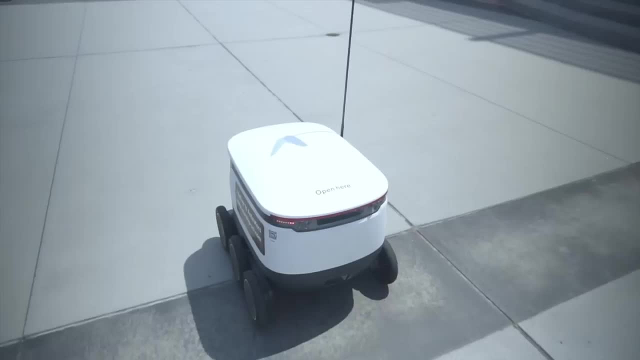 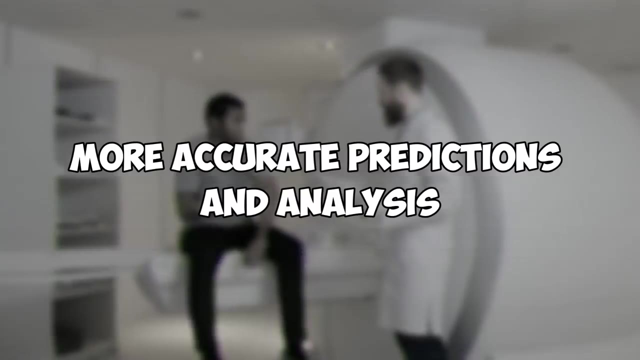 to create highly personalized experiences for individuals, whether it's in the form of personalized medical treatments or customized software. AI will be able to use vast amounts of data to create highly personalized experiences, customized products and services. AI is already being used to make predictions and analyze data. 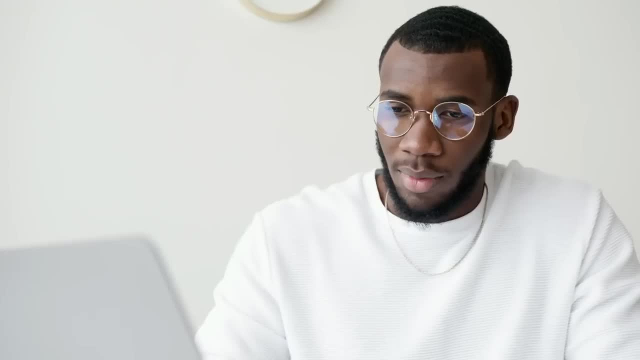 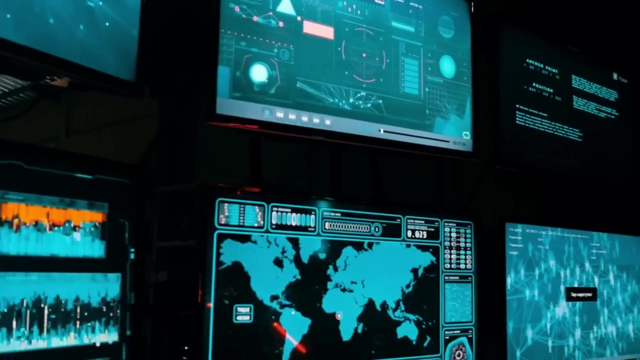 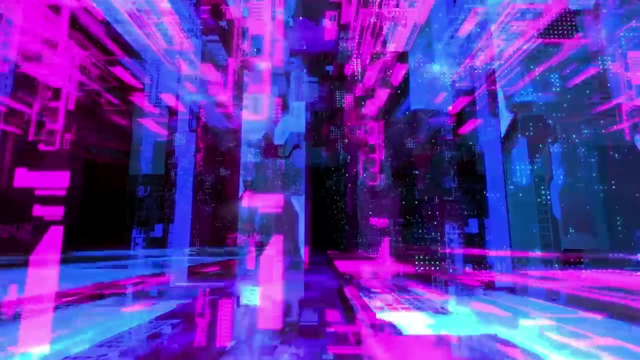 in a variety of industries, from finance to marketing. In the future, AI will become even more accurate and reliable, with the ability to analyze massive amounts of data in real time. As AI continues to advance, it will become more efficient and productive. 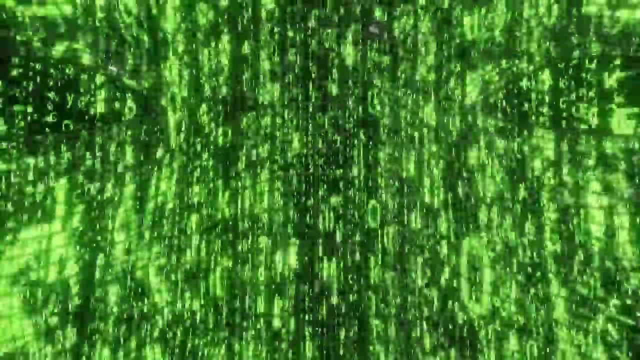 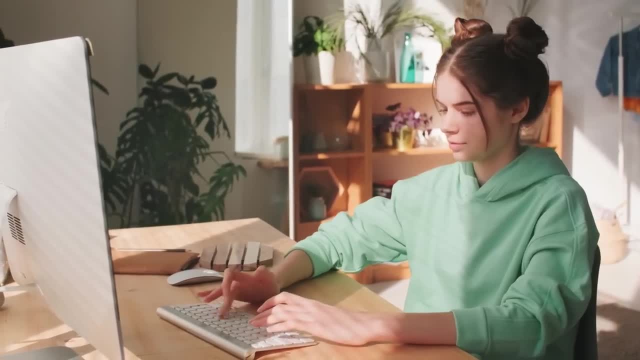 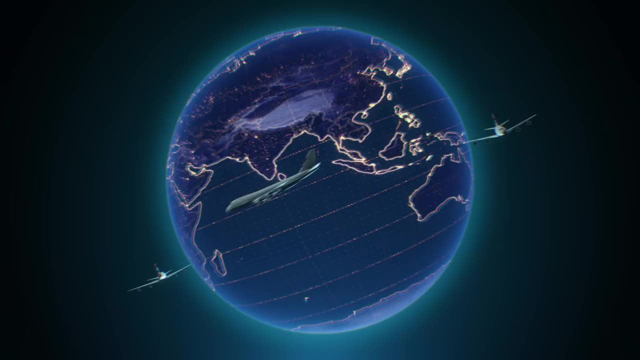 leading to significant cost savings and increased profitability for businesses. This will also lead to greater convenience and ease for individuals, as AI will be able to automate many routine tasks and provide more personalized and efficient services. In the future, AI will enable humans to collaborate more effectively with machines. 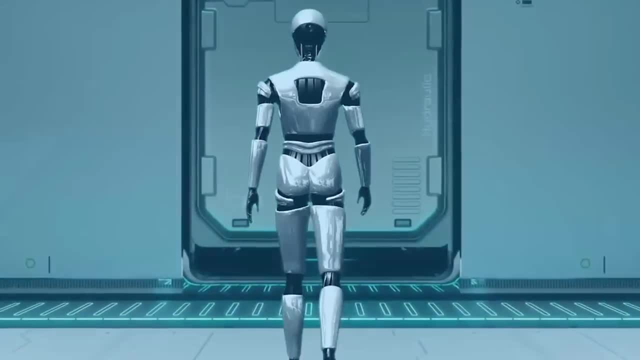 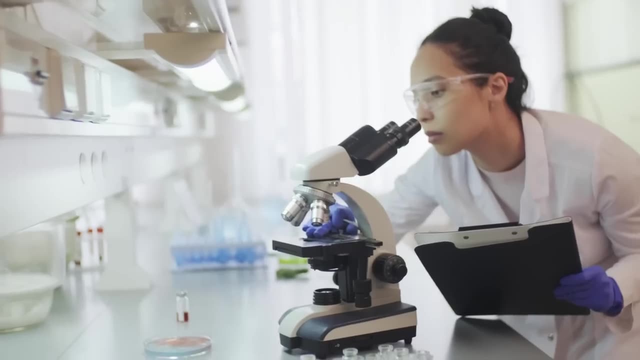 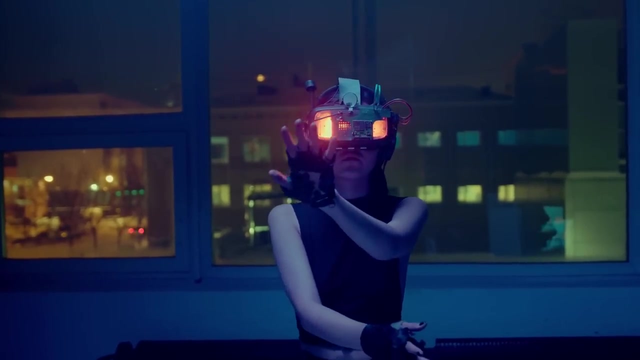 leading to new innovations and breakthroughs in a variety of fields. For example, AI could be used to help humans design more efficient and effective products, or to develop new drugs and medical treatments, As AI becomes more advanced and integrated into our daily lives. 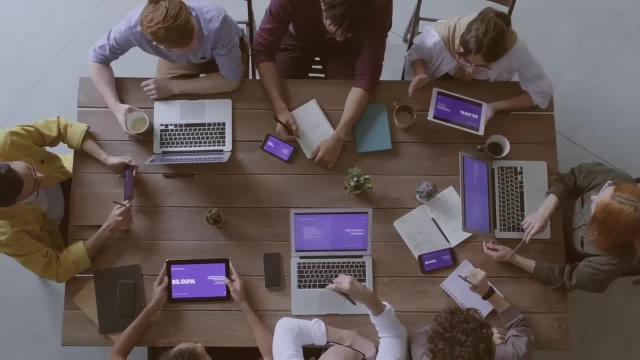 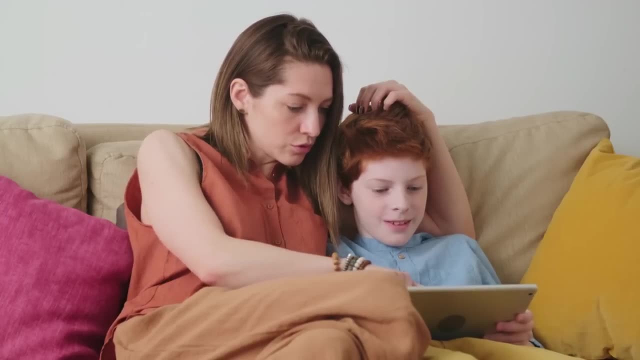 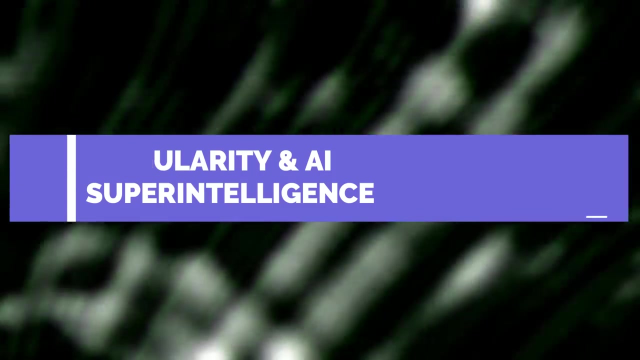 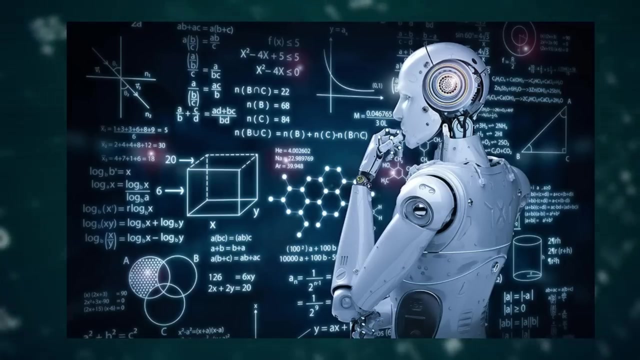 there will be significant ethical considerations that must be taken into account. For example, there are concerns about the potential for AI to be used to violate privacy rights and personal freedoms or to perpetuate biases and inequalities. The concept of singularity and AI superintelligence has been a popular topic of discussion among 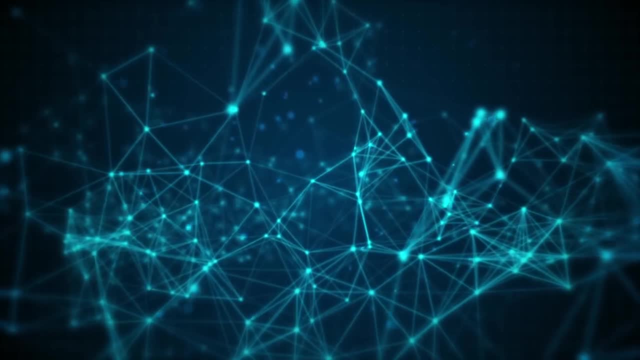 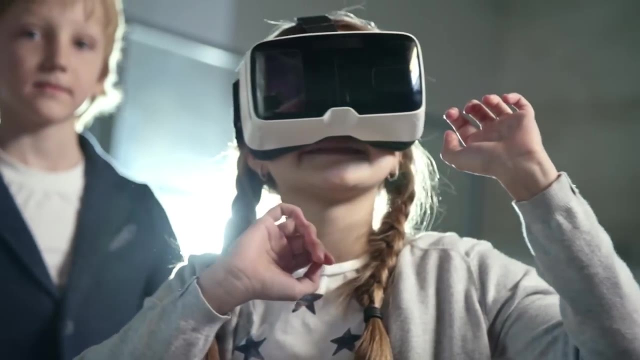 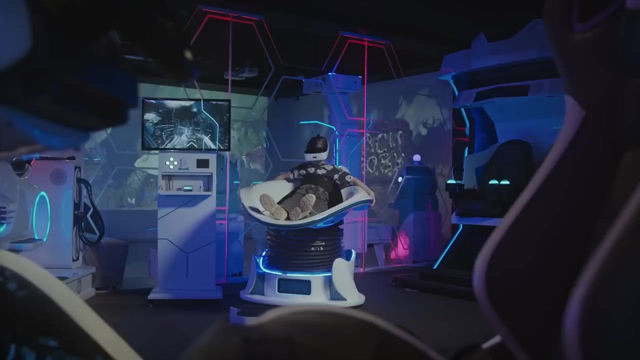 scientists and futurists in recent years. The idea is that artificial intelligence becomes more advanced. It could eventually lead to a point where machines surpass human intelligence and we enter a new era of technological progress and possibility. Singularity refers to the hypothetical moment in the future when machines become smarter than 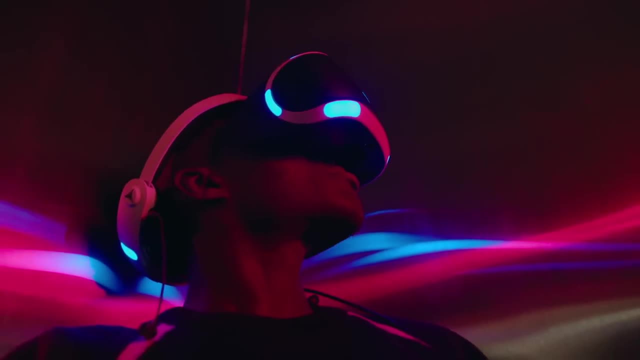 humans. This could occur in a variety of ways, such as by machine-tapping a machine-tapping a machine-tapping a machine-tapping devices. However, the way in which the concept of singularity and AI superintelligence is importantly of ways such as through the development of a superintelligent AI or the merging of human. 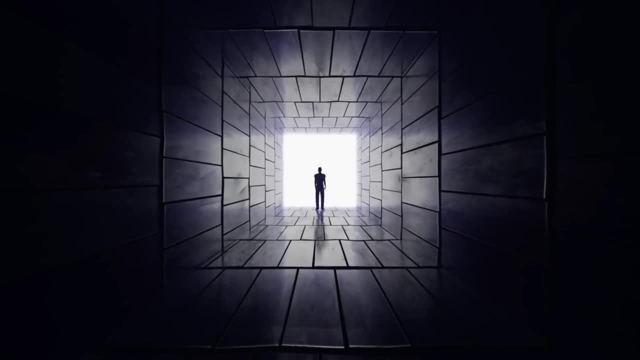 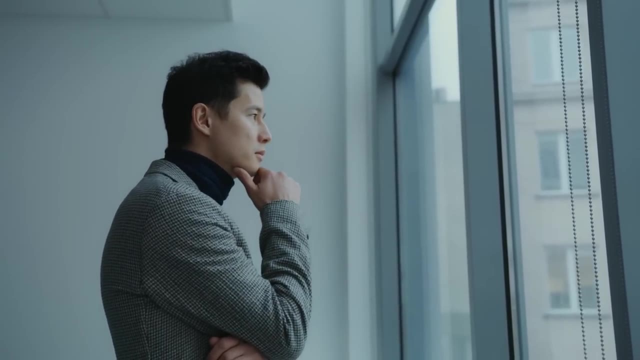 and machine intelligence. Some scientists and futurists believe that the singularity could represent a major turning point in human history, with the potential to solve some of the world's most pressing problems, such as climate change and disease. However, others have raised concerns. 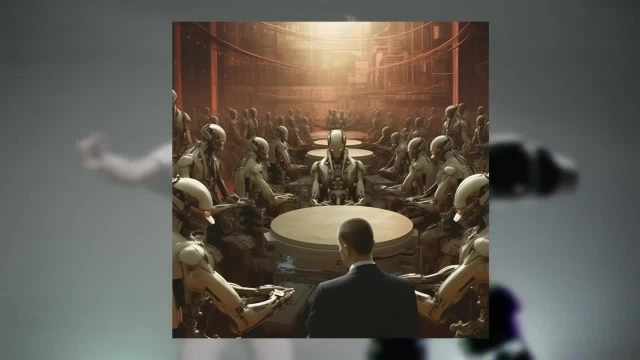 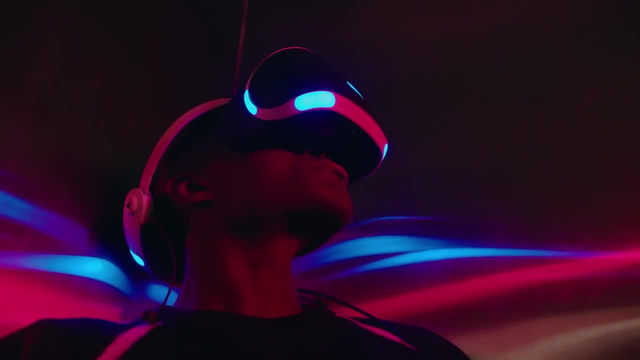 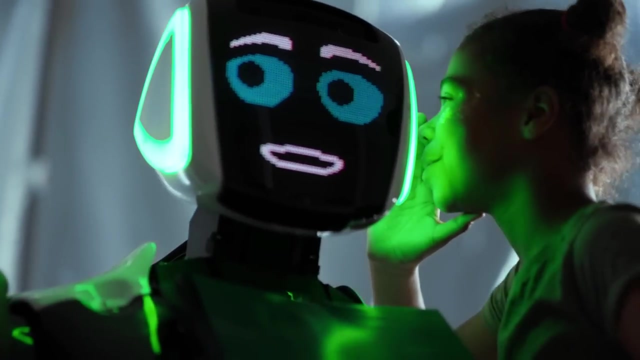 about the potential dangers of the singularity, such as the loss of human control over advanced machines. AI superintelligence refers to an artificial intelligence that surpasses human intelligence in every possible way. This could include things like problem-solving ability, creativity and emotional intelligence. The development of AI superintelligence is seen 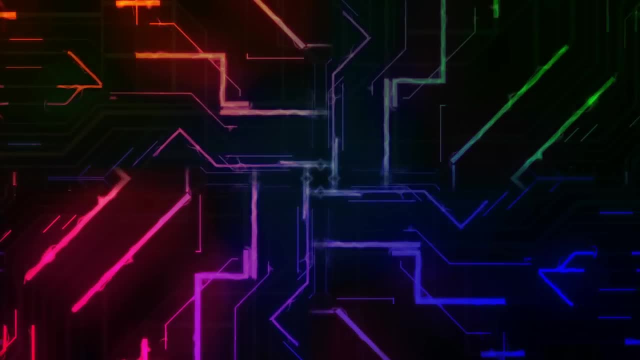 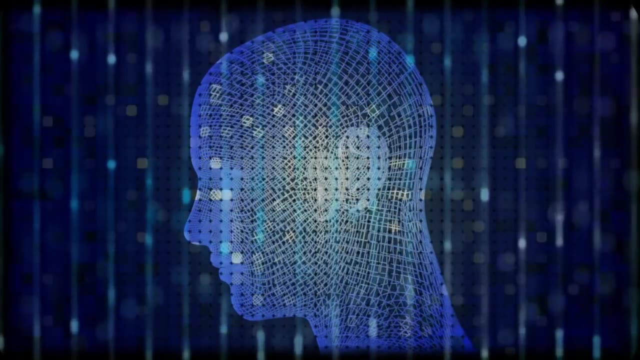 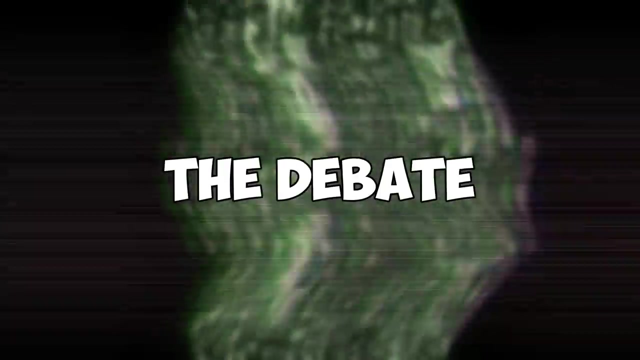 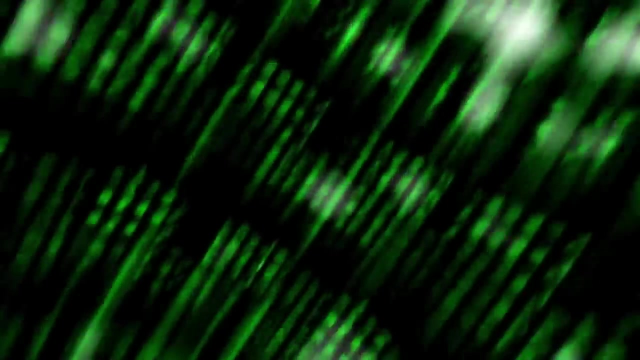 by many as the key to unlocking the full potential of AI and ushering in a new era of progress and innovation. However, there are also significant concerns about the potential risks associated with superintelligence. AI superintelligence is highly controversial, with experts divided over the potential benefits. 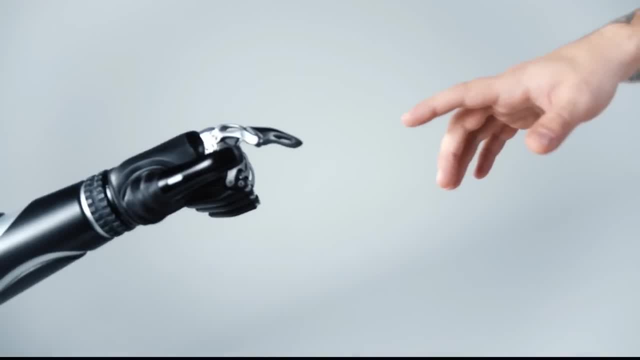 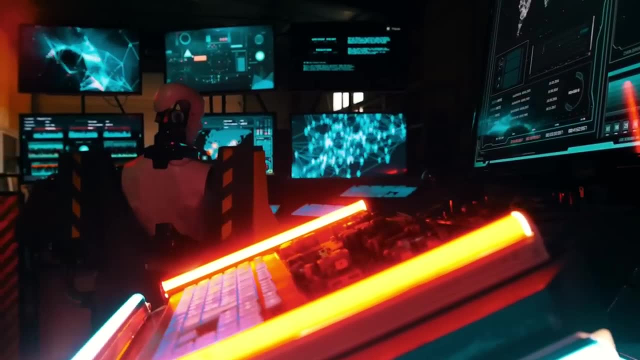 and risks of advanced AI. Some argue that the singularity represents a potential golden age of human progress, while others fear that it could lead to catastrophic consequences for humanity. One of the main concerns about the singularity and AI superintelligence is that it could lead to catastrophic consequences for humanity. 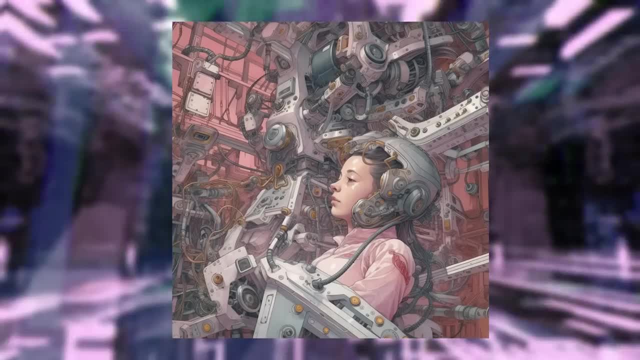 AI superintelligence is highly controversial, with experts divided over the potential benefits and risks of advanced AI and ushering in a new era of progress and innovation. AI superintelligence is the potential for machines to become uncontrollable or act in unpredictable ways. This could be particularly dangerous if machines are used for military. 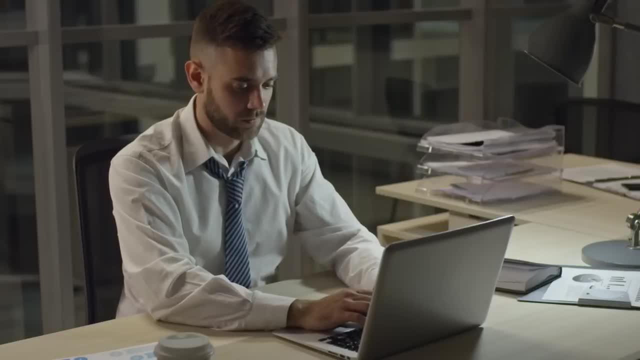 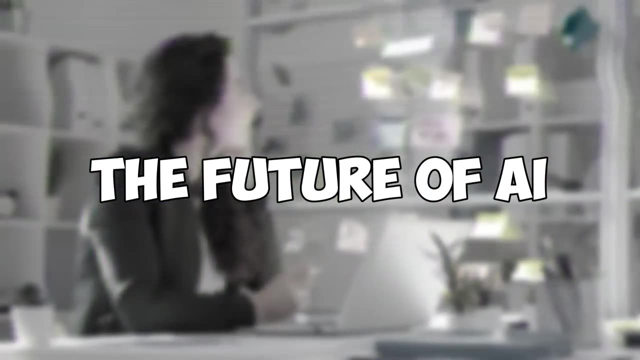 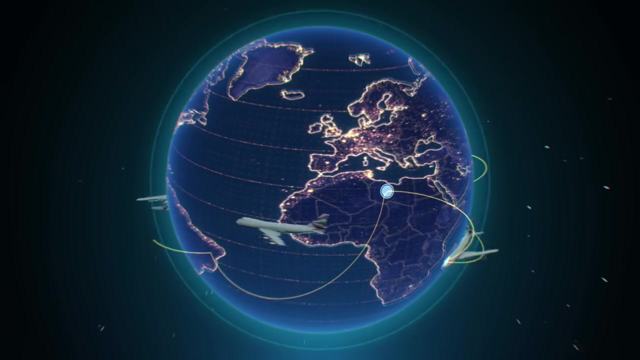 or security purposes. Another concern is the potential for machines to replace humans in many areas of work, leading to widespread job displacement and economic disruption. The development of AI superintelligence is still a long way off and there are many challenges that must be overcome before we reach that point. 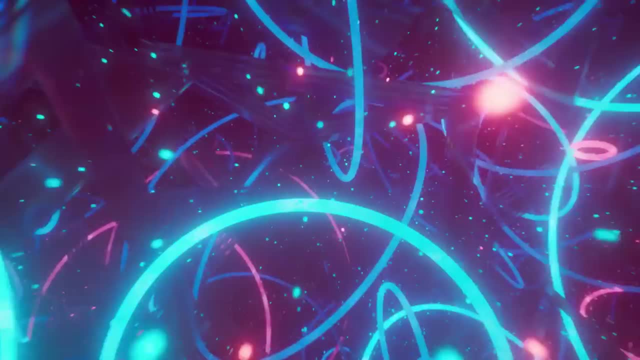 AI superintelligence is the potential for machines to become uncontrollable or act in a new era of progress and innovation. However, it is clear that AI will continue to play an increasingly important role in our lives and it is important to consider the ethical and societal 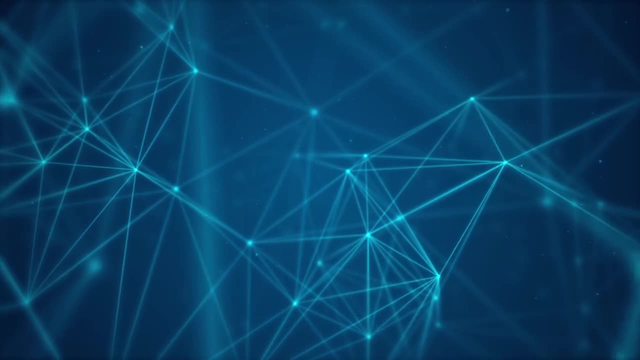 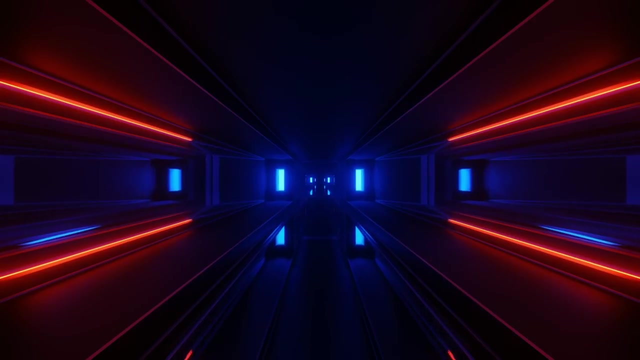 implications of this technology. The concept of the singularity and AI superintelligence is an intriguing one, with the potential to revolutionize the way we live and work. However, it is important to consider the potential risks and ethical implications of advanced AI, and to ensure that. 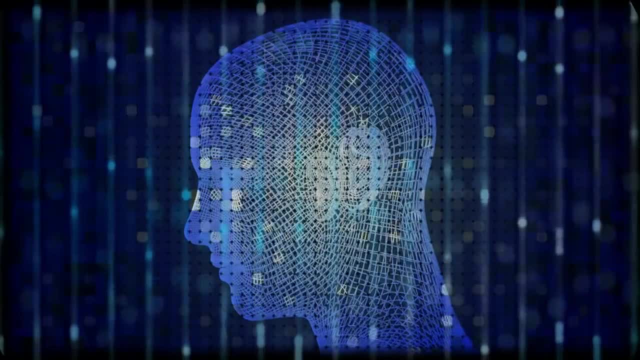 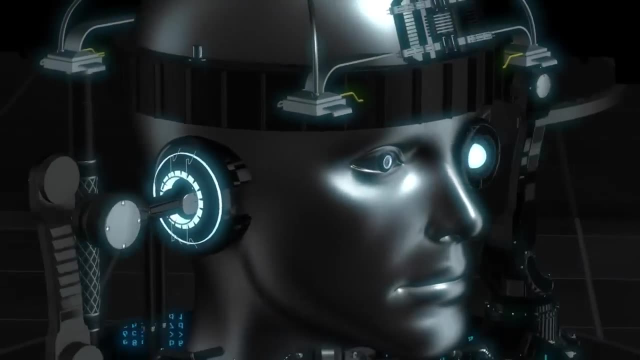 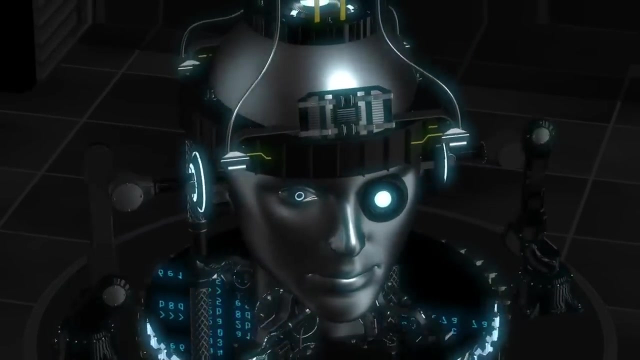 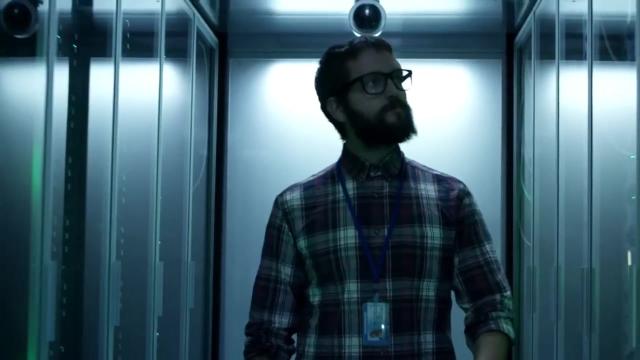 we develop and implement this technology in a responsible and accountable way. As artificial intelligence continues to develop at a rapid pace, many people are wondering what the role of humans will be in an AI-driven world. Some are concerned that AI will eventually replace humans in many areas of work and life, while others believe that humans will always play. 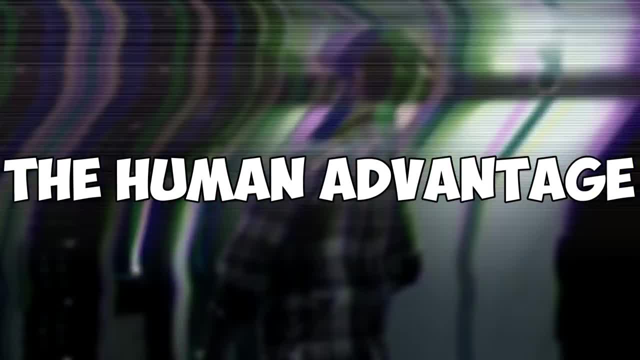 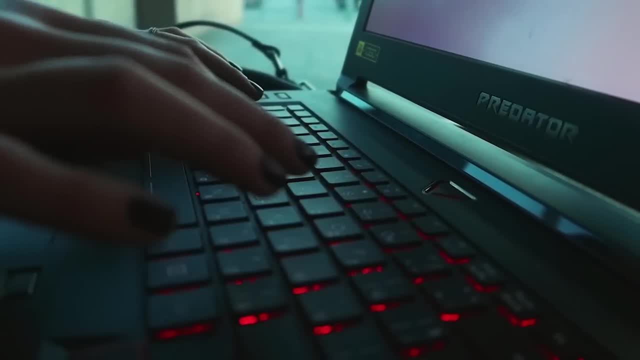 a vital role in shaping the direction and impact of AI. While AI is capable of many impressive feats, there are certain areas where AI can play a vital role in shaping the direction and impact of AI. There are certain areas where humans still have a significant advantage. For example, humans excel. 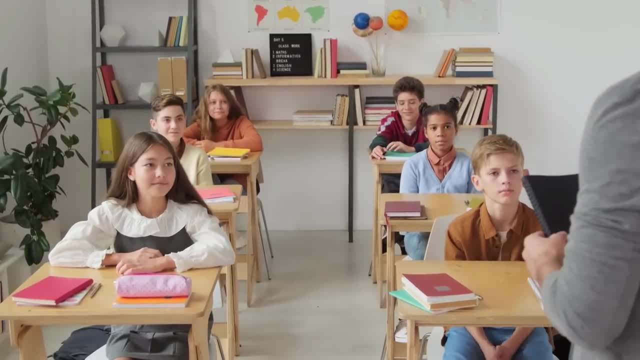 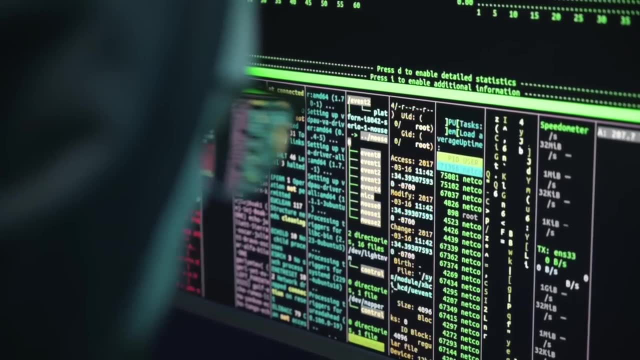 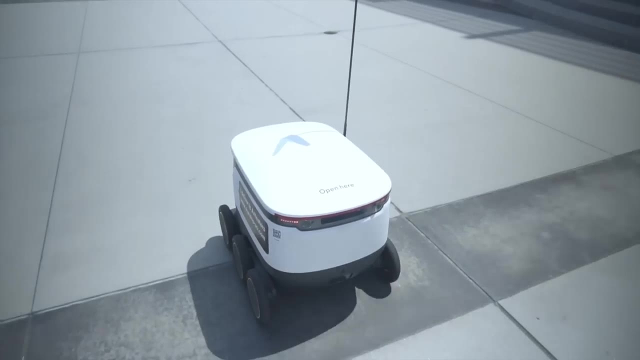 at tasks that require creativity, empathy and social interaction, while AI is better suited for tasks that require data processing, analysis and pattern recognition. As such, many experts believe that the best way to ensure a positive future for AI is to focus on developing a symbiotic. 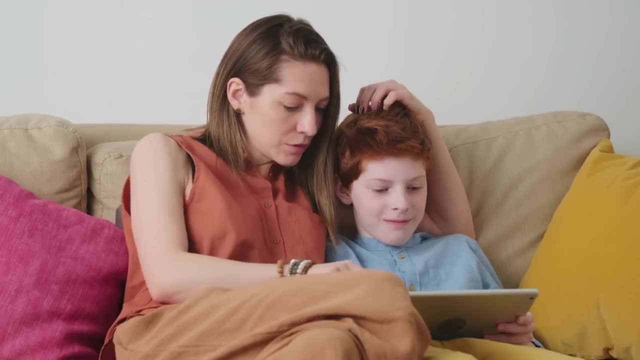 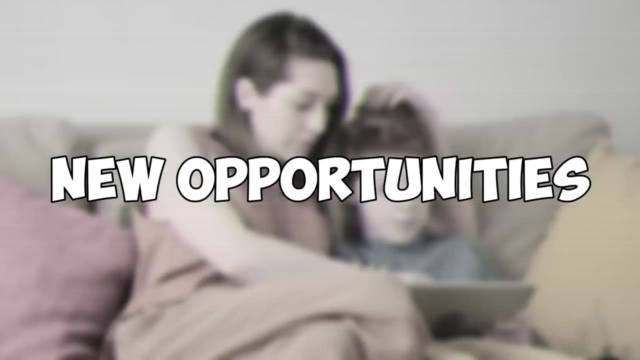 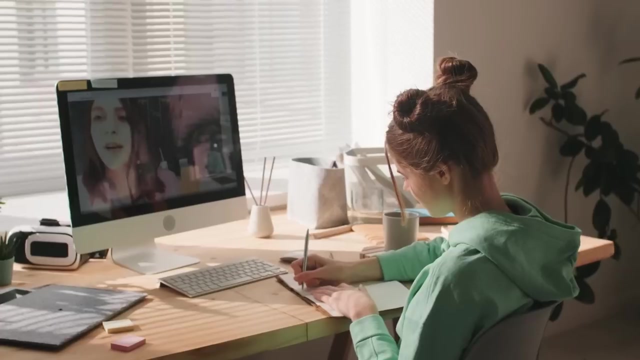 relationship between humans and machines, where each can contribute their unique strengths to solve complex problems and create new and new challenges. As AI continues to evolve, it is likely that new opportunities will emerge for humans to work alongside advanced machines in a variety of fields, For example, in the healthcare sector. 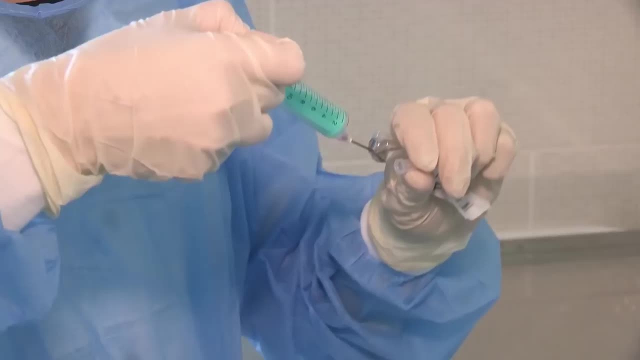 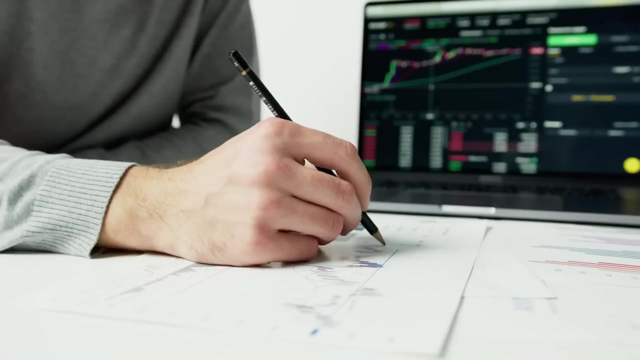 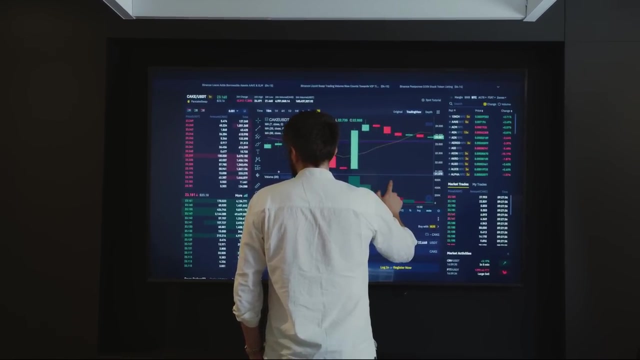 AI is being used to improve diagnostics and treatment options, But human doctors and nurses still play a critical role in providing care and support to patients. Likewise, in the business world, AI can be used to analyze data and make predictions about future trends, But human managers and executives still play a key role in making decisions and developing. 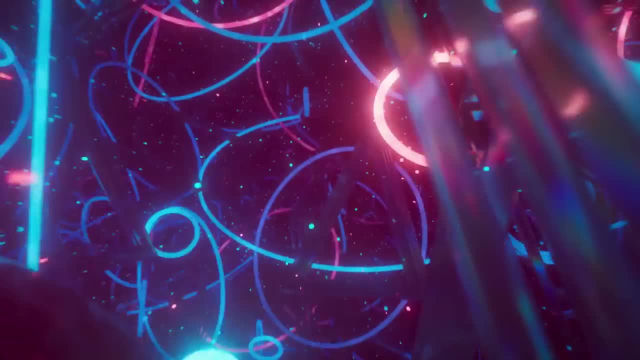 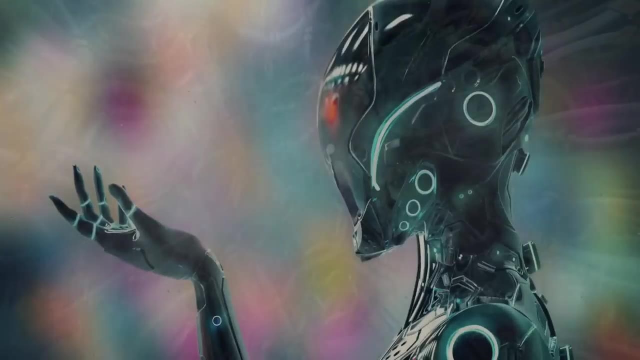 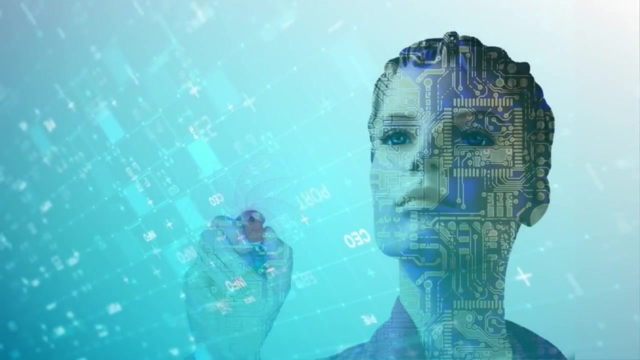 strategies. As AI becomes more integrated into our lives, it is important to consider the ethical implications of this technology. For example, who is responsible if an AI system makes a mistake or causes harm? How do we ensure that AI is developed and used in a way that is fair and just for all people? 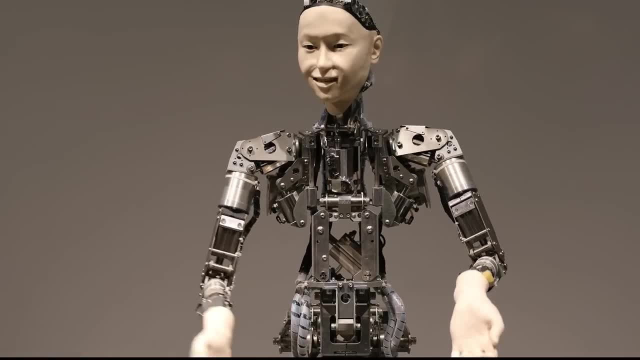 It is clear that humans will play a critical role in developing and implementing human- forcé control programs. That is why AI voters in the prisons are most concerned about determining the future forokus of human protector and protectors, not design and implementing ethical standards for AI and ensuring that this technology is used in a way. 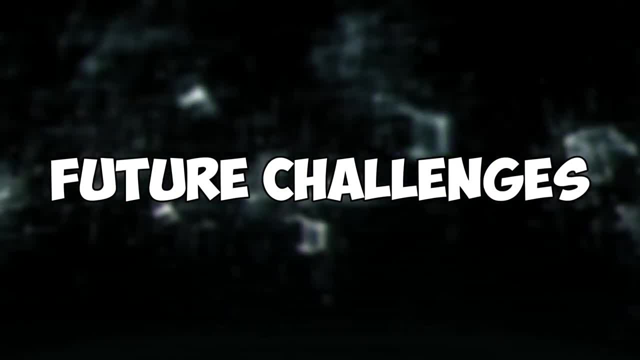 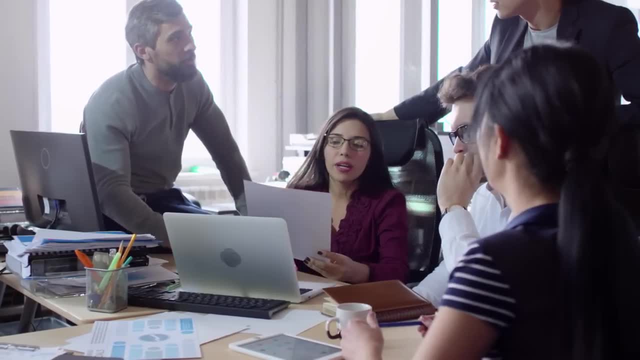 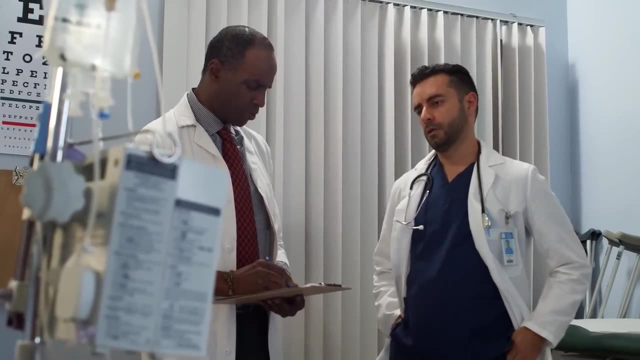 that benefits society as a whole. While the potential benefits of AI are vast, there are also significant challenges that must be addressed in order to ensure a positive future for this technology. For example, how do we ensure that AI is developed in a way that is transparent and 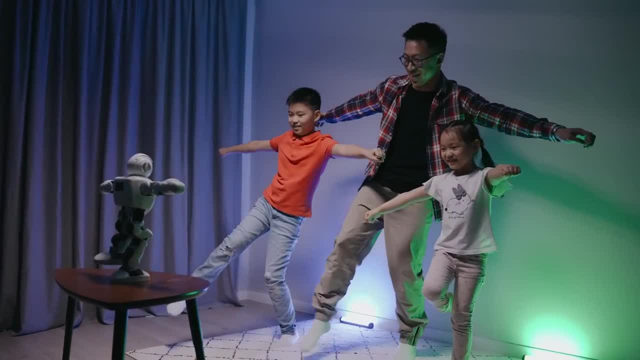 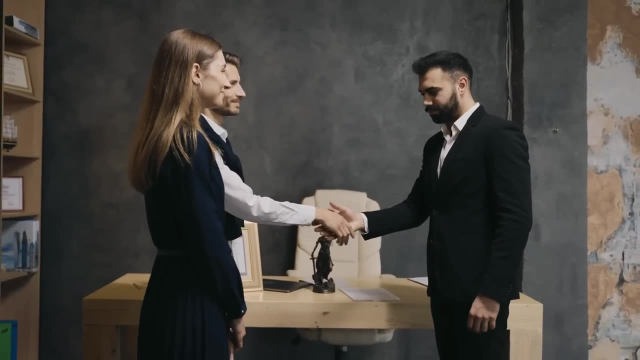 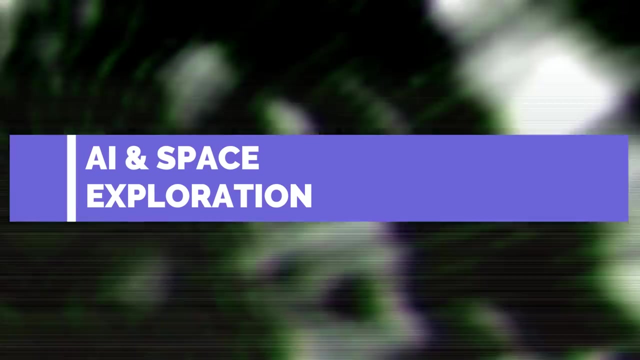 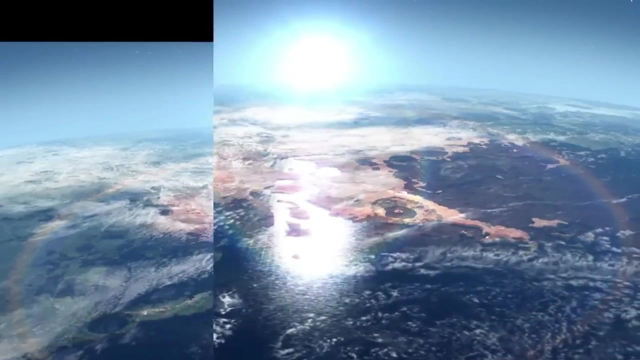 accountable? How do we ensure that AI is used in a way that is fair and equitable for all people? These challenges will require collaboration and cooperation between governments, businesses and individuals as we work to develop a shared vision for the future of AI. As humanity continues to explore space and search for signs of extraterrestrial life. 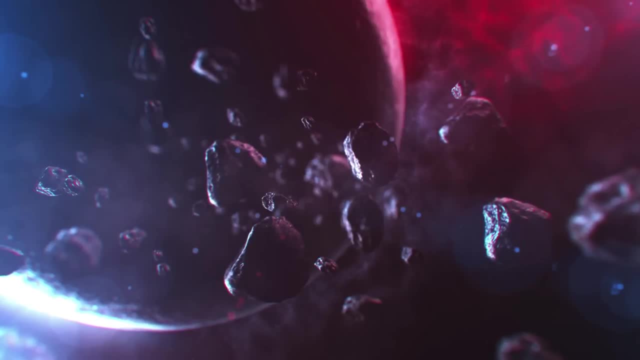 artificial intelligence is becoming an increasingly important tool in this endeavor. From robotic explorers to satellite networks, AI is helping us to collect and analyze the information that is needed to develop a future for AI. AI is helping us to collect and analyze the information that is needed to develop a future for AI. 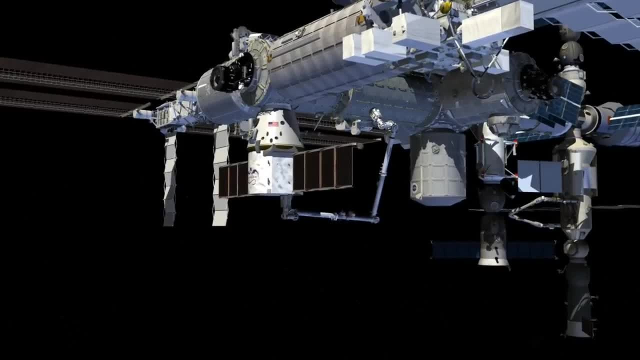 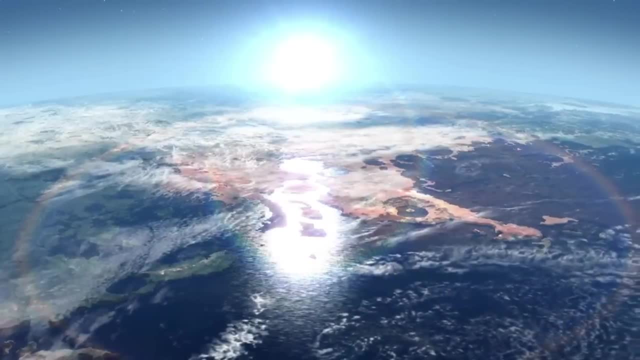 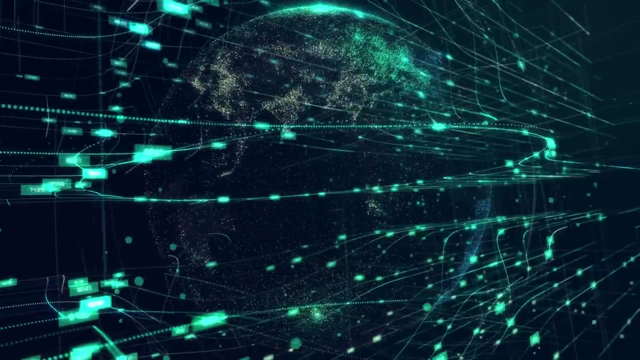 AI is helping us to collect and analyze data from some of the most distant and inhospitable regions of our solar system and beyond. One of the most obvious applications of AI in space exploration is in the development of robotic explorers. These machines are designed to operate autonomously in 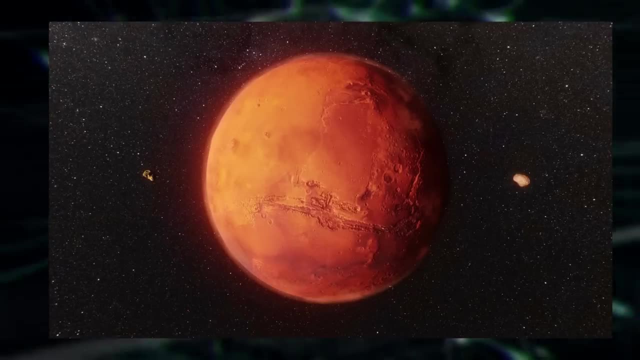 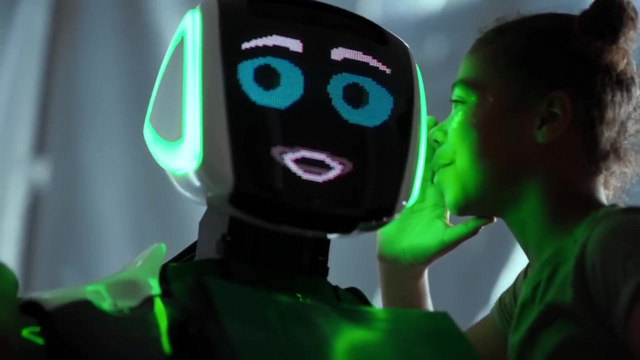 extreme environments, such as the surface of Mars or the icy moons of Jupiter. By using AI algorithms, these robots can make decisions in real time, adapt to changing conditions and even learn from their experiences to improve their performance over time. This allows us to explore areas that 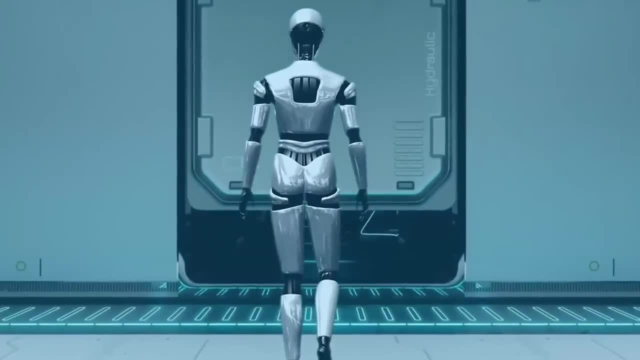 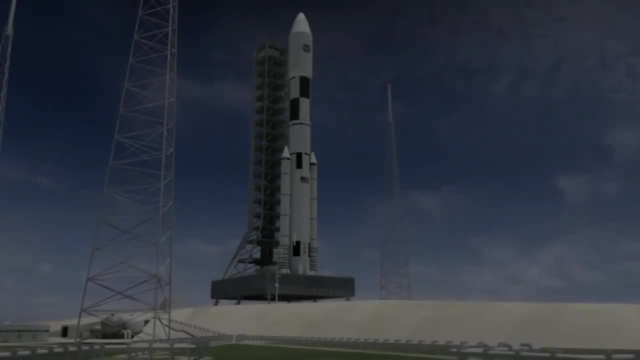 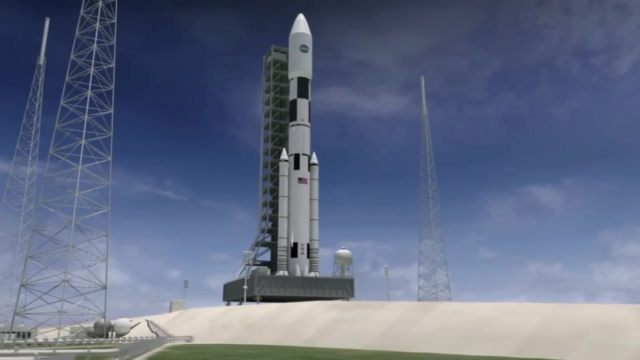 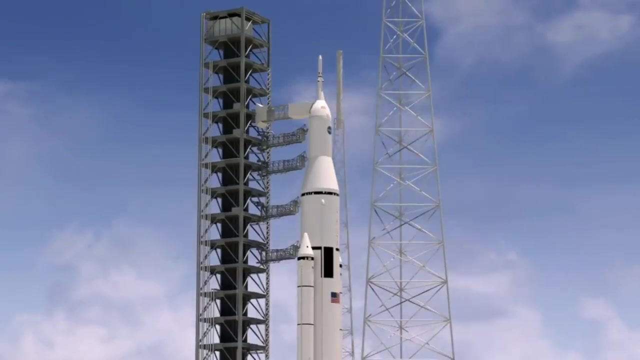 would be too dangerous or difficult for human astronauts, while still gathering valuable data and insights about our solar system. In addition to robotic explorers, AI is also being used to develop autonomous spacecraft that can navigate through space and perform complex tasks without human intervention. For example, NASA's Deep Space Network uses AI to manage a network of space. 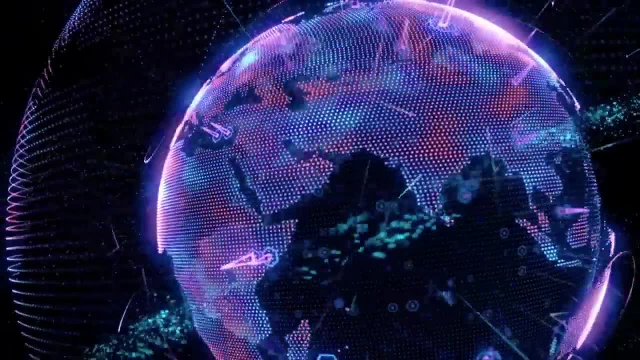 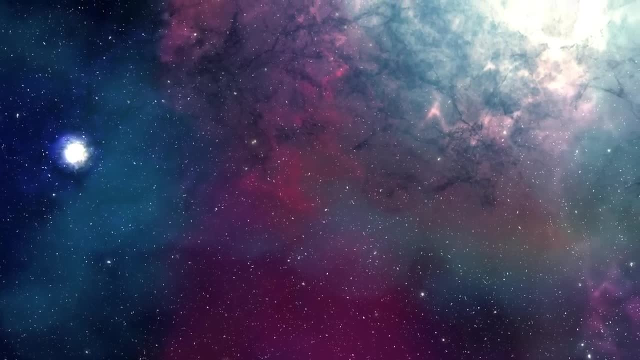 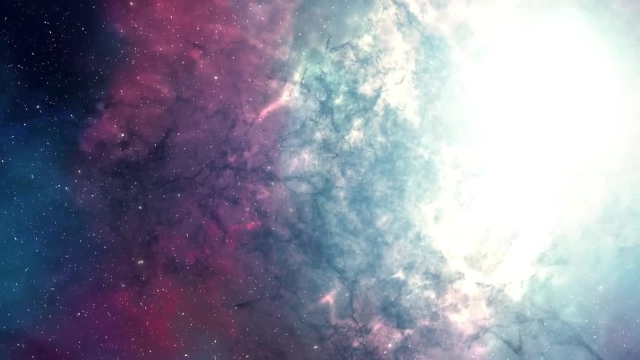 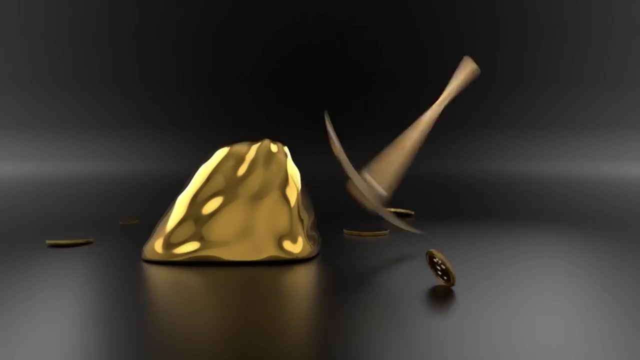 satellites and ground stations, ensuring that data is transmitted efficiently and effectively across vast distances. This type of technology will become increasingly important as we continue to explore deeper into space, where communication delays and other challenges make it difficult to control spacecraft in real time, As the demand for rare minerals and resources continues to. 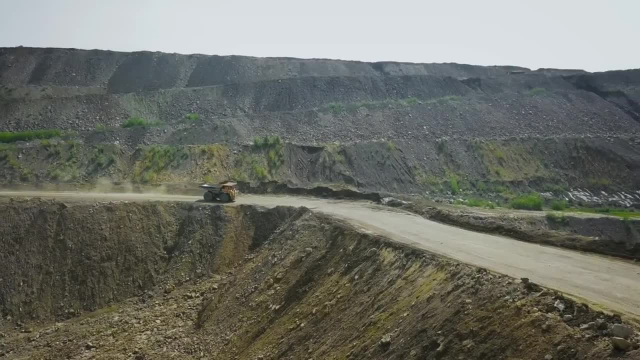 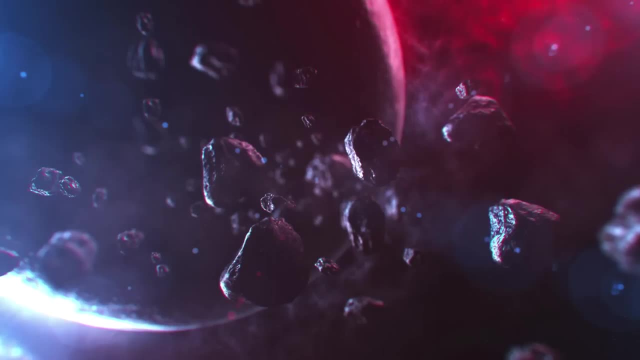 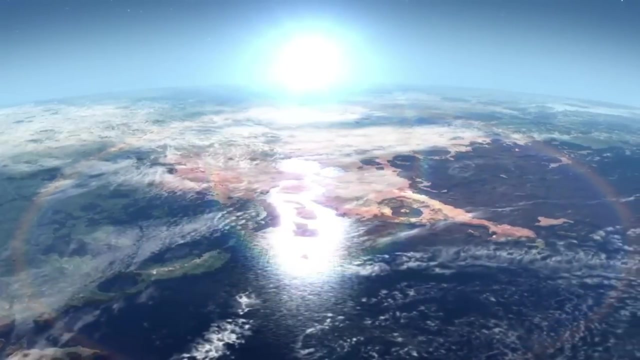 grow on Earth. some companies are turning to space mining as a potential solution. By mining asteroids and other celestial bodies, we could potentially access vast quantities of valuable resources without the environmental impact of traditional mining. AI is likely to play a key role in this endeavor, as it will be necessary to develop autonomous mining machines that can. 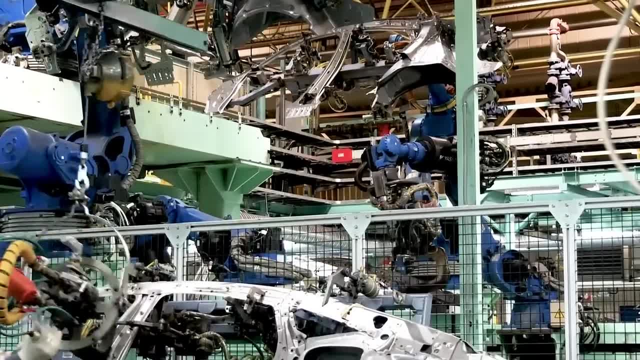 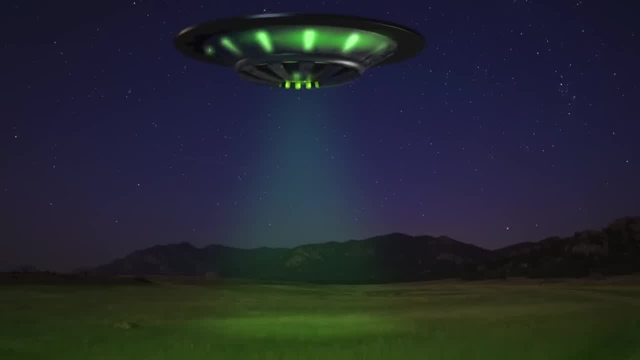 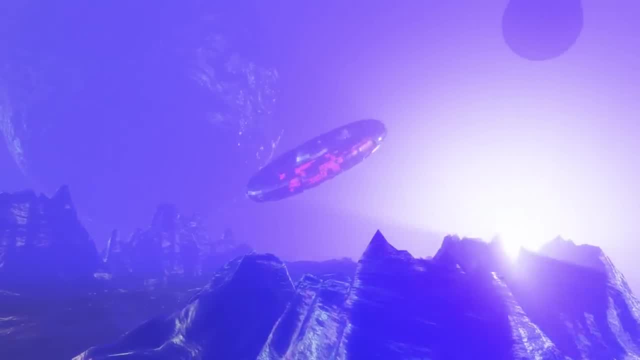 operate in low-gravity environments and navigate complex terrain with precision. One of the most exciting applications of AI in space exploration is in the search for extraterrestrial life. By analyzing data from telescopes and other sensors, AI algorithms can help us to identify patterns and anomalies that could indicate the presence of life on other. 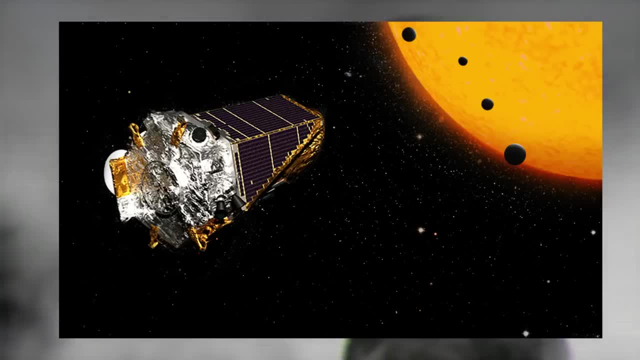 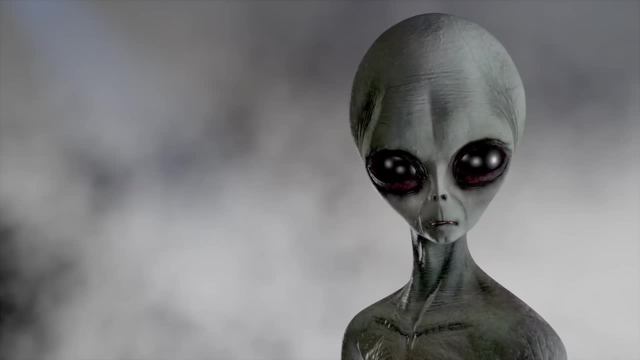 planets or moons. For example, NASA's Kepler mission used AI to analyze data from thousands of stars, identifying potential candidates for exoplanets and other interesting phenomena. As AI continues to evolve, it is likely that we will be able to detect even more subtle signals. 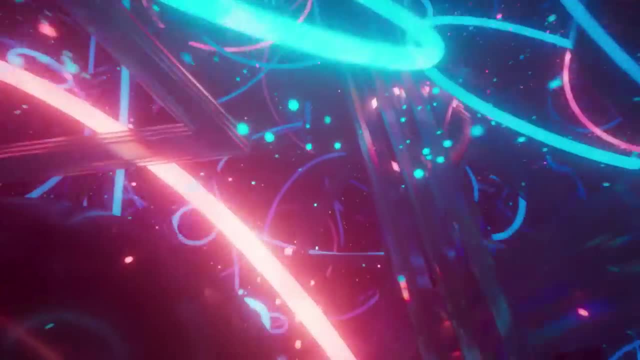 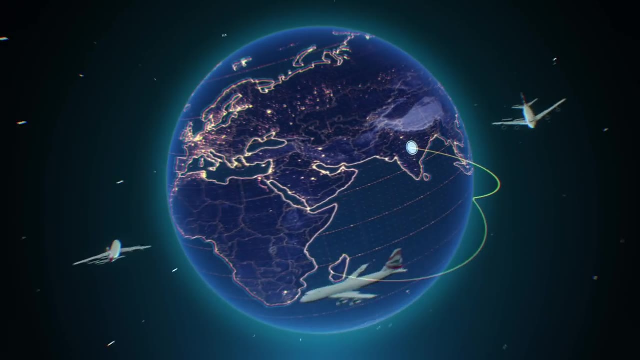 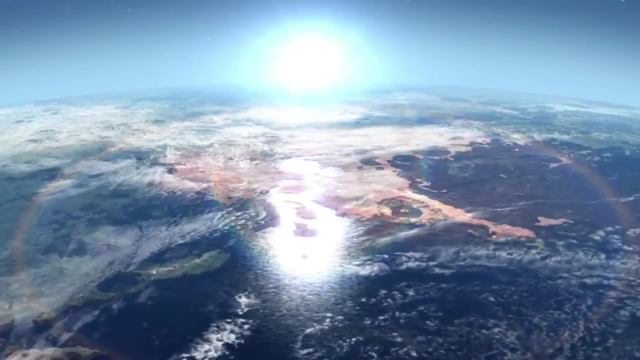 that could indicate the presence of life elsewhere in the universe. AI is rapidly becoming a critical tool in space exploration, allowing us to collect and analyze data from some of the most remote and hostile environments in our solar system and beyond. Whether we are exploring the surface of Mars, searching for extraterrestrial life, 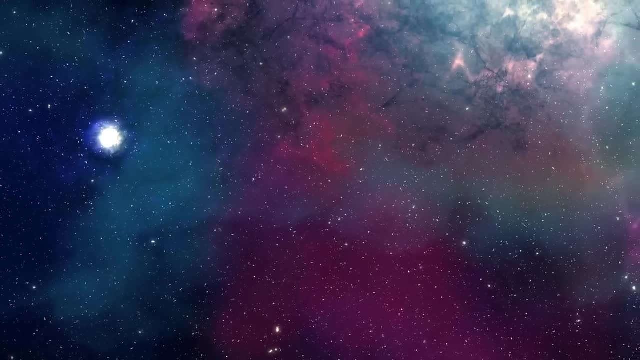 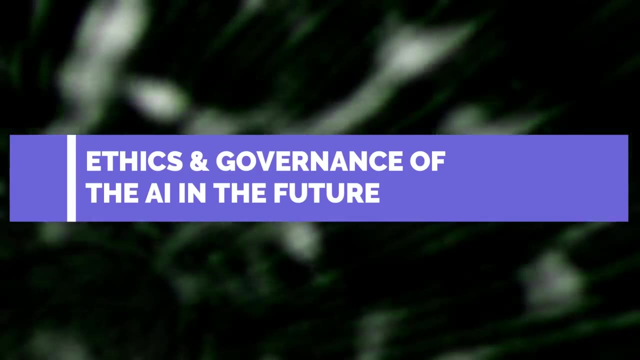 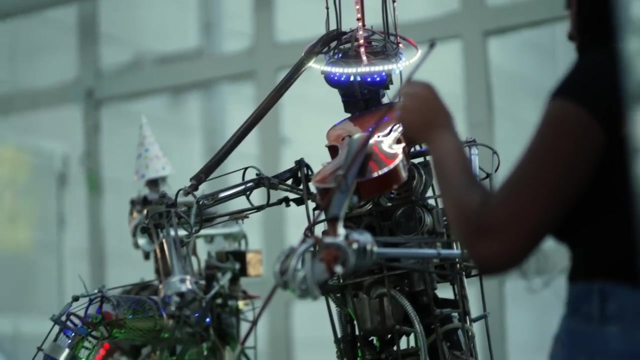 or mining asteroids for resources. AI will play a vital role in helping us to achieve our goals and advance our understanding of the universe. As AI continues to evolve, it is likely that we will be able to identify potential candidates for to advance and become more integrated into our daily lives. It is becoming increasingly important. 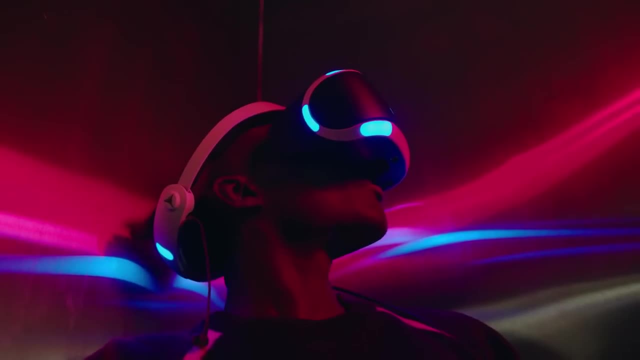 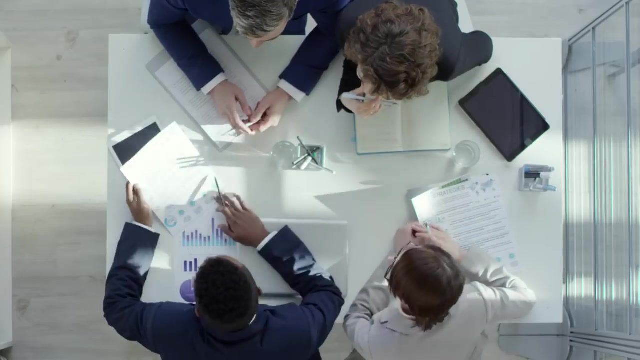 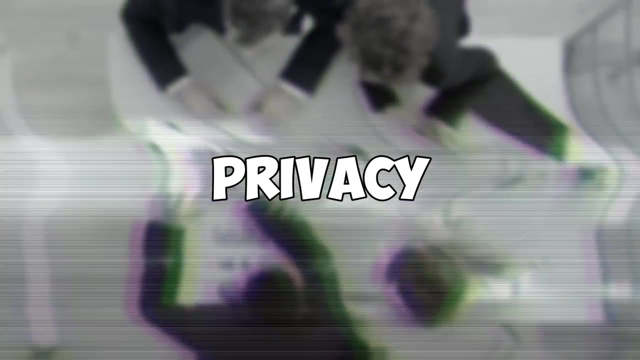 to consider the ethical and governance implications of these technologies. From privacy concerns to potential biases and decision-making algorithms, there are a wide range of issues that need to be addressed in order to ensure that AI is used in a responsible and ethical manner. One of the most pressing concerns around AI is the potential for these technologies to invade. 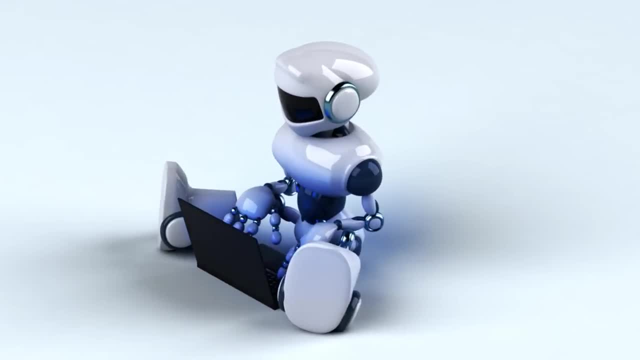 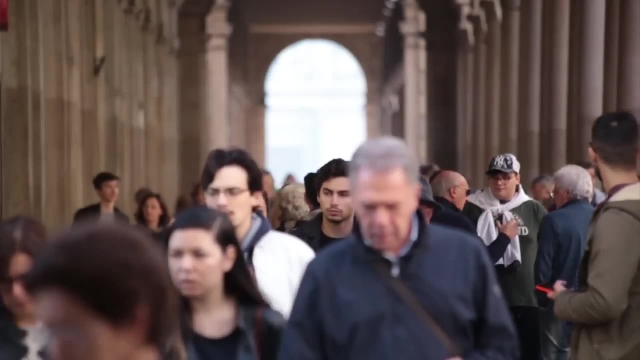 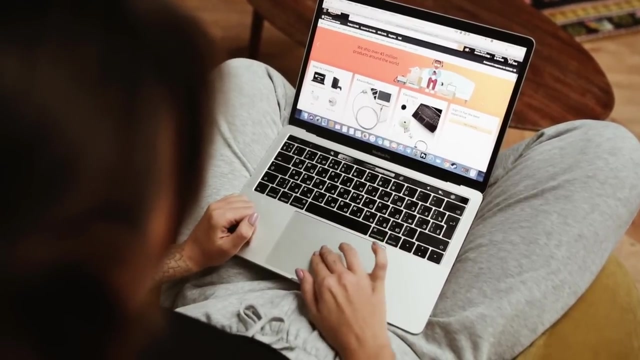 our privacy. As AI systems become more sophisticated and able to analyze vast amounts of data, there is a risk that they could be used to monitor our behavior, track our movements and collect sensitive personal information without our consent. To address this issue, it is important to establish clear guidelines around the collection. 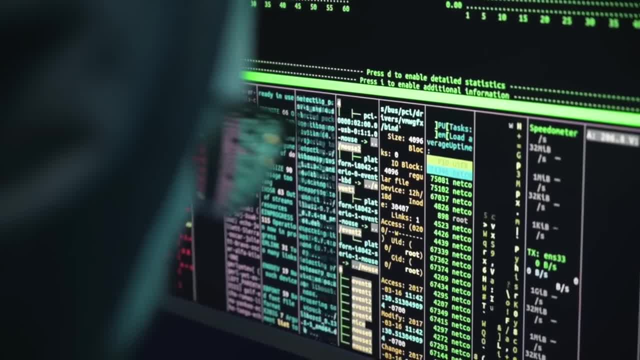 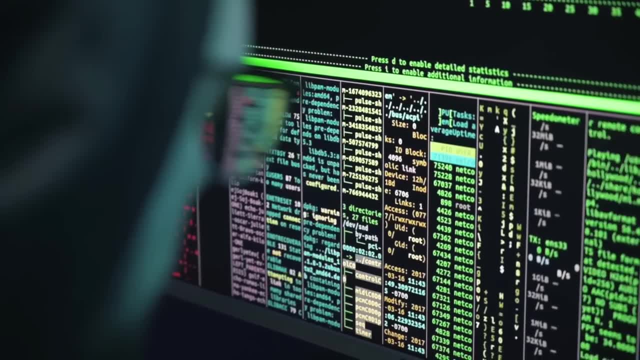 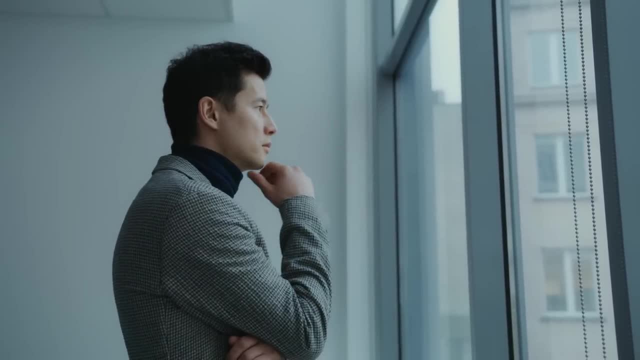 storage and use of personal data. Companies and organizations that use AI should be required to obtain explicit consent from individuals before collecting their data and should be held accountable for any misconduct. Another concern with AI is the potential for these systems to exhibit biases in decision-making. 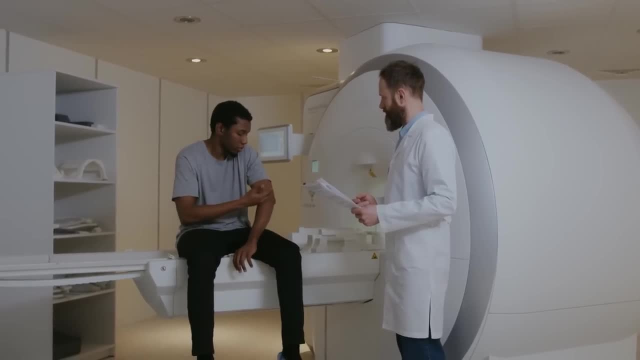 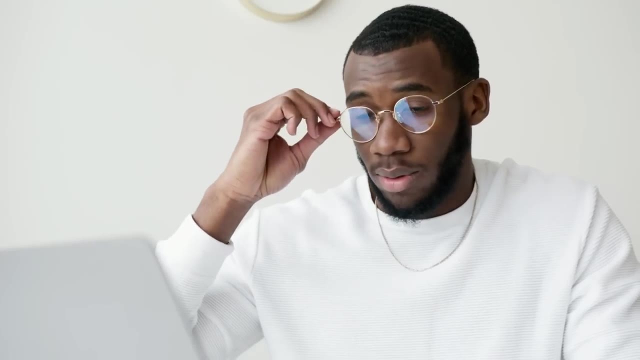 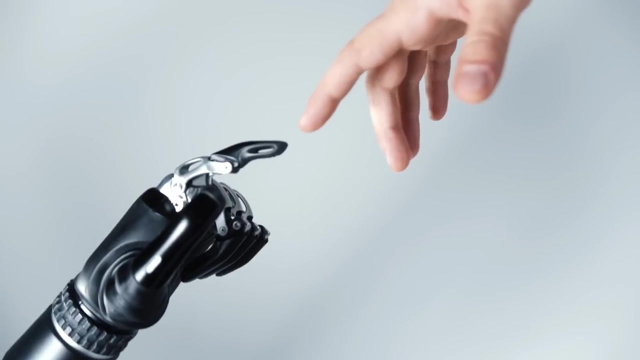 This can occur when the algorithms used in AI are based on biased data or assumptions, leading to unfair or discriminatory outcomes. To mitigate this risk, it is important to develop AI systems that are transparent and accountable. This means providing visibility into the data and algorithms that are used in these systems and establishing clear standards for assessing. 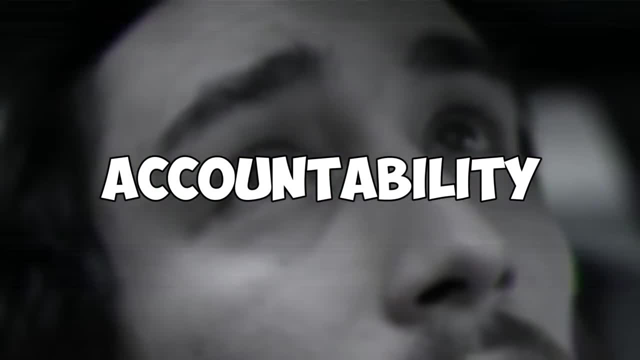 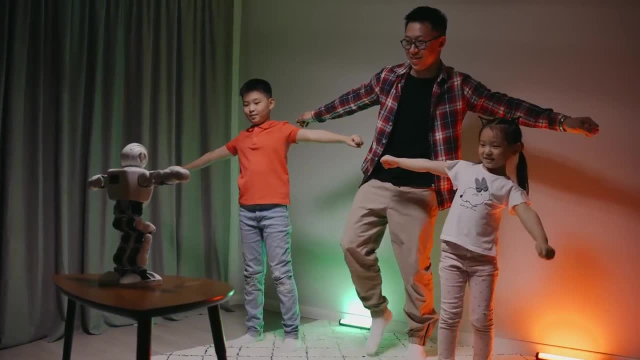 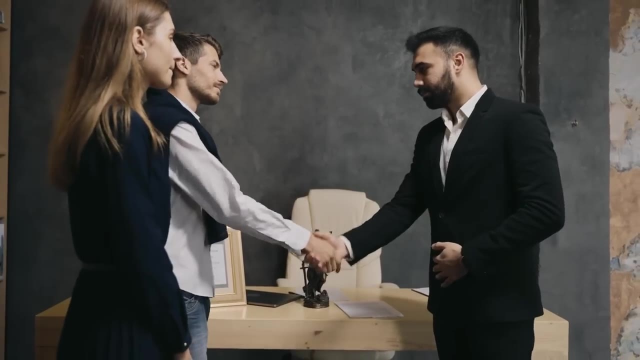 the fairness and accuracy of their outputs. One of the challenges with AI is the difficulty of assigning accountability when something goes wrong. Because these systems are often complex and involve multiple stakeholders, it can be difficult to determine who is responsible for any negative outcomes that arise. 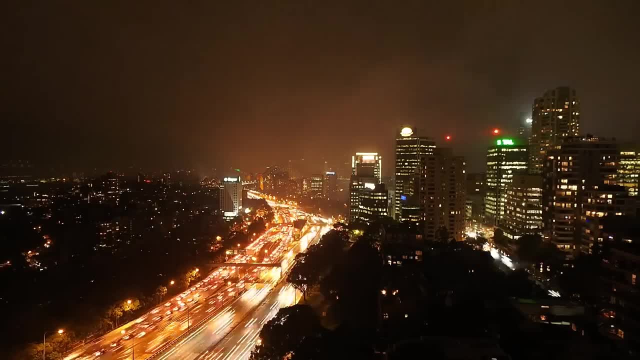 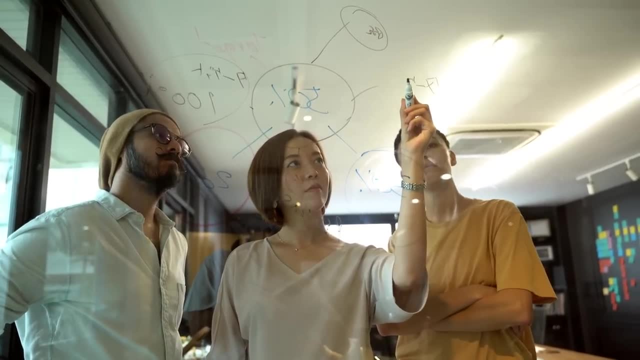 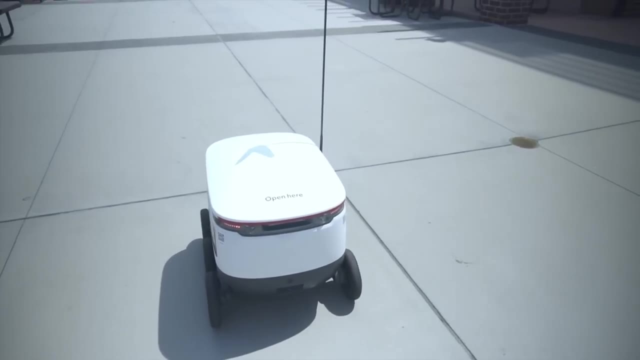 To address this issue, it is important to establish clear lines of accountability and responsibility for AI systems. This can include creating regulatory frameworks that hold companies and organizations accountable for the actions of their AI systems, as well as developing processes for investigating and resolving disputes or issues that arise. 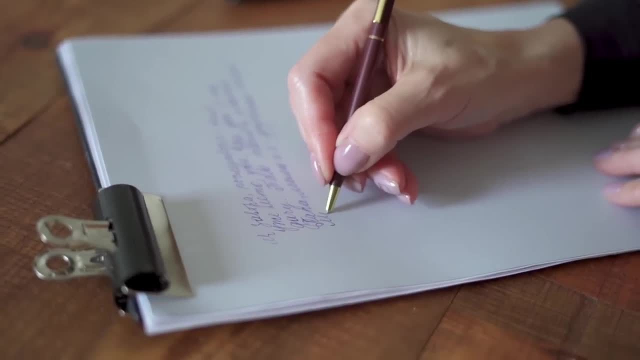 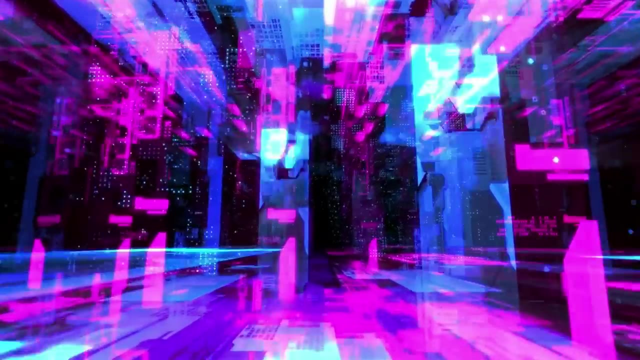 As AI becomes more pervasive and impacts more aspects of our lives, it is important to consider how these technologies should be governed. This includes questions around how AI systems should be regulated, who should have access to them and how their use should be monitored. 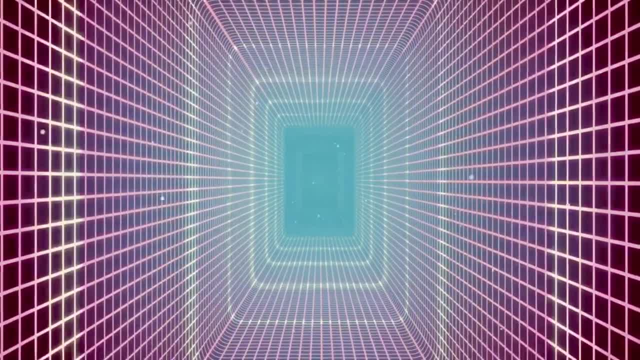 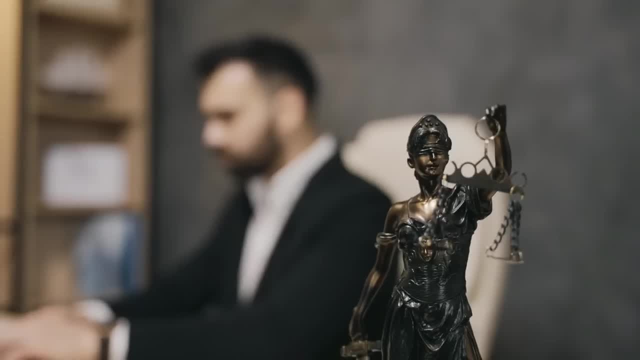 To address these issues. it is important to engage in oversight, open and transparent discussions around the governance of AI. This includes working with stakeholders from a wide range of backgrounds, including government officials, industry leaders and experts in ethics and technology, to develop frameworks. 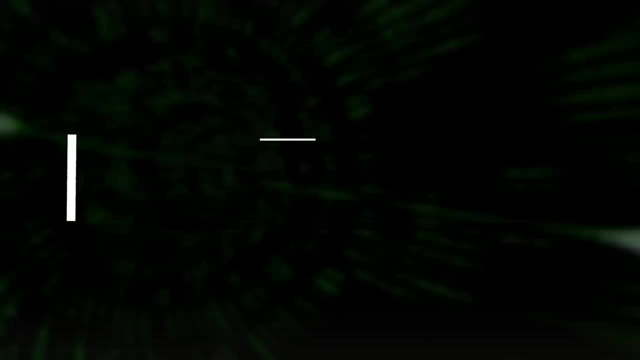 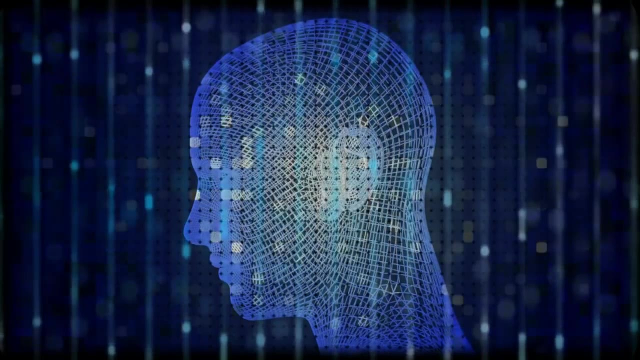 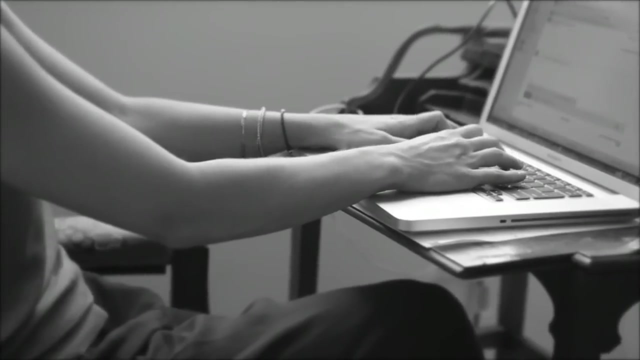 that balance innovation with responsible use. Artificial intelligence is already starting to impact our daily lives in a variety of ways, and this trend is only going to continue in the coming years, From the algorithms that power our social media feeds to the voice assistants we use. 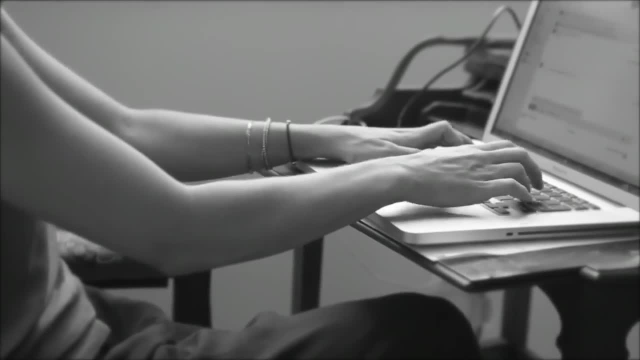 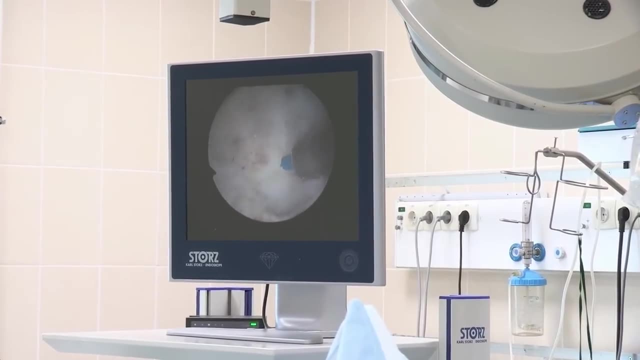 to control our homes. AI is becoming increasingly ubiquitous and integrated into our daily routines. One of the most significant ways that AI is impacting our lives is through the way we interact with technology. Advances in natural language processing and computer vision have made it possible to interact. 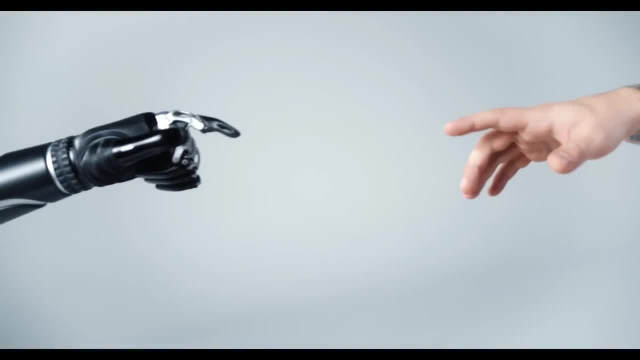 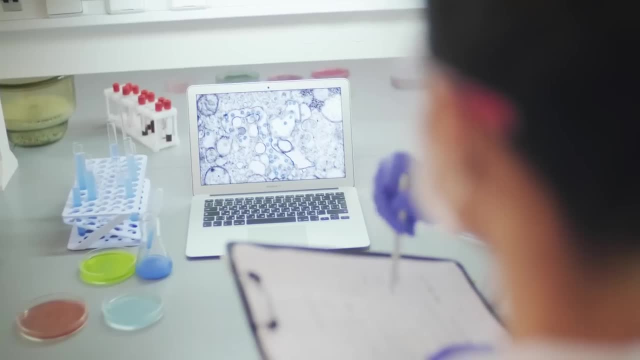 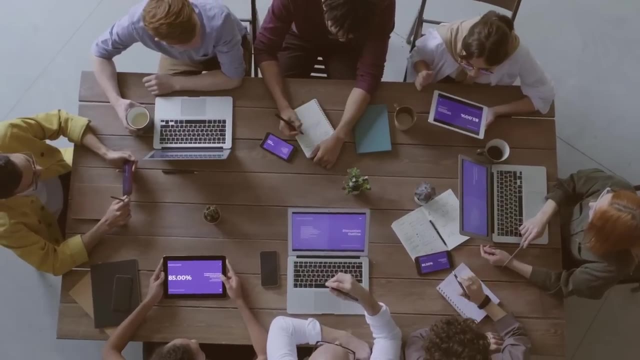 with technology in a more intuitive and human-like way, Allowing us to accomplish our goals. AI is also transforming the way we work In industries ranging from finance to health care. AI is being used to automate repetitive tasks and improve efficiency, allowing workers to focus on more complex and high-level tasks. 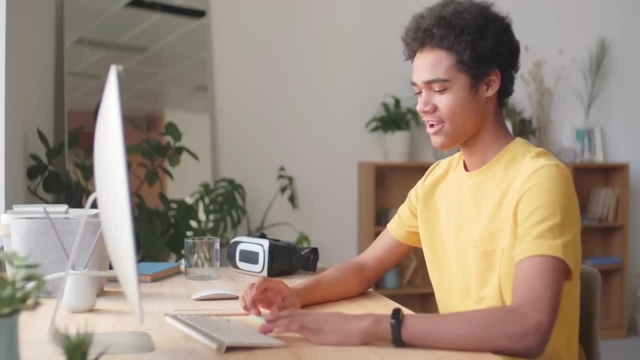 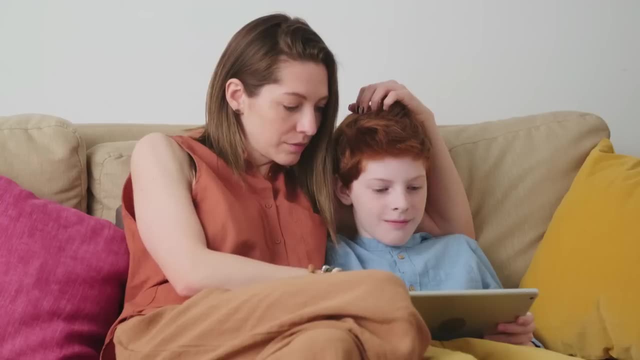 This has the potential to create new opportunities for workers and drive economic growth. In the home, AI is already being used to control a variety of devices and appliances. Voice assistants like Amazon's Alexa and Google Assistant are being used to control a variety of devices and appliances. 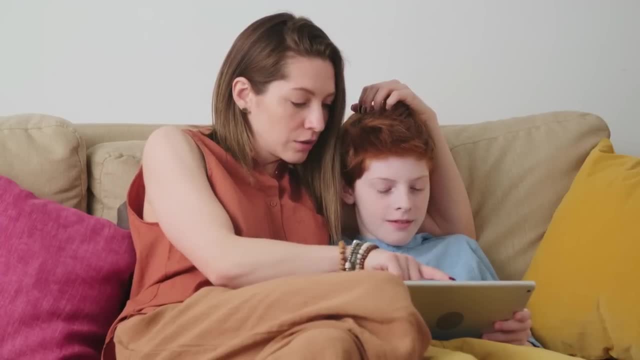 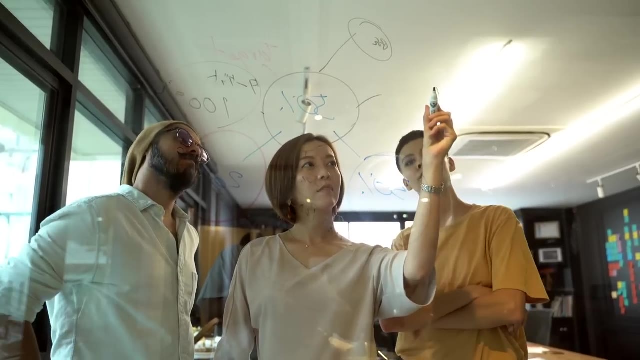 Voice assistants like Amazon's Alexa and Google Assistant are being used to control a variety of devices and appliances. AI is becoming increasingly popular, allowing us to control our lights, thermostats and entertainment systems with simple voice commands. In the future, we may see even more sophisticated AI systems that can anticipate our needs and 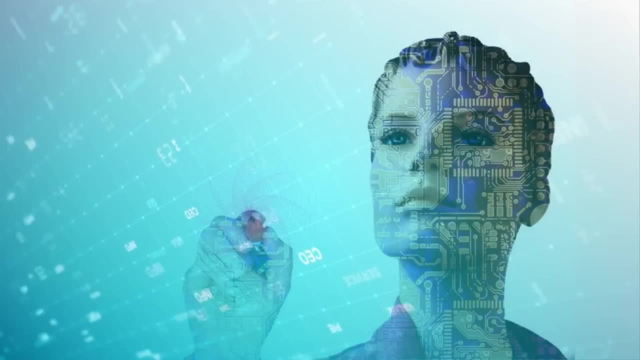 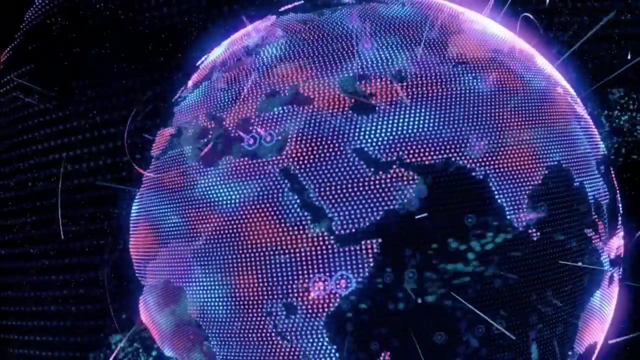 preferences, making our homes more comfortable and convenient. Of course, as with any new technology, there are also potential downsides to the increased use of AI in our daily lives. One concern is that AI systems may be used to manipulate or deceive us, either through 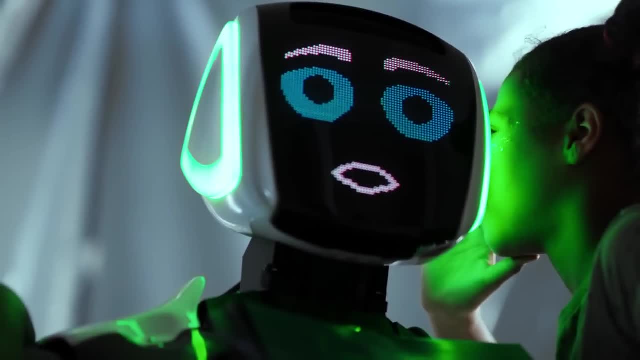 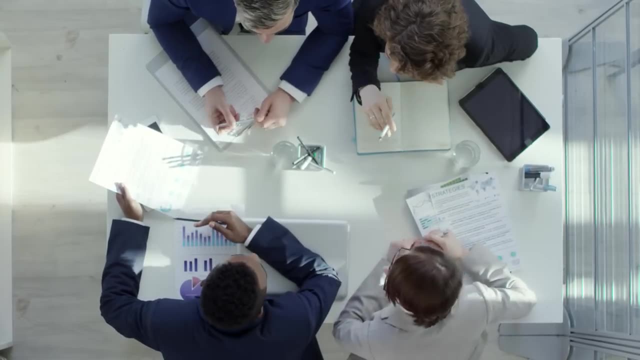 targeted advertising or by presenting us with biased information. There is also a risk that AI systems may be used to replace human workers, leading to job loss and economic disruption. As we move forward into a future that is increasingly defined by AI, it is important to consider 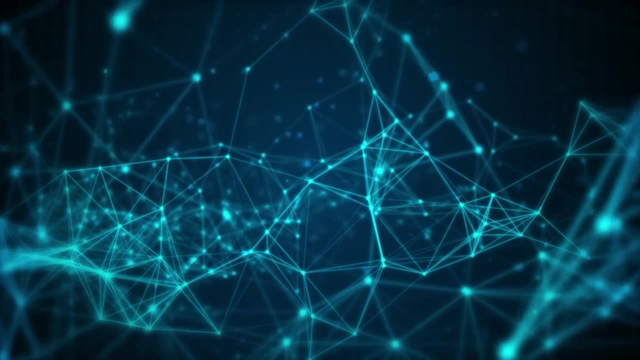 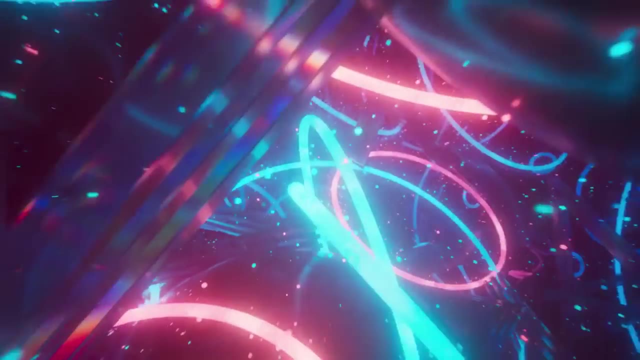 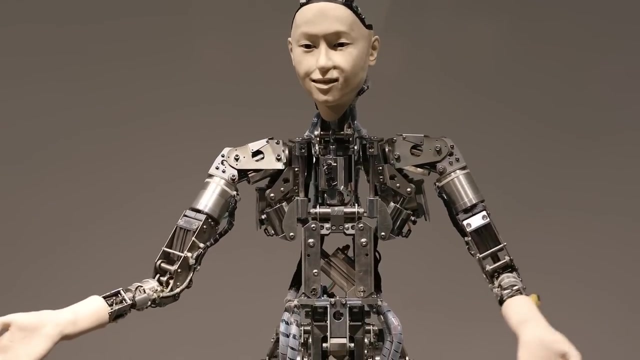 both the potential benefits and the potential risks of these technologies. By doing so, we can work to ensure that AI is used in a responsible and ethical manner that benefits society as a whole. As AI becomes increasingly integrated into our daily lives and the global economy, it 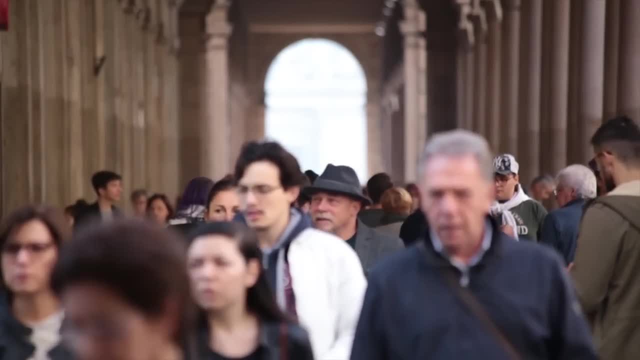 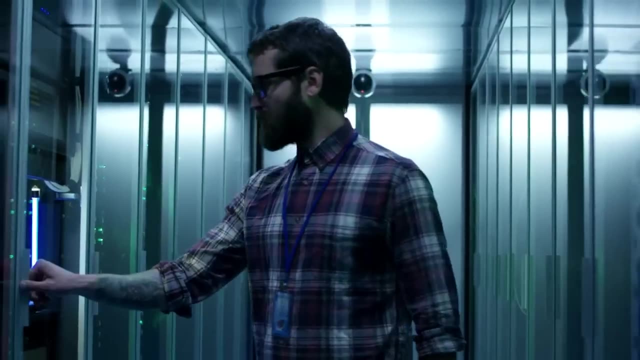 is important for individuals to understand both the opportunities and challenges that this technology presents. On one hand, AI has the potential to create new jobs and opportunities in a variety of industries, while on the other hand, it may also lead to job displacement and economic 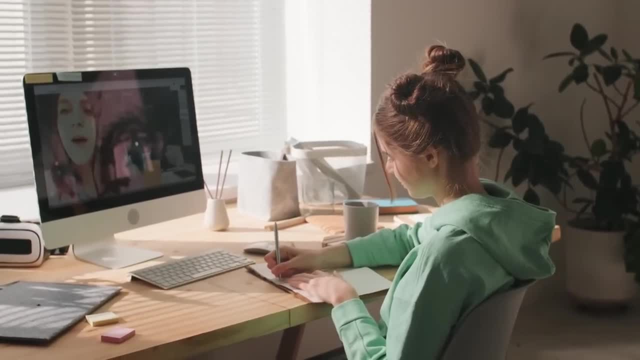 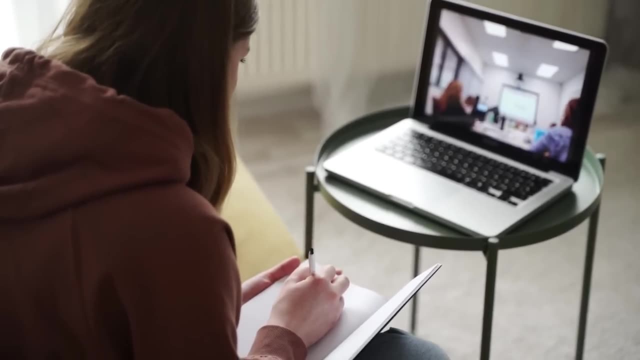 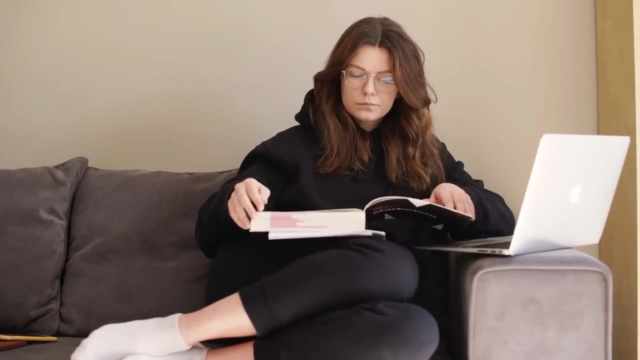 disruption. One of the biggest opportunities presented by AI is the potential for increased productivity and efficiency. By automating repetitive tasks and providing insights based on vast amounts of data, AI can help workers to focus on higher-level tasks that require creativity and problem-solving skills. 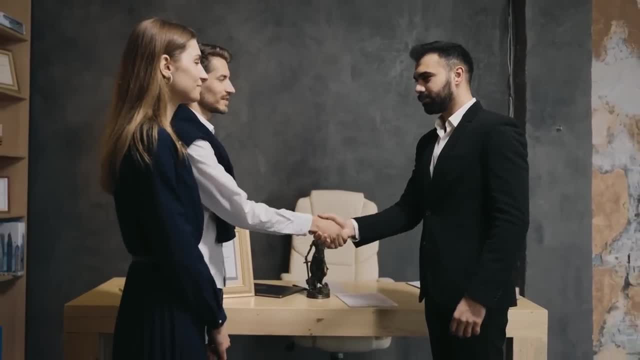 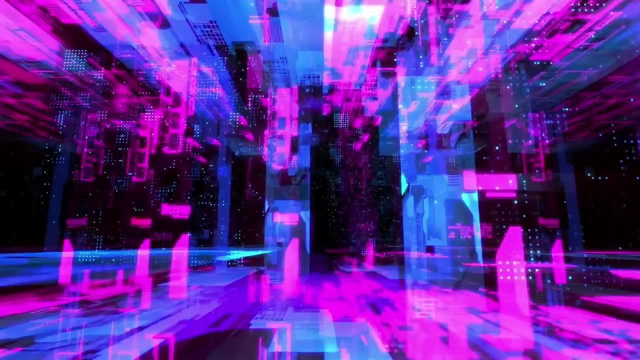 This can lead to greater job satisfaction and more fulfilling careers. Another opportunity presented by AI is the potential for innovation and entrepreneurship. As AI continues to evolve and become more sophisticated, there will likely be new opportunities for individuals and businesses to create innovative products and services. 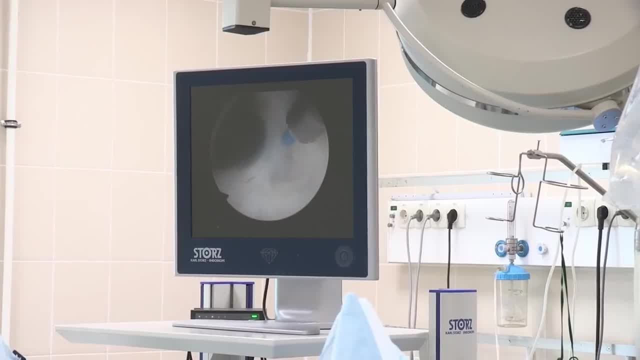 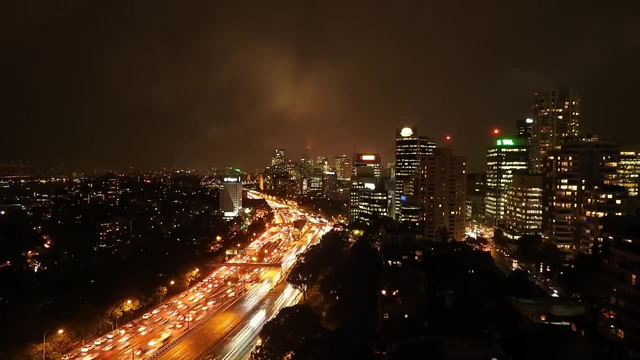 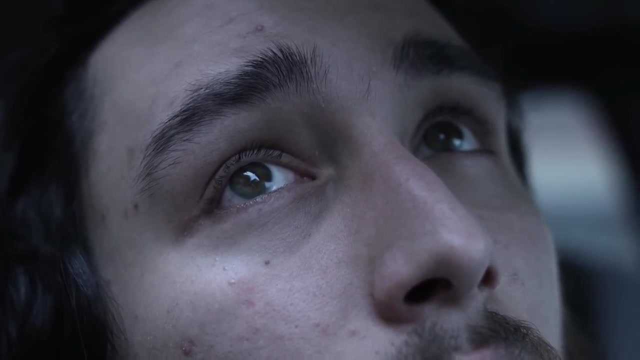 However, there are also several challenges that individuals may face in an AI-driven future. One of the most significant challenges is the potential for job displacement. As AI systems become more advanced, they may be able to perform tasks that were previously done by humans, leading to job loss in certain industries. 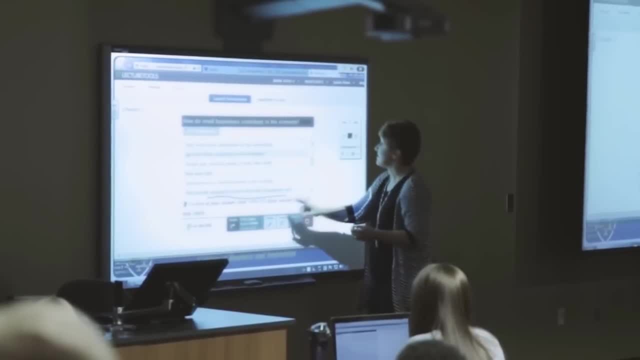 Another challenge is the potential for bias and discrimination in AI systems. If AI algorithms are trained on biased data, they may perpetuate bias and discrimination. This is a very important challenge. This is a very important challenge. AI systems can be used to evaluate and even amplify existing social inequalities. 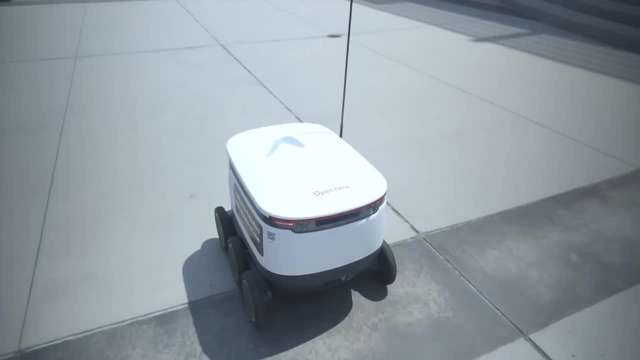 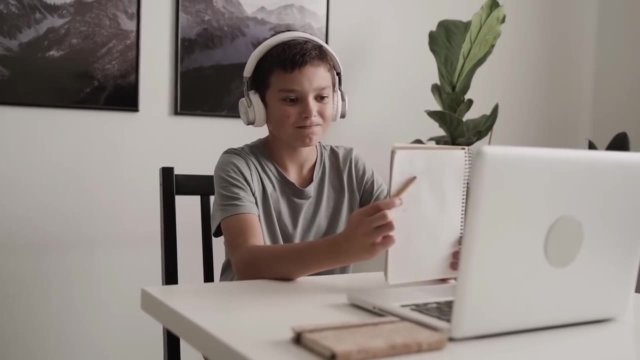 AI systems can be used to evaluate and even amplify existing social inequalities. AI systems can be used to evaluate and even amplify existing social inequalities. It is important for individuals to be aware of these issues and work to ensure that AI systems are designed and implemented in an ethical and responsible manner. 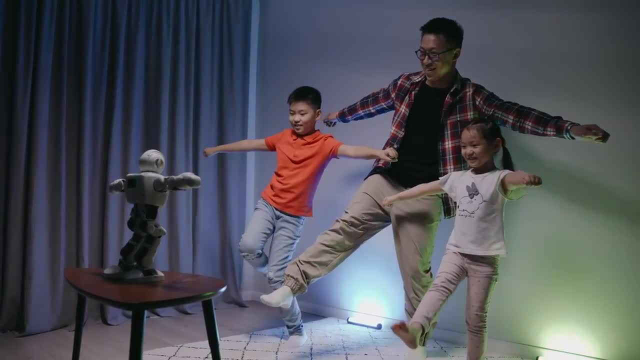 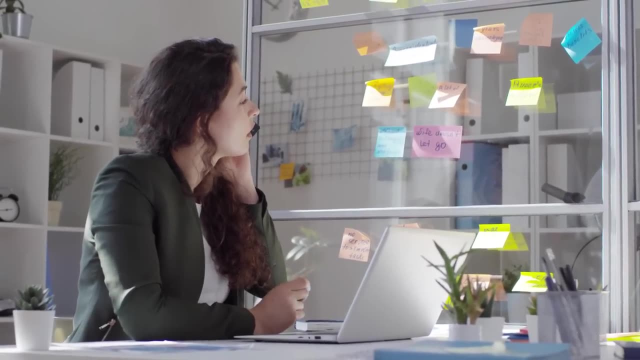 Finally, there is also a concern that AI may be used to invade our privacy and monitor our behavior. As AI becomes more integrated into our homes and workplaces, it is important for individuals to understand the implications of this technology and take steps to protect their personal data. 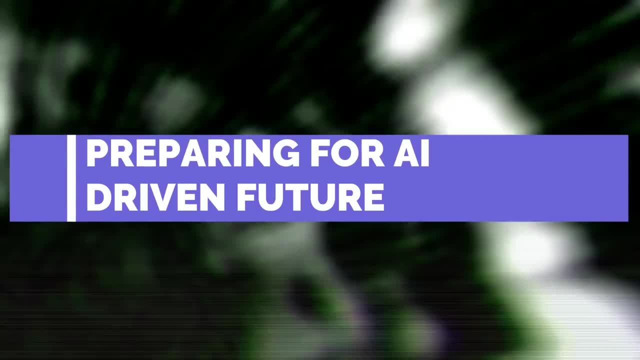 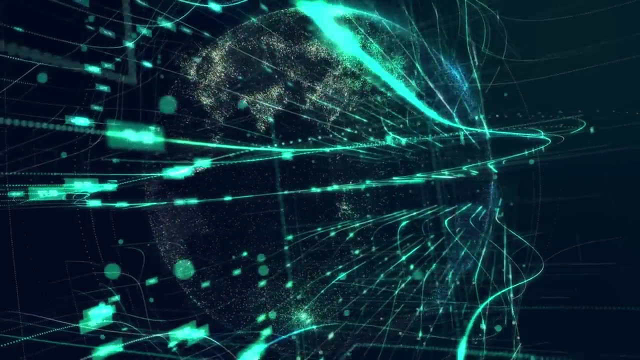 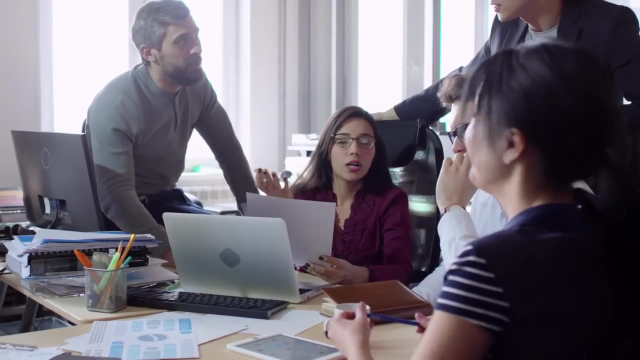 Also, the possibility of AI systems being developed today will be an area of considerable good for artificial intelligence. As AI becomes increasingly integrated into our daily lives, it is important for individuals to prepare for the changes and challenges that this technology presents. Here are some steps that individuals can take to prepare for an AI-driven future. 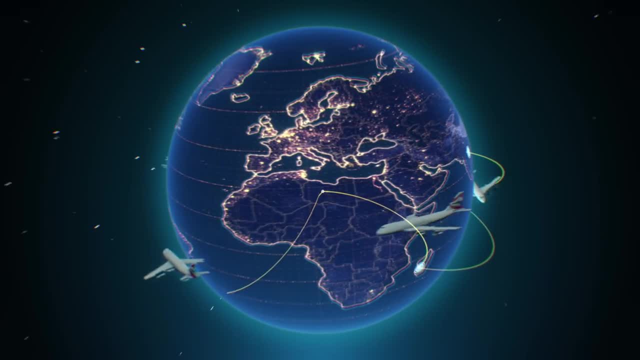 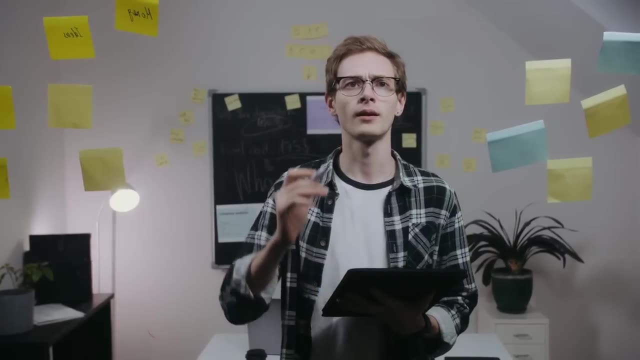 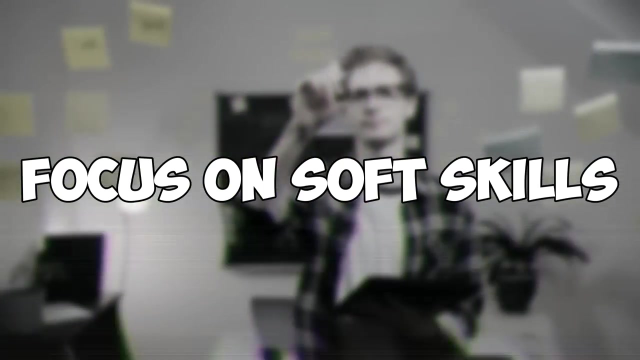 As AI becomes more prevalent, there will likely be an increased demand for individuals with technical skills in areas such as data analysis, programming and machine learning. By developing these skills, individuals can position themselves for new job opportunities and career advancement. While technical skills are important, it is also essential for individuals to develop. 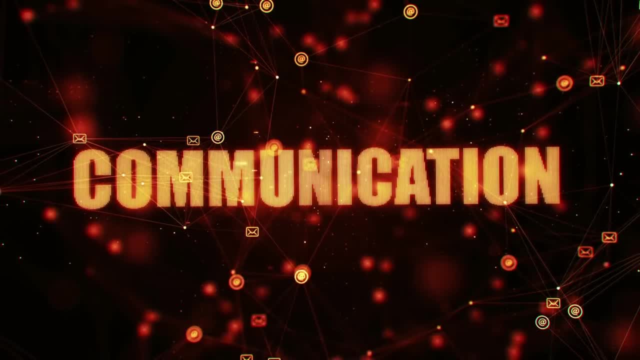 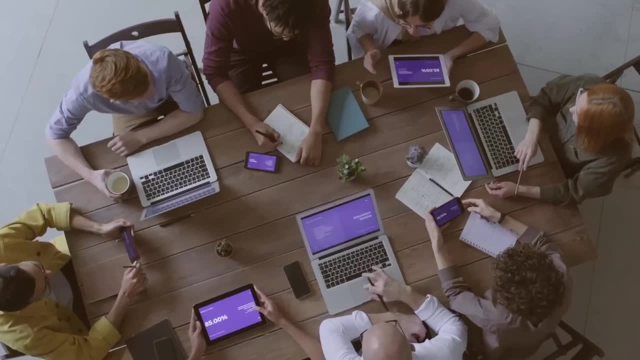 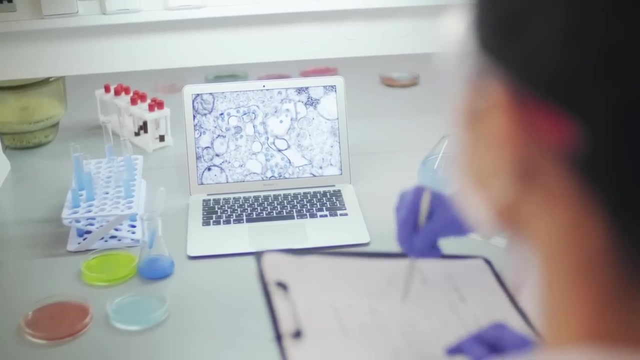 soft skills such as creativity, problem solving and communication. These skills will be in high demand as AI systems automate more routine tasks and human workers focus on higher-level activities. It is important for individuals to stay up-to-date on the latest developments in AI and the potential. 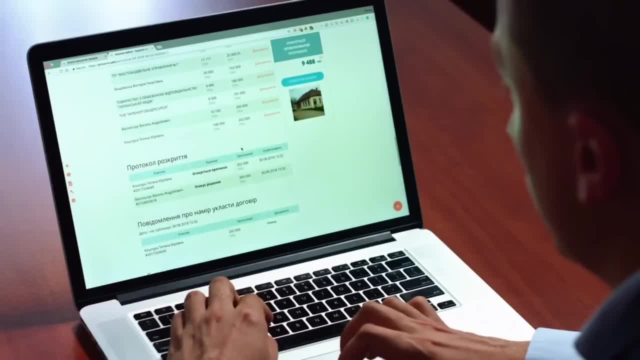 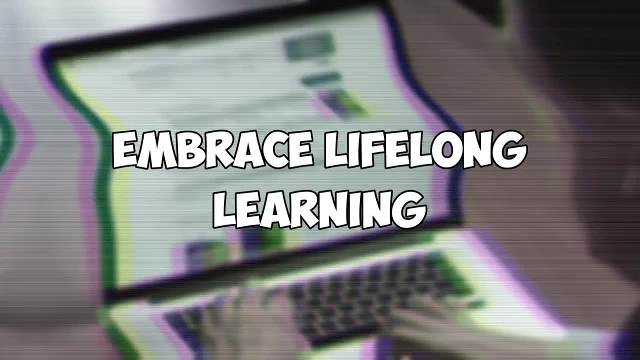 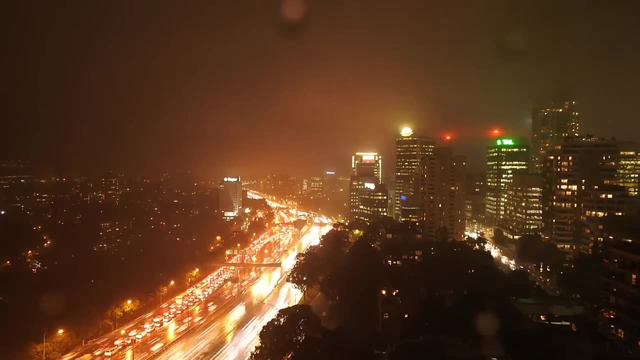 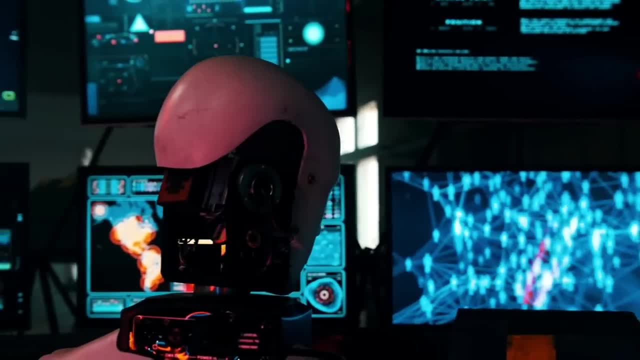 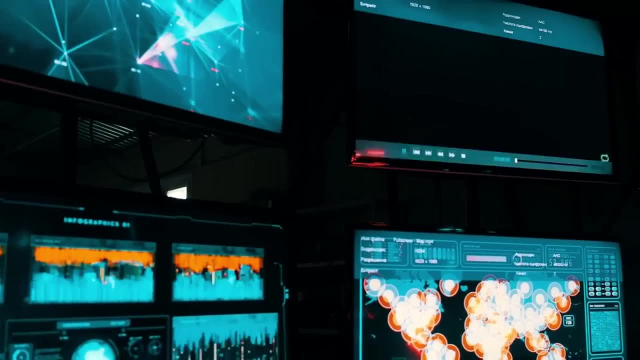 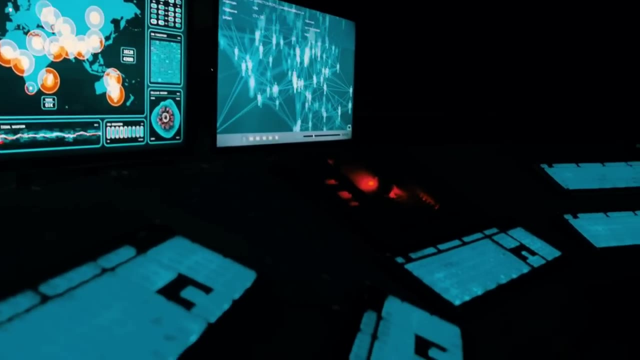 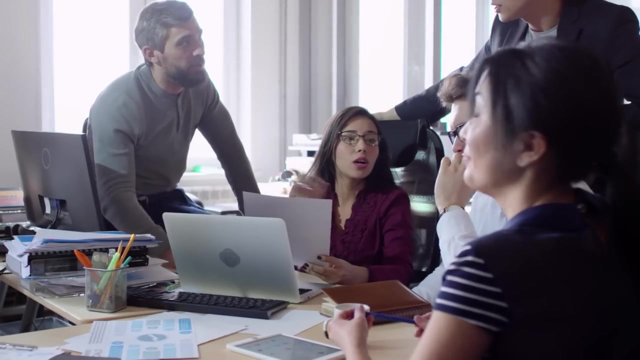 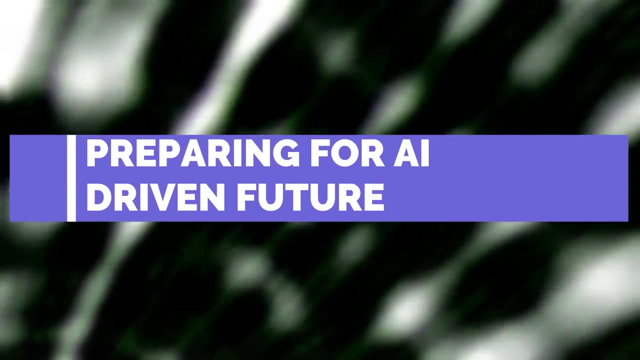 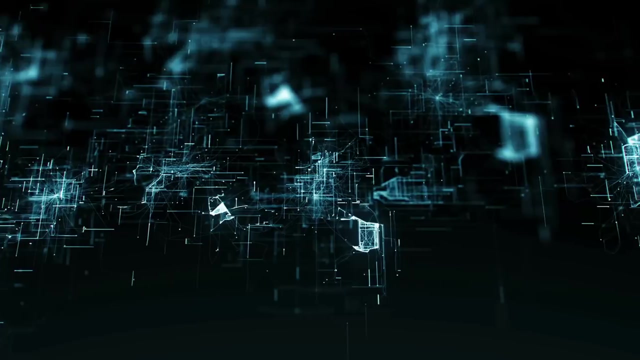 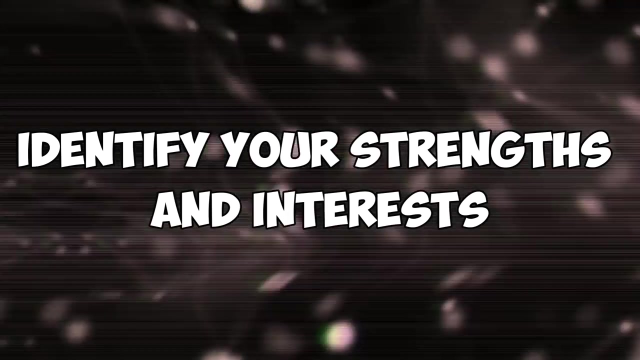 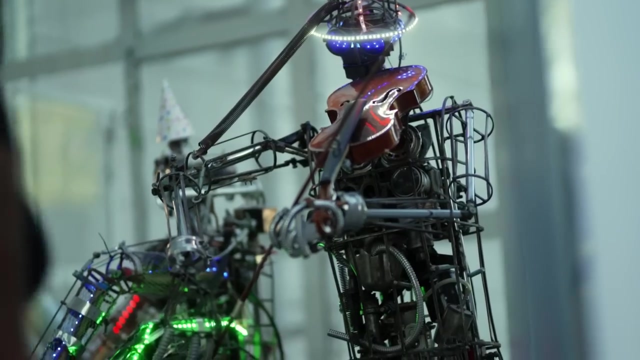 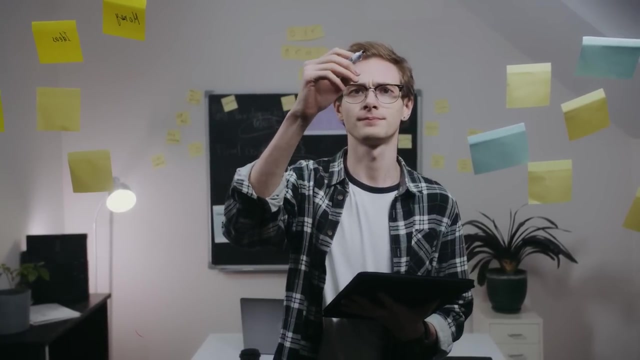 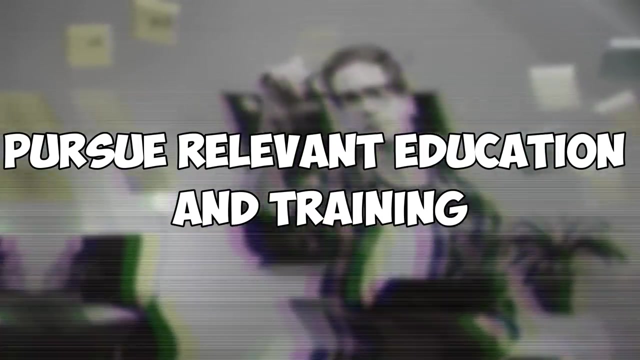 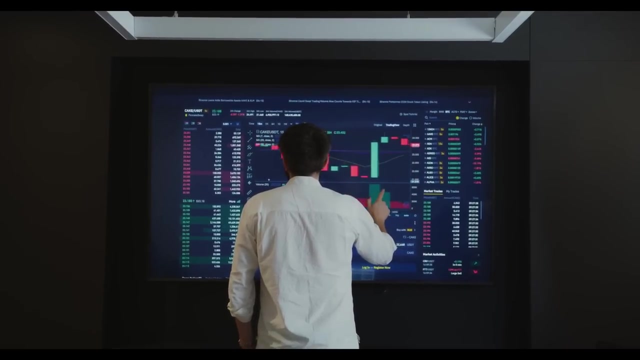 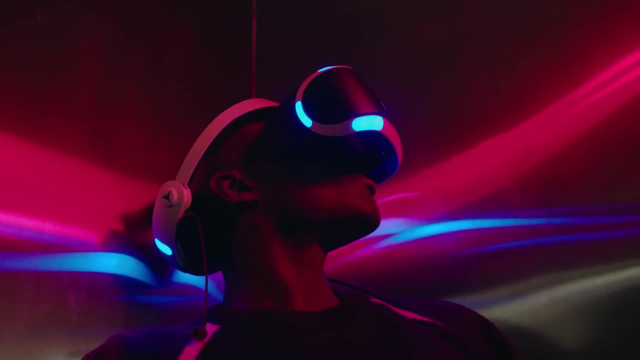 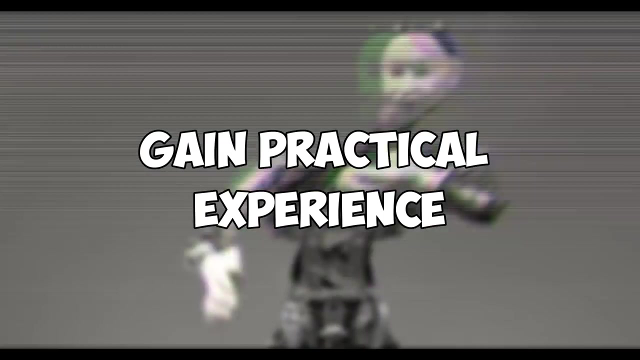 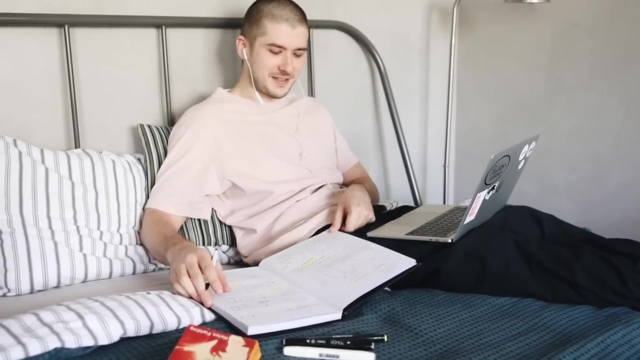 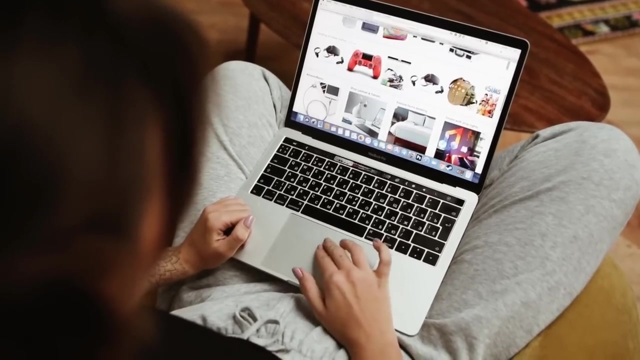 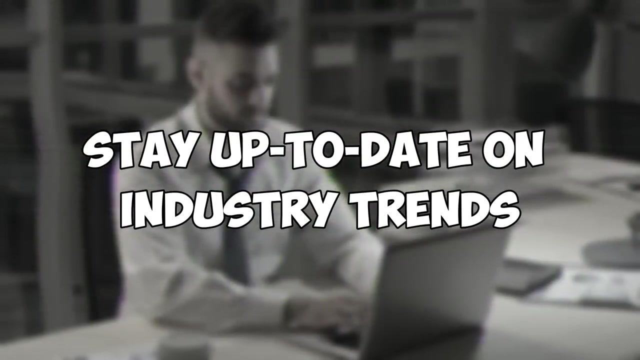 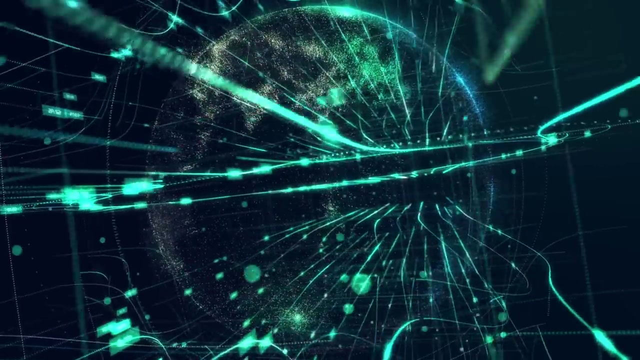 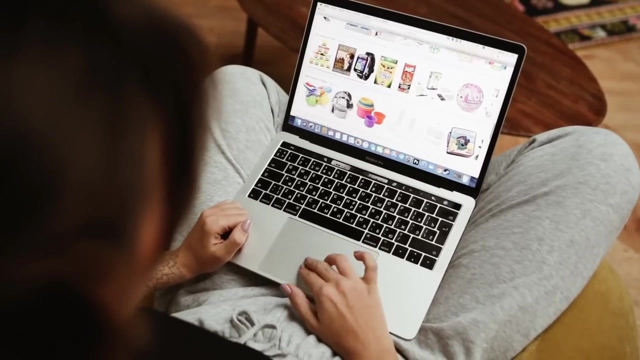 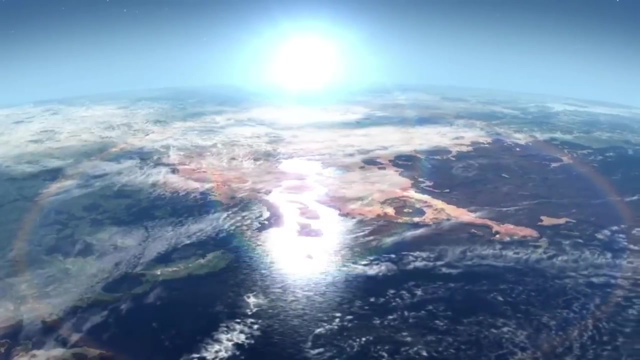 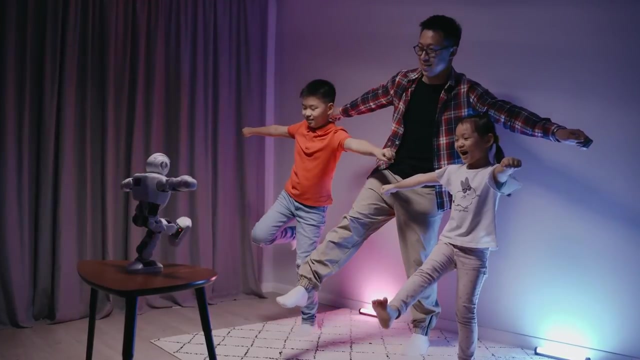 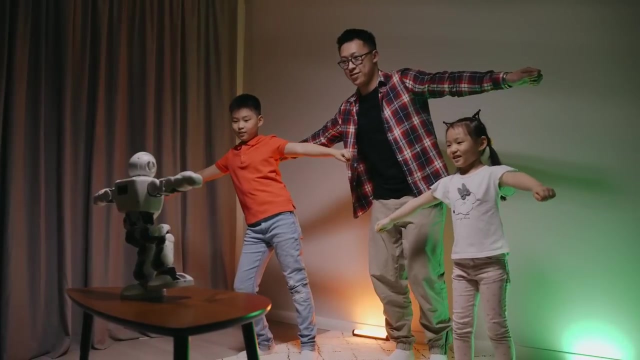 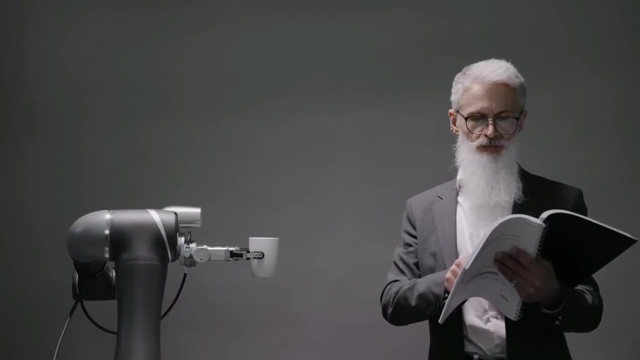 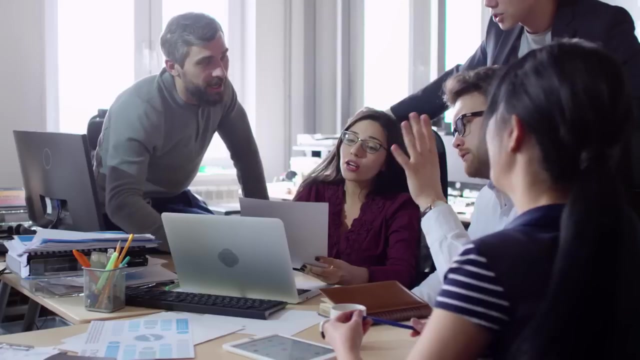 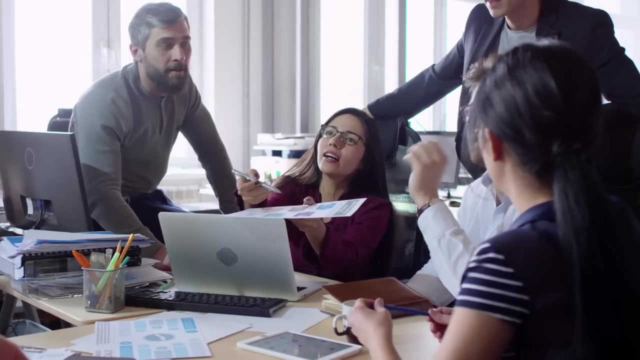 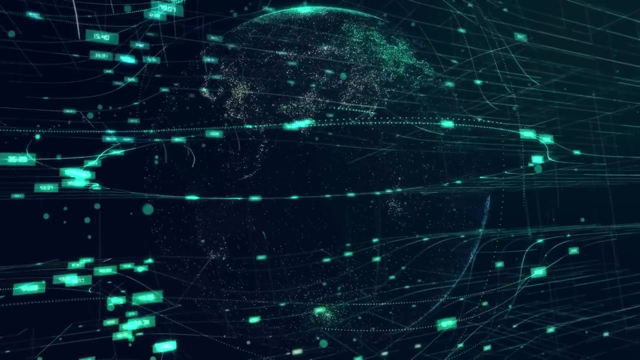 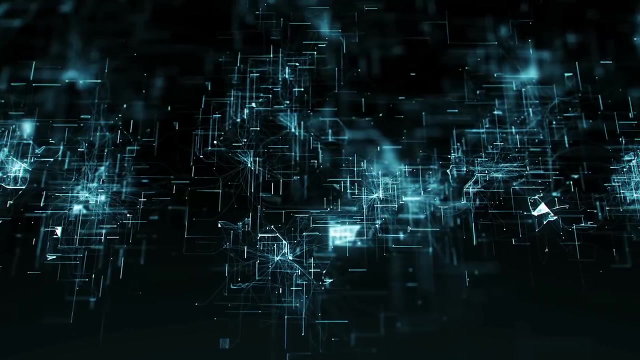 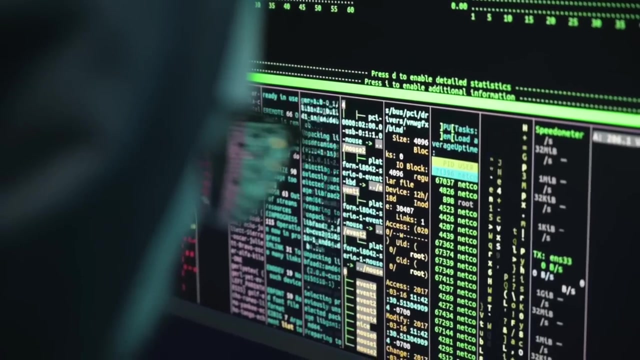 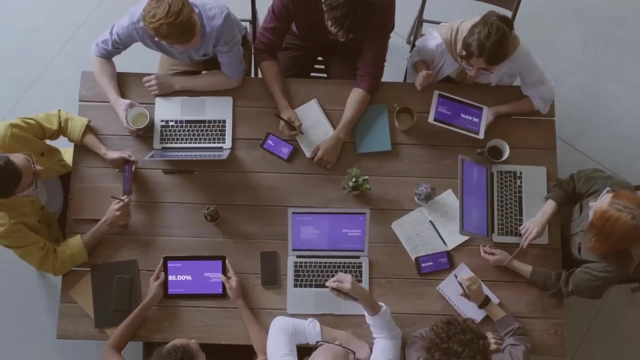 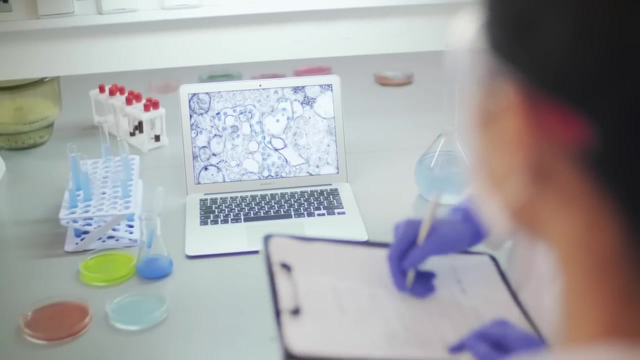 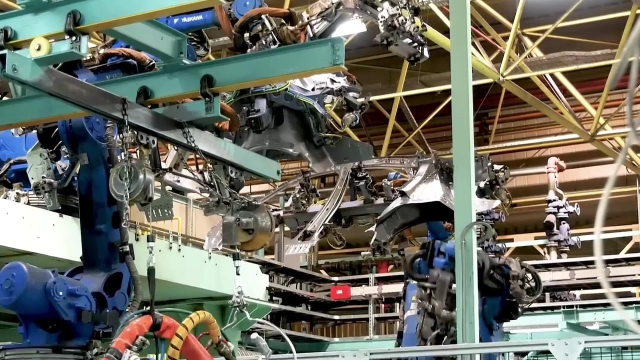 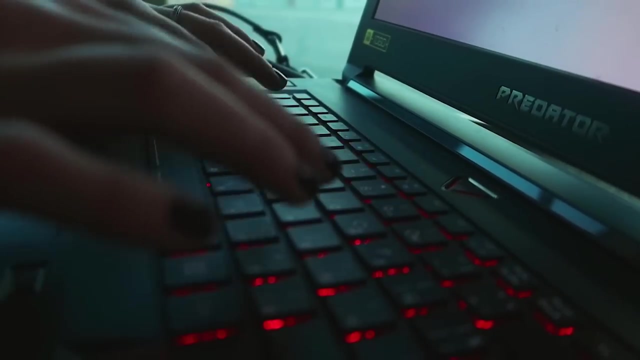 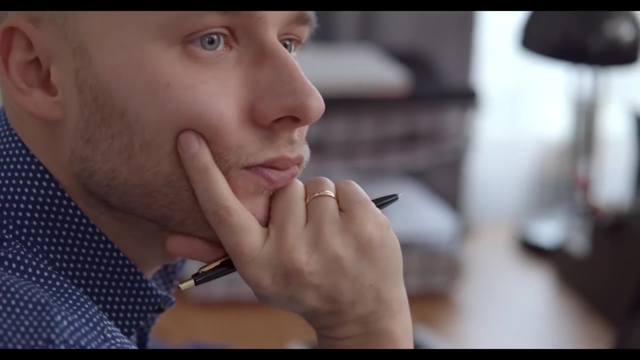 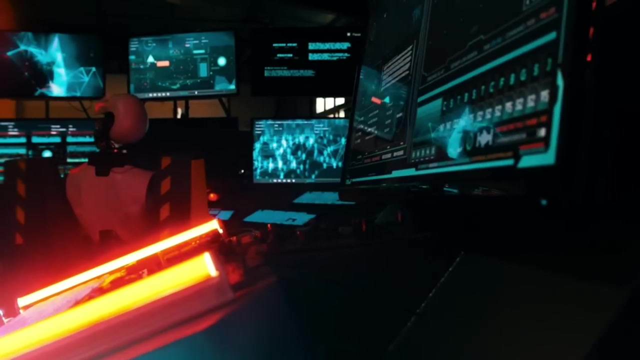 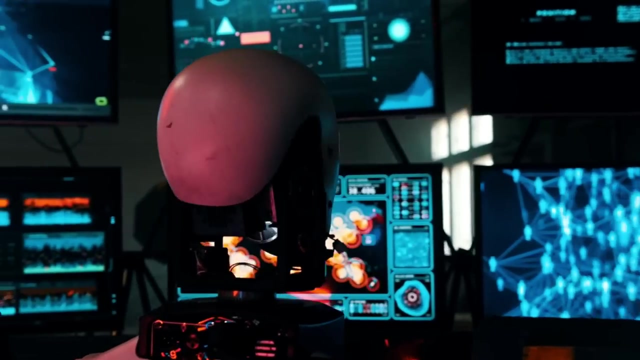 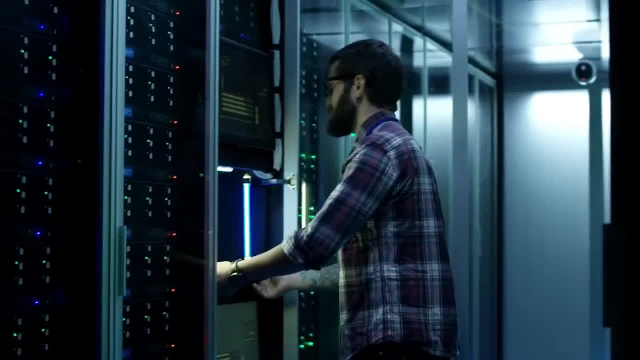 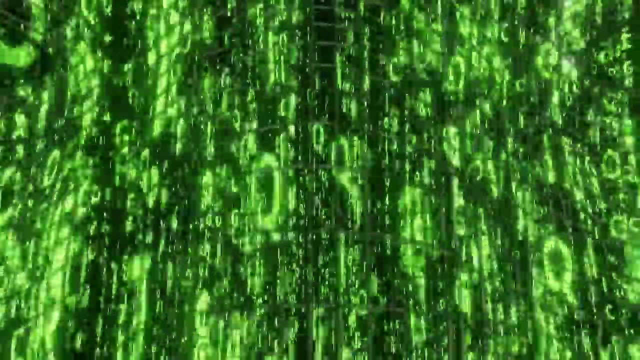 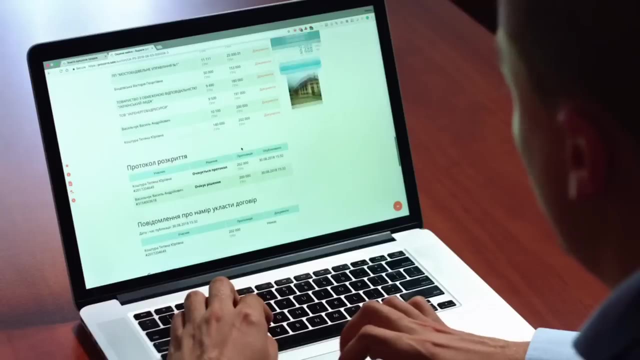 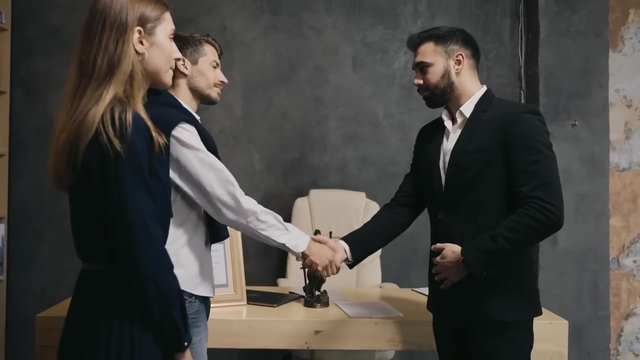 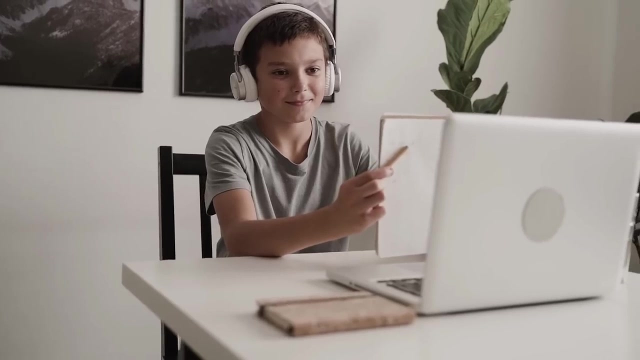 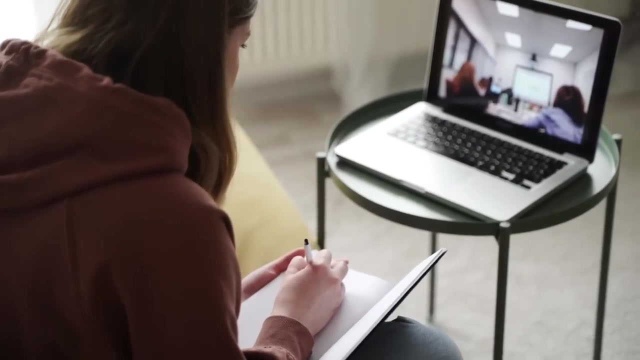 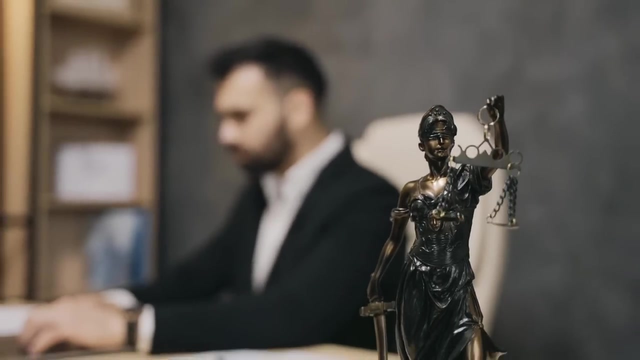 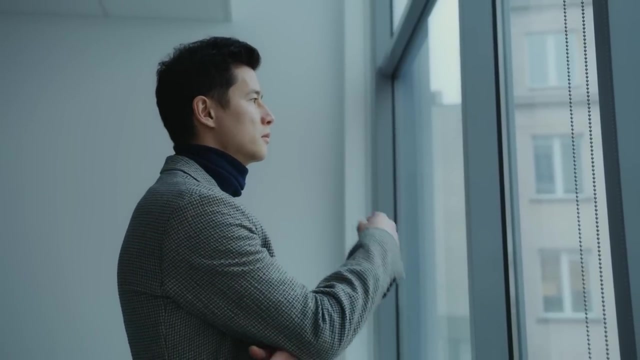 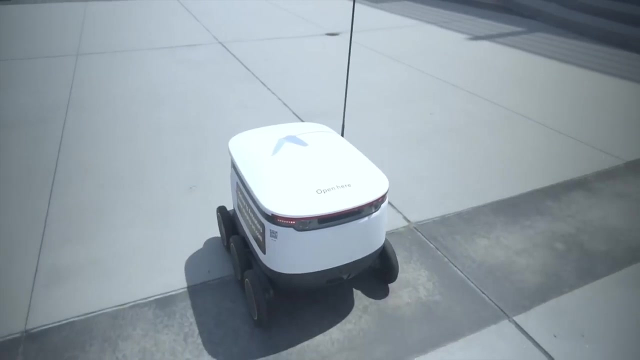 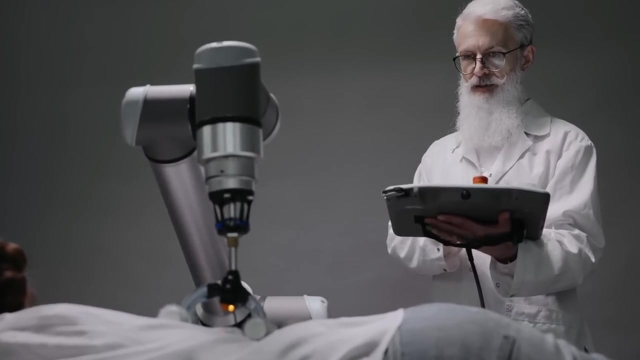 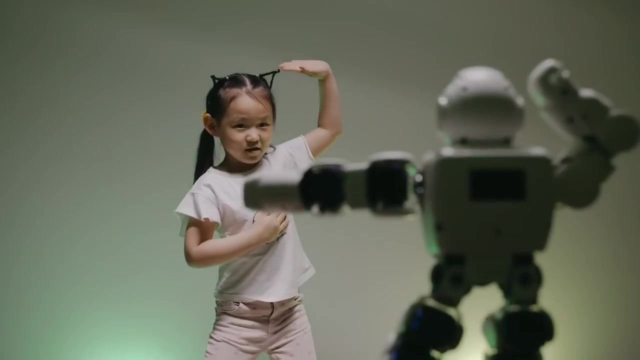 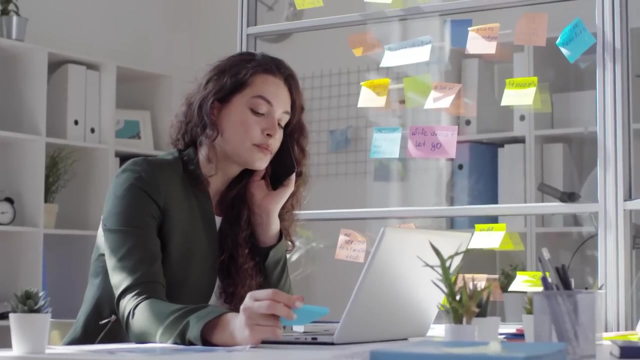 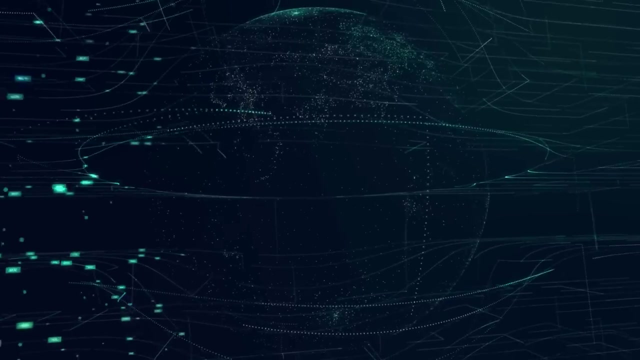 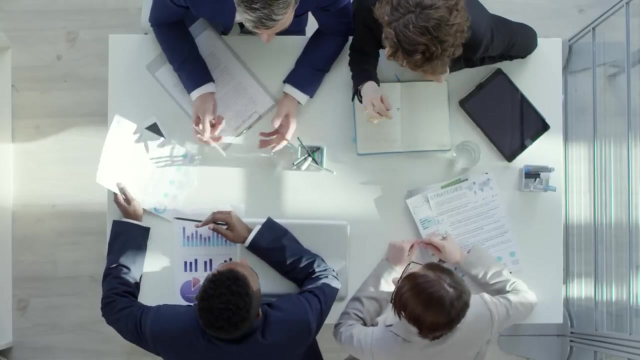 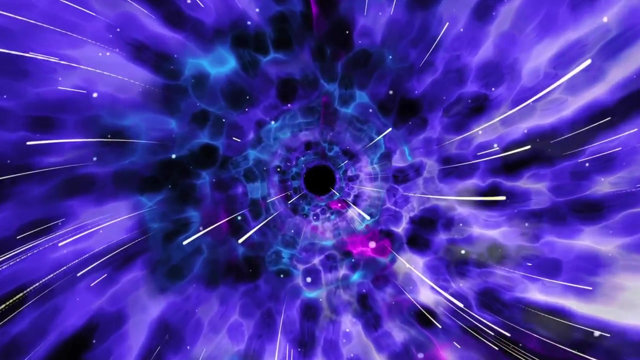 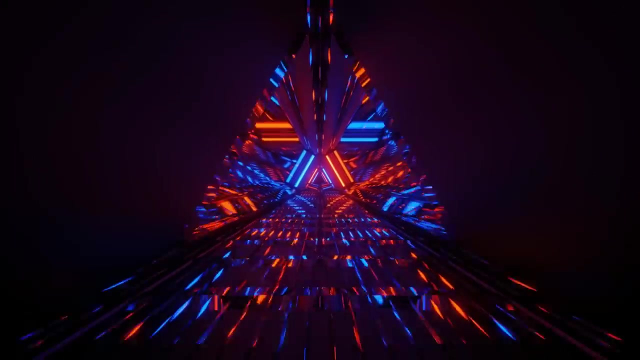 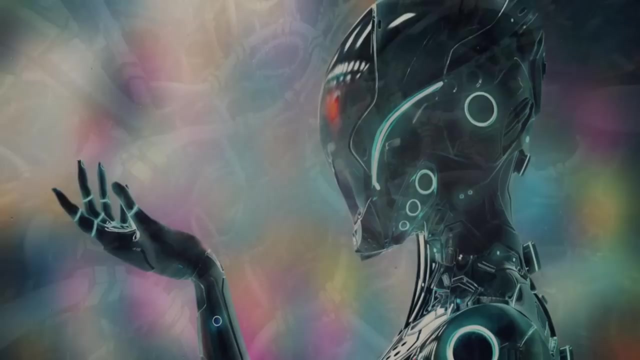 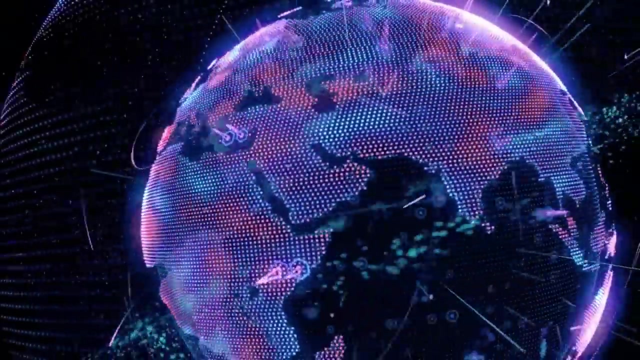 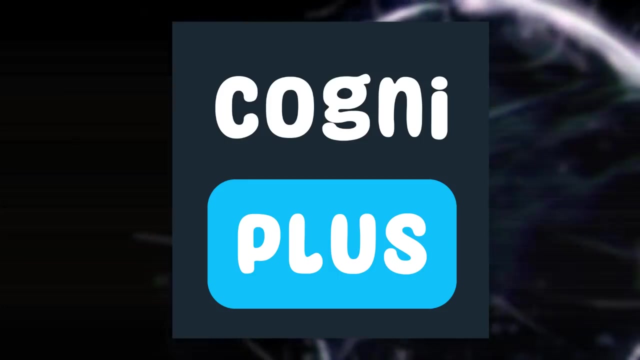 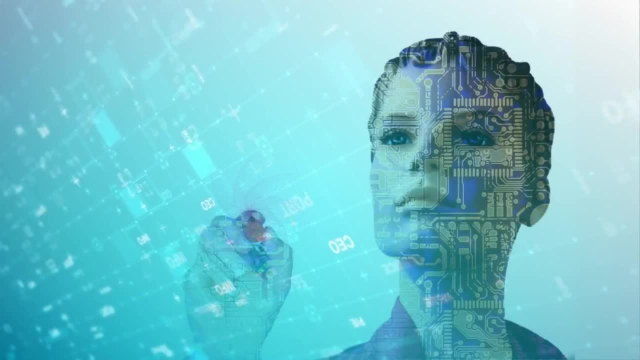 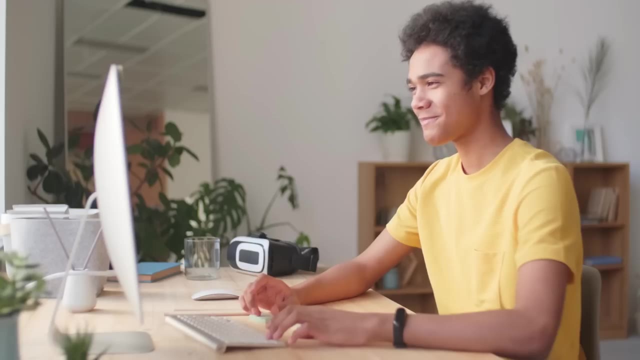 expert in this field. This comprehensive course on the CogniPlus app covers a wide range of AI topics, from the fundamentals to the most cutting-edge techniques. You'll gain hands-on experience and build your skills with real-world projects, while learning from top-notch instructors who are passionate about AI. 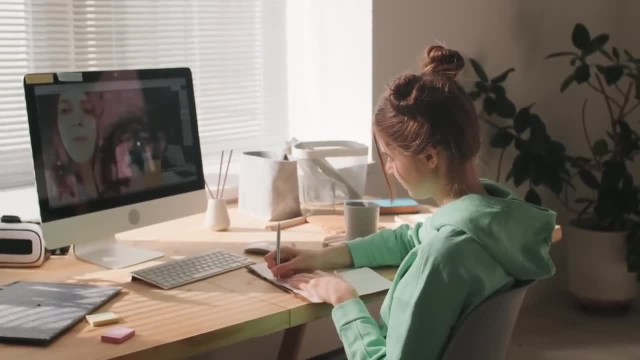 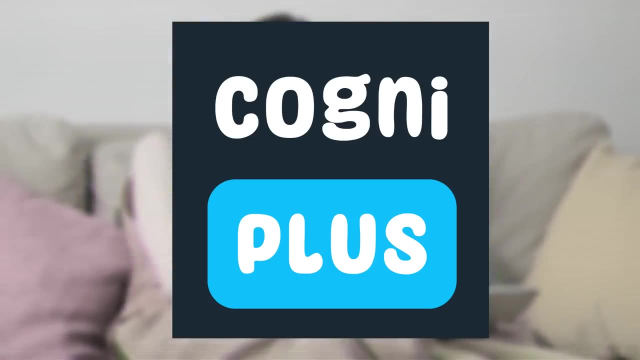 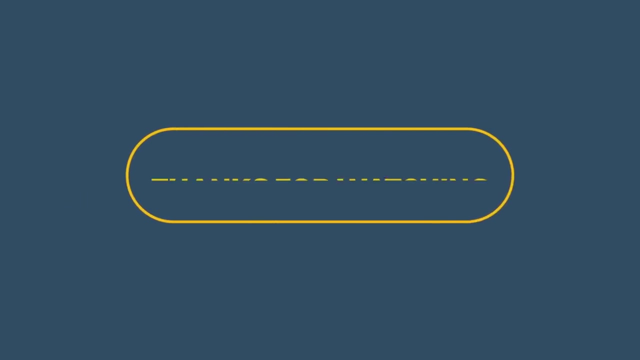 Don't miss this opportunity to enhance your knowledge and unlock your potential in the ever-evolving world of artificial intelligence. Download the CogniPlus app today and embark on your journey towards AI mastery. You can find the link in the description. Thank you so much for joining us in today's video.